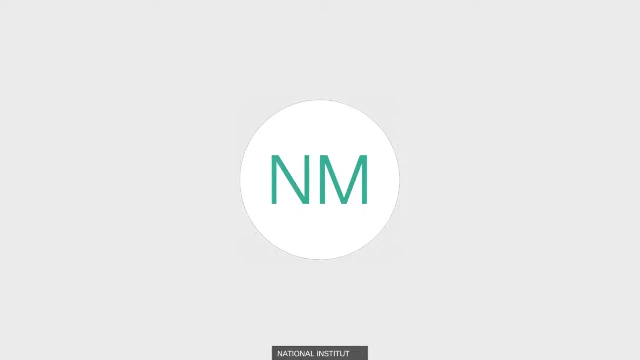 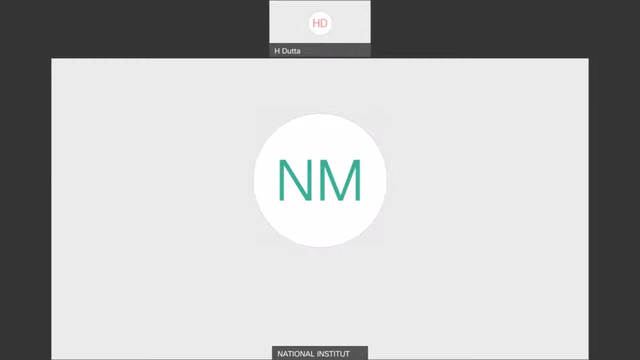 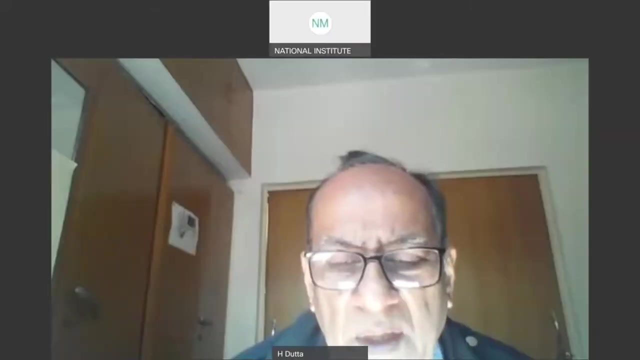 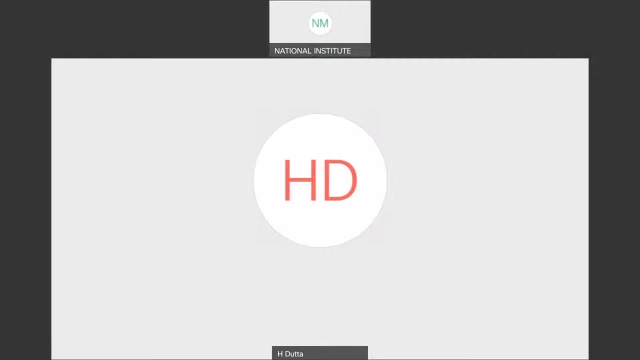 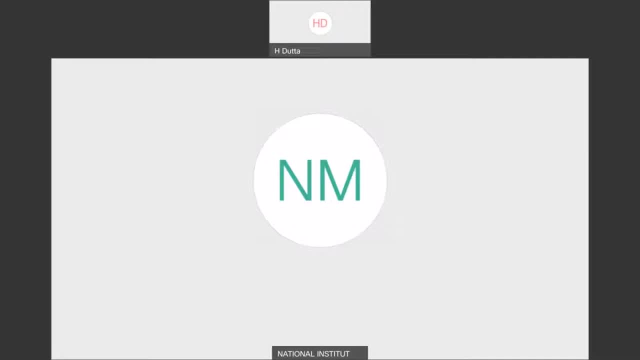 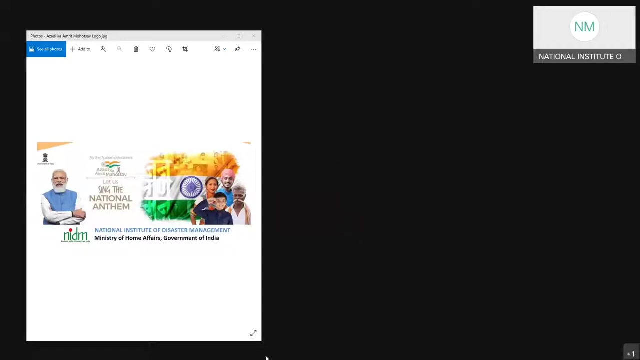 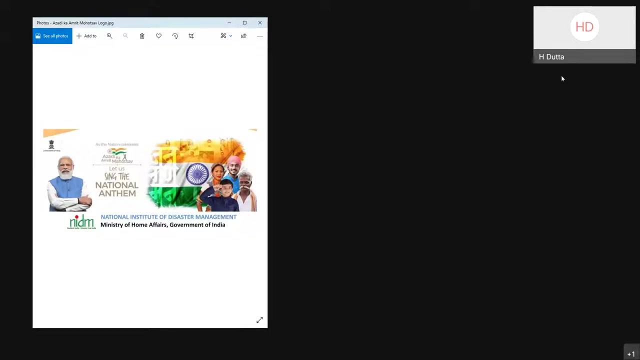 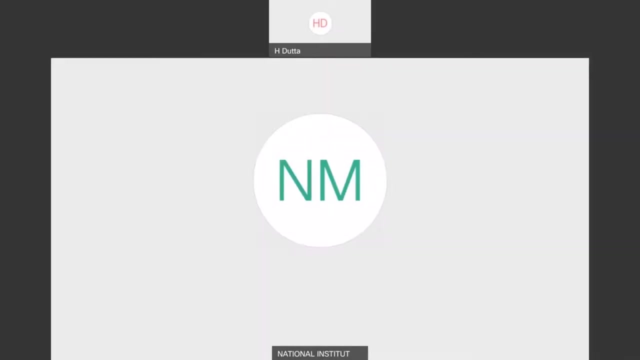 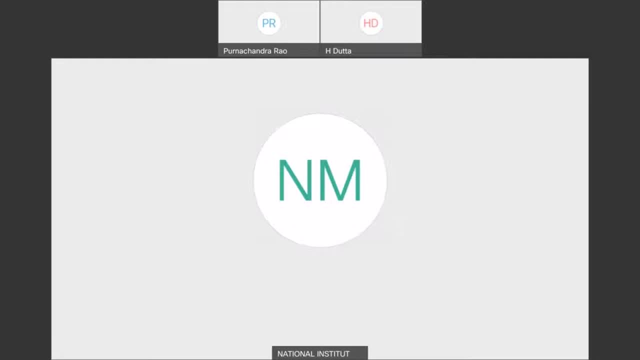 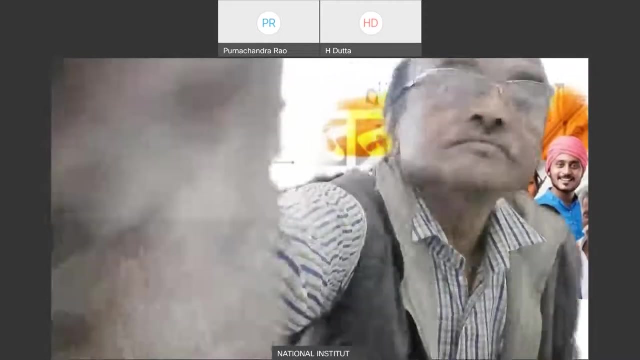 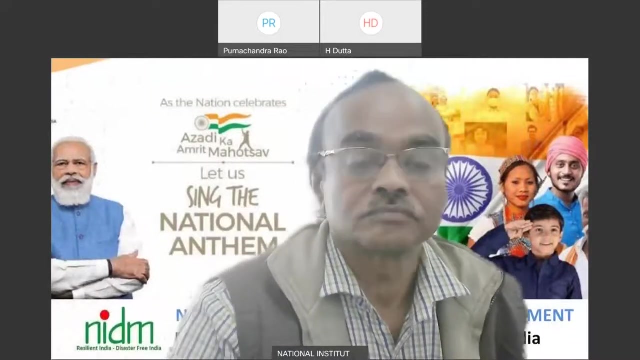 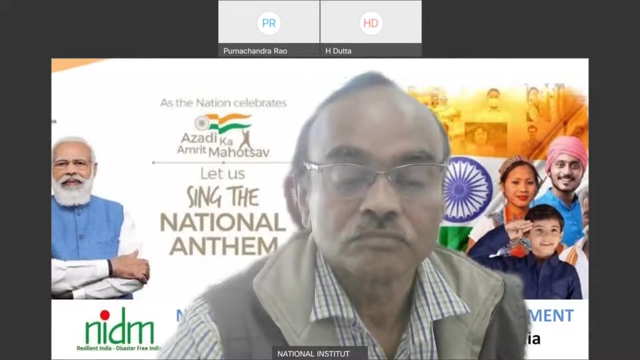 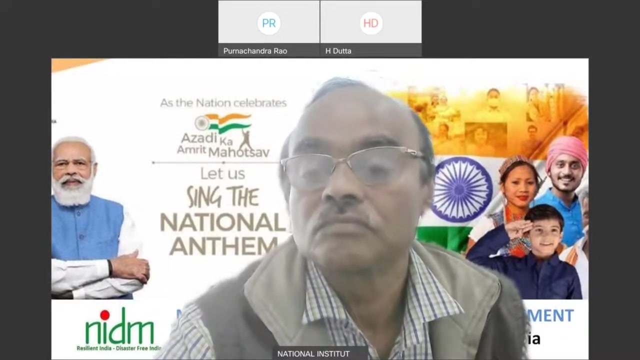 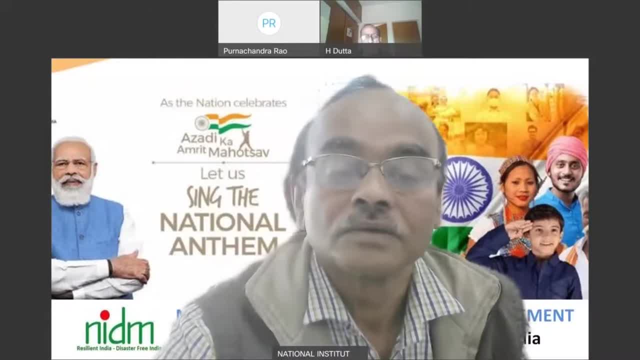 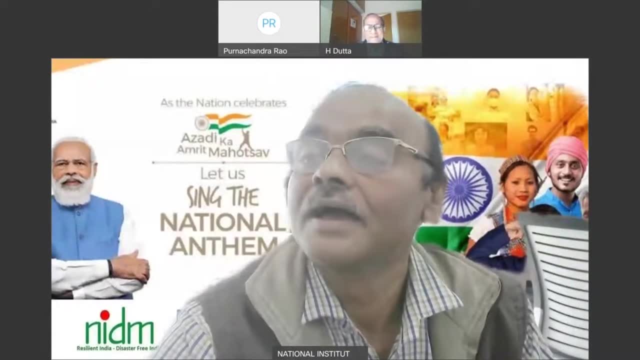 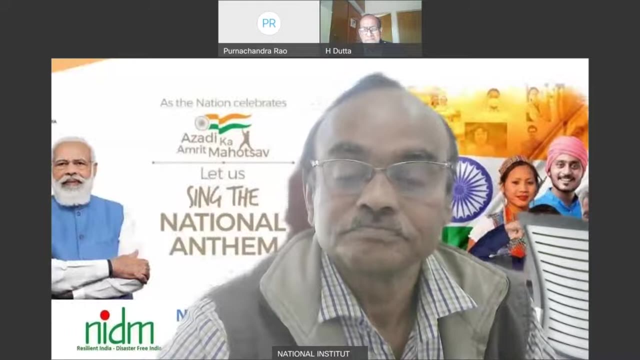 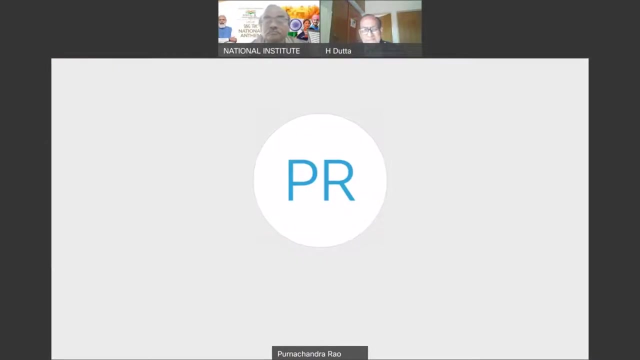 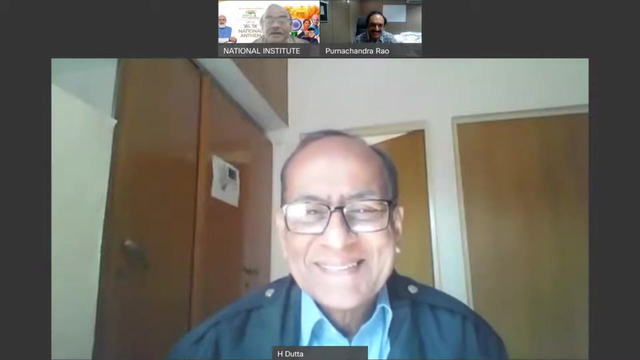 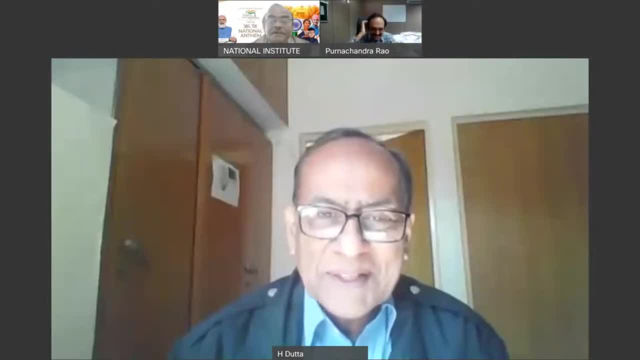 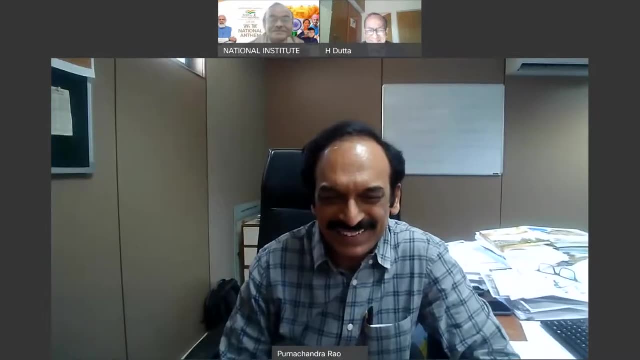 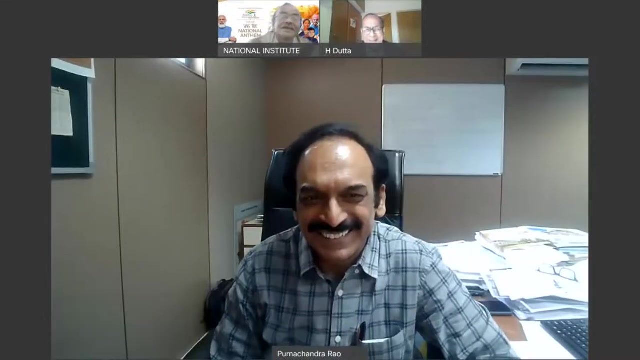 Thank you. In fact, I'm pleased that you are going to speak before I will speak. Oh, I see That will take care of a lot of many things you know. Oh, I hope so, But sorry, I'm sorry for the last minute change here. Oh, come on, I'm sitting at home, Okay. 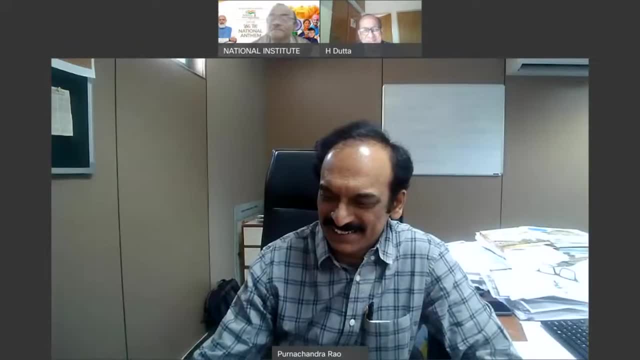 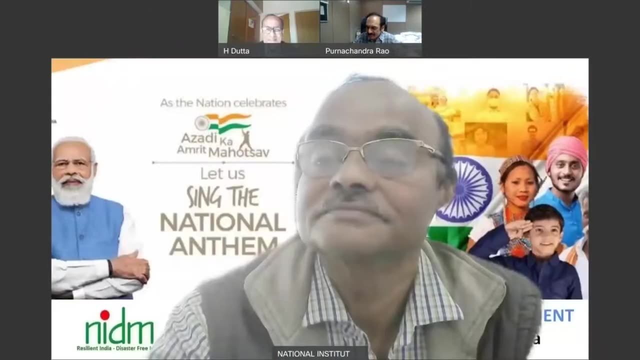 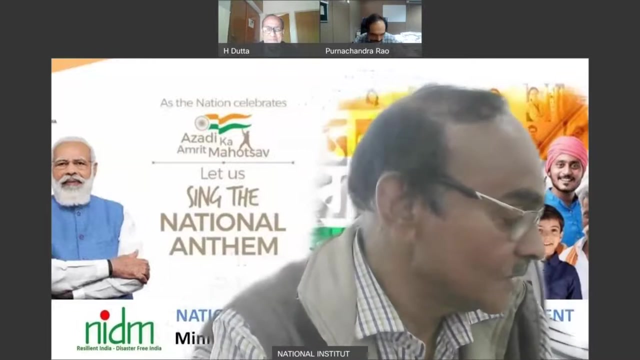 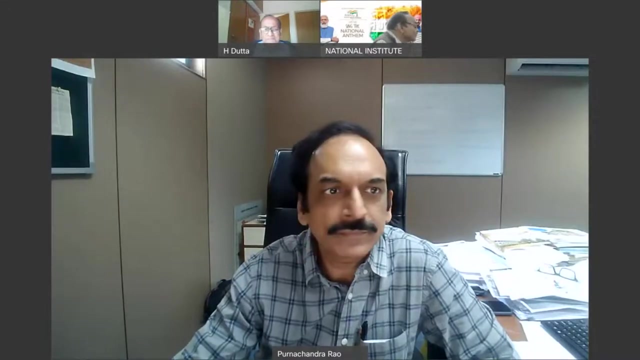 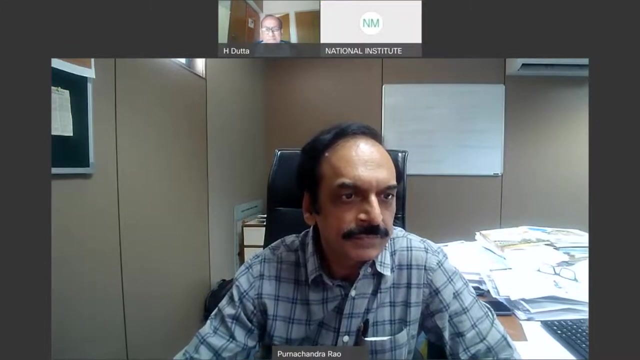 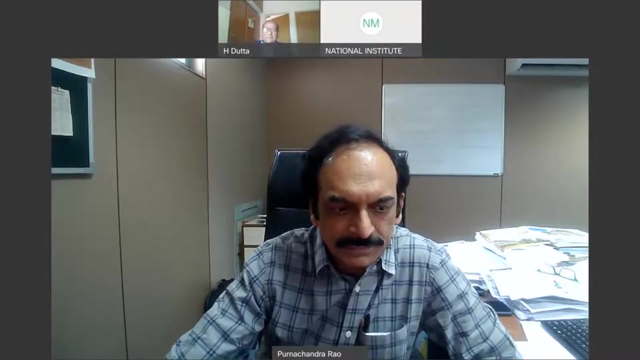 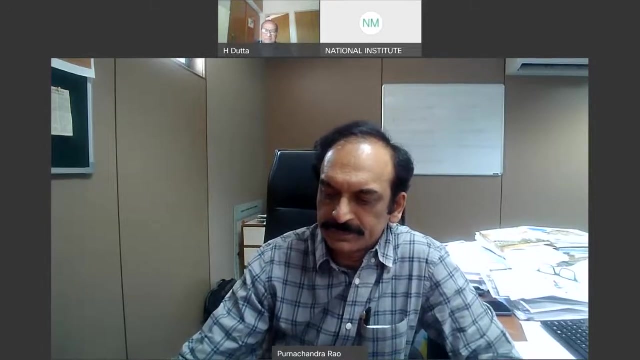 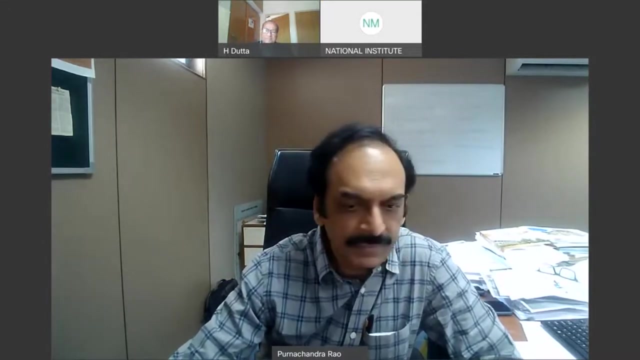 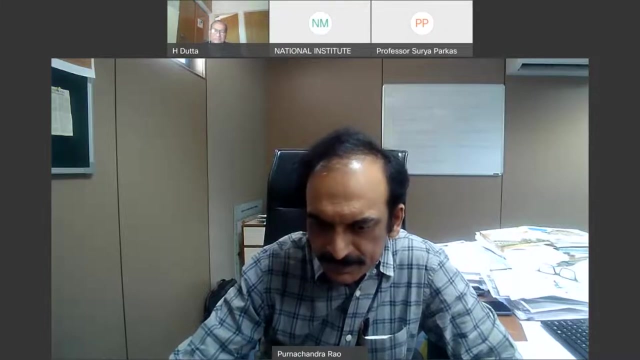 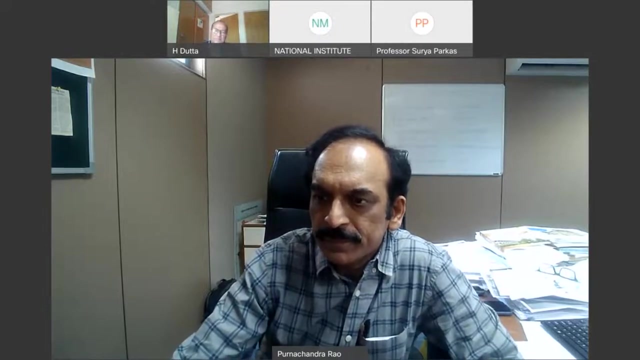 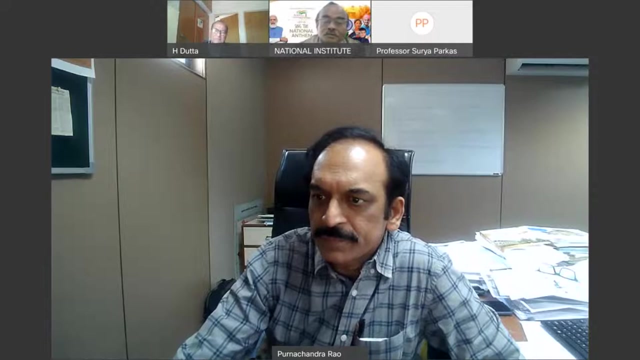 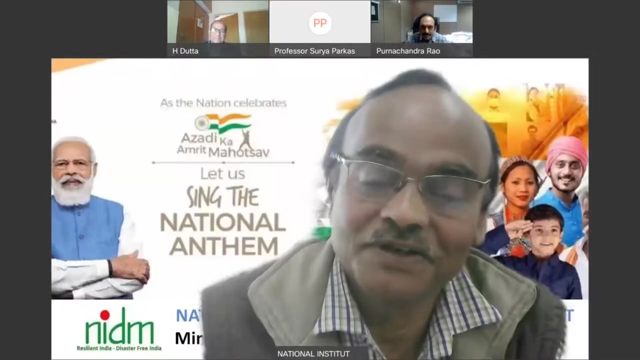 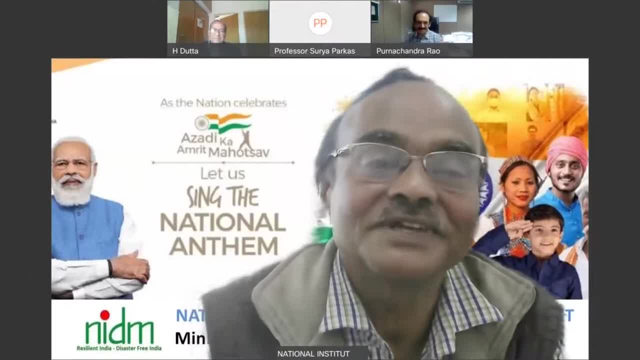 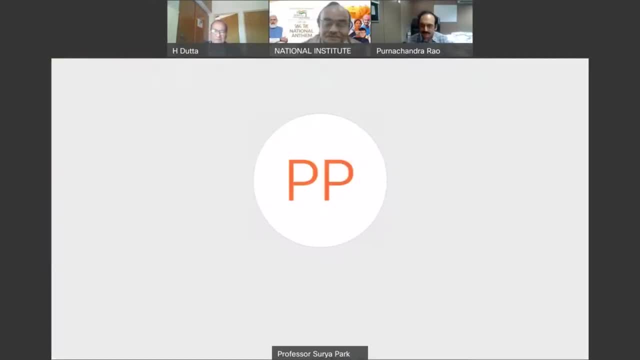 So now, uh, we can start, because, uh, there is a little hurry for Dr Z, So he'll be busy after the section for their his own activity in science. Now, shall we start right now, sir? Yeah, please, Please. 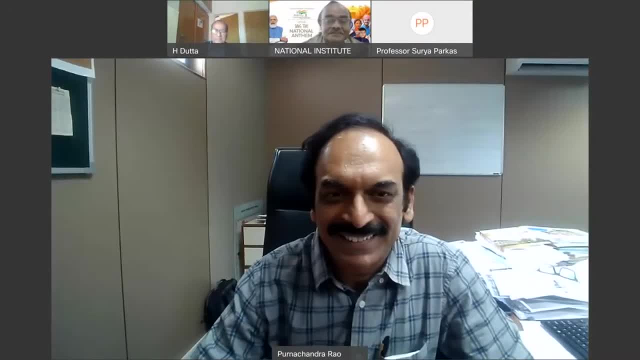 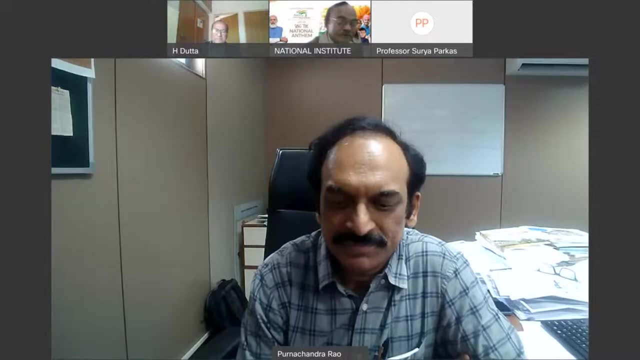 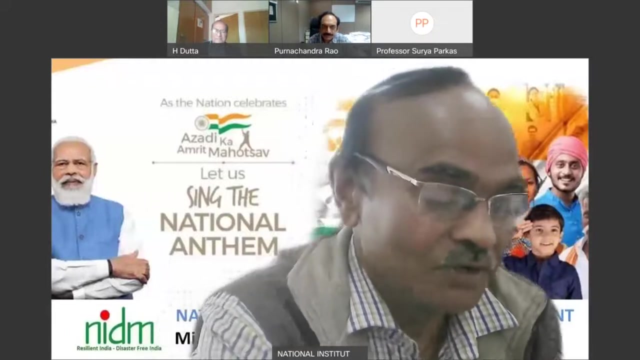 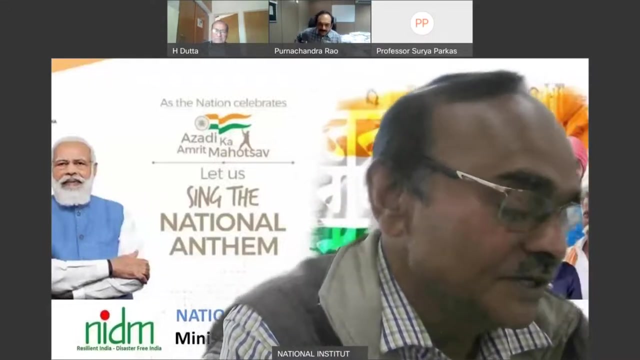 Good morning professor, Good morning sir. How are you? I'm fine, Thank you, Good morning everybody. Now in the series of webinar, today we'll be conducting that webinar from in the topic earthquake precursor detection in the Indian context. 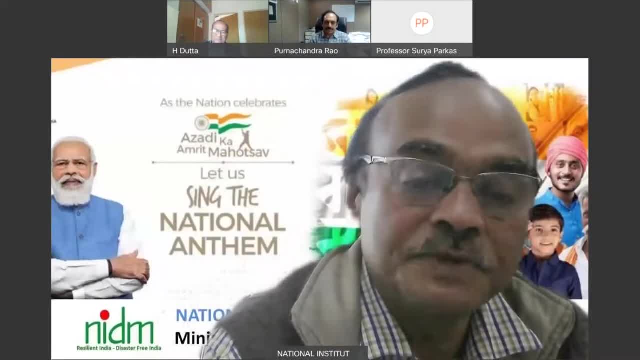 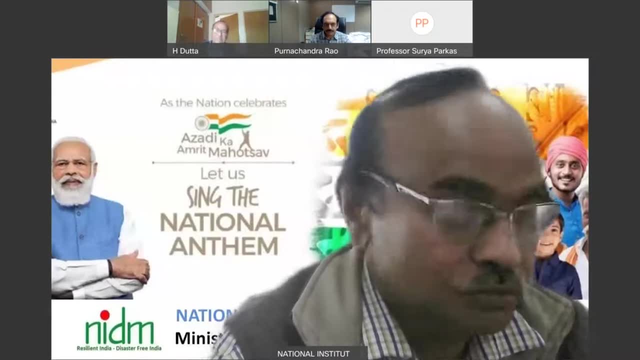 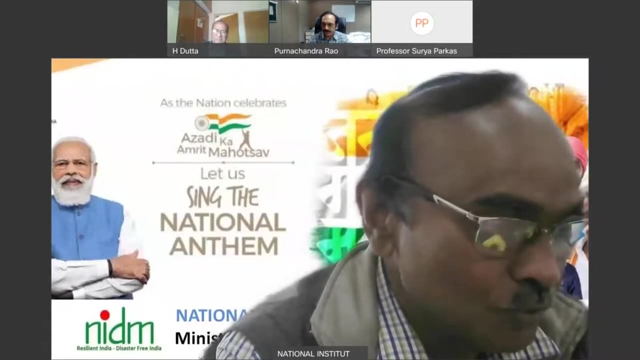 So in this series there will be two speakers: Professor H N Dutta and Dr Puranchand Rao. Now, due to certain things, that we'll be starting the lecture with Dr Puranchand Rao, Chief Scientist NGRI. 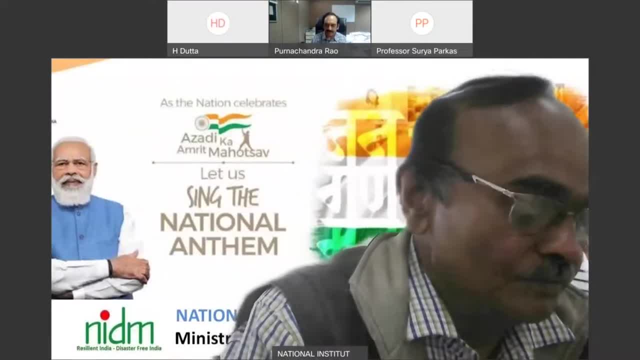 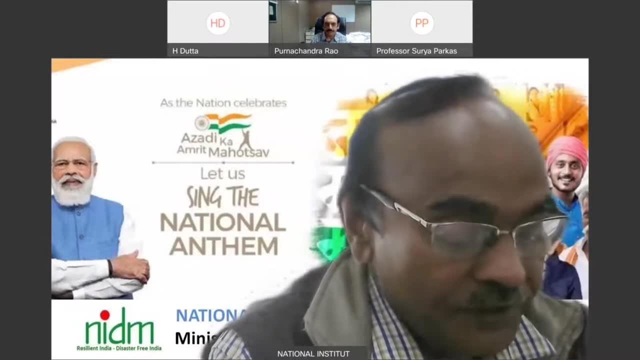 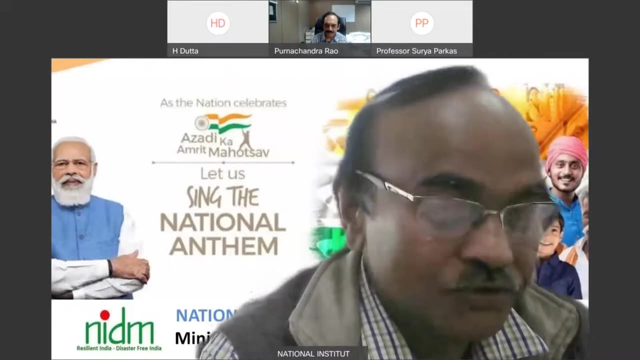 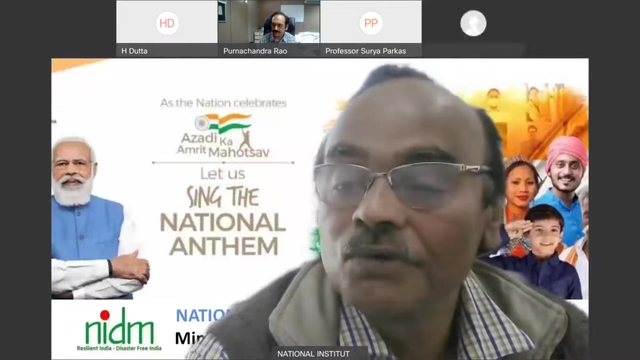 Now, before that, I would say a few words about the introduction and welcome. So I heartfelt And as well as I welcome from my core of heart to all the distinguished speaker and our head, Professor Srivastava, and all the panelists and as well as the participants who have joined quite a long back. 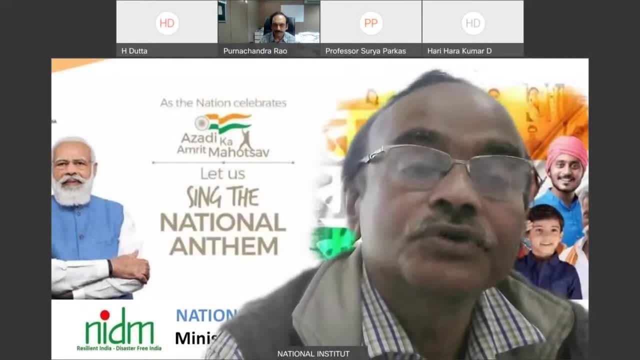 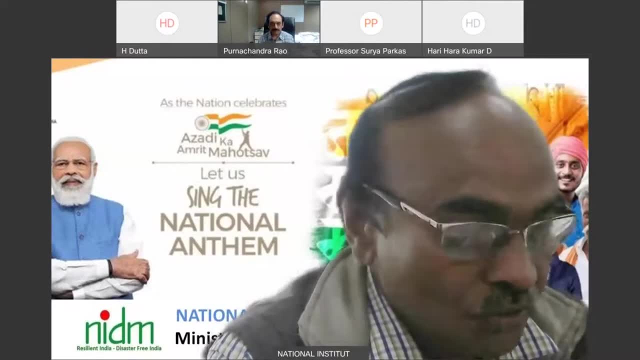 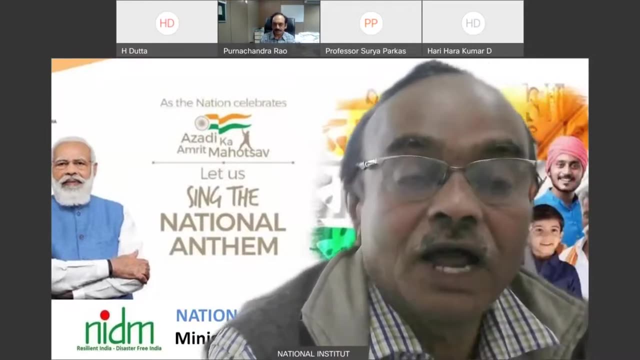 And it is a pleasure to us that we'll be having the good participant right now. a good amount of participant has joined. Now we'll still wait. Still, we are expecting some more participants And now we know in the context the earthquake. it is a very devastating phenomena due to sudden movement. 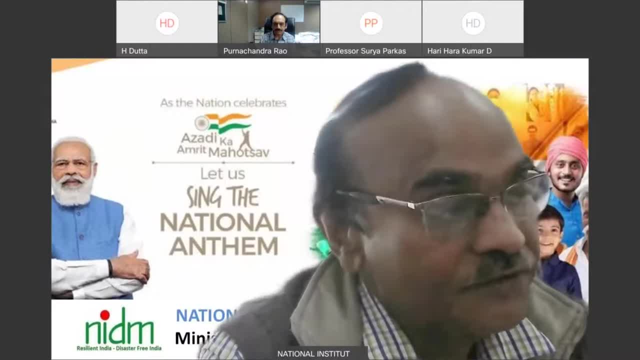 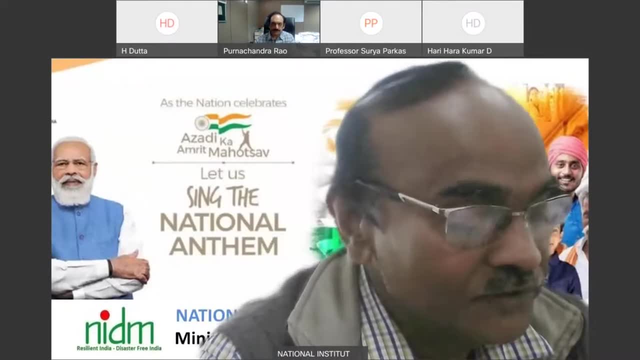 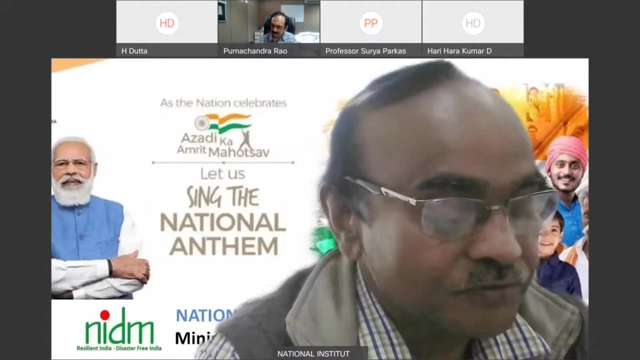 Our tumbling of the arts due to the insight that is the code from court, certainly instantly some energy used to release and that will give the jerk in the surface of the earth, and also due to the movement of technically plates That also creates sex in the ground and 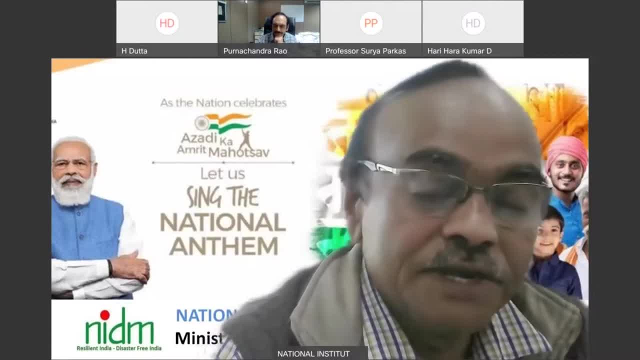 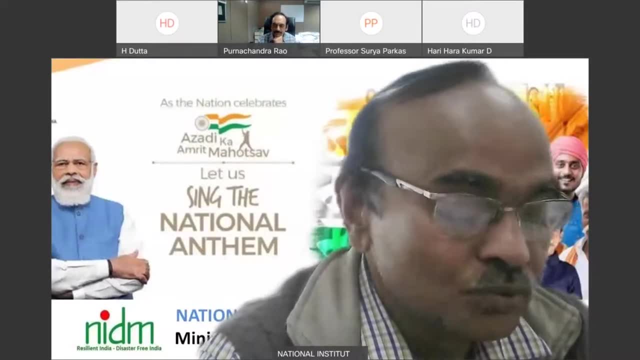 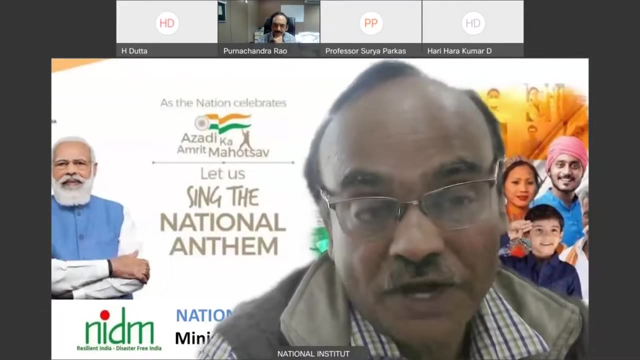 Causes. earthquake, as well as tsunami, is also very common phenomena, not obviously all the times, but it is a great devastation due to the sudden release of energy from the inner core of Earth, And this seismology is a study about the cause and repeat, type, size of earthquake and earthquakes. 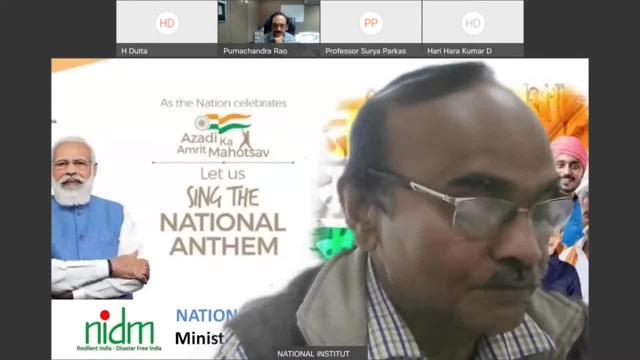 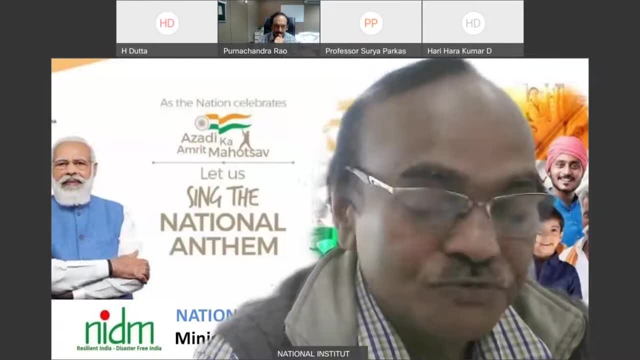 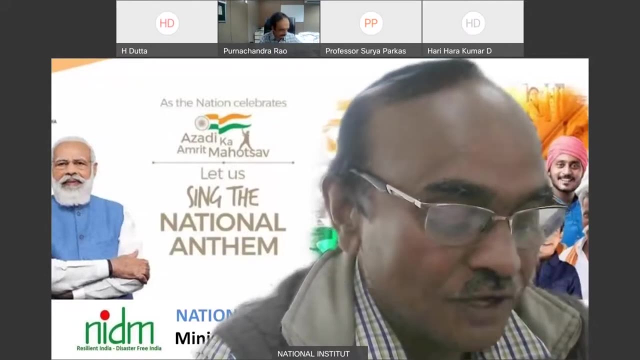 are measured using watching from seismogram. Now, the seismogram is a record of ground motions caused by seismic waves from the earthquake. A seismograph, or seismometer, is the measuring instrument that causes seismogram. Almost all seismometers are based on the principle of inertia. 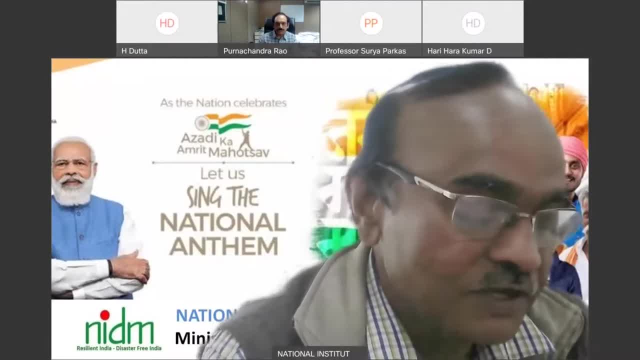 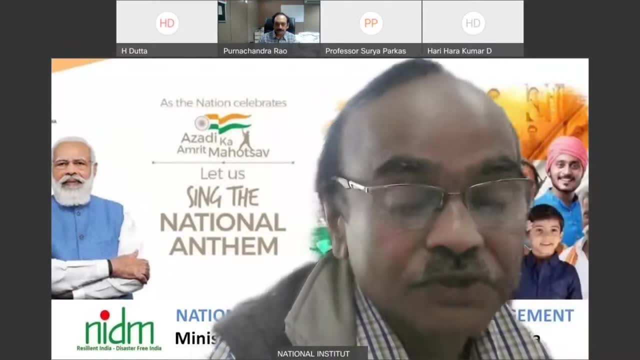 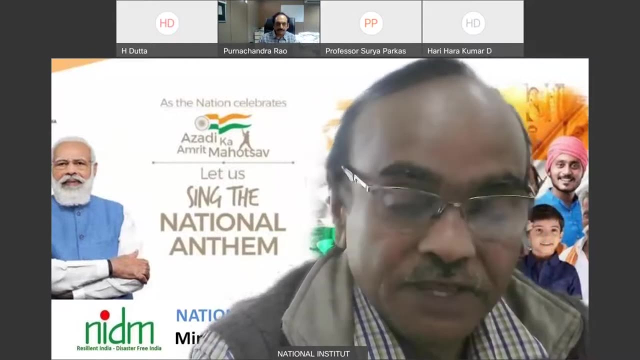 That is where a suspended mass tends to remain, still when the ground moves. So very few words I will say, In keeping in view the time constraint. earthquake prediction is a popular topic among the scientists. However, this task is challenging and exhibits uncertainty. 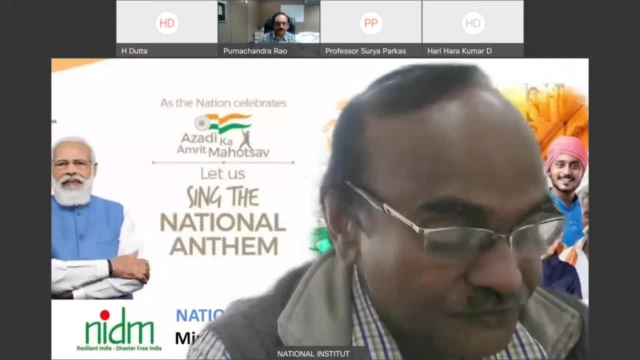 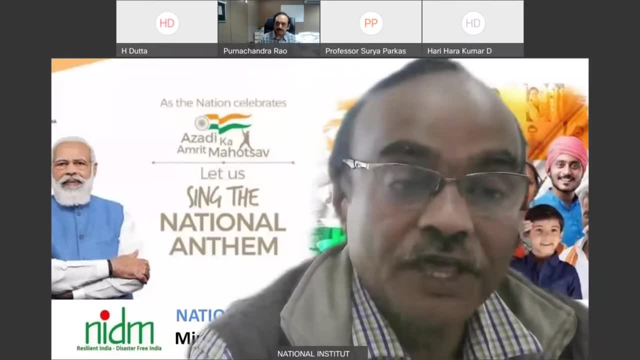 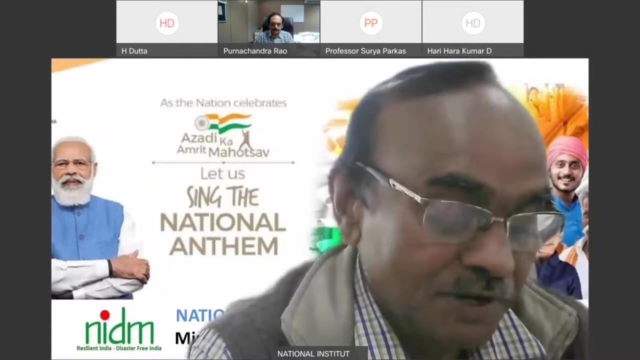 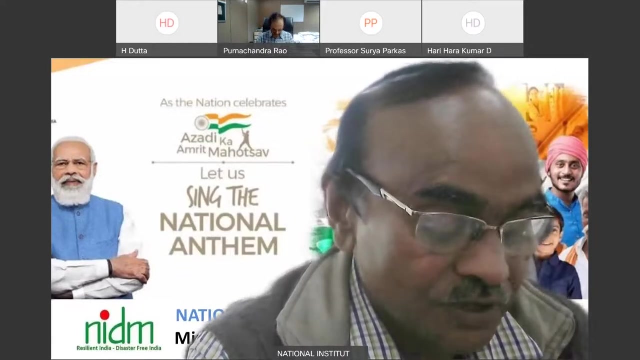 Therefore, probability assessment of indispensable in the current field. during the last decade, the volume of seismic data has increased exponentially, adding scalability issues to probability assessment model. Several machine learning methods, such as deep learning, have been applied in the large-scale images. 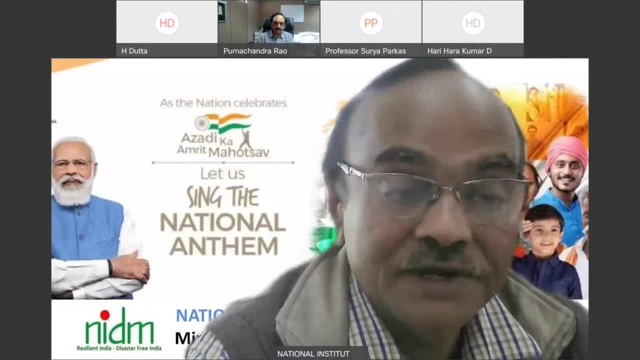 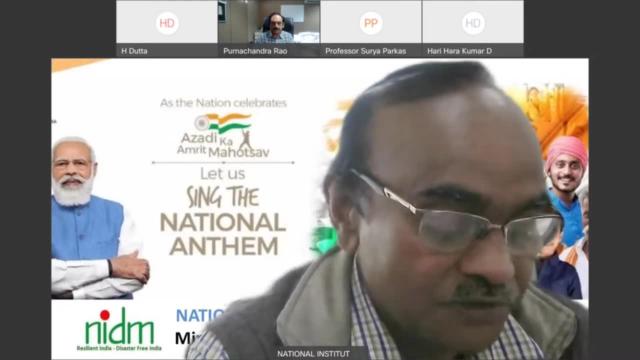 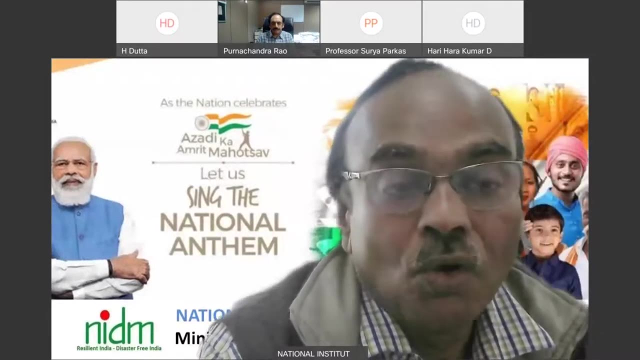 Video text processing. however, there have been rarely utilized in earthquake probability assessment. Therefore, it is need of research leveraged, advanced in deep learning techniques, to generate scalable earthquake probability mapping. Also, a lot of work is going on in the India's leading 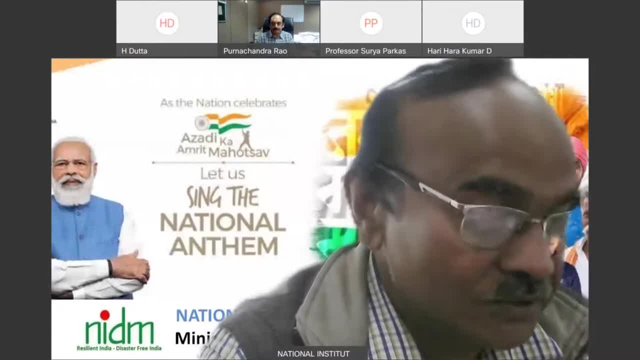 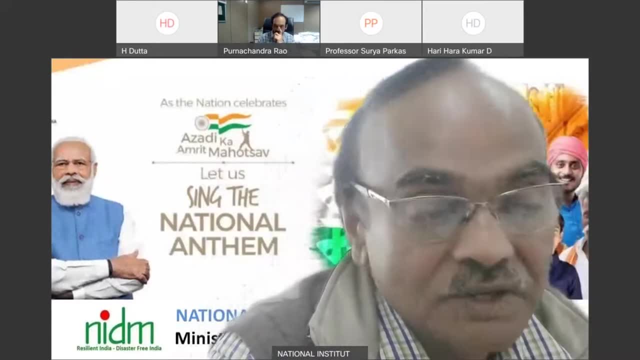 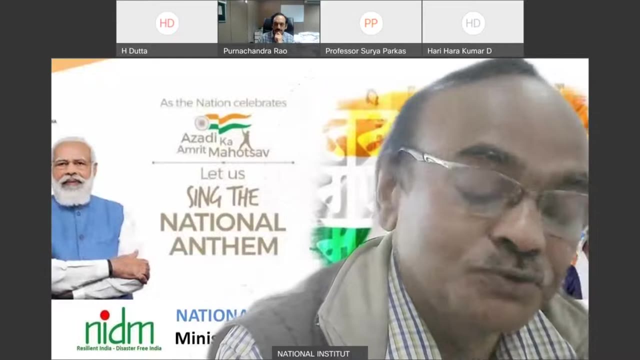 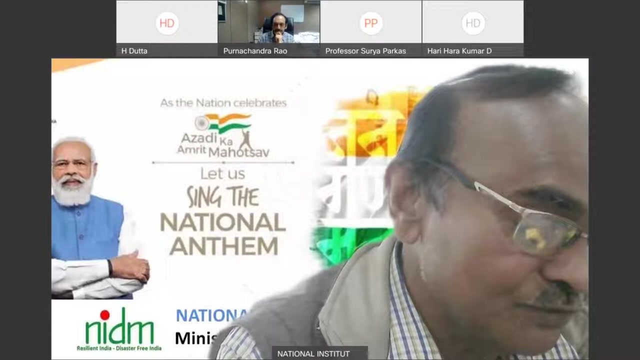 organization, NGRI, and other organizations that are doing, And also that among the pet animals, that is, dog bar, they'll be, since before this type of events, Even the animals are able to detect the past, Why animals have been seen snapping to attention. 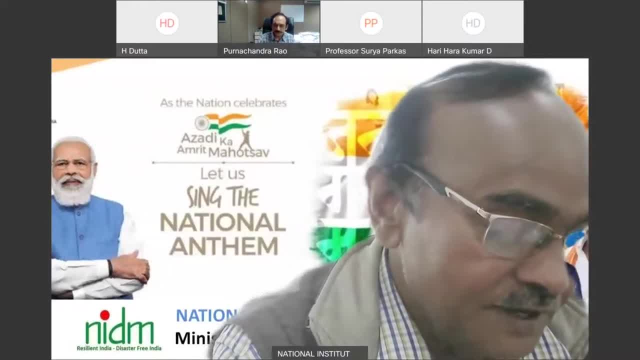 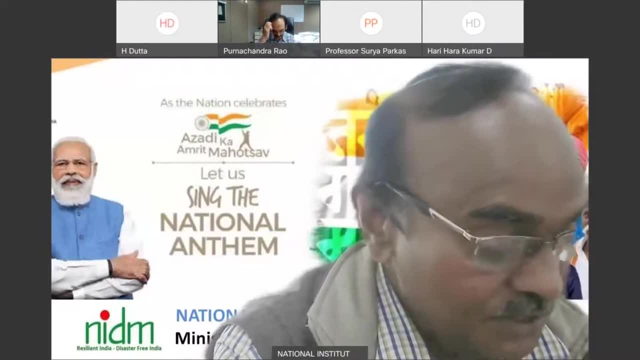 Okay, So the dog is acting confused, running right before the ground starts to shake. They used to grudge, And even the dogs. they are having very much sensitivity for smell and hearing And they can. they have the heightened sense of what I am telling: smell and hearing. With their heightened sense, they can tell when there's a change in barometric pressure, which changes with different weather patterns. So dogs know when the pressure is changing, because scent will either travel faster or slower with the changing pressure. Now, as for the dog owners, the key factors reported by the owners who have witnessed 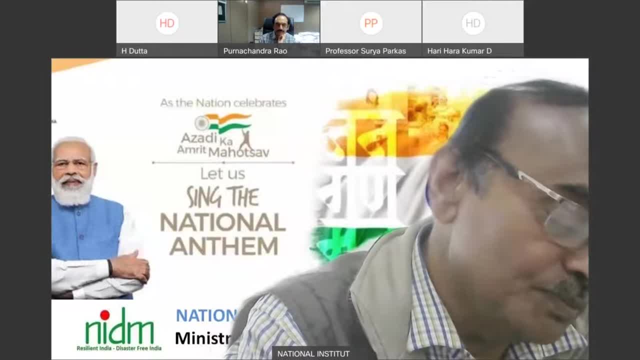 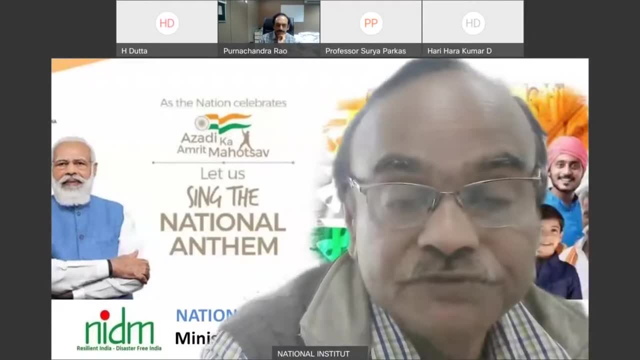 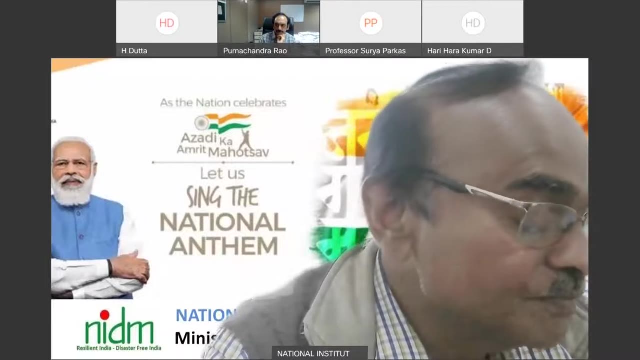 their dogs acting out of the ordinary. out of the ordinary before the earthquake is simply taking place and abnormal changes behavior in their pets. This could be an average in dogs' community activity levels: heightened anxiety, barking, weaning and even trying to escape or leave. 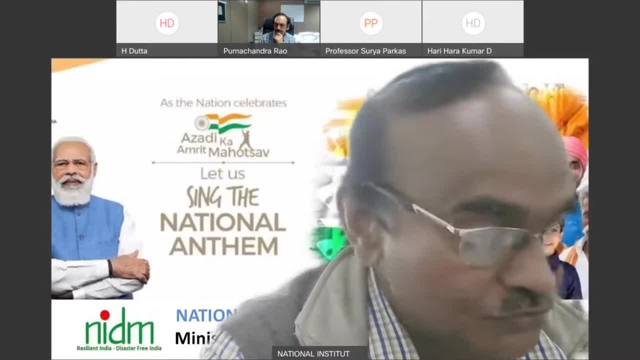 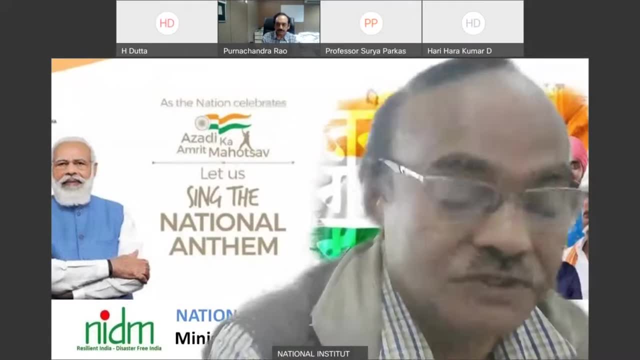 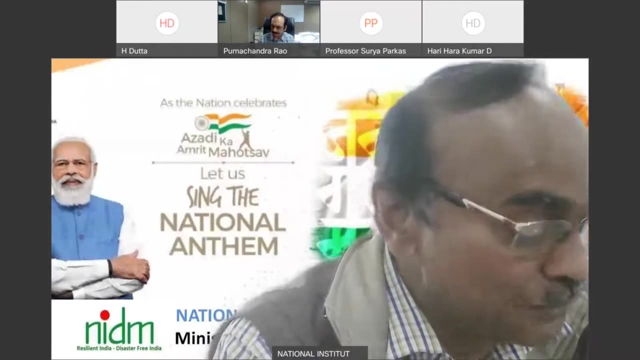 So these are the certain things that they also sense, and they have to give the symbol before the disaster. Now I will not go further. Before our eminent speakers are there. they'll speak a lot about this, I expect. Now, before I hand over to the speaker, I will request our professor to speak. 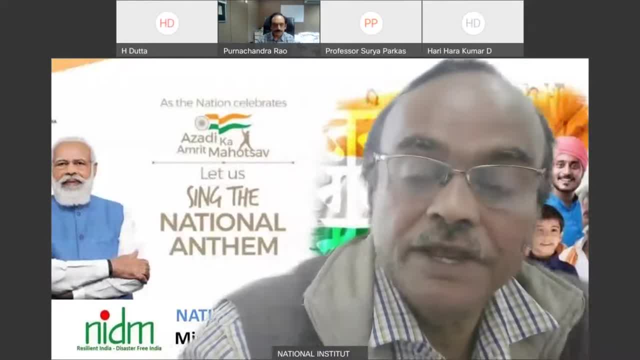 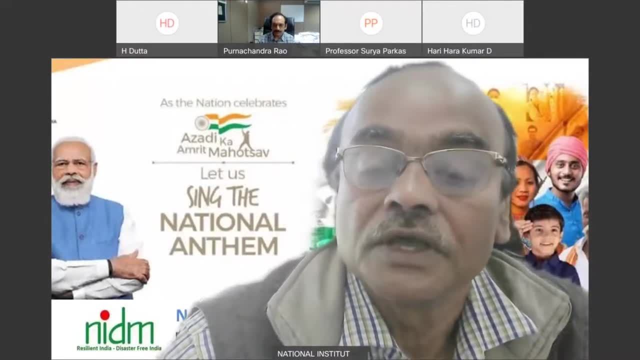 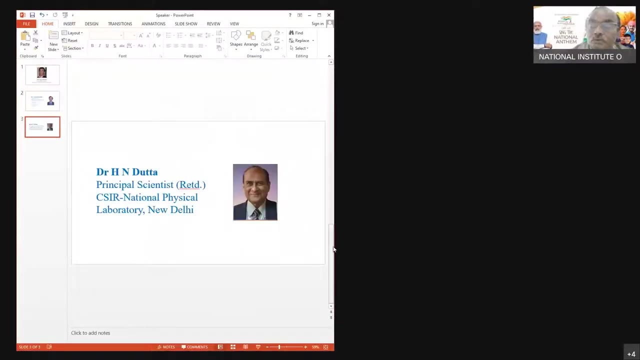 Okay. So this is the first time we're seeing a keynote at this in this issue. Now I will introduce this, Dr. Just one second. I think it is visible. sir, This is your slide. Yes, Yes, Okay. 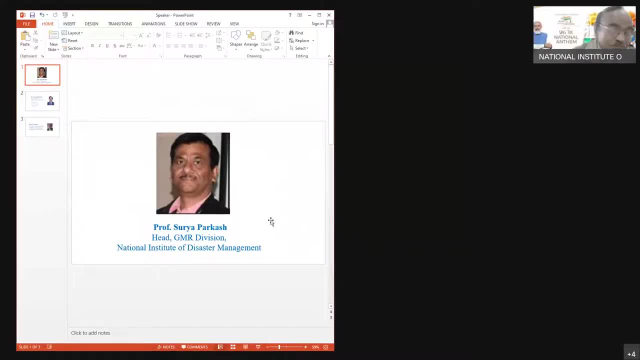 Now Professor Sudyaprakash. he's presently speaking. Yes, it is. Yes, He's currently working in this NIDM, National Institute of Disaster Management, as head in GMR Division. He is a nodal officer for coordinating with central ministries, departments of disaster risk management-related planning, research and capacity building for Ministry of Mines, Ministry of Coal, Ministry of Petroleum and Natural Gas, Ministry of Communication, Ministry of Shipping Ministry and Department of Northeastern State Parliamentary Affairs, News and Renewable Ministry of New and Renewable Energy. 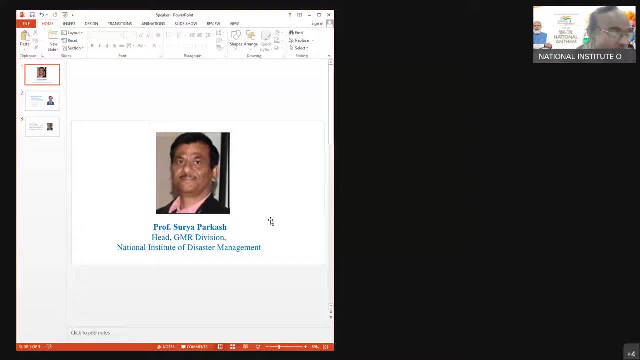 Labor Employment and National Postal Academy. He's the faculty in charge in six specialized centers, that is, Army Winding and Communication, Hill Area Development, Coastal DRR and R CBRN, Industrial DRR and Cyber DRR. 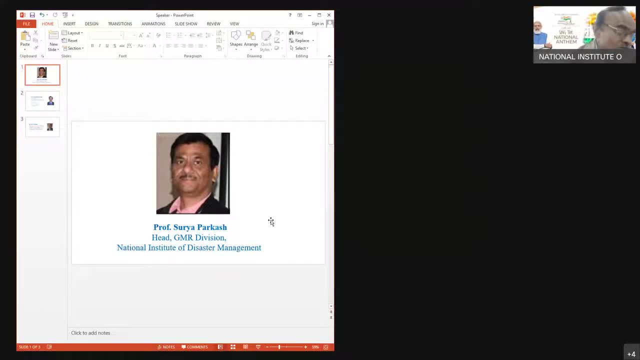 He is also team leader in World Center of Excellence in Landslide and Disaster Reduction from 2011 to 14, again 2020 to 2023.. He is also supervisor in charge of Flood Monitoring Cell and Emergency Operations Center. With this introduction, I'll request Professor Suryaprakash to take the stage and put his keynote at this. Professor Suryaprakash, please. 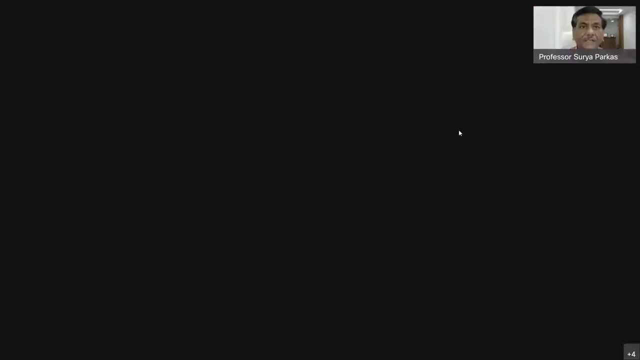 Good morning to all and thank you, Dr Haldar sir, for providing me this opportunity to speak today. Thank you, Dr Haldar sir, for providing me this opportunity to speak today. Thank you, Dr Haldar sir, for providing me this opportunity to speak today. 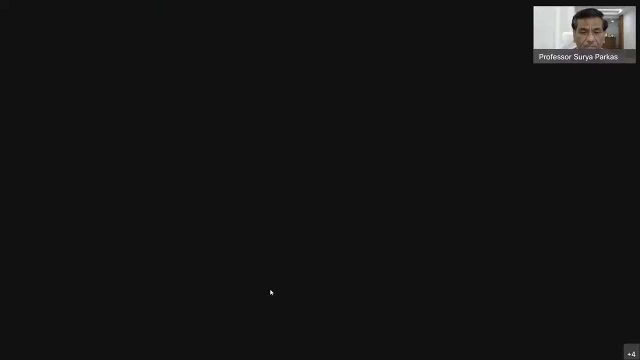 In the inaugural program. earthquakes, as most of us know, are very important hazards in terms of their widespread impacts, as well as the current state of our non-predictability, particularly in terms of temporal framework, and also the level of unpreparedness in terms of earthquake-resistant structures and infrastructures. Thank you. Thank you, A lot of earthquakes have happened in the recent past. I can recall from the historical figures we have been talking much about Uttarakhand, which suffered earthquakes way back in 1803.. And then 1819, Gujarat earthquake 1897, the Shillong earthquake 1905, Kangra earthquake 1934, Bihar-Nepal earthquake 1950, Assam earthquake, which happened on our Independence Day. 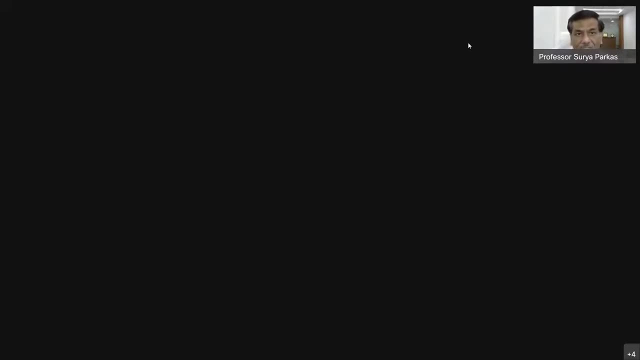 And then the recent ones. I can recall from 1990, since I've been involved with that earthquake, which happened on 20th October early morning in the Uttarakhand State, followed by another earthquake which took place in 1993 in Latur. And then in 1995, we had an earthquake in Himachal and in 1997, I remember Jhapalpur. In 1999, again the earthquake. And then in 1995, we had a large earthquake in Jhapalpur. And then in 1995, we had a large earthquake in Himachal, and in 1997, I remember Jhapalpur. And then in 1995, we had a large earthquake in Himachal, and in 1997, I remember Jhapalpur. 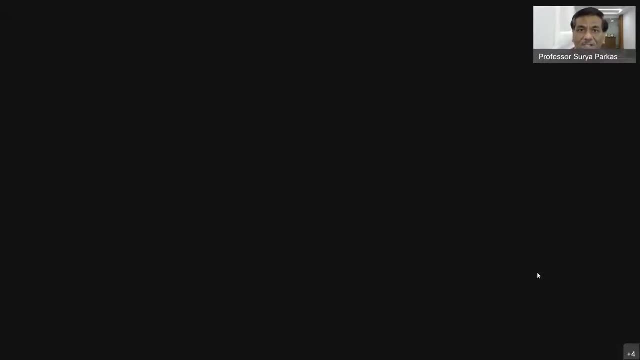 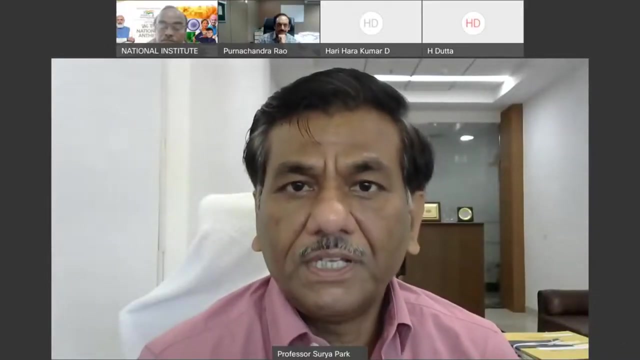 we had an earthquake in Chamoli and 2001,. 26th January, Republic Day- we had an earthquake in Gujarat, Kutch area, followed by another earthquake which took place in the Indian Ocean, Swamy, leading to the major disaster of loss of thousands of lives around the coast of the Indian. 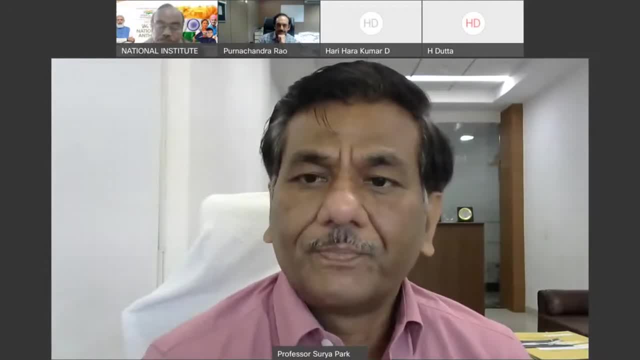 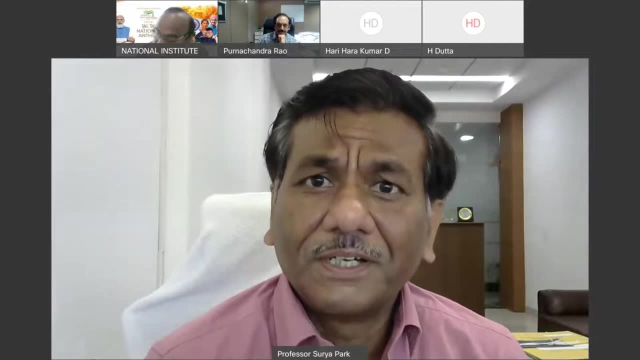 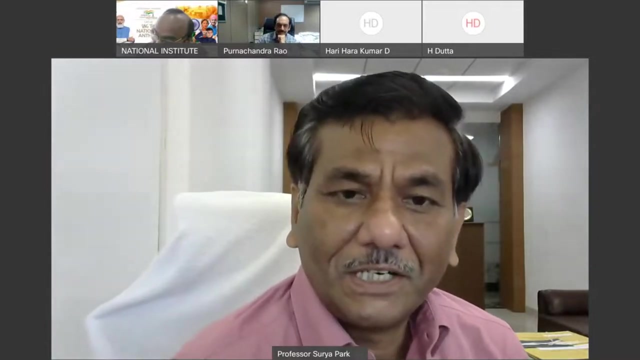 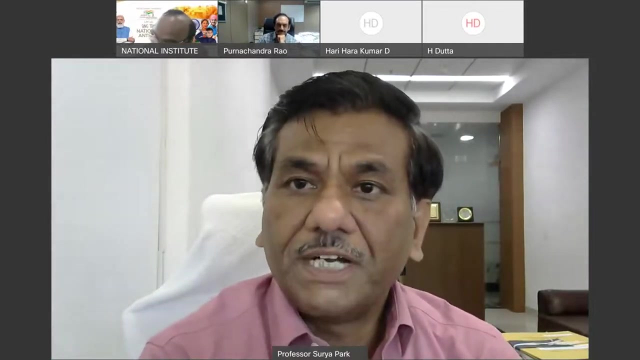 Ocean, affecting more than almost 11 countries, Then followed by another earthquake which happened in Kashmir- I think it was 8th or 10th October 2005,- and then we had an earthquake in Manipur in 2016,- sorry, 2006,- and then there were earthquakes which had happened in Nepal. 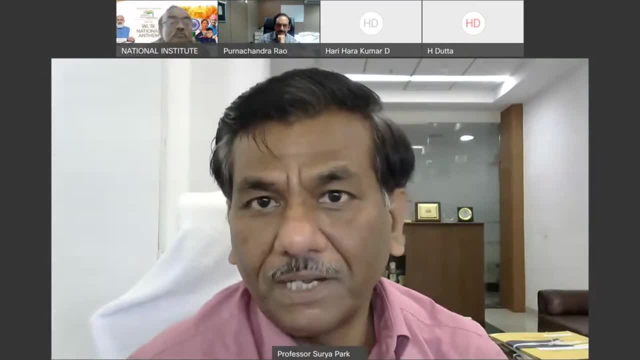 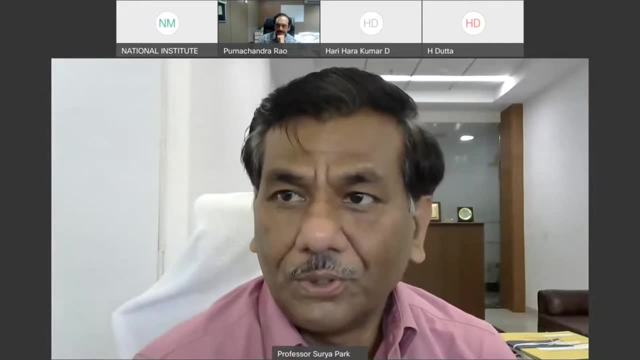 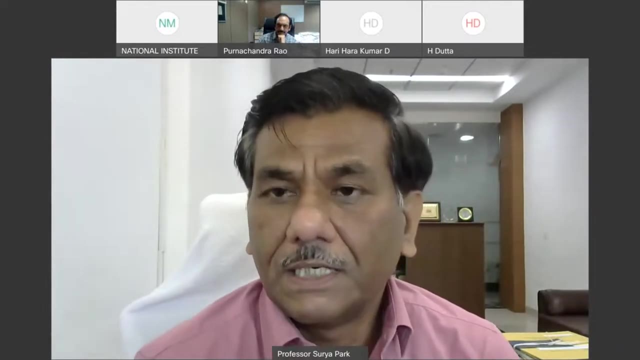 2015 earthquake also, which in April, and followed by another earthquake in May- 25th April and 12th of May, and so on- There was another major earthquake- I should make a mention of that, which is important for us- that earthquake which happened on 18th September 2011 in Sikkim. 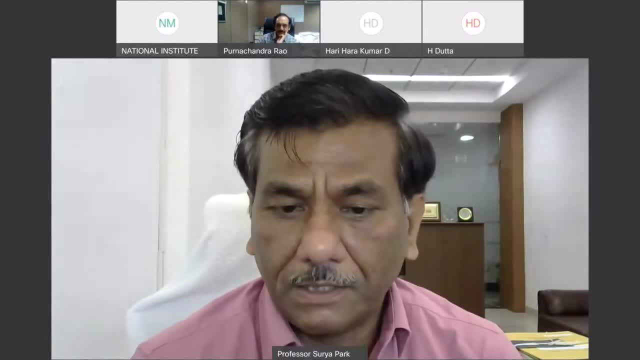 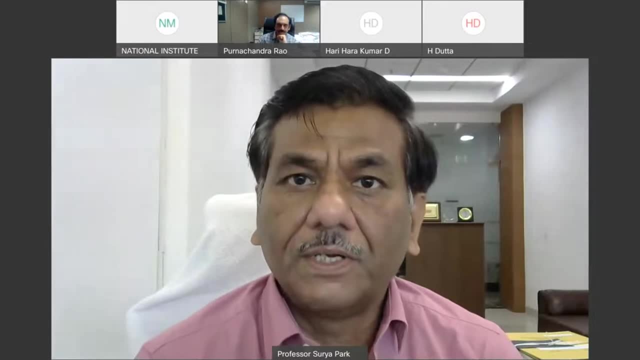 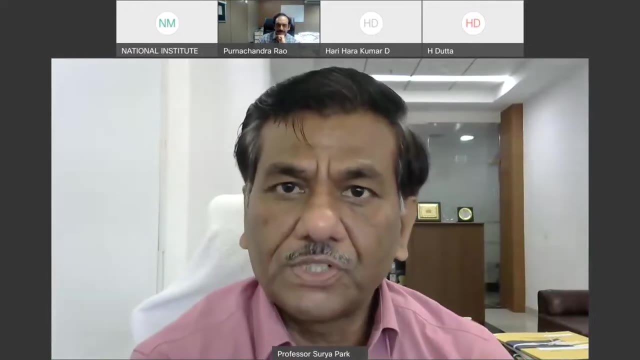 All these earthquakes which are actually happening in the Himalayan territories. they are not only just causing damages because of the structural damage or loss or destructions, but also leading to landslides- earthquake-triggered or induced landslides- which are actually blocking our 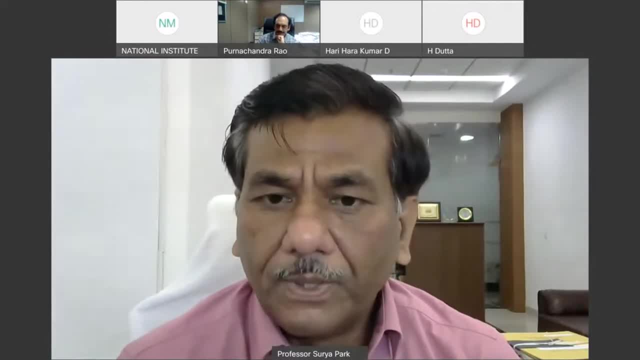 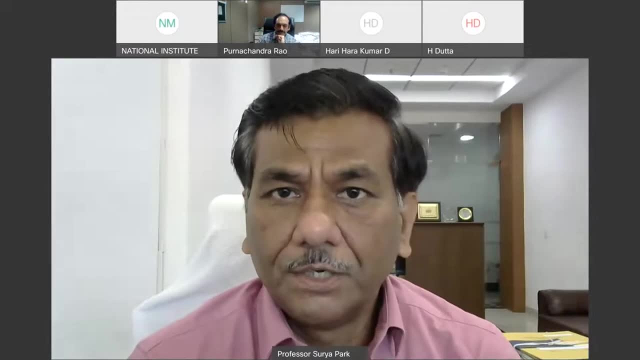 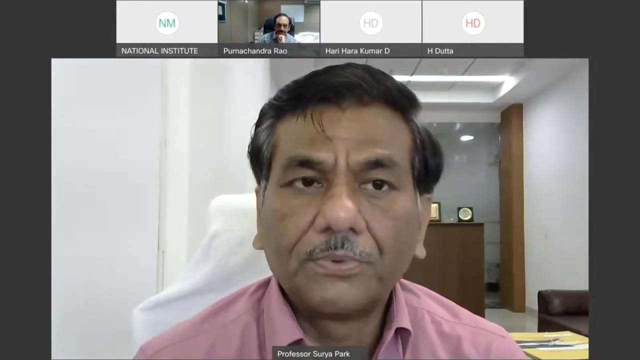 operations during the disaster times. I remember when the Sikkim earthquake took place, we were actually hindered by the road blockades due to landslides that happened co-simultaneously with the earthquake at that time. Similar observations were also there during the Uttarkashi earthquake and the Chamoli earthquake. 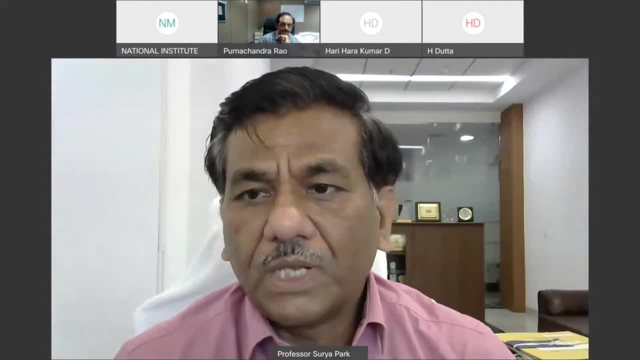 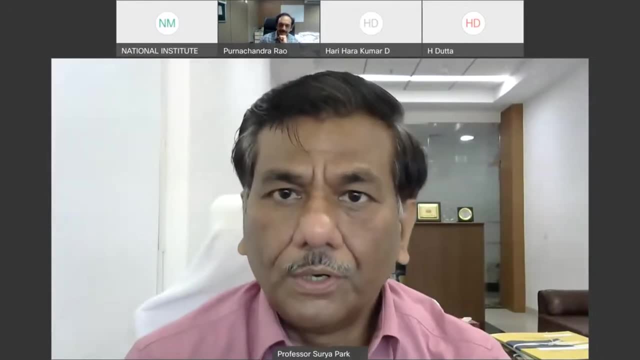 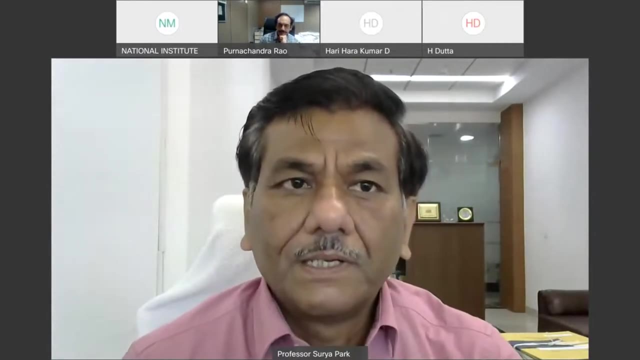 as well as during the Kashmir earthquake. So when we are dealing with the earthquakes, we have a multi-hazard perspective and we need to know not only the structural damages to the buildings, to the highways, to the infrastructure, utilities, services, but also the consequences of earthquake-related disasters. 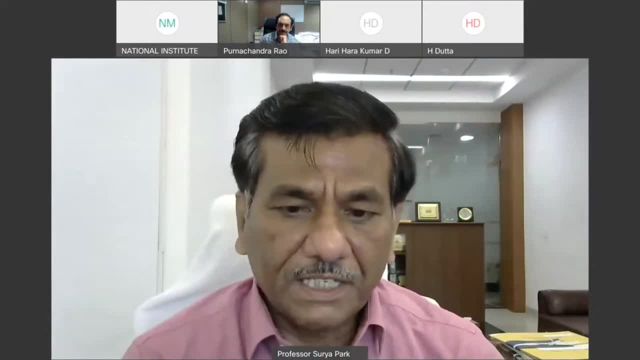 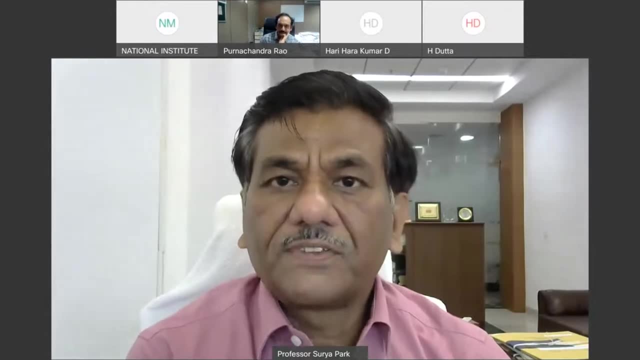 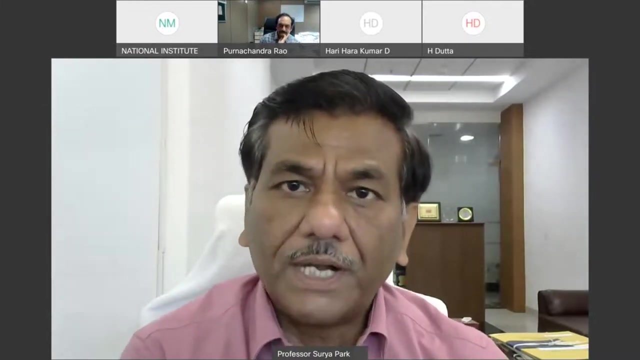 So they also need attention. Then the second point which we are more interested in is in terms of undersea earthquakes which are leading to tsunami. Government of India, after the occurrence of the 26th December 2004 Indian Ocean Tsunami, actually established a dedicated institute in Kwaiz for studying these earthquakes in 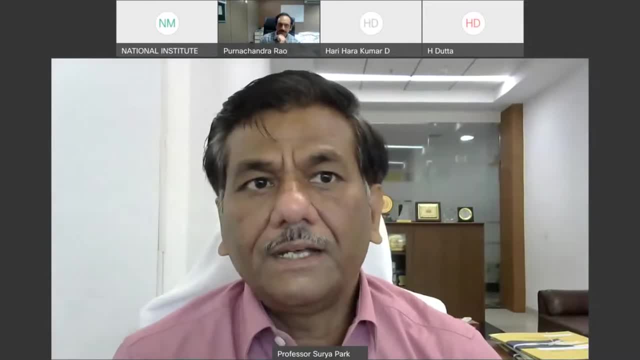 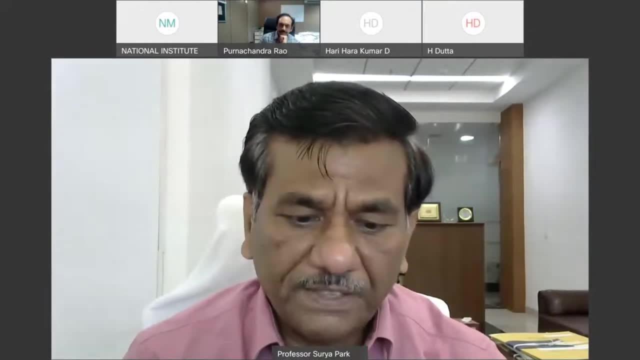 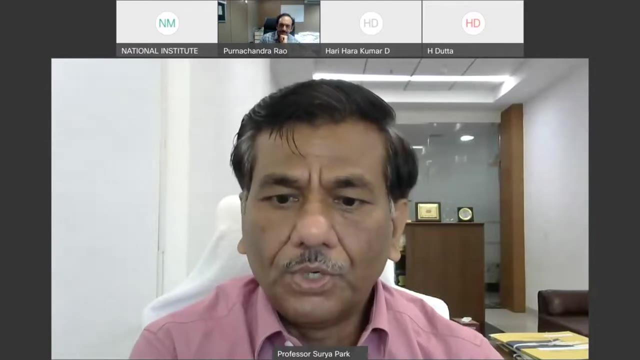 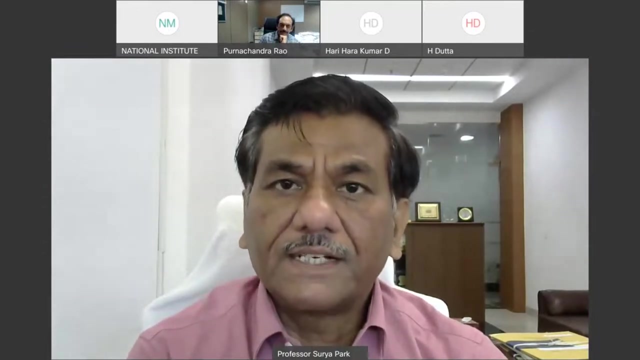 the region. They are also given a design in the project. They are also dedicated to the development of a sewerage system to help the earthquake-induced tsunami And they are also issuing early warning in that perspective, which is quite comparable to the Pacific Tsunami Warning Center, which was one of the renowned centers prior to 2004. tsunami who issued the early warning related to that event. But in our cases in the recent times, whatever undersea earthquakes happened, the related tsunami was not there. That's the reason why these earthquakes are that important. That's the reason why the earthquake happened. 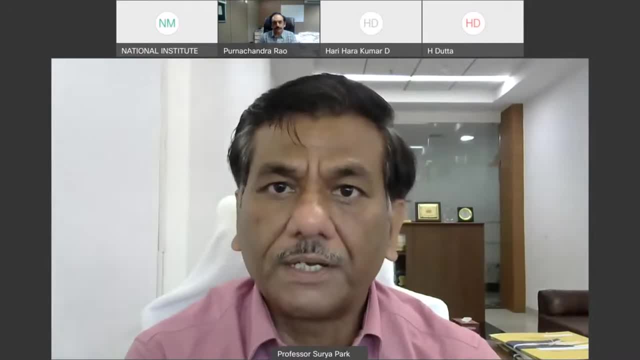 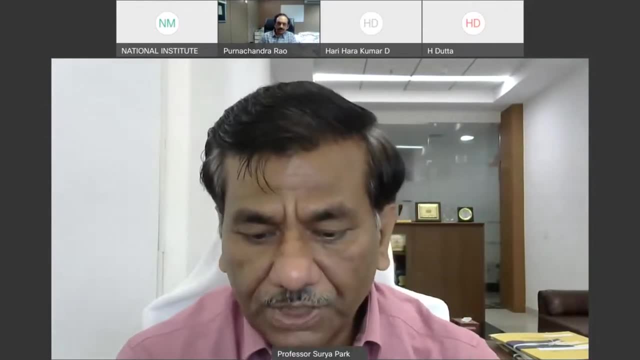 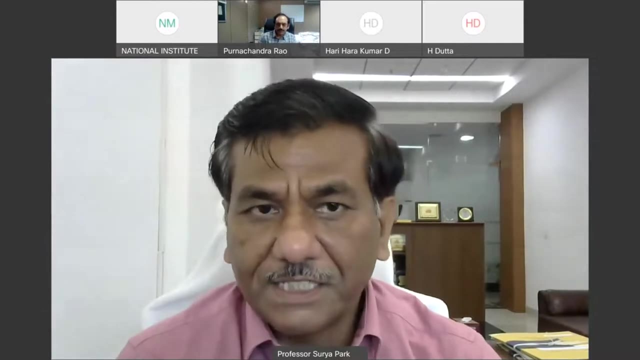 That's the reason why the earthquake happened. warnings were also issued by the inquires, which were found to be quite credible and reliable in terms of their forecast and modeling. So these are some of these issues which are of importance to us as earthquakes have been striking us. I just mentioned some of those examples which are: 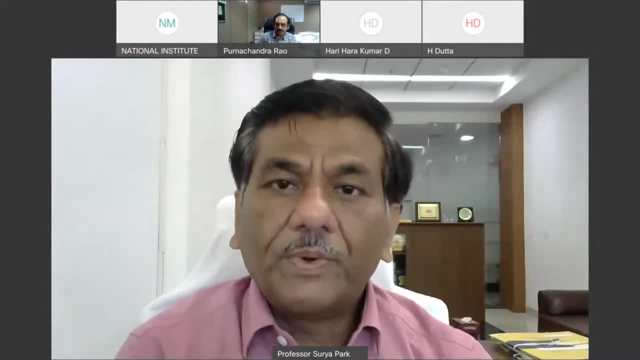 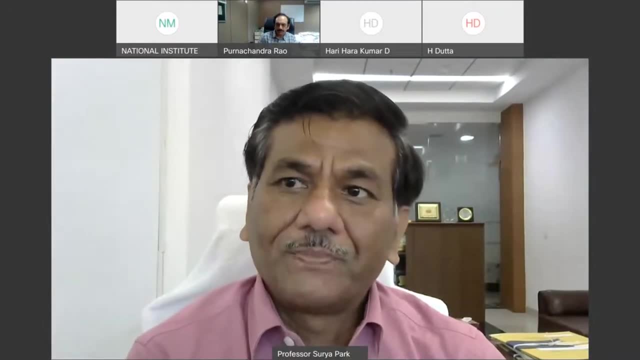 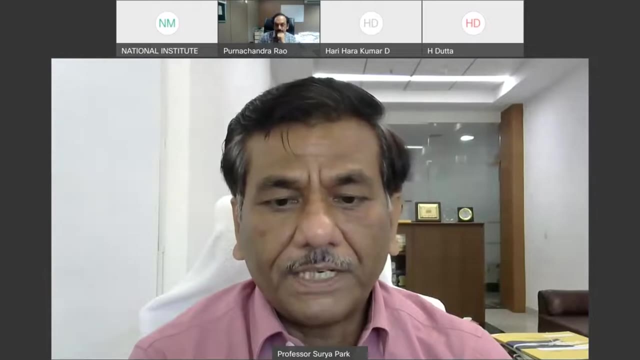 indicating almost an earthquake of magnitude more than six on a biannual basis. Almost every two years I can count on an earthquake that has happened in or around our country, And these studies are very important. I remember way back in 76 when Chinese actually tried to infer an. 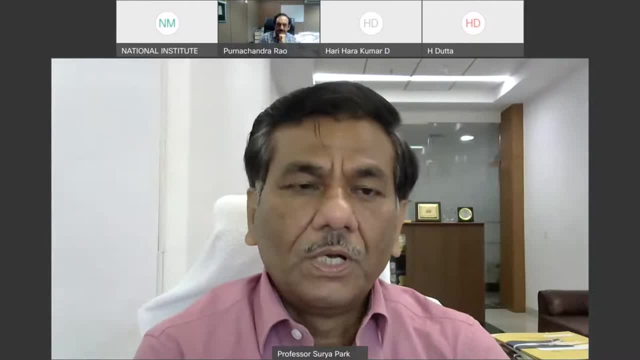 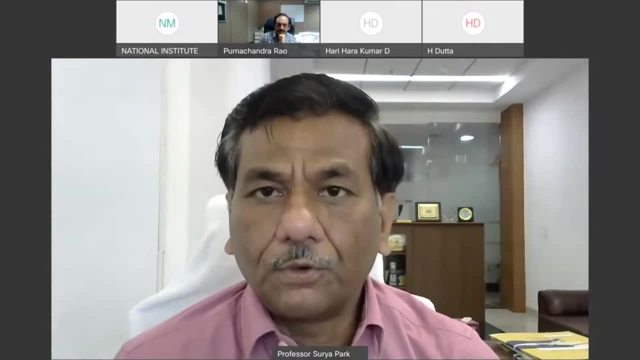 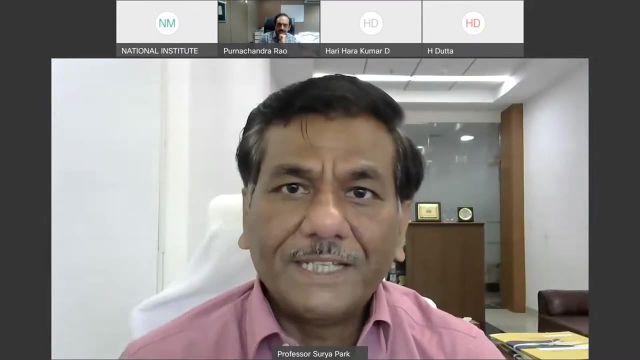 earthquake based on multi-parametric studies, biogeophysical parameter studies- which actually led to a correct forecast in one of the earthquakes, but the subsequent earthquake in the next year could not be predicted by them. So there are still some uncertainties, certain limitations. 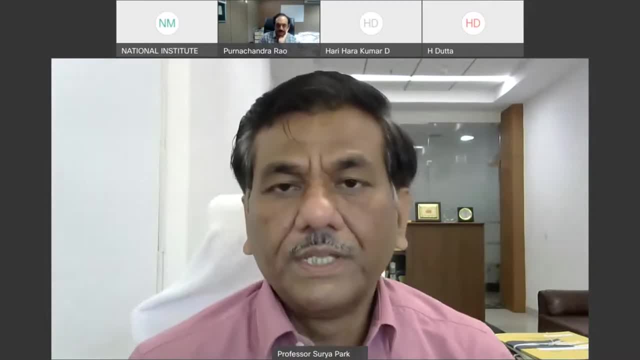 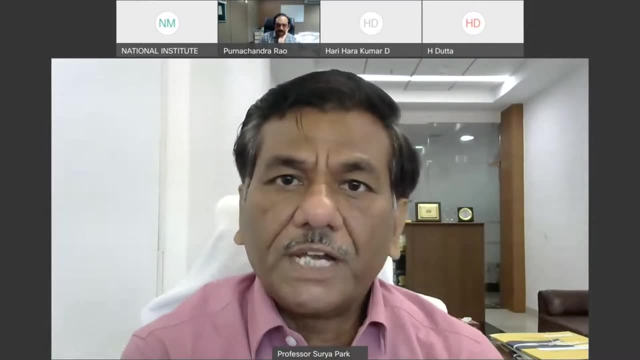 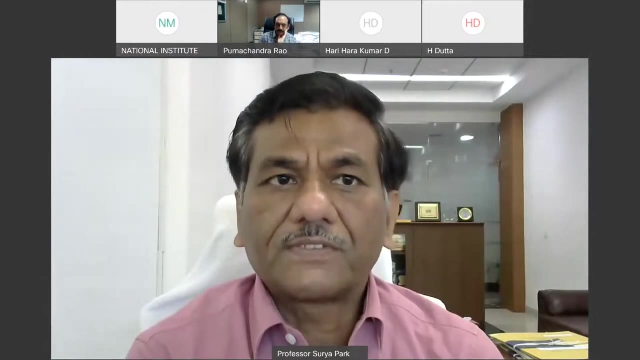 in our understanding of the earthquakes. Now we know the related tectonic features or structural features which are leading to this geodynamic phenomena And we can map those features, but still there are many hidden features which are subsurface and not easily detectable can also lead. 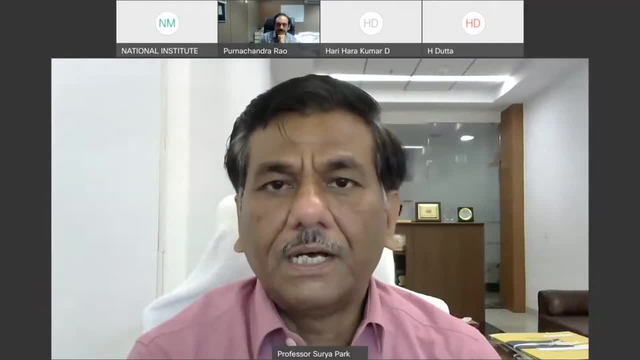 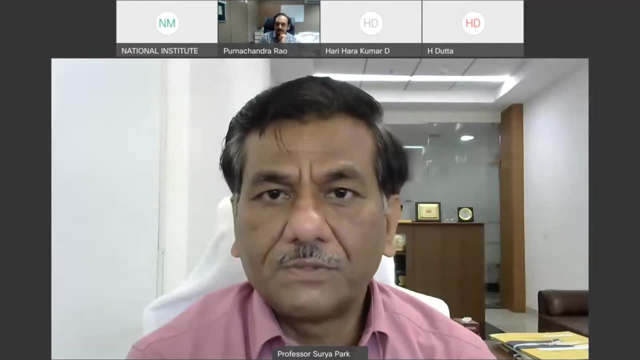 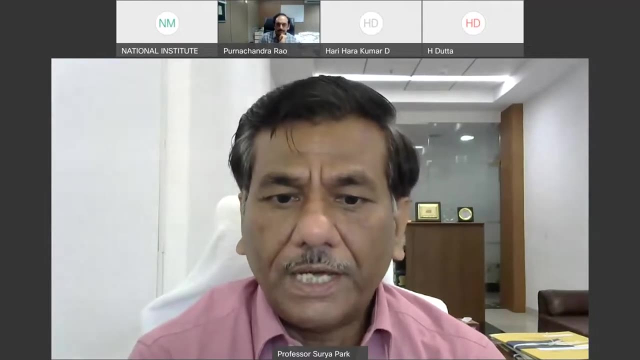 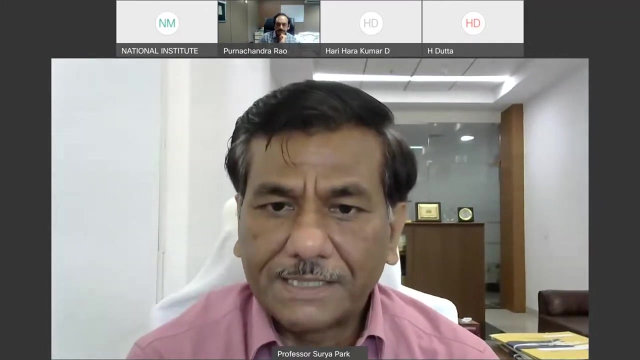 to earthquakes with unexpected locations, So or unexpected magnitudes. However, the current studies which have taken place in terms of the active tectonic mapping actually also helped us understanding the object locations in terms of spatial predictions for the earthquakes, as well as the instrumental technologies which have developed been developed recently. 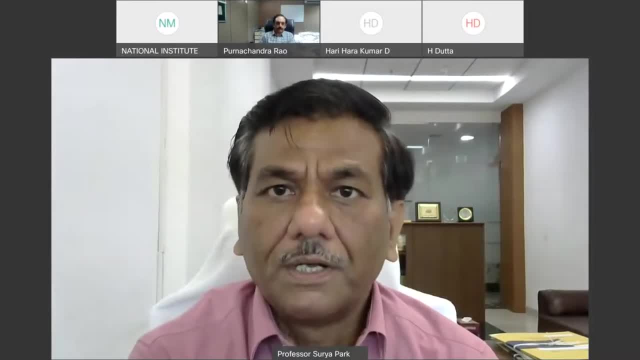 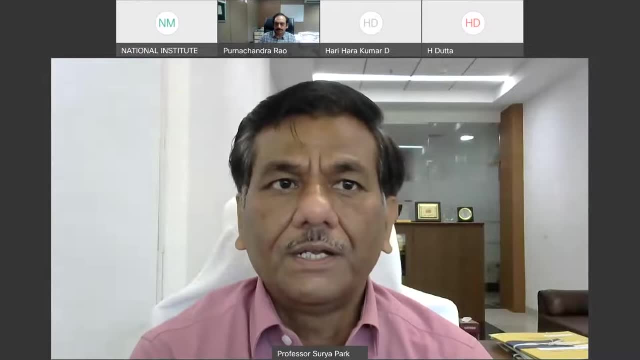 and been implemented, And now you may notice that the traceability of the objects in the video have actually given us some time slot or time lag for the earthquake early warning as well, But that's not good enough for humans to act, However. 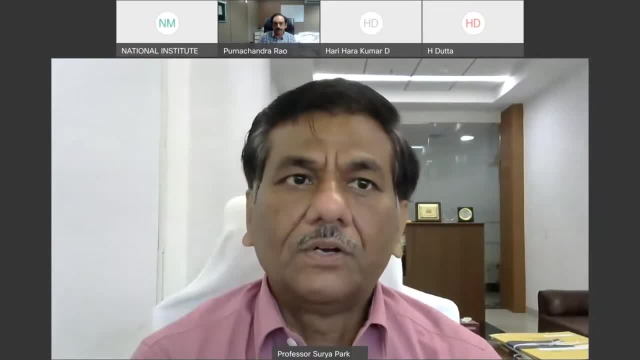 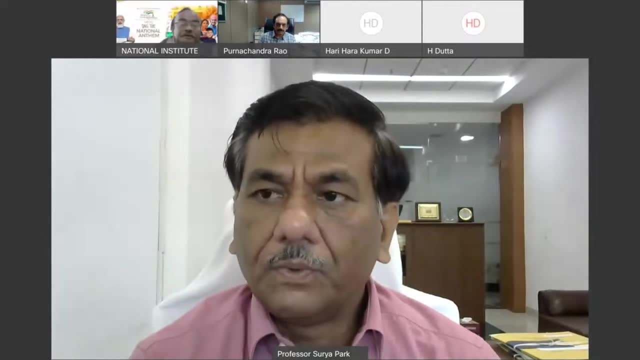 the automated systems. they can depend on that early warning, which is only for a few seconds to a minute only helps in the automated infrastructure systems, But on people need to be prepared against that, you know. So that is just the background on this slide. against that, we need to go for mitigation In terms of the follow-up of earthquake resistant features in our all constructions and developments, as well as retrofitting and re-strengthening of the existing structures and infrastructure to reduce the risks and enhance the resilience. 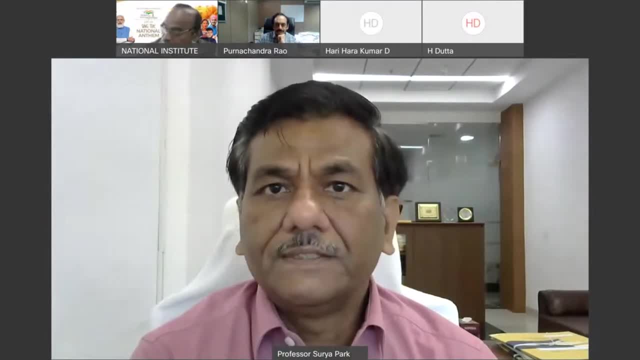 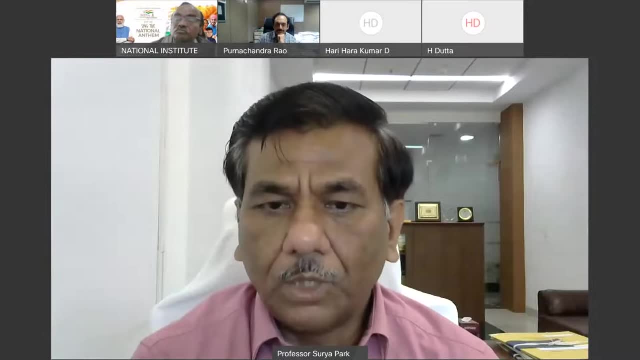 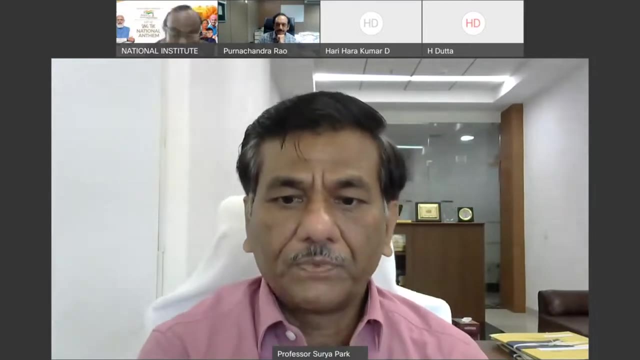 of our infrastructure, as well as the human beings, through adequate information, awareness and preparedness, with the involvement of experienced scientists that we are involving today, For example, Dr Puran Chandraoji and Dr H N Dardaji. both are very known figures. 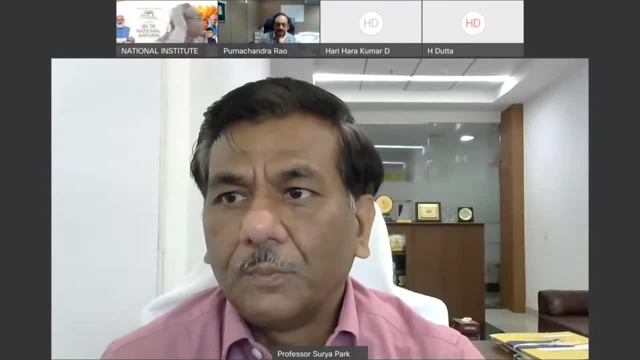 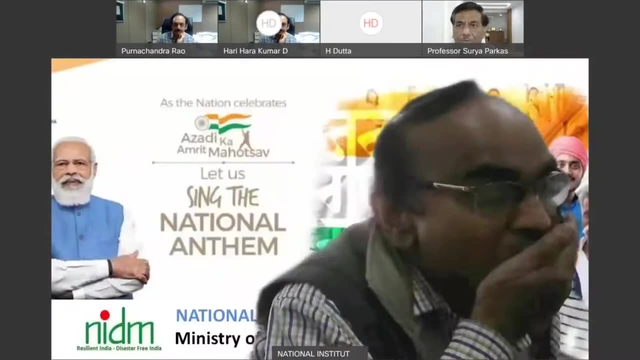 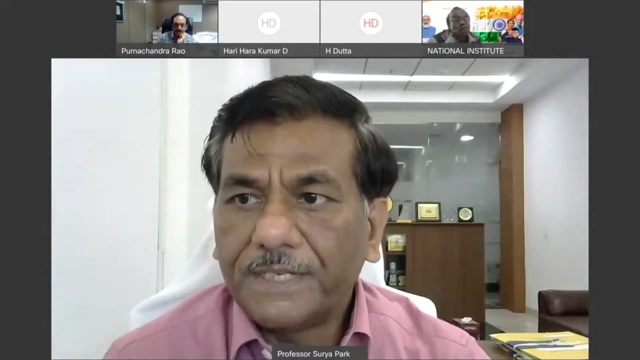 in this field, And Dardaji will be also talking about the precursors and potential early warning systems, And also they will be discussing about the detection of earthquakes and the earthquakes in Indian context. So I wish them all the best for their lecture, because 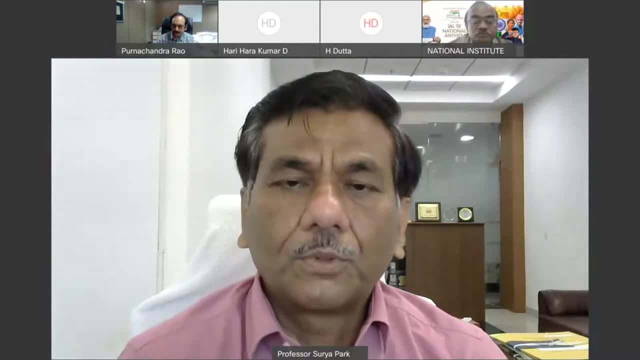 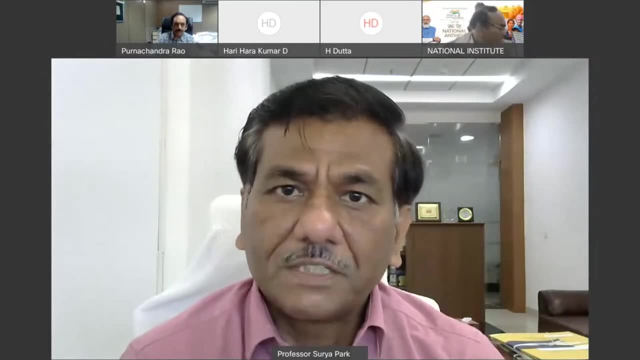 there will be more details about this program from their side, And I thank them for joining with us and sharing their rich knowledge, ideas, experiences and information, as well as innovations in this field. I would urge all the participants to kindly do ask questions. 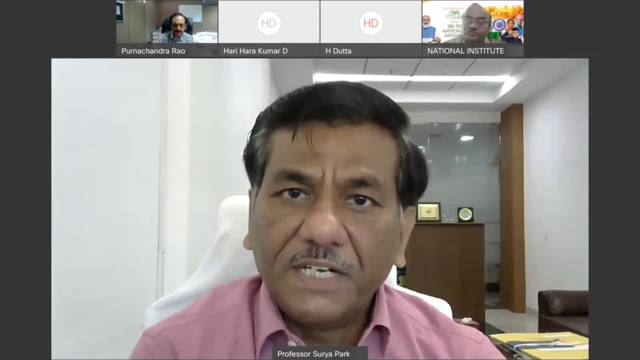 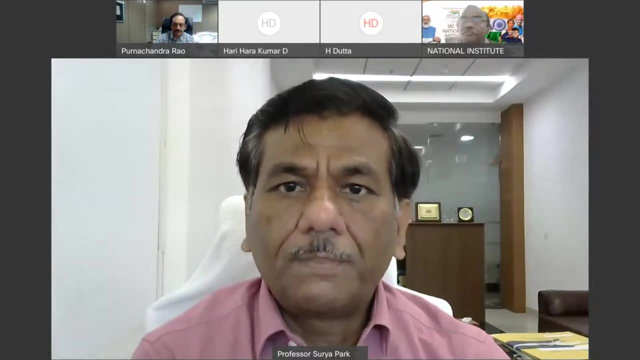 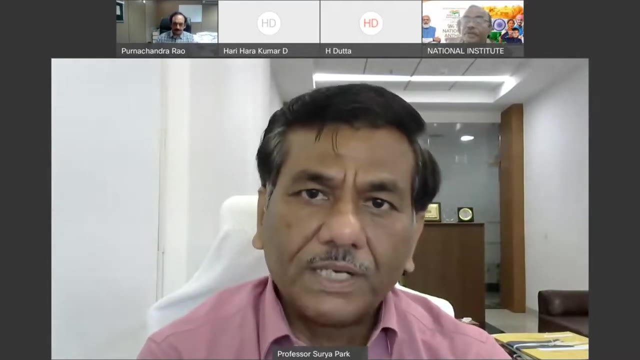 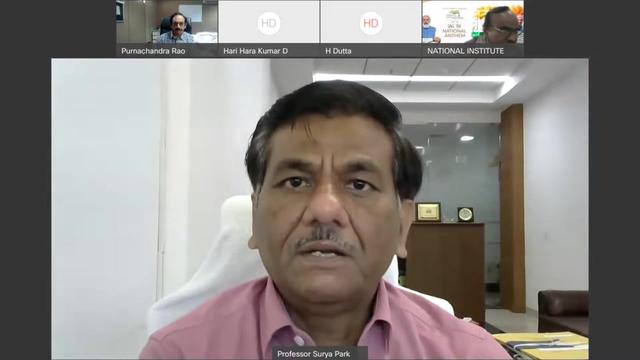 to them to gain requisite knowledge that is needed by you, And how can we actually deal with such disasters, which are still not well-predictable And we need to prepare against that? We cannot avoid, we cannot prevent the occurrences of earthquakes, So therefore we need to you know, enhance our awareness, information. 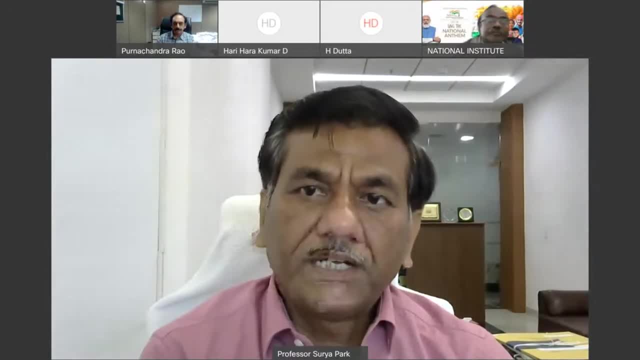 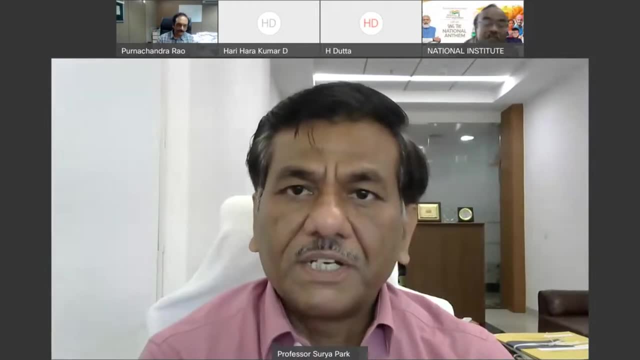 and preparedness against them, as well as mitigate the impacts of these disasters through appropriation. Dardaji Bhatnagar. Thank you very much, Thank you Haldar, Thank you everyone for your great interventions in terms of retrofitting re-strengthening. 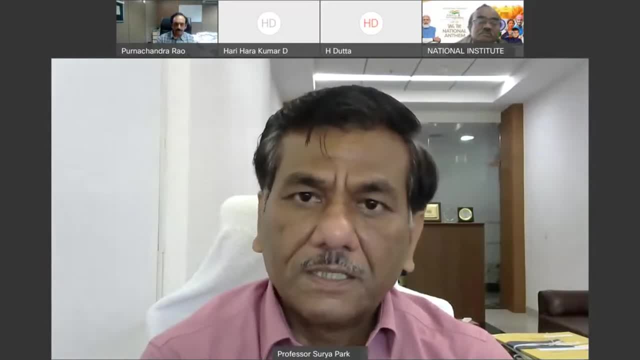 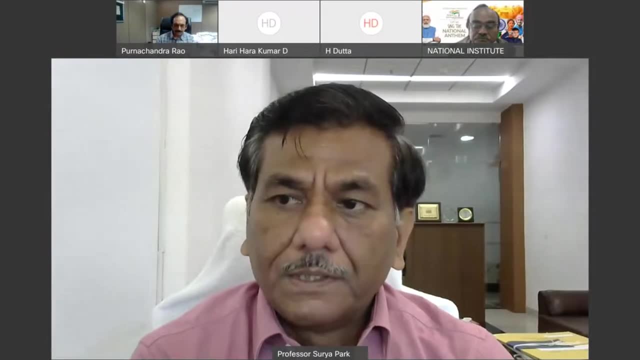 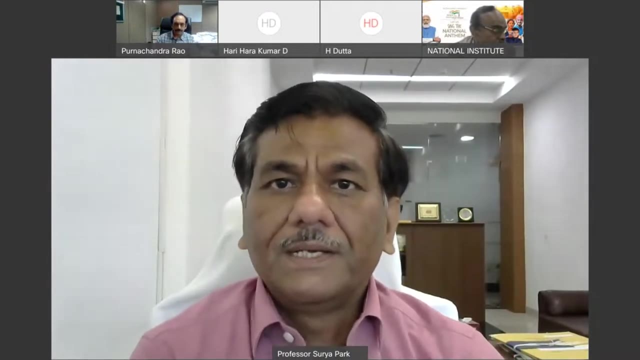 and earthquake-resistant features in workers, structures and infrastructures. So I wish them all the best And thank you very much for this. Wish you all a safe, healthy and good quality life on an equitable, justifiable and right-based manner, with good fraternity. 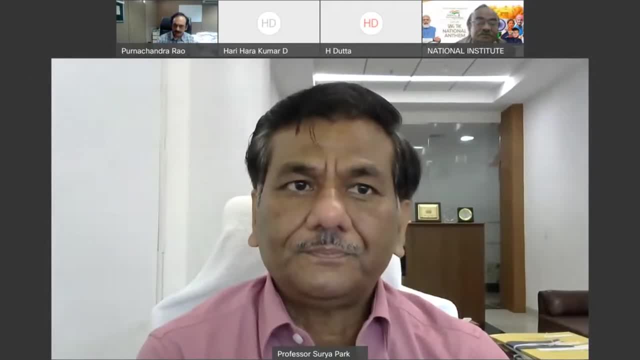 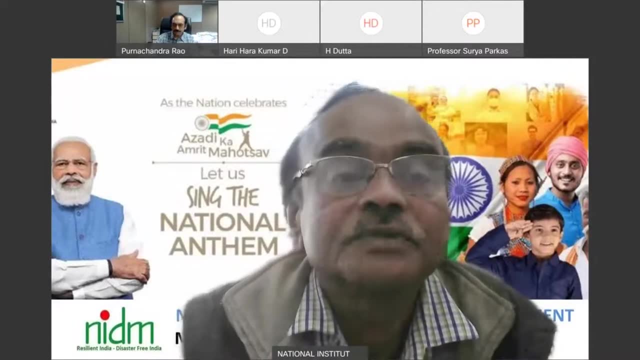 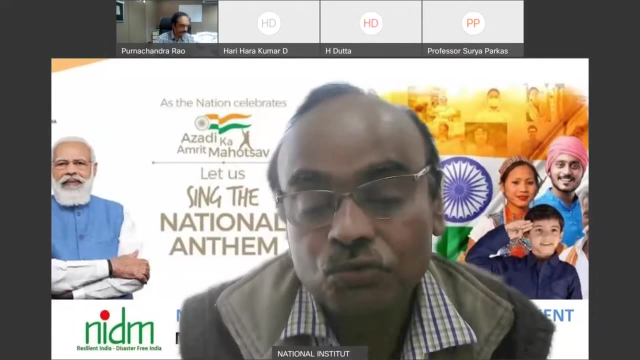 Thank you very much, Haldar. sir. Back to you. Thank you everyone. Thank you, sir. Definitely you are also right that we cannot prevent the earthquake, first thing. Second thing, we should motivate the people for the preparation and also we should put force for the mitigation and rehabilitation. That is all the things are true. 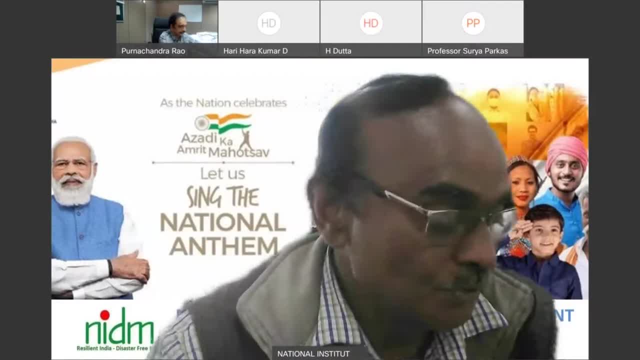 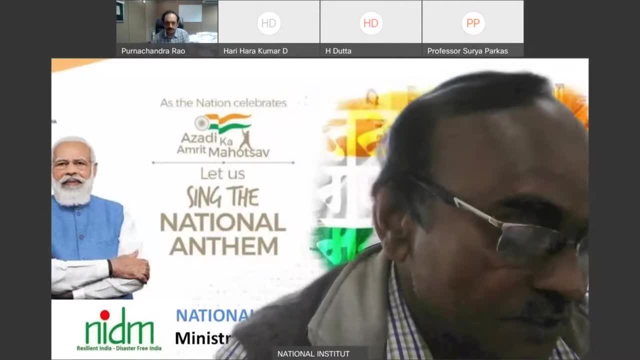 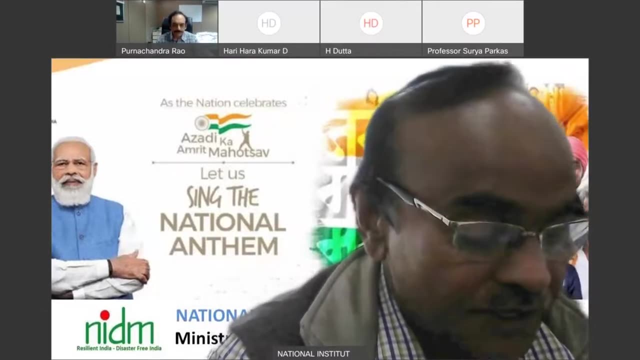 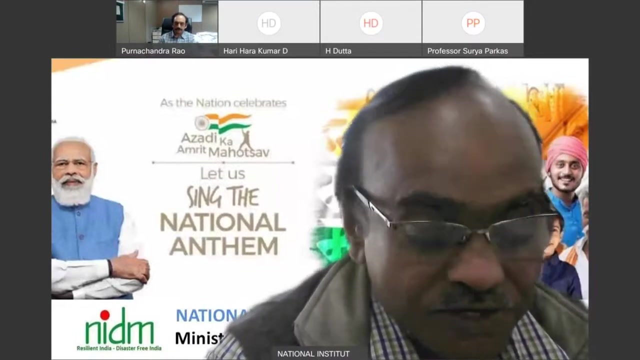 Now. next, I would request, in this continuation of the lecture after this keynote address, that Dr Puran Chandra Rao, Chief Scientist, NGRI National Geophysical Research Institute, that is, the CSIR, Hyderabad-based, and he'll put his lecture on earthquake prediction, forecast and early warning and current status. 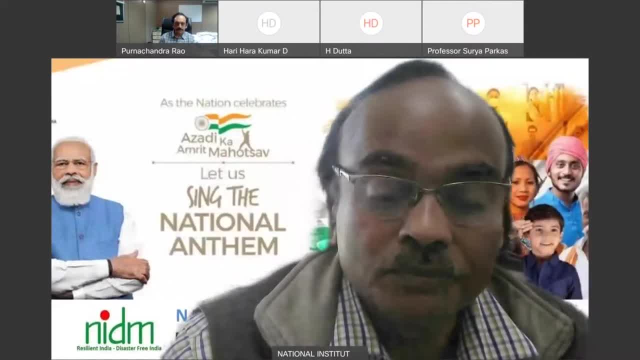 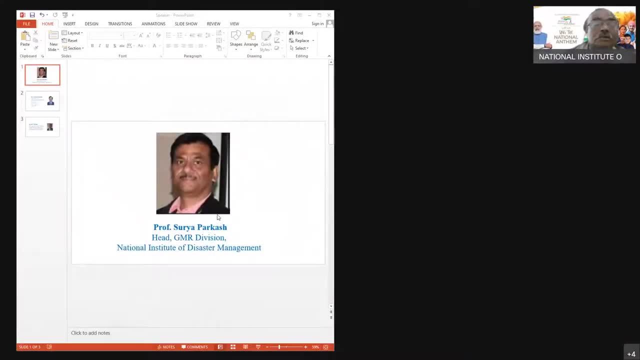 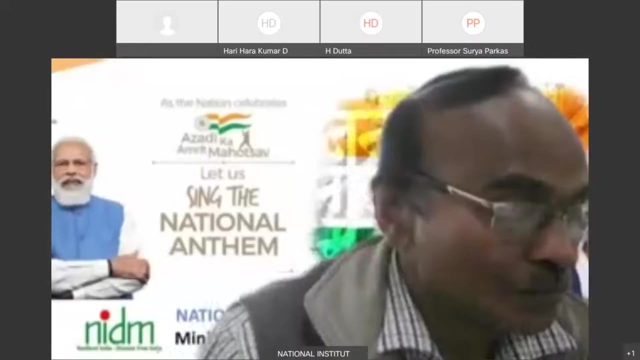 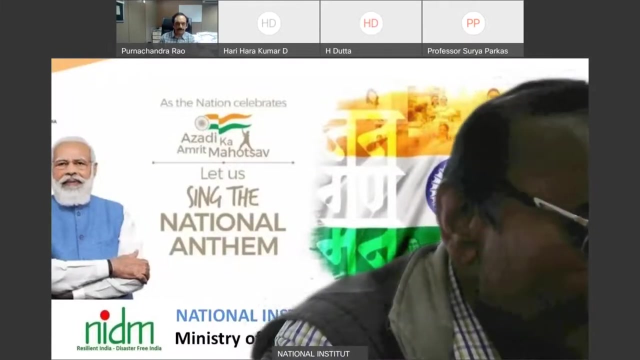 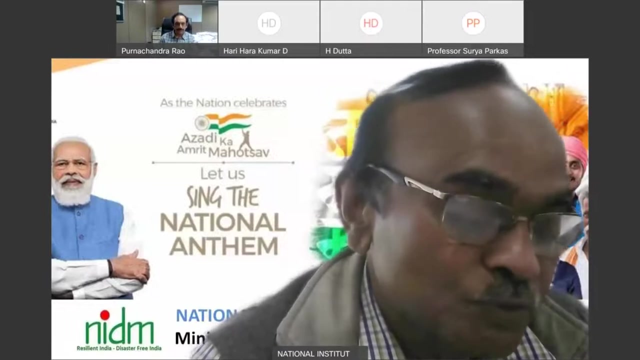 We know That Dr Puran Chandra Rao, he's a He's a chief scientist from NGRI and he's quite a long time he's working there And basically he's eminent speaker on earthquake. Dr Rao is an oil-owned seismologist. 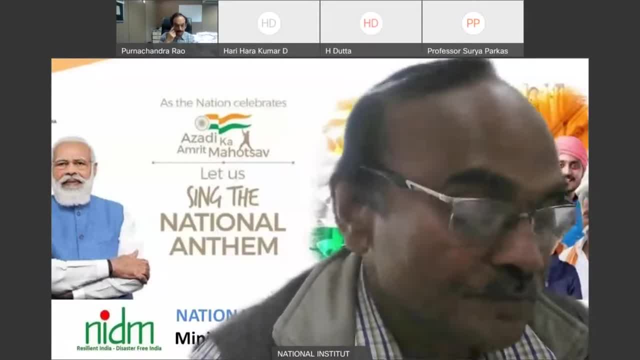 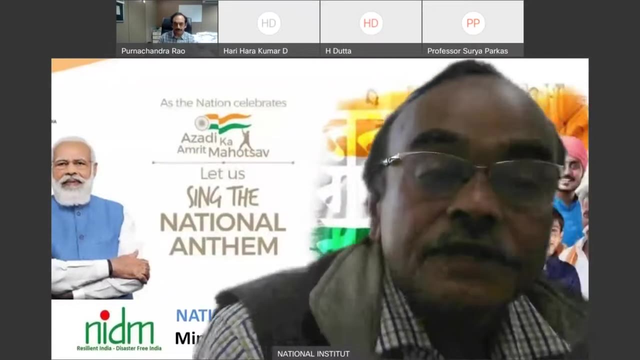 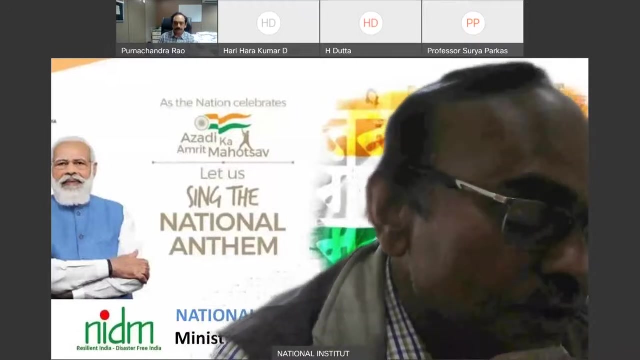 with over three decades of research experience and having worked in India and abroad. Currently he is working as a chief scientist, an AC SIR professor and the CSIR NGRI, NGRI and a premier research lab in the country, where he heads newly formed group of environmental seismology. Earlier, he worked for three years as a director of the National Geographic Research Institute. and the CSIR NGRI and a premier research lab in the country where he heads newly formed group of environmental seismology. Earlier he worked for three years as a director of the National Geographic Research Institute and he's quite a long time. he's eminent speaker on earthquake prediction, forecast and early warning and current status. 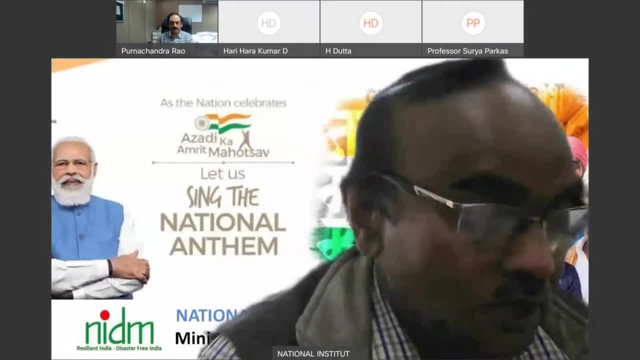 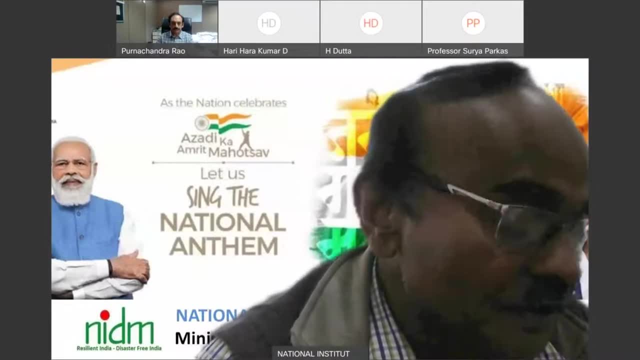 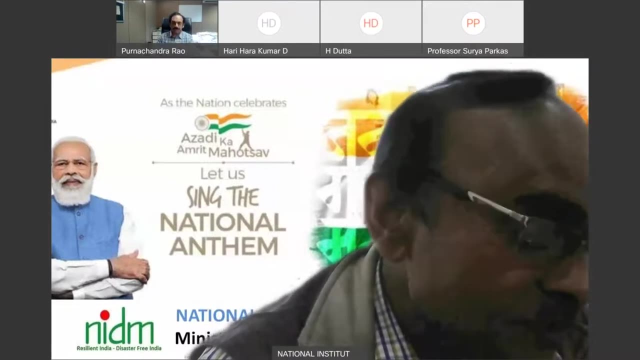 He worked for 3 years as a director of national center for our sense studies Under the Minister of our sense of India, where he did several new research program and activities, Dr how. he has his masters And in geophysics from university Hyderabad and also a degree in psychology from the University of Tokyo, Japan. 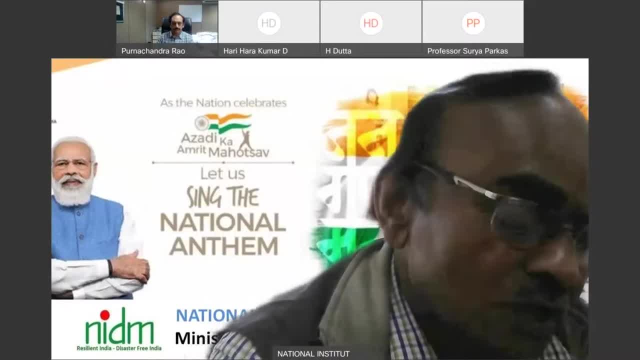 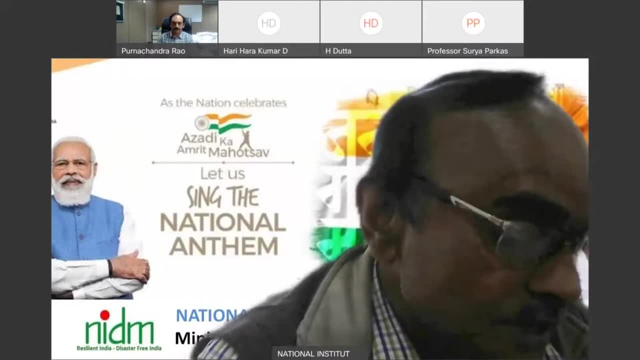 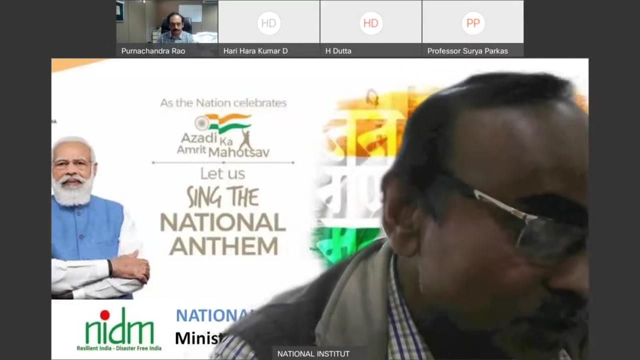 Specializes in seismic modeling for earthquake resource mechanism, as well as arts internal structure. His current interest include environmental seismology, ambient seismic, noise, tomography, tomography and reserve. He was involved in global assessment program of the Indian region and was the principal investigator from 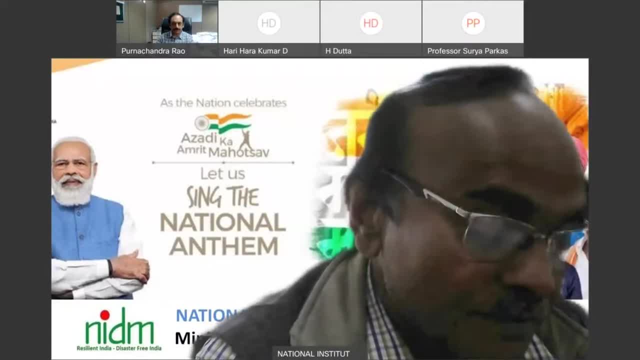 For the past seismic micro generation project Of the country in central India. he has led several important research projects, including seismic deep learning program In the region, a prestigious flagship program, a ministry of our sense government of India in his in its initial stage. Dr how has worked extensively on the seismic techniques. 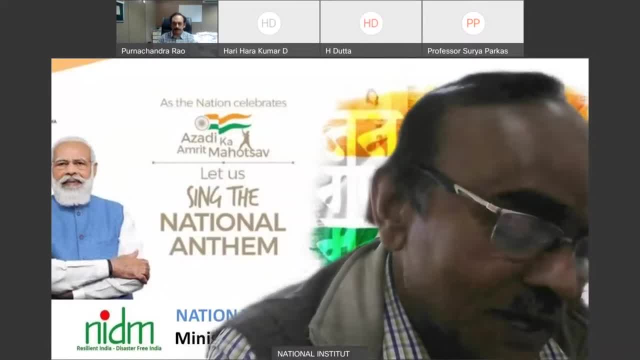 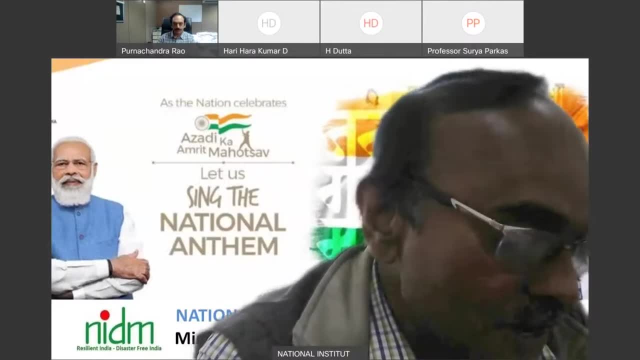 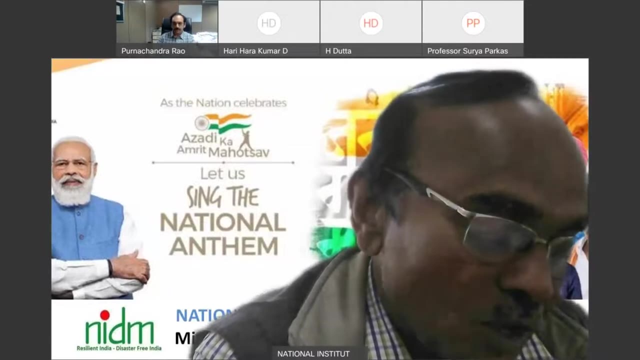 Of the Indian plate region, based on Local mechanism and space modeling studies. His work has provided several new models in the Indian plate techniques, The model as the most significant 1, being the explanation of session of subjection Of Burmese arc region, a result that appeared on the cover page of the geophysical research. 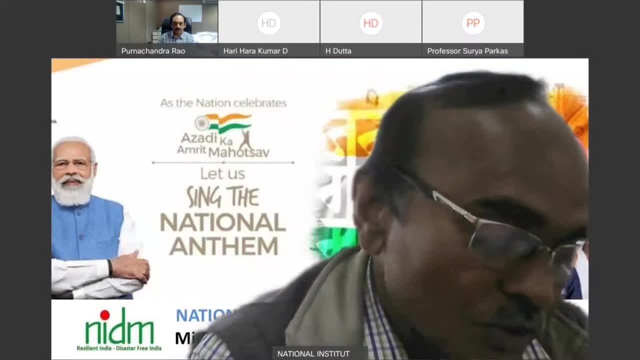 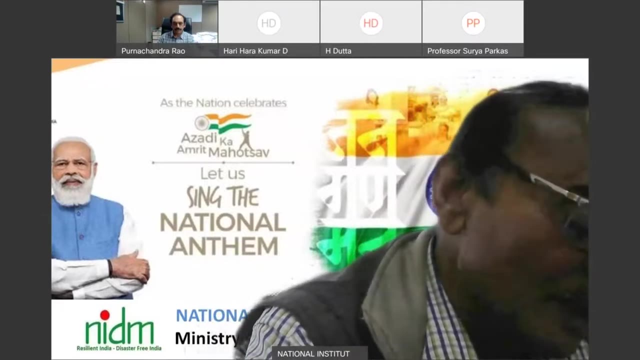 Letters in 2005,. he was fast To propose a unique Up uplift mechanism of the ceiling plateau in 1997.. Dr how he's in his credential. he's having more than 100 published paper reports, book chapters. She has doubled widely in. 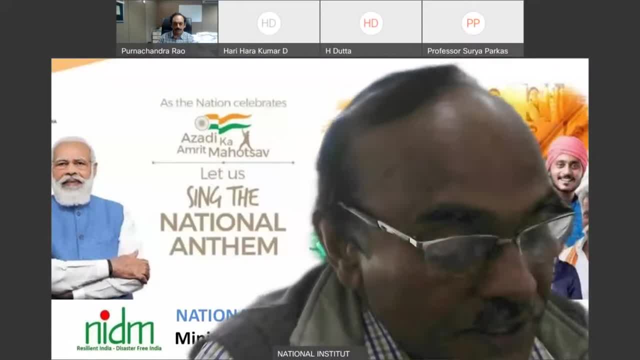 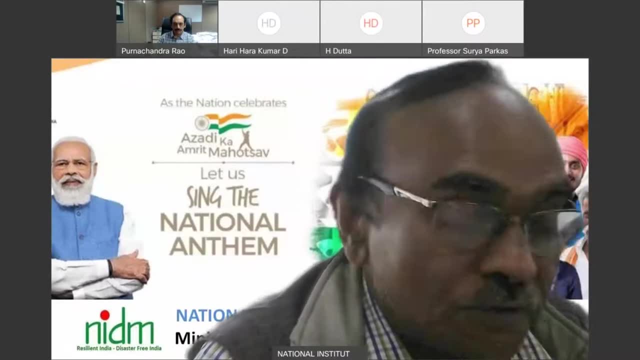 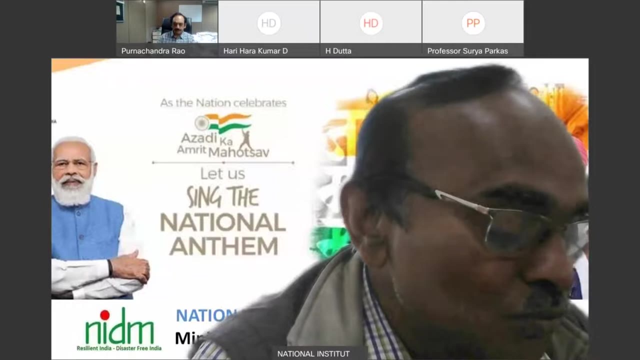 Uh, in global or a visiting scientist. over 20 countries. he has guided And basically guiding also more than 12 PhD students, including a foreign student from Vietnam. His latest work on seismic monitoring and with reference to 2nd February. 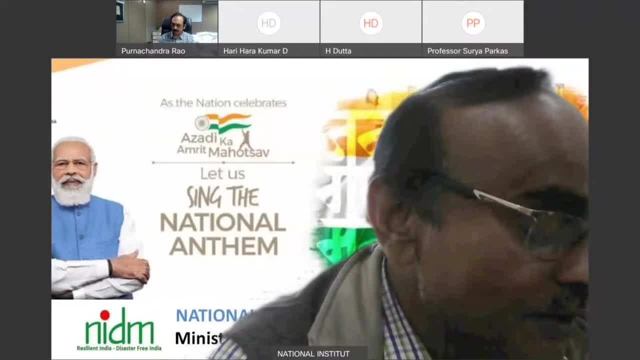 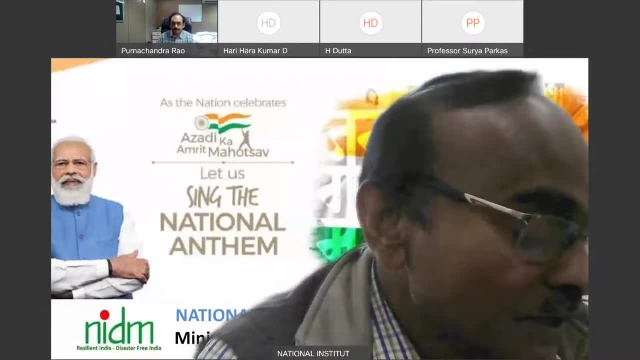 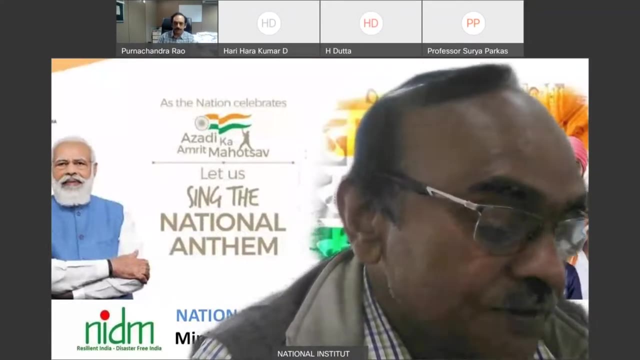 And that is 7th February 2000, 2021,. it was recently published in Uh prestigious general science general. Dr Was the 1st recipient, when you see PhD thesis award and it was instituted in 1997.. 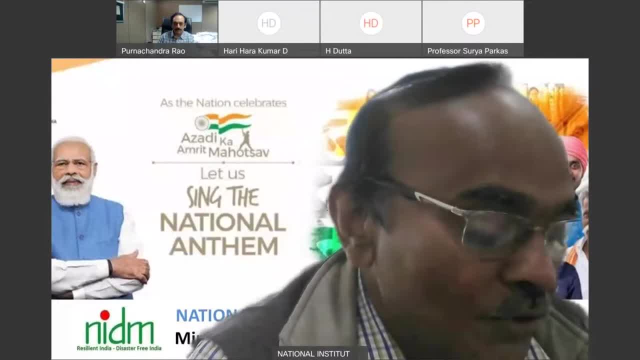 He's also a recipient of the prestigious Humbled fellowship in Germany. He was fellow at the earthquake research Institute University of Tokyo during 1995 to 2000. letter. He was a visiting professor at the University of Tokyo, Japan, in 2008, a research fellow. 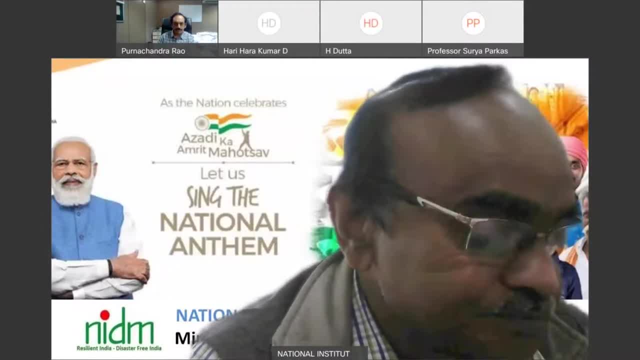 At the University California, San Diego, USA. He's a recipient of a national Science our 2016 from the mystery of minds government of India. He's the fellow of geological society of India, a fellow of both under a position and academic science. 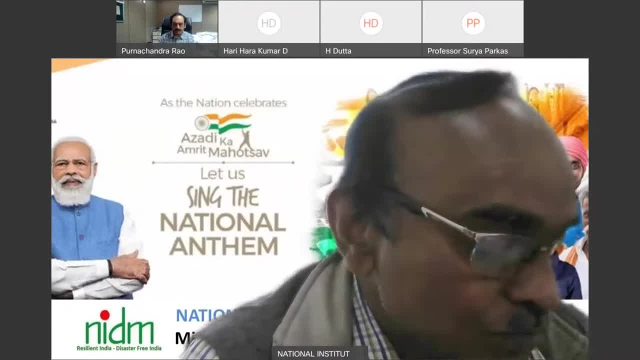 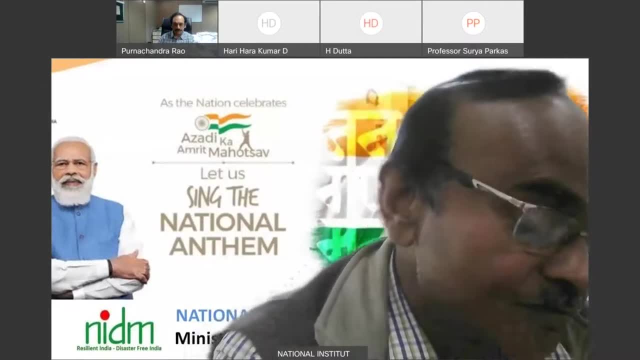 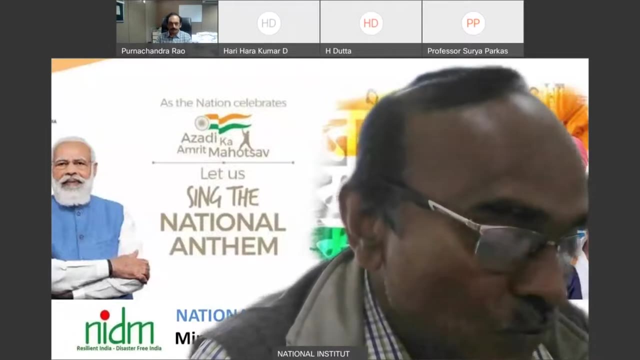 He's a member of several important committees: We're up standards, government of India and Department of atomic Energy committees for tsunami studies. He was an associate editor of the journal of science, Art system science editor, a board member Of general Asian art senses and editorial board of advisory. member of Indian general of our senses. 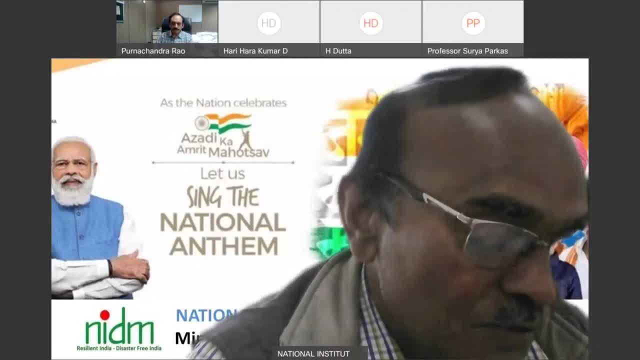 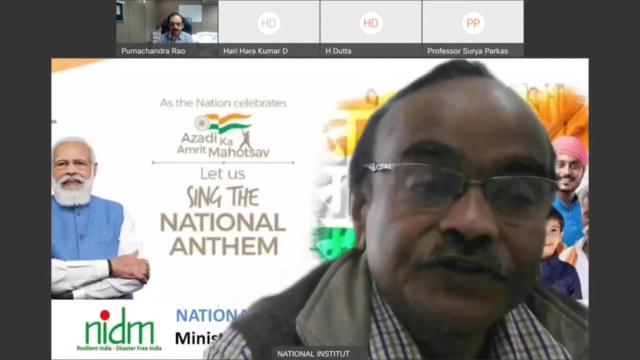 He was guest editor for several special issues And reviewer for top journals in ourselves. Additionally, Dr how has been spoke person and social media handler in CSR in dealing with the press and media for several years now. in this, the science day, he's having this Roman fellowship Also. 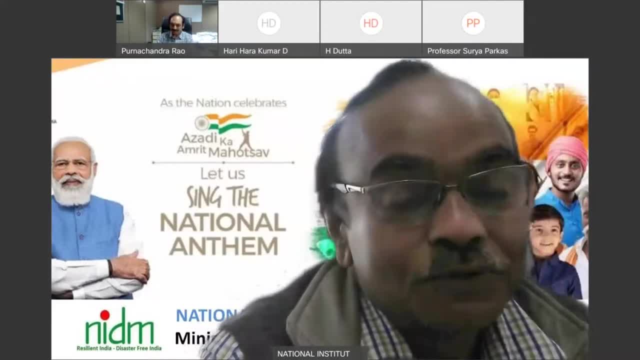 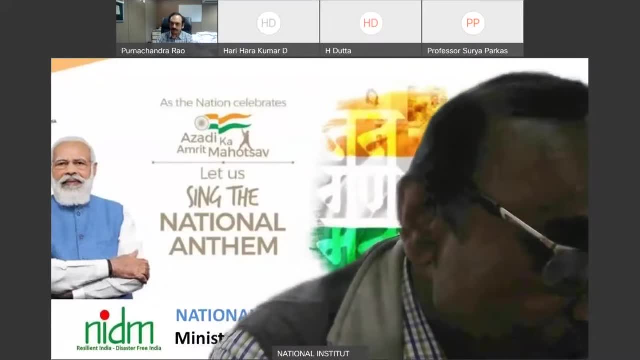 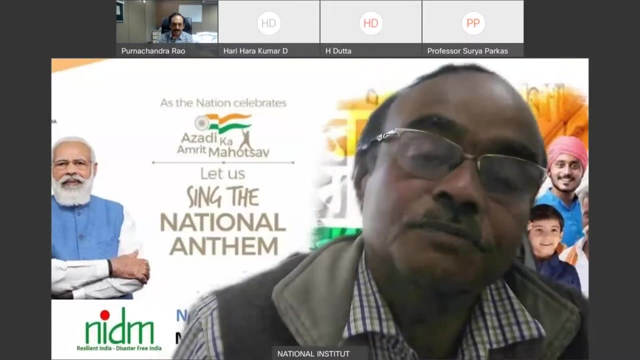 It's very appropriate that we got So Dr how to have put his lecture on the topic, That is, the earthquake prediction, Forecast and early warning and current status. with this I will hand over the stage to Dr, or to take up the stage and please go ahead. 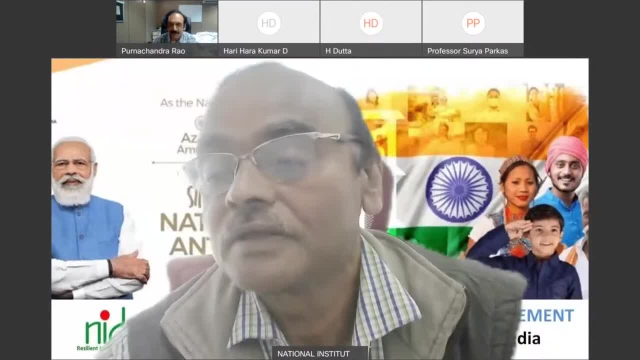 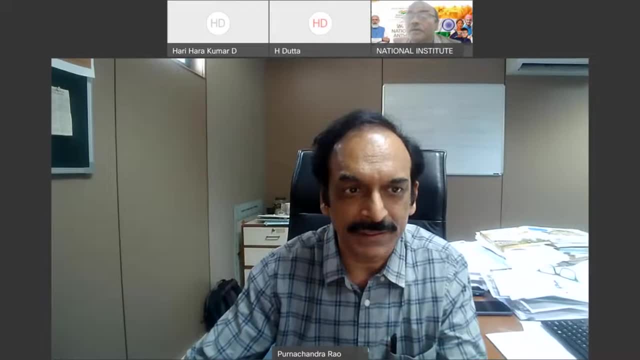 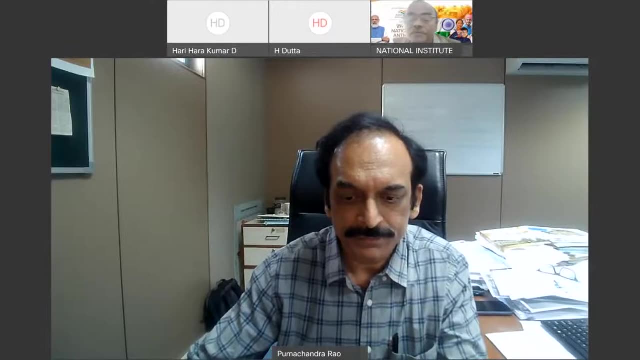 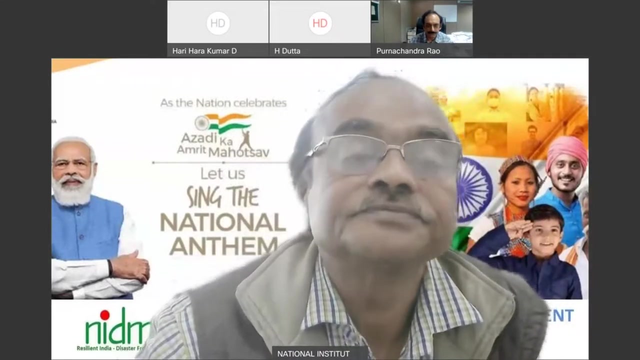 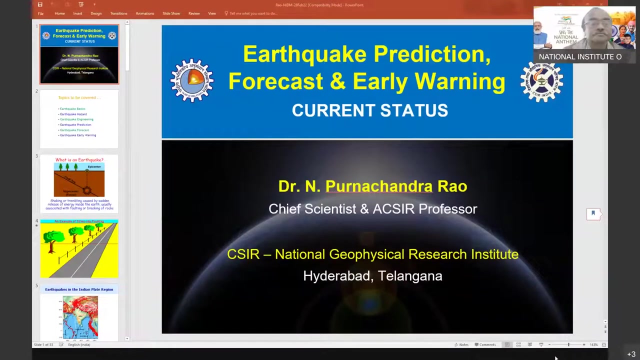 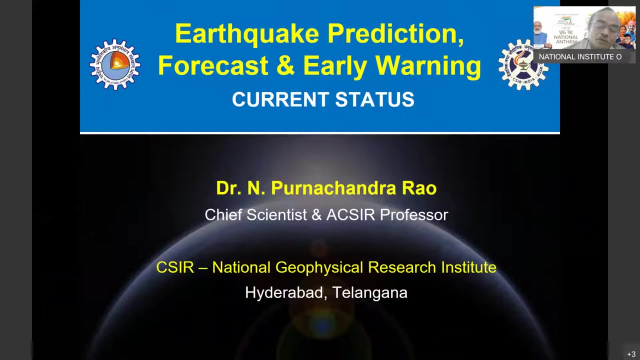 Thank you very much for your very kind words. Uh, Professor, data Professor, and uh, very distinguished scientists and students who must be attending this stock. may i load my presentation just one second? okay, yes, you are visible and yeah, all right. yeah, so i have been working as a seismologist for more. 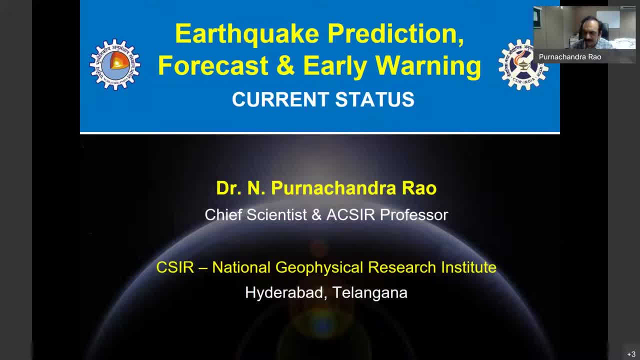 than 30 years now, and during most of my lectures, the the most standard question that was asked was: can earthquakes be predicted? i'm sure you will all agree, and unfortunately the answer is no. so we start off with a very sorry face, saying that it is not possible. but then we, we 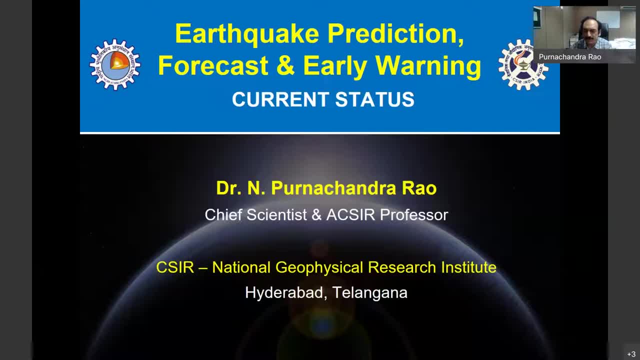 also need to understand, apart from this, what else is possible, because it's not just about prediction yes or no. there are so many other responsibilities that we have, uh, which were outlined by professor siri prakash a little while ago, so in this talk i will, i would like to um try to bring in the perspective what prediction 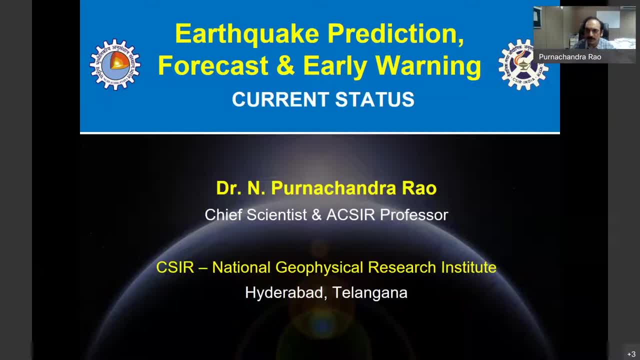 means and what forecast means, what early warning means what we can do and what we cannot do, and i'll give you some examples so that will highlight where we stand. i think it's very important to understand and all these elements so that we know where, which way, we are going. so the topics that i briefly 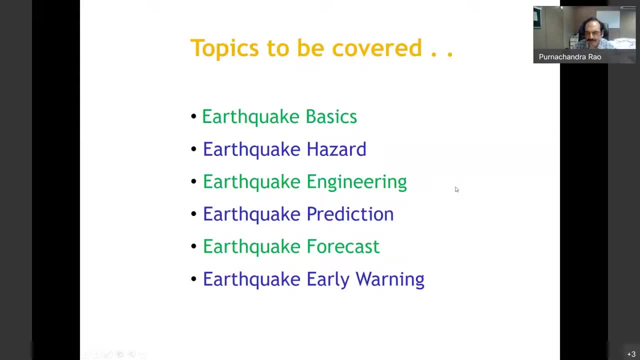 touch upon will be the little basics of earthquakes. in case there are non-specialists, then i'll deal with earthquake hazard, earthquake engineering, earthquake prediction, earthquake forecast and finally, earthquake early warning. so let us quickly see what these all mean and where we stand now. this is a basic definition of earthquake. as you all know that it's basically a block moment, the 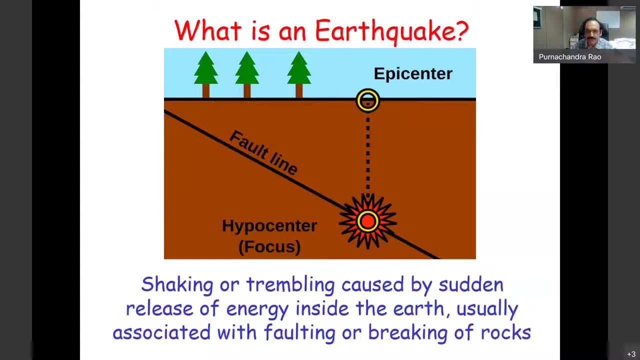 shaking or trembling caused by sudden release of energy, and this is associated with faulting, which is a block moment. it's very important to understand that this is distinct from a new, an explosion. so an explosion, the energy goes radially out, so it's a. it's a circular transmission of energy. 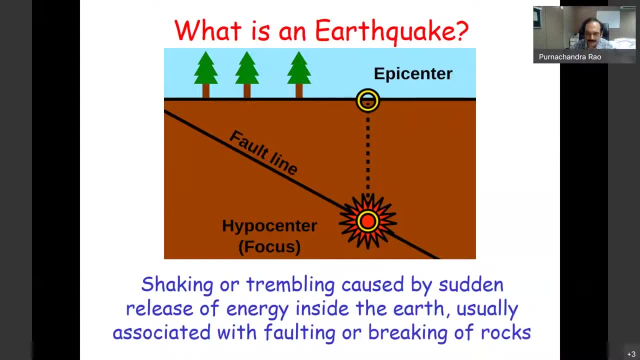 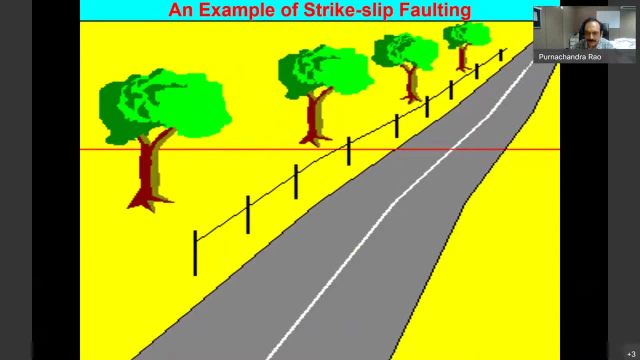 whereas in an earthquake it is a block moment along a line or along a fault. now this is an example of a strike slip type of earthquake where the as long as the stress can be resisted by the medium it resists, and once the critical limit is reached, then it breaks. so this 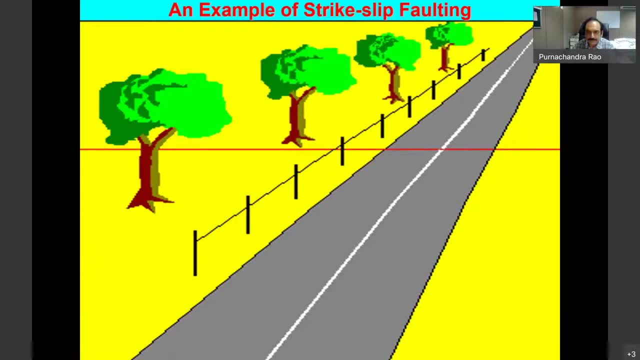 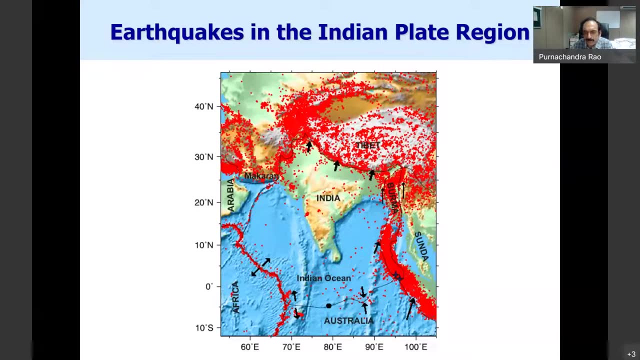 very clearly explains how an earthquake occurs. now this is the indian region and you can see the last 50 years of earthquakes have been plotted in this diagram and this very clearly shows which are the hazardous regions: the himalaya, the burma, andaman arc. these are the most hazard. 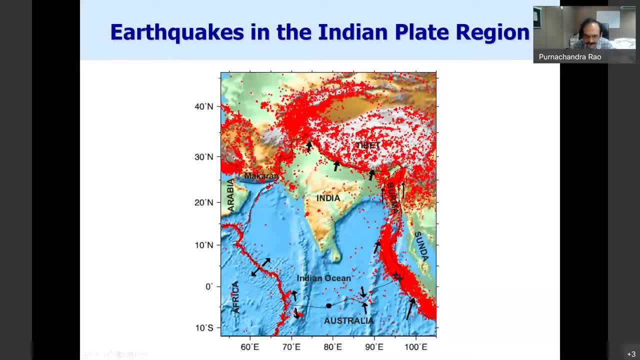 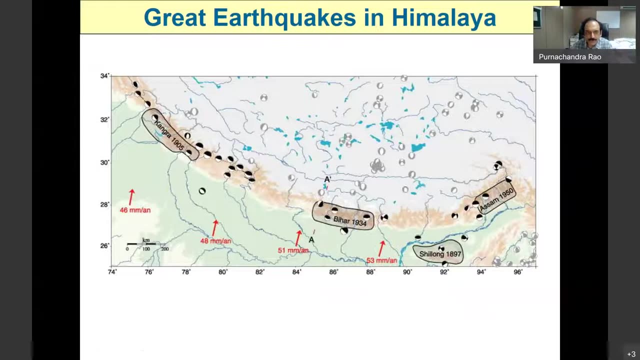 hazardous regions. you also have earthquakes in the indian ocean region which are smaller in magnitude, and some within the continent which are called intraplate earthquakes. now, coming to the himalaya, we have seen the greatest earthquakes, at least four. we have seen the 1905, kanga, the 1890s and shillong earthquake, the 1934. 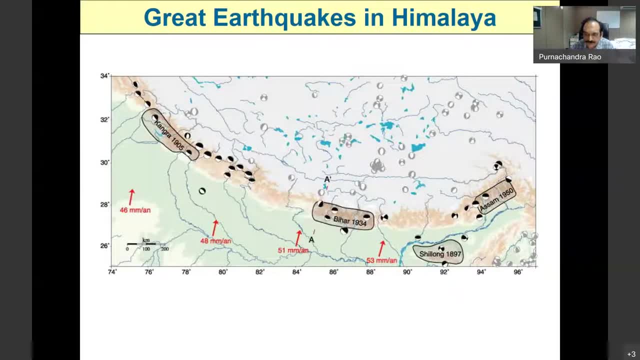 bihar, nepal earthquake and the 1950 assam earthquake. so ever since we have not seen any earthquake in the himalaya and therefore it is anticipated that another great earthquake is already overdue. and which region is most likely to have this great earthquake? it's a rather obvious because 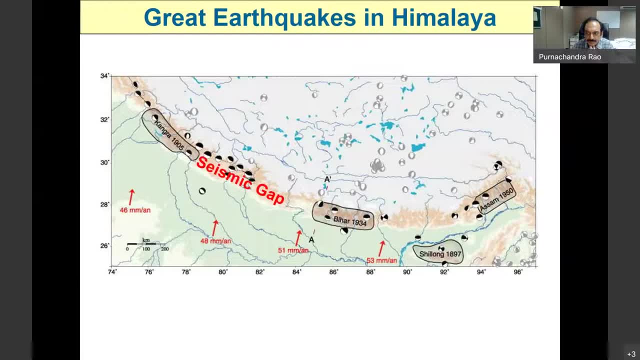 you have a huge seismic gap over here, so it is believed by experts that another great earthquake is around the corner in this region, and you also know that in 2015, there was an earthquake in nepal which killed several people, but unfortunately, it turned out that this was not the gap filling. 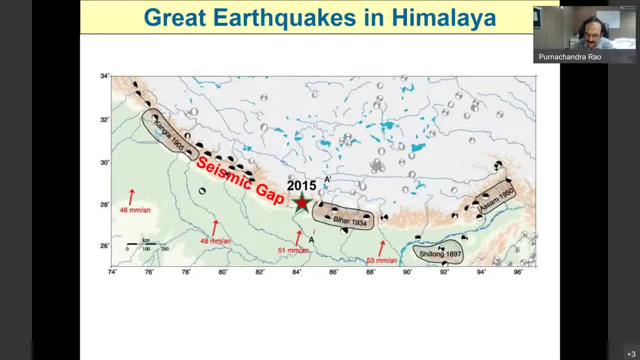 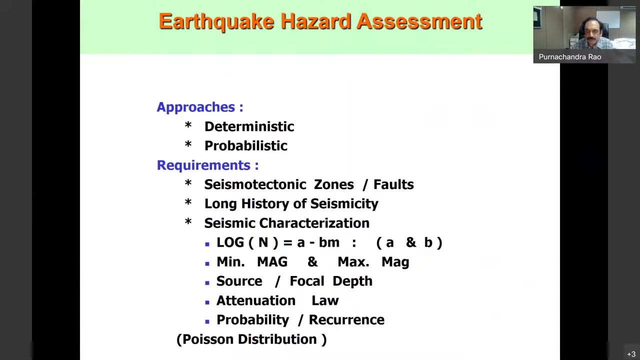 earthquake, so it was just like a precursor or it was just like a teaser, i would say. i'm sorry to say that. so, which means that the hazard very much exists and there is an anticipated great earthquake in this gap region now in in the in. in the face of this situation where we have to face great earthquakes in future, 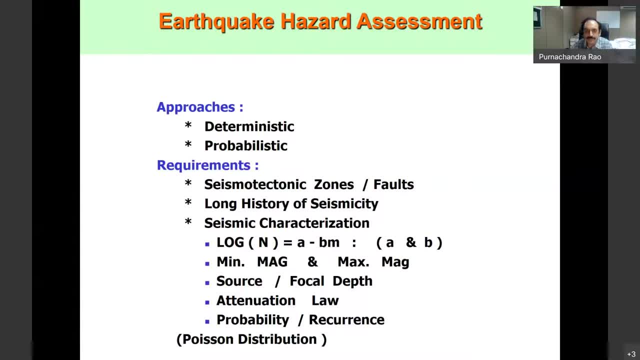 what are the approaches that seismologists generally take? so, as you all know, earthquake hazard assessment is a very important thing so that we are aware of how much of hazard we can expect in different parts of the country or at different seismic zones. so there are two approaches. 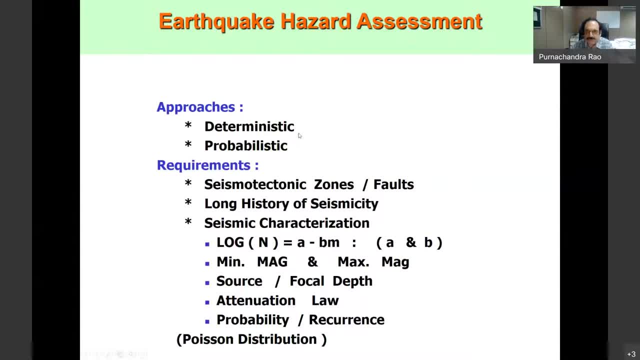 deterministic and probabilistic. so this term deterministic is basically a forward computation, where we assume all the values and we do a forward calculation of how much hazard we can expect at a region. the other, more popular approach is the probabilistic approach, which is based on all the past data, so it's basically an assessment of the existing seismic. 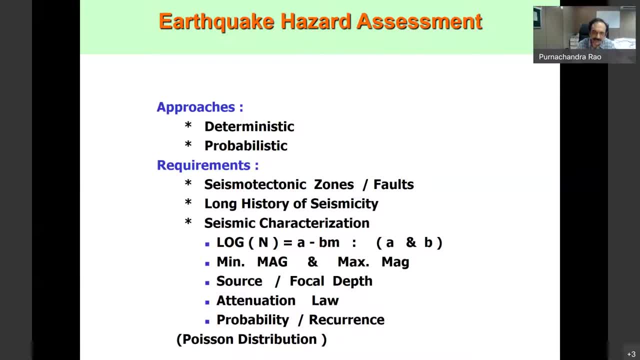 seismotectonic data of the region. so the process involves identifying all the seismotectonic zones, making a history or a catalog of the seismicity from the past. so you know past represents the future. so if we study the past carefully and see what kind of seismicity happened in a place, 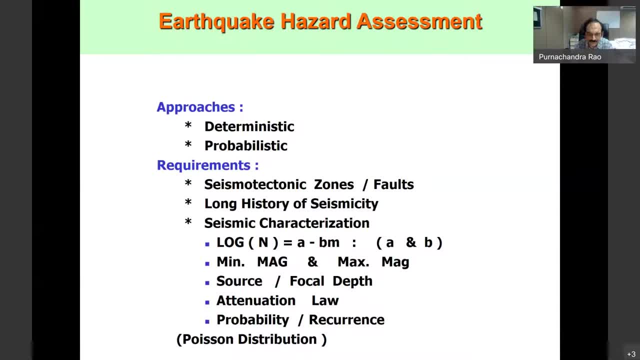 then it gives a clue to what can be expected in future, and then you have various other things. these are all technical aspects where you need to develop the b value for the region. i'll come to that. then the minimum and maximum magnitude: what? what are the expected? 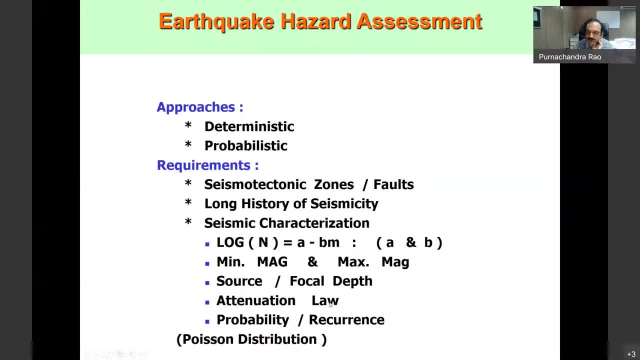 source, locations and focal depths. and what is the attenuation law? that means how the energy attenuates as the seismic waves propagate. and what would be the probability or recurrence of an earthquake. that means the larger earthquakes occur less frequently. so what would be the return time, return period for such big earthquakes? so these are all the aspects that are required to be. 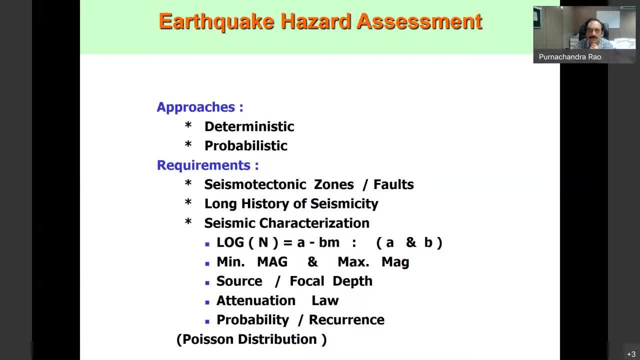 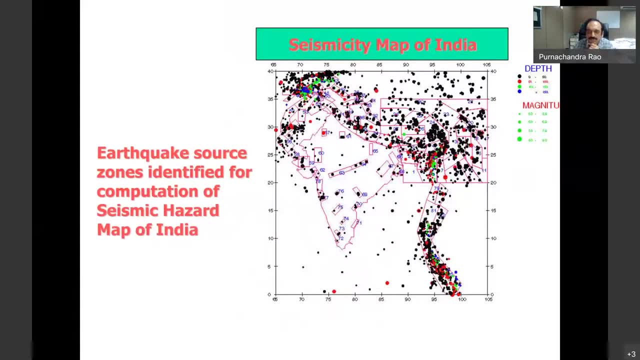 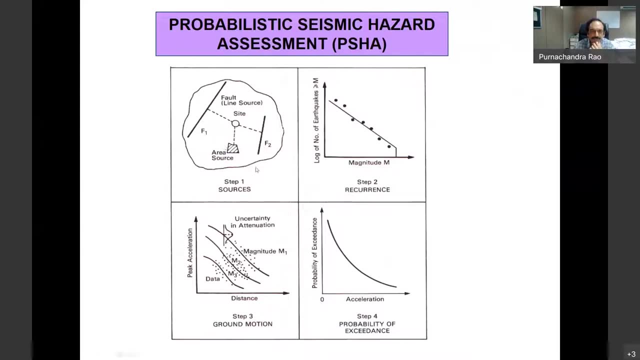 analyzed in order to compute a probability, probabilistic, hazard assessment map. so this is an example of how the seismic zones can be delineated based on their characteristics, and of course, there are various other things. like you have to: uh, from a defined site, what is the distance to each of these fault or the seismic zones we need to calculate, and then we 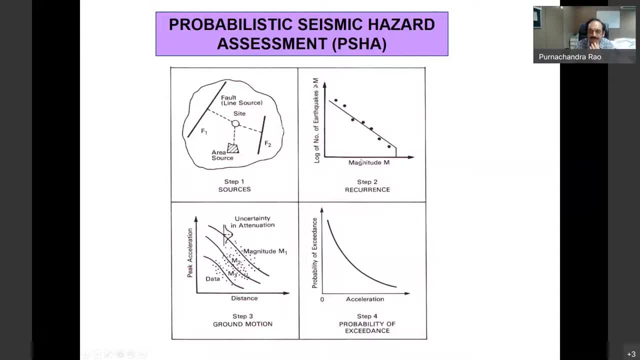 have to see the magnitude rate, the, the recurrence rate. that means uh, this is also called the gutenberg victor relation and which means, with increasing magnitude, how the number of earthquakes increases. the slope of this curve is an important parameter called the b value, which goes into the 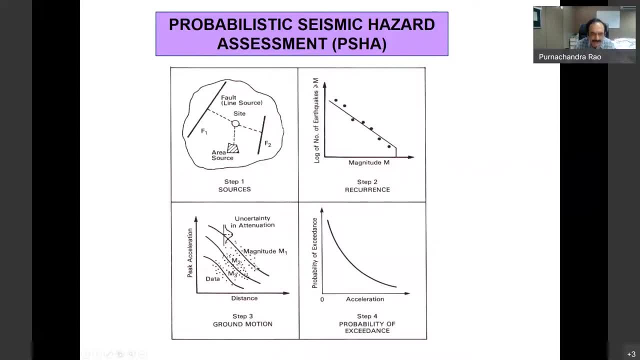 calculation and then you have to also see the the, the attenuation, how it is happening with distance. so this varies from place to place, depending on the structure of the earth in that area. and finally you need to calculate what is the probability that a certain level of acceleration 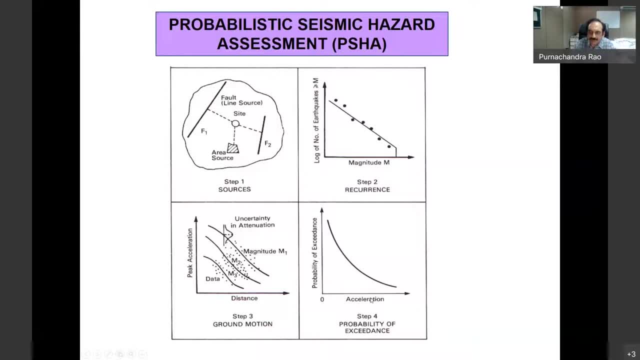 will increase. we define a level of acceleration for a certain region which we can tolerate, and then we calculate what is the probability that this level will be exceeded. so these are some of the technical aspects of calculating probabilistic seismic hazard assessment, and a lot of work is going on in this direction. so this is an example of g sharp, which 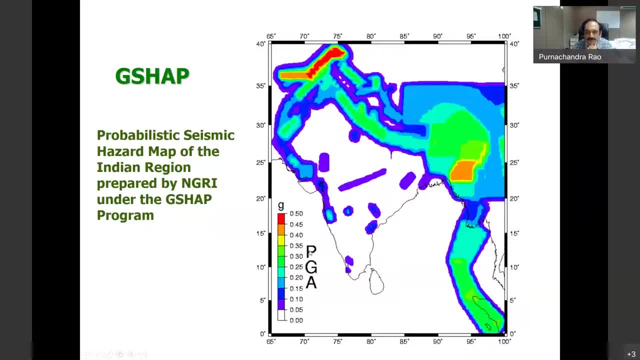 is the global seismic hazard assessment program, where we try to calculate the peak ground acceleration that can be expected in different regions and, as you can see, the red and the orange zones are the having the highest acceleration values, and then comes the yellow and the green regions, that is, the himalaya and northeast india. 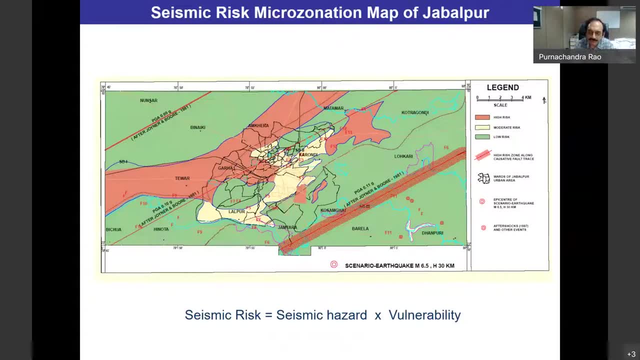 and if you go to a finer scale, when you take up a particular city or a town and do a very detailed study, very detailed analysis of the seismic hazard and risk that is called microzonation and this i am showing you an example of the very first. 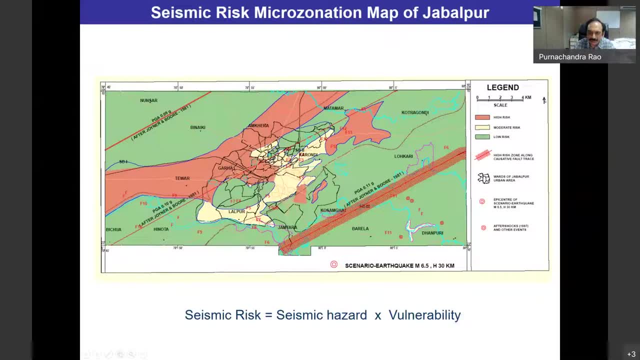 study done in the country in the 1990s from the city of jabalpur so you can see the different hazard levels that have been delineated for the city. and basically we need to understand that seismic hazard is just a computation of what might happen due to an earthquake. but at the end of the day, 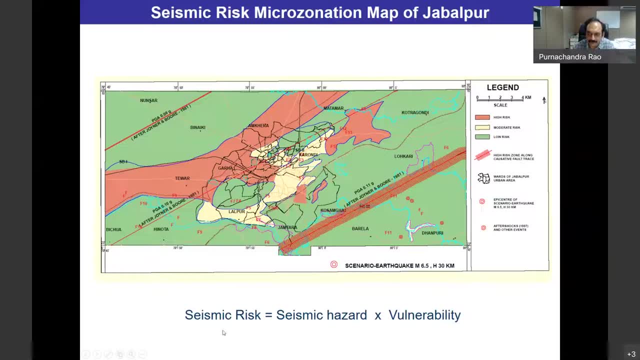 it's very important to know what is the seismic risk to the mankind. so to calculate that we need to get into vulnerability and the product of seismic hazard and vulnerability gives you the seismic risk of that region. so seismic risk directly relates to the public, the population, the 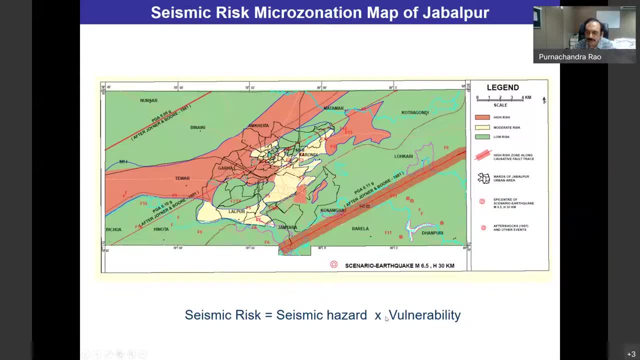 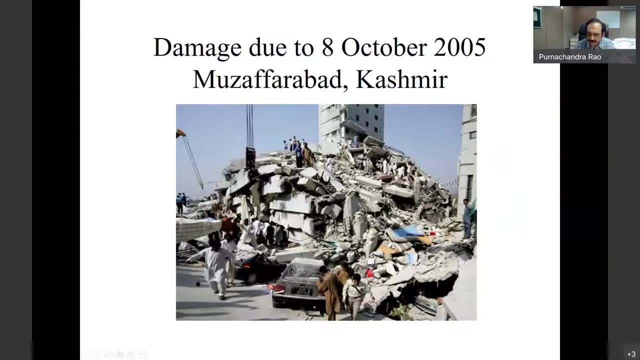 the dwellings and so on. so because if you have a bigger earthquake in somewhere in the middle of the ocean, it is not very risky. so that is the meaning. now, in spite of all these things, earthquakes keep happening and you have serious damages. this is an example of the kashmir earthquake of 2005, and you can see that even the magnitude was below 8. 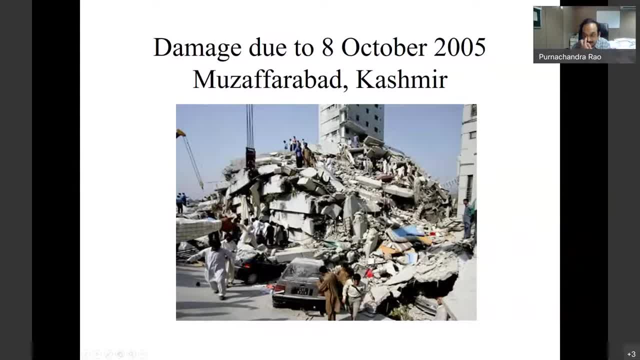 the destruction was enormous and more than 30 000 people were killed. so this essentially is because the buildings are very poorly constructed. so one very important uh take home here is that earthquakes do not kill the buildings do. so very important to construct proper buildings with the proper codes. 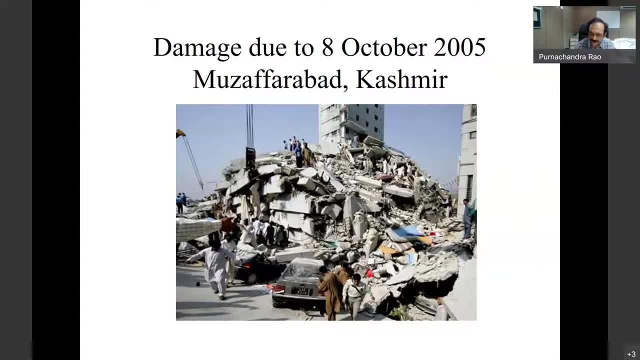 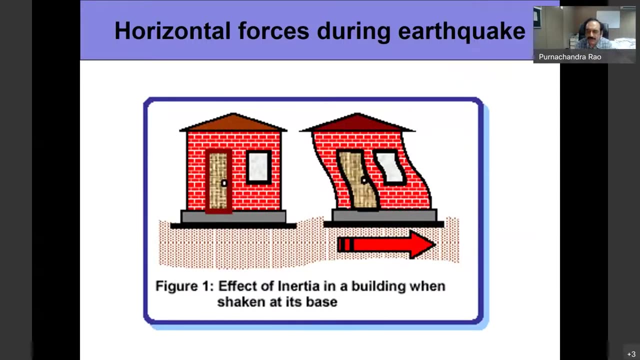 that have been prescribed, very, very important. so for every citizen, whether earthquake can be predicted or not, the buildings we should construct in such a way that we can withstand any earthquake that is likely to happen in that region. now, what is the main reason for the buildings collapsing? the main reason is that the most of the civil engineering, uh, the designs they take care of. 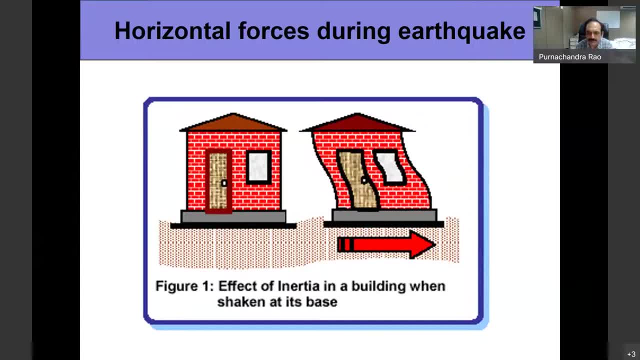 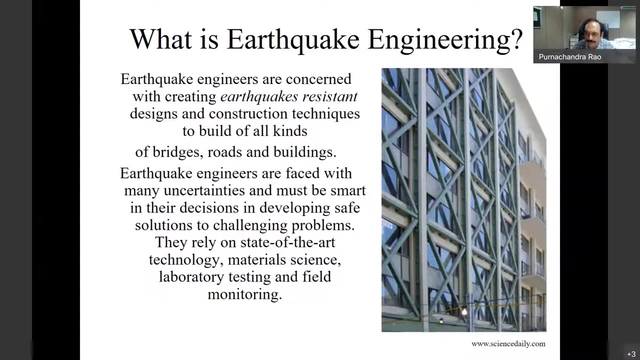 the vertical loads and not really the horizontal loads, and whereas the surface waves, they travel horizontally from side to side and this is precisely why the buildings collapse. so there are a lot of designs which come under earthquake engineering, which help to hold the building even if there are forces from the sides. so you can see this in this picture. you have this: the brackets. 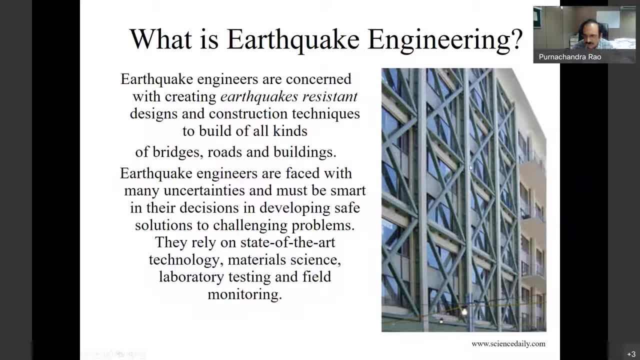 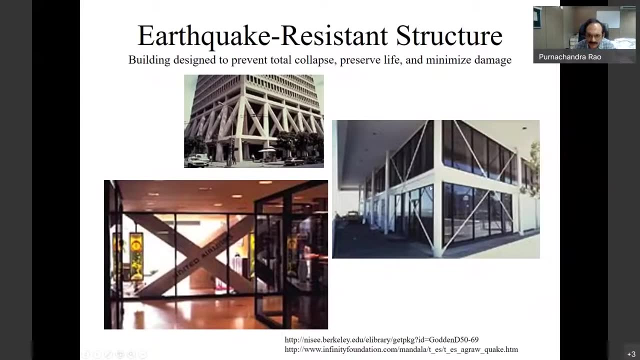 which are in the shape of x, so these are helpful in holding the square. otherwise it will deform and become a rhombus. so as long as the building stays like a square, it is safe. otherwise it gets deformed and it collapses. so these are some more examples of earthquake resistant buildings. so this is by. 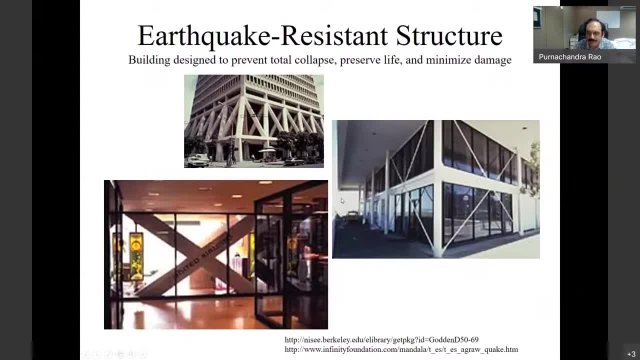 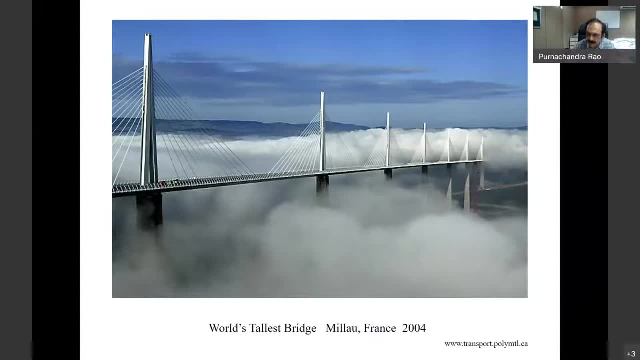 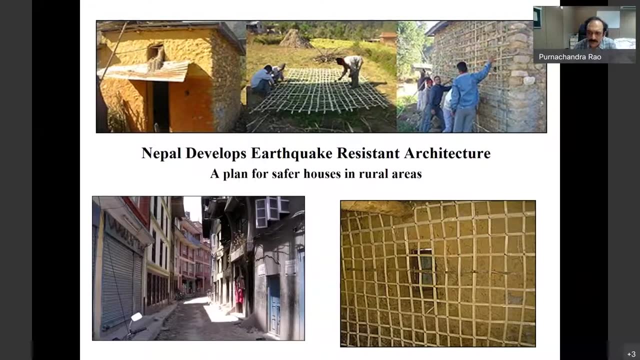 itself an important subject, where you keep construct buildings which are safe. now this is an example of the world's tallest bridge in france, which was made earthquake resistant with the same concept. now, even in poor countries which cannot afford expensive technology, is possible to have earthquake resistant buildings. so here you see an example where, using bamboos and 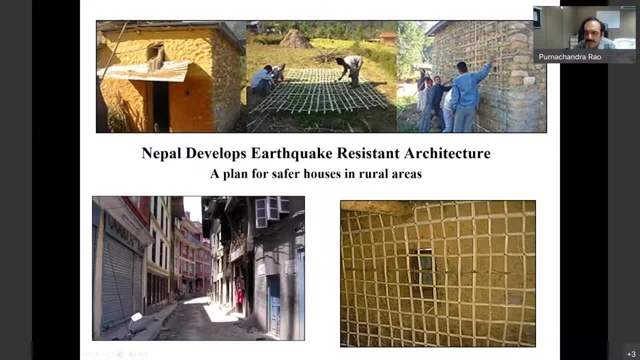 nails, it is possible to build a mesh like this which is directly nailed into the hut. so this is not a cement construction. very so it's very weak and in the in case of an earthquake it will not withstand. so this kind of simple techniques can also help to withstand any major earthquake. 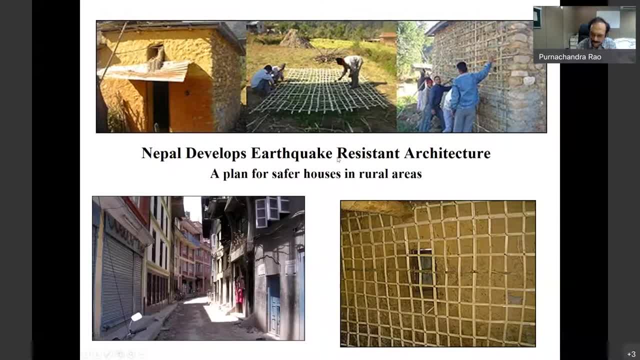 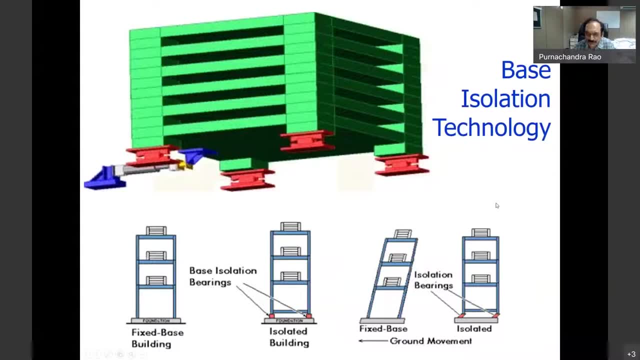 this is from nepal. in nepal, for example, they use this kind of protection. now, the richer countries, they can afford what is called the base isolation technology. so here what happens is the base is not fixed to the ground, but you construct the base of the building. 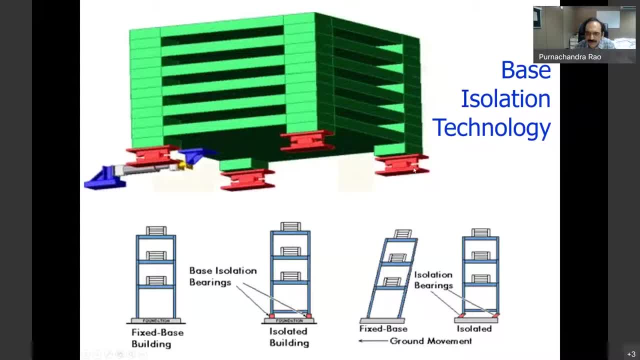 in such a way that whenever there is an earthquake, the building oscillates to the sides because because of detachment from these bases, and therefore it does not collapse. so this is a very useful technology, but also it's very expensive. countries like japan have adopted this immensely. now we need to understand the difference between, uh, what is earthquake prediction and what is. 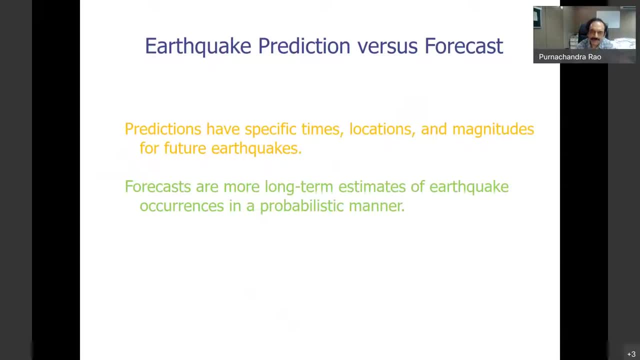 earthquake forecast. so, uh, prediction is a more specific thing where the date, time, location and magnitude has to be specified. so otherwise, if you say there is going to be an earthquake in himalaya, it doesn't make sense because smaller earthquakes they happen in himalaya almost every. 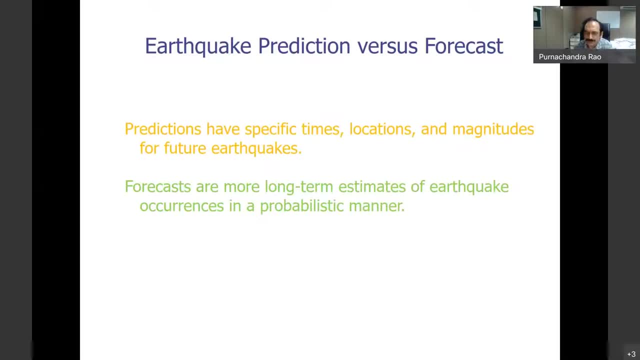 day if you go to the very small magnitudes. so a prediction has to specify the magnitude also in the location and at what time it is going to happen. so this as on date is an impossible thing, although people have tried and several people have claimed that they can predict. but let us. 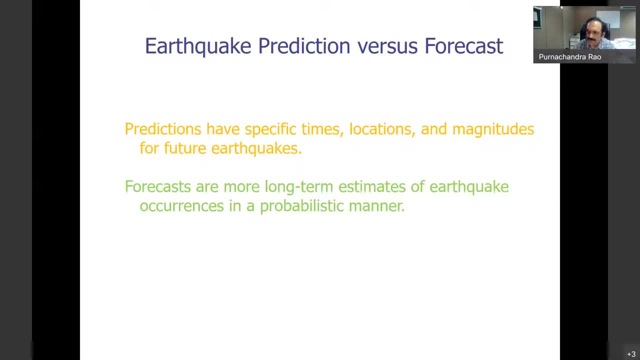 understand that there is no reliable, uh dependable, method as on date. now, what is a forecast? forecast is a slightly lenient thing compared to prediction. so forecast is basically where you observe a region, monitor a region for a long time and you find various precursory changes, and then you 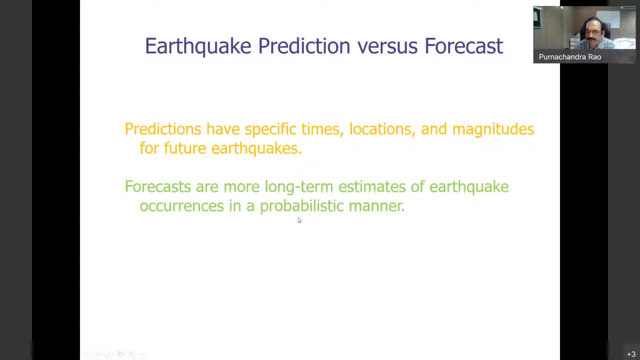 have a forecast that the region is developing stress and it's very likely that there's going to be an earthquake. so maybe in the next few weeks, or maybe in the next few months, so that sort of um. it's sometimes confused with prediction, but this is, uh, more appropriately called a forecast. 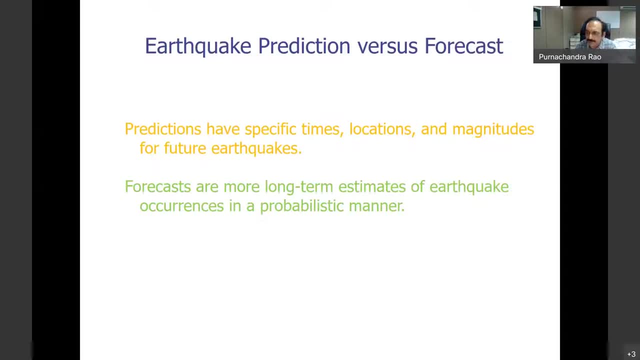 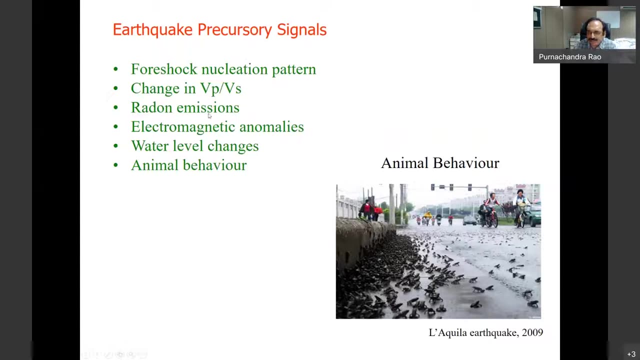 and i will show you some examples of forecasts that we were able to do in the koina region of maharashtra. now, the earthquake precursory signals. there are several signals, because before an earthquake you find a lot of changes. uh, for example, four shock nucleation. 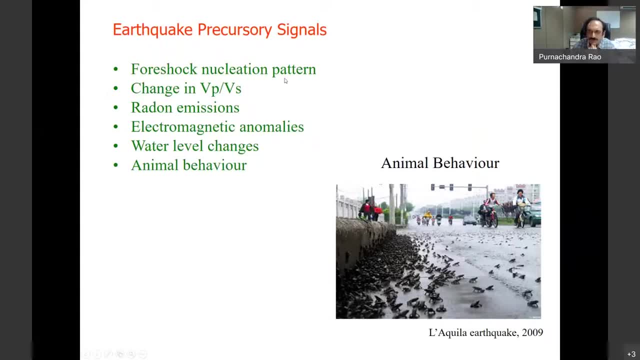 pattern. that means the earthquake, four shocks, suddenly increase in some areas and then there is a quiescence before a major earthquake happens. this has been reported from various places. and then there is a change in the ratio of p wave and s wave velocity in that region, or you have emission of gases. so this is possible if the region is stressed. 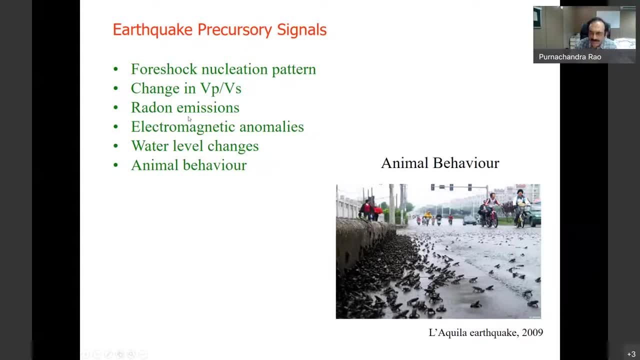 and somewhere already fractured, it is possible that gases from within can escape and come onto the surface. then you have electromagnetic anomalies. i will show you some examples later on. and then water level changes, for example if there is a squeezing of a region, the water. for example, if you are monitoring some boreholes, you will find that suddenly the level is increasing. or 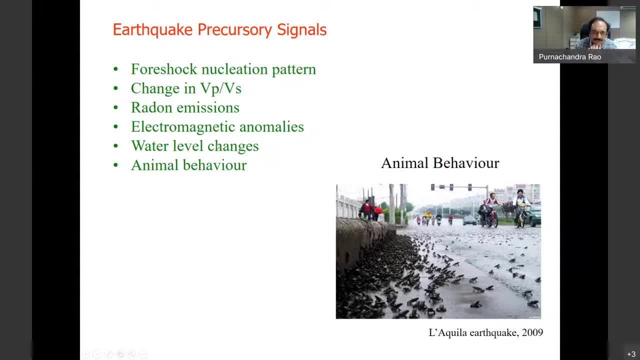 decreasing depending on some tectonic squeeze or force. and lastly, we have animal behavior. there's been a lot of research on animal behavior. several animals seem to be sensitive, but unfortunately we don't utilize any of these because they are not very reliable and they keep changing from time to. 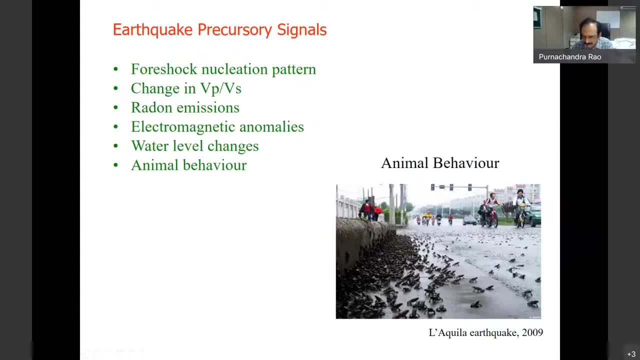 time. so it's very hard to depend on behavior of animals to make a prediction of earthquakes. so so these studies are still going on. all these precursors have been studied and are also being studied right now, but we have still not reached a concrete stage where we can forecast or predict earthquakes very confidently. now let's look at the past: whether there 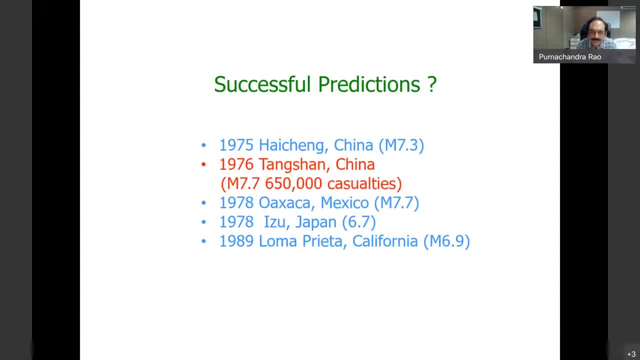 have been some successful predictions. in 1975 in haicheng, china, a magnitude 7.3 earthquake was predicted and it came true. and since all the since, it is in china and they could manage to convince all the people to evacuate. so it was regarded as a very successful prediction. but the very 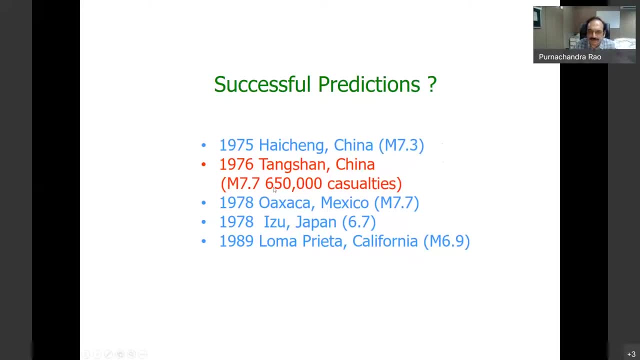 next year in tangshan there was a 7.7 earthquake and 6.5 lakh people died, and there was absolutely no clue that this earthquake is going to occur. so this raises questions whether we are really very clear on the methodology or is it more of a? 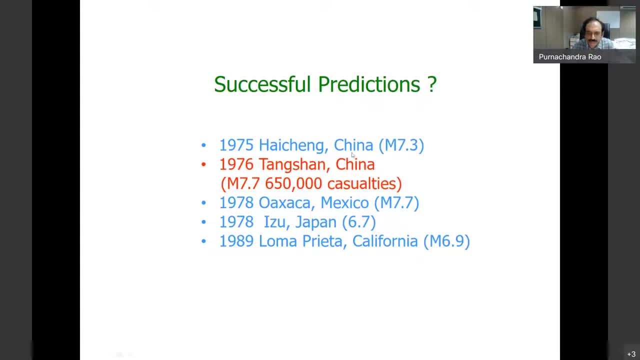 fluke, some kind of a fluke that we could manage to predict anyway. subsequently, some predictions have come out true. you had one in mexico, one in japan and one in california. these earthquakes have apparently been predicted. but again the same problem: the methodology is not very clear. 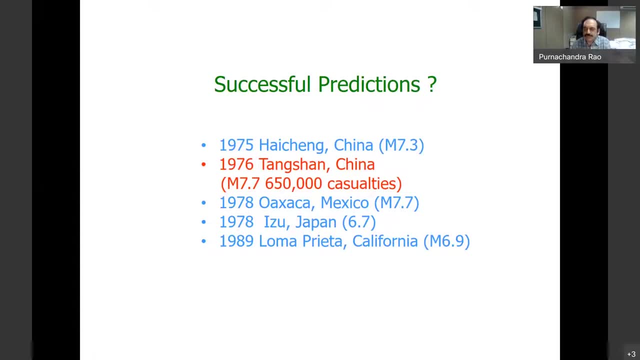 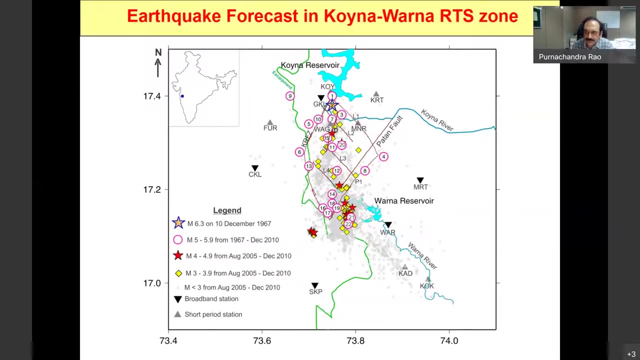 so we cannot claim that, yes, earthquakes can be predicted. it's not like that. now i'll give you a few examples of precursors that were monitored in the koinon region. uh, i was the project leader. uh, for about almost about 10 years, we worked in koinon region, where 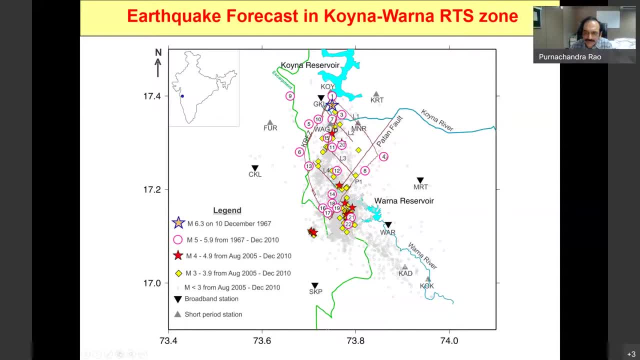 we have an excellent network of seismographs which are monitored in real time, so we get data in real time to ngri, hyderabad. i did not go too much into the details, except that kohinoi is the world's number one site of reservoir triggered seismicity, and that's the reason why we have been studying. 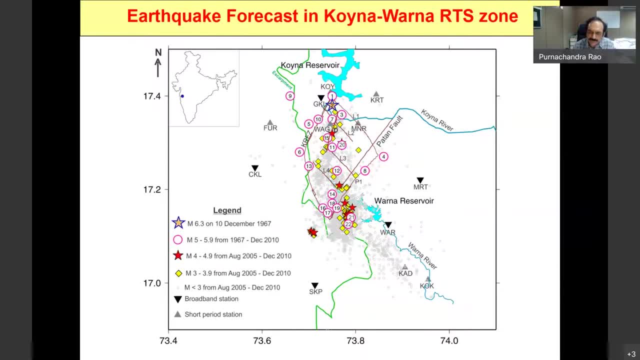 these earthquakes here and that's why we have been studying these earthquakes here. now i'll show you some data which shows clear-cut precursory changes before an earthquake. so a precursory study was done using various aspects, not just seismology. we also try to monitor the gravity field- we monitored. the electromagnetic field- we monitored. 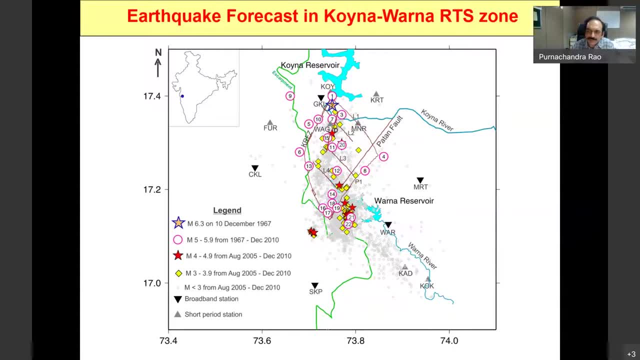 the gps. we monitored the water level changes, we monitored the hydrochemistry and so on. so many things we try to monitor in order to see if there can be changes noticed before earthquakes. so i'll just show you some examples now you can see. these are the different boreholes. 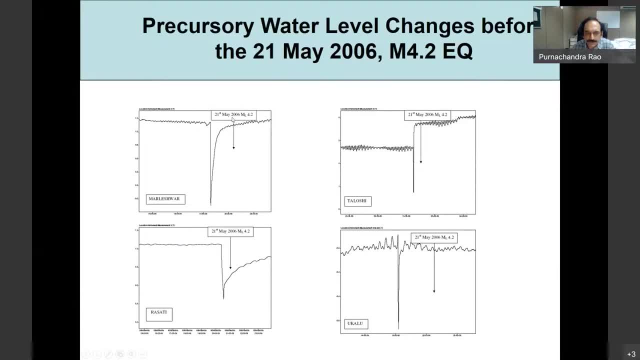 and prior to an earthquake of magnitude 4.2 in may 2006, we could see a drastic drop in the water level. see, there are four wells- bore wells- and in all the four we could see a very drastic drop in the water level. and this usually happens if there's a tectonic stress, a squeeze on the 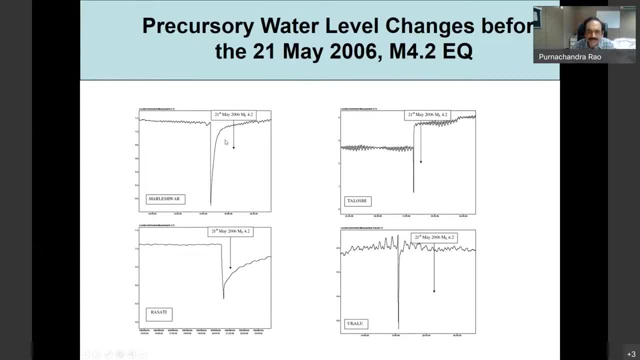 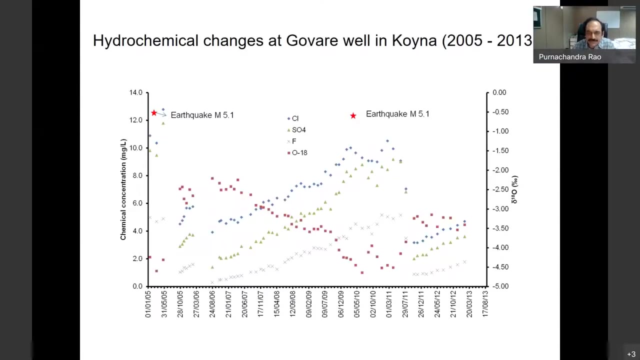 medium. but it's important that you should monitor this in real time so that you can in in real time. if you don't do it, then you miss the signal. so real-time monitoring will help us to make a forecast that an earthquake is going to happen. similarly, hydrochemical changes. 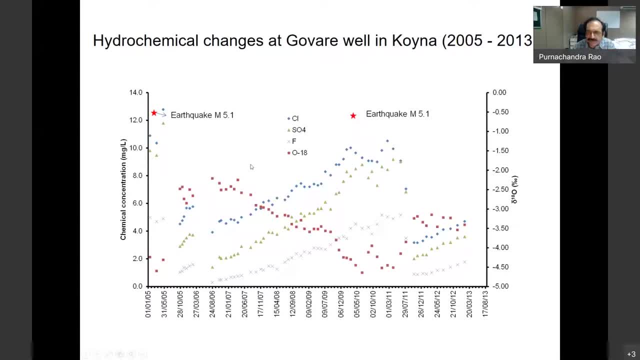 this is really very convincing because not just one chemical, but various, like you have the chloride, sulfate and fluoride, and you have also have the oxygen isotope. that the the content of the chemical concentration. it changes over a period of time and, what is interesting, we find that between two 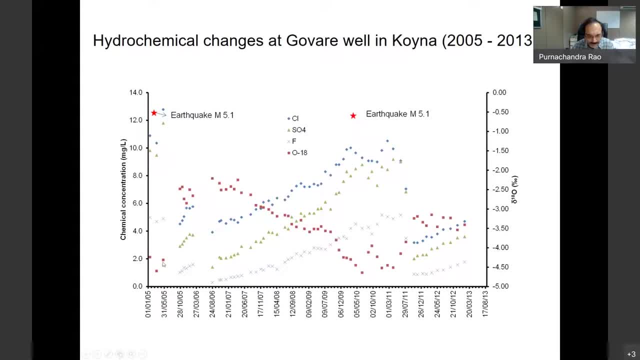 earthquakes of magnitude 5 that occurred in koina, we could find that, uh, there's a sudden drop in this. for example, if you take the o18, there's a sudden drop prior to the earthquake and then there's a rise after the earthquake. and if you take the chloride, for example, there's a rise and. 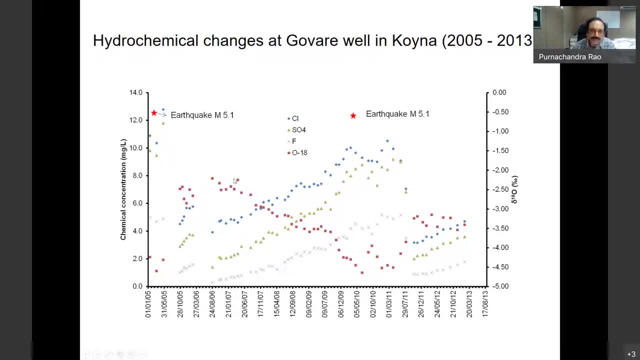 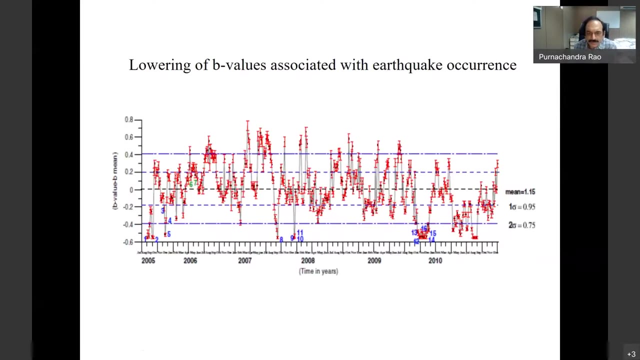 then there's a drop. so the anomaly is very clear for whichever component you take and using this data, this earthquake was predicted, which occurred in 2009. this earthquake was predicted, or rather, i would say, forecasted. similarly, we find that there's a lowering of the b value. you can see these blue colored numbers. 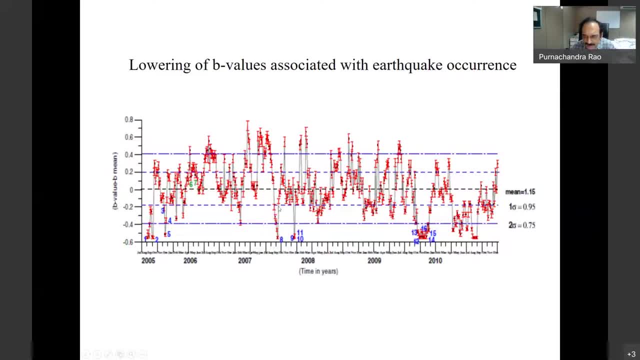 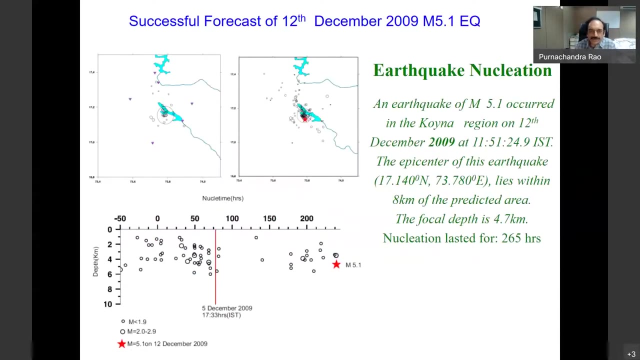 you will find that the b value is lowest just prior to, or maybe exactly during, the occurrence of earthquakes. so we found almost 70 percent coincidence with the lowering of b value during an earthquake occurrence. similarly, we found this nucleation was a very successful thing: the clustering of earthquakes prior to a few days before the occurrence of a. 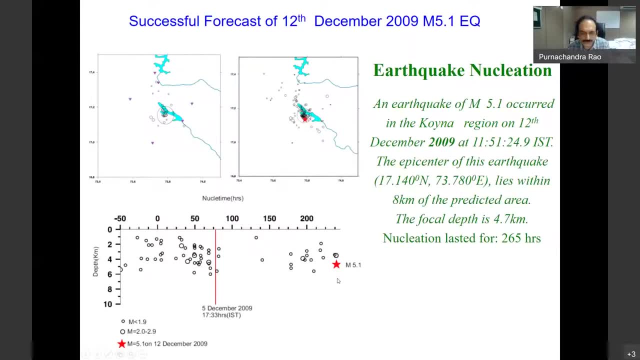 larger earthquake. so in koina, large earthquake means four or five magnitude because, uh, it's not a plate, a tectonic plate boundary, so please bear with that and similarly so. this is the list of earthquakes that were forecasted. at least four earthquakes we are. we were able to forecast. well. 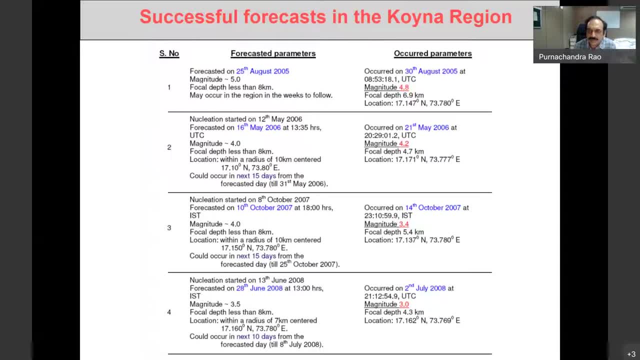 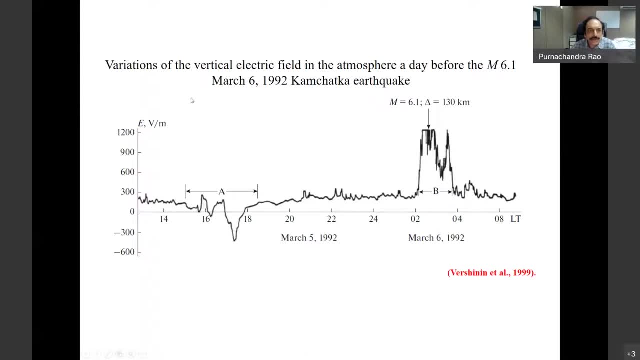 in advance and this was published before occurrence of the earthquakes. similarly, i'll show you some outside india also we. it's found that there are variations of the vertical electric field in the atmosphere few days before. this is for the kamchatka earthquake. you can see here that the electrical field is the sudden change. now i'll also explain. 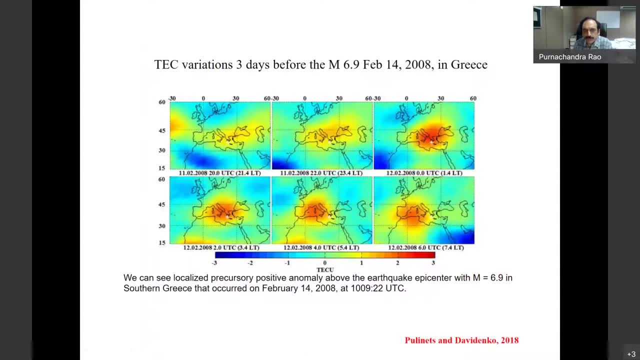 why these things happen now. for example, this is the total electron content in the ionosphere. so it is found that in the region of the earthquake suddenly the tec changes a few days before the occurrence of earthquakes. so now a lot of people are working on this one, so there are a lot. 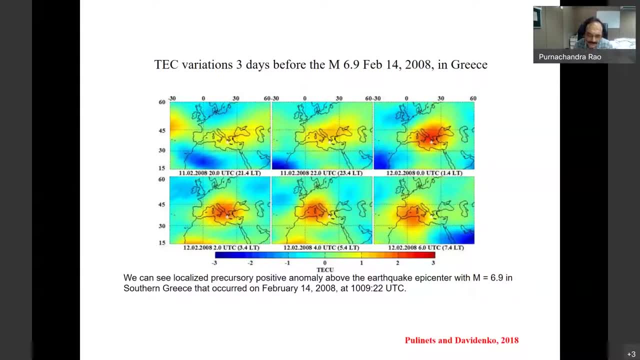 theories as to how this happens, and one of them is that the earth, when it gets stressed before an earthquake, so it also behaves like a piezoelectric substance that generates an electric field of its own, and this goes and interacts with the ionosphere, where the tec suddenly changes. so 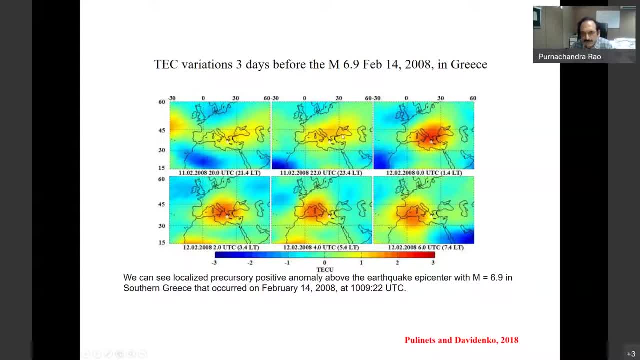 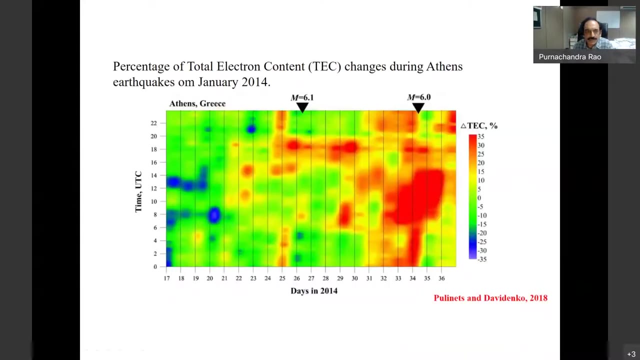 you can see here, three days prior, how the tec is gradually changing over this. uh, this white plus is the earthquake location in greece. so the the change is very, very clear just before the occurrence of earthquake. so three days prior, this kind of thing was observed here also. you can see. 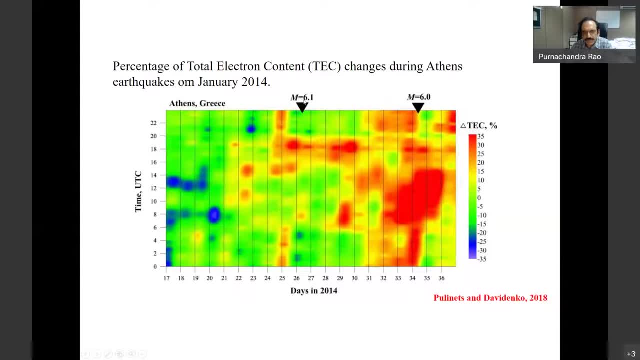 as a function of date, that before the 6.1 earthquake and the sixth earthquake the tec count has suddenly changed here and here also. but then you will find that for this first earthquake the change is less, for the second one it is more. so these are some of the challenges every time. 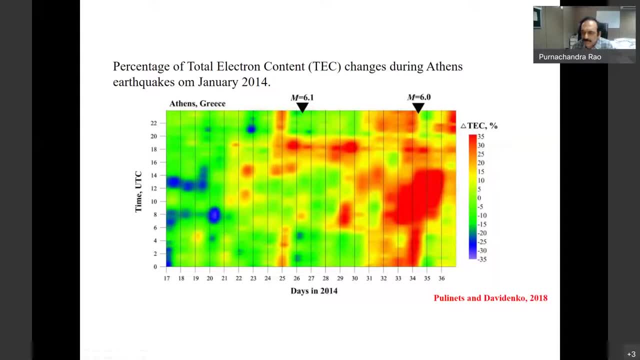 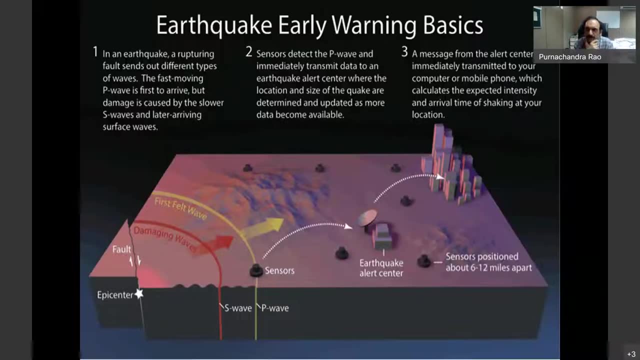 you don't get similar results, so how you are going to rely upon these observations to make any forecast? that is the biggest challenge that we face today. now, earthquake or early warning is a possibility, and countries like japan and mexico are already utilizing this. so here the concept is that, since 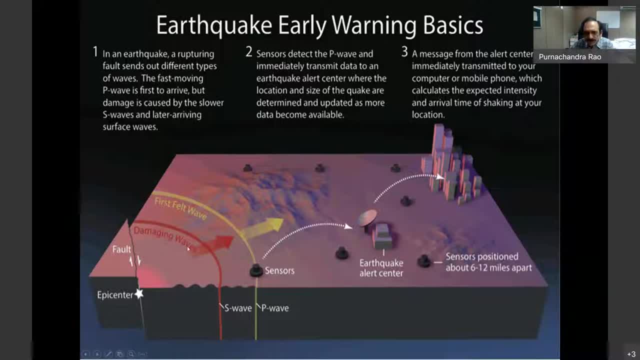 the p wave arrives first because p wave travels with about six kilometer per second velocity, compared to the surface waves, which are less than 3.5 kilometer per second. so before surface waves arrive, the p wave arrives several seconds before. so if in real time you can automatically analyze, 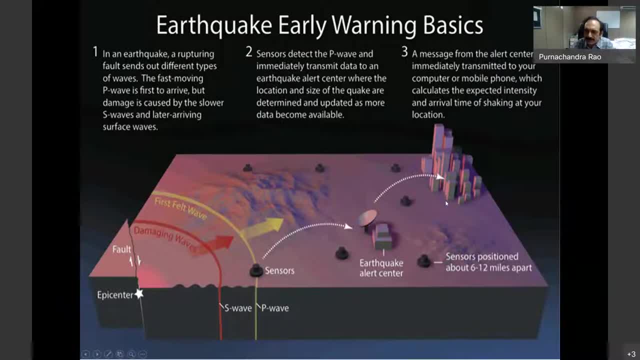 the p wave and then find- i find out that the earthquake is approaching, then you have something like 5 or 10 seconds time, depending on the region. so these few seconds of warning- sometimes even that- can be very useful, for example, if you have a super fast train that is traveling at a very high. 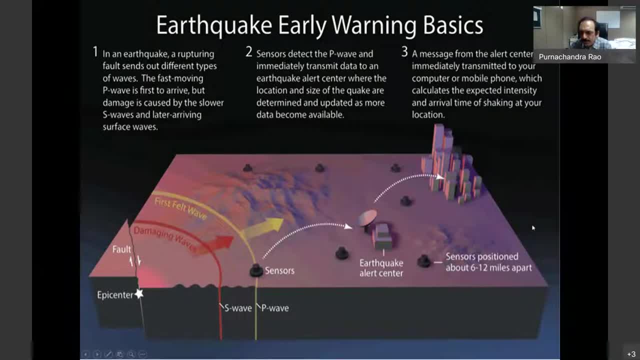 speed, so at least the driver will have time to apply brakes and bring the train to halt so that the damage is reduced, or if some nuclear power plant has to be shut down, or if there's some major surgery going on in some hospital, so things like that. so this is not the extreme, it's not extremely. 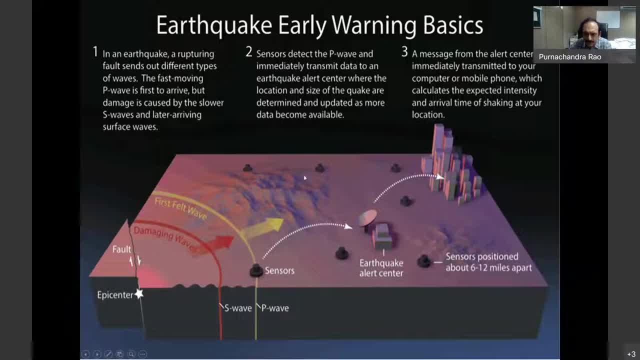 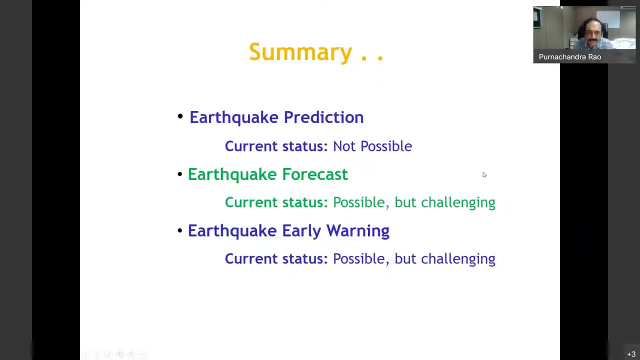 useful, but nevertheless it is useful, provided we have the technology and we implement it properly. so in summary, i would like to say that the earthquake prediction: current status: it's not possible. earthquake forecast: the current status is: it is possible, but is very challenging. earthquake early warning also is possible, but very challenging. now these 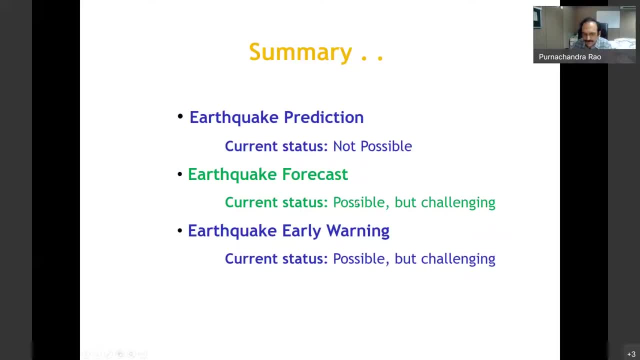 two challenges are different. that's an interesting thing to notice that the challenge in earthquake forecast is different from the challenge in early warning. in forecast, the biggest challenge is to find consistent precursors, precursors which do not, i mean which behave in the same fashion every time. 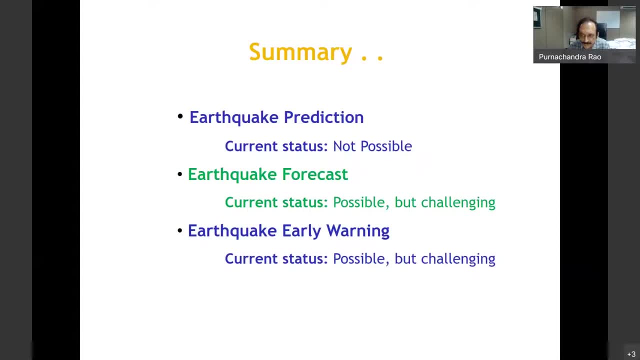 so, so that we can rely upon. otherwise there will be false alarms, we'll issue a forecast and then it doesn't happen. so the biggest problem is: if you go on making false alarms, then people don't trust you. so next time, even if you make a correct prediction- 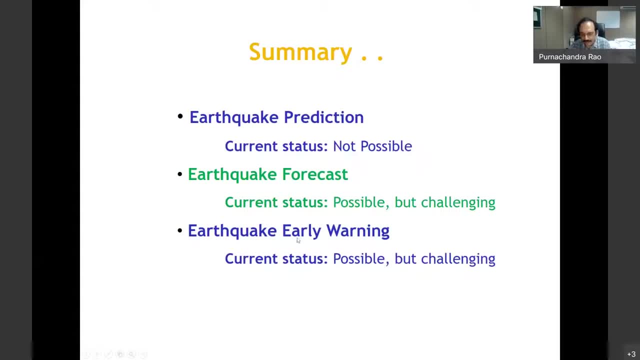 people will not believe there is a challenge there and in early warning. the biggest challenge is to have the best technology so that you have a maximum possible warning time, and the second challenge is to educate people and to interact with the stakeholders about how we can utilize this very limited time. 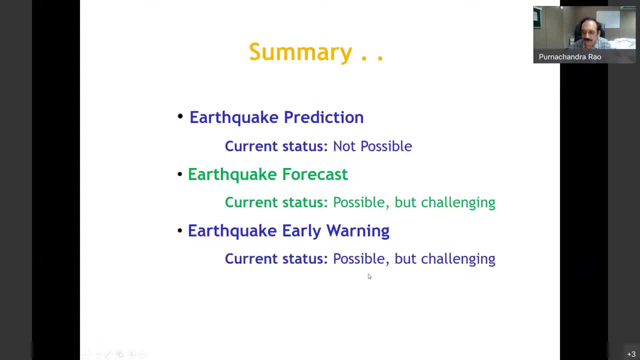 in order to, you know, protect ourselves from the earthquake. so very small time is available during early warning. how to utilize that? one success story in the country was, i think, csio uh chandigar. they have done an experiment for the delhi metro where, when there was this afghan earthquake, 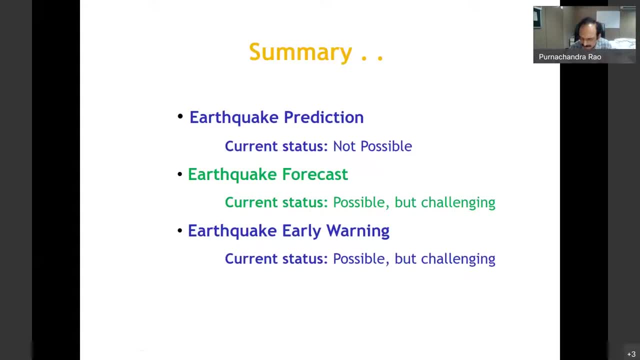 which was felt in delhi. i think all the metros trains could be stopped just in time. so it was a trial basis. it was done and i think it was successfully. but we still need to progress in the field of early warning. we need to a lot more. 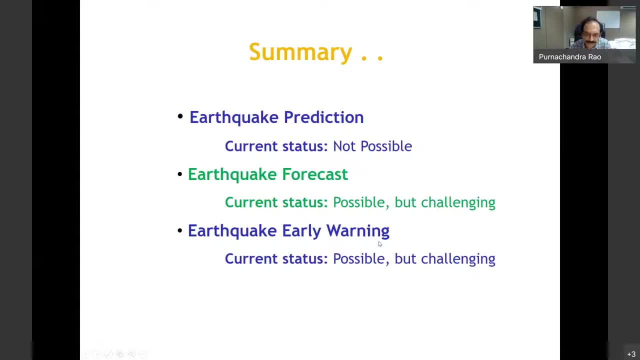 uh, i think there is one field where we are lacking, uh, right now. so, uh, with this i will conclude, but i must also mention that tsunami warning, because a lot of people are confused. although tsunami is caused by earthquake, tsunami warning actually is much easier because there you have a lot of time, depending on the region, like an earthquake. 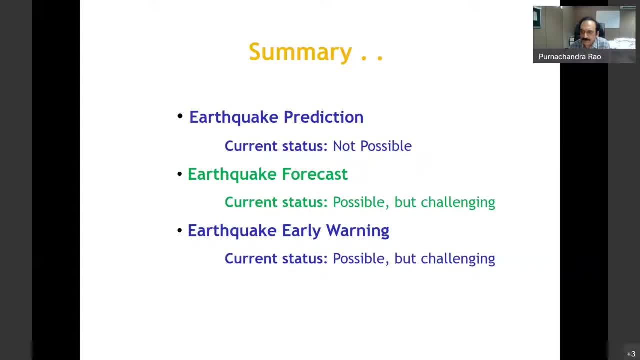 in andaman or sumatra. if it generates a tsunami, you have something like two to three hours time before the tsunami reaches the coast. so tsunami warning is much easier actually compared to any of these other things. and now we are also able to do flood warning, like i presented in my last talk. that 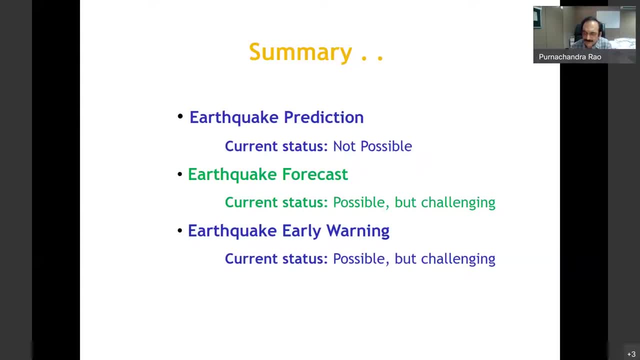 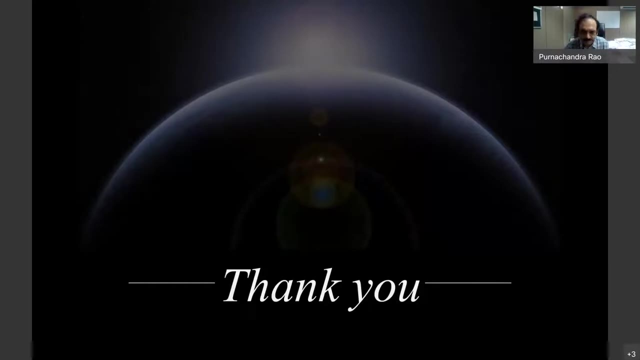 using seismic monitoring, it's possible even to track the floods and to give an early warning before the flood arrives at any point. so this is what i would like to conclude as far as earthquake is concerned. thank you very much for your patient hearing. thank you, thank you. 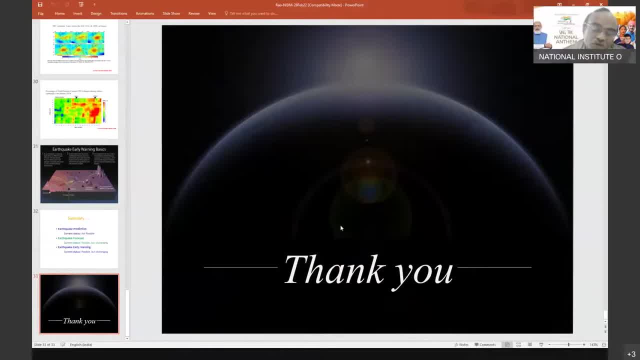 uh. dr kuran chandra very informative talk what he says, that it is very, very difficult to predict in uh in in advance, but a lot of works still that indian leading institutes are doing and it is going on. so let me check please if any question is there or not. 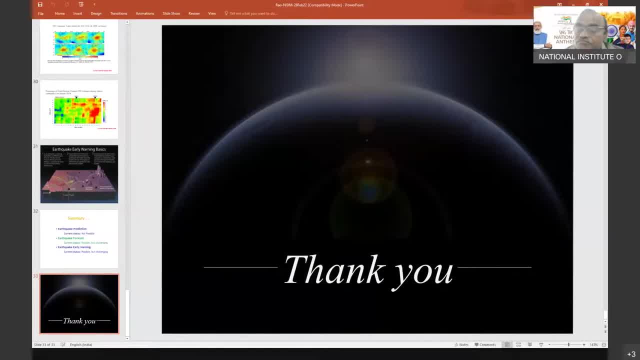 okay, so far, no, no question is raised by any of our participants leave, so that that's fine. yeah, thank you very much. thank you, dr elder, for this opportunity. Yeah, Though you are busy so much, but still you have kept your promise to make a little adjustment. 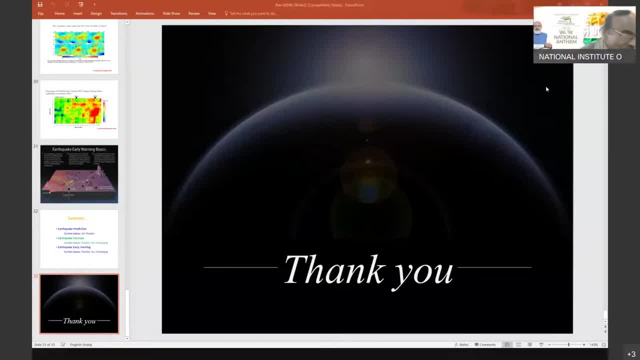 And thank you very much. Thank you so much. Now we will go to the second lecture, that is, with the Professor HM Datta. that is earthquake precursor detection in the Indian context. So, Professor Datta, he is a – just one second. 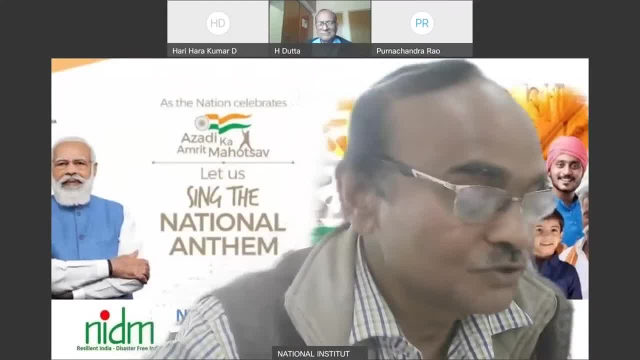 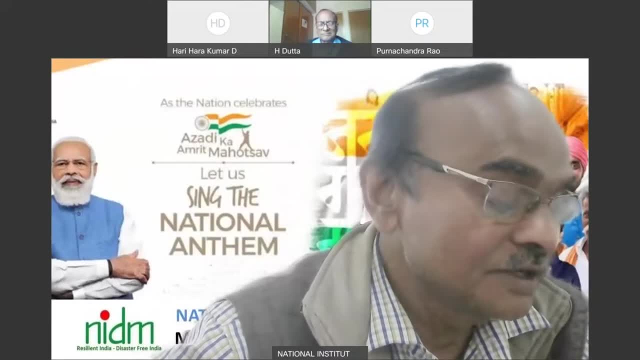 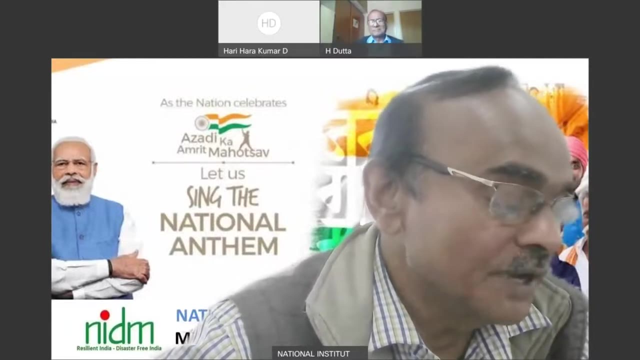 Professor HM Datta is a former principal scientist from CSR National Physical Laboratory, New Delhi. Of course he got retired quite some time back where he designed and developed various types of acoustic radars. So these radars give photograph in the air right from the surface of earth to a height. 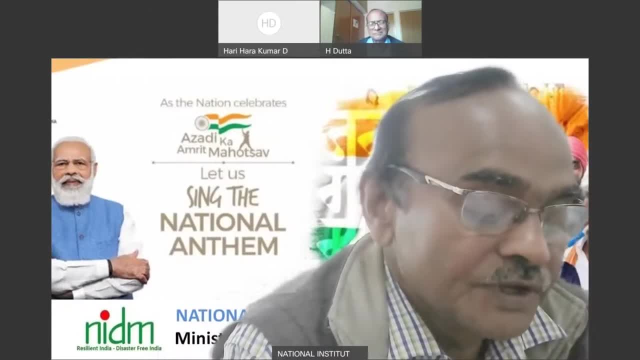 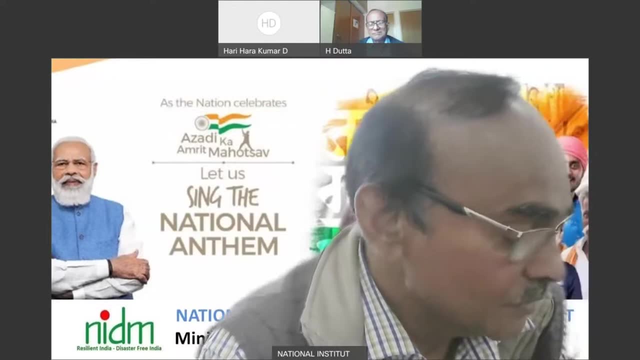 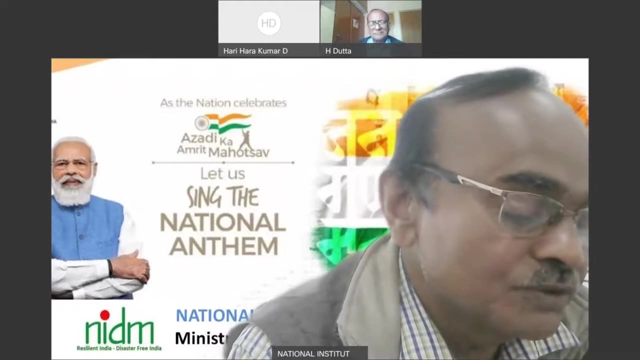 of 1.5 meters, One kilometer on continuous basis. So he established a chain of these radars in India, Antarctica, on both various sheaths and sailing over the Antarctic Ocean, and even exported to other countries. Thrice he led to CSR, National Physical Research Laboratory, NPL terms in Indian Scientific 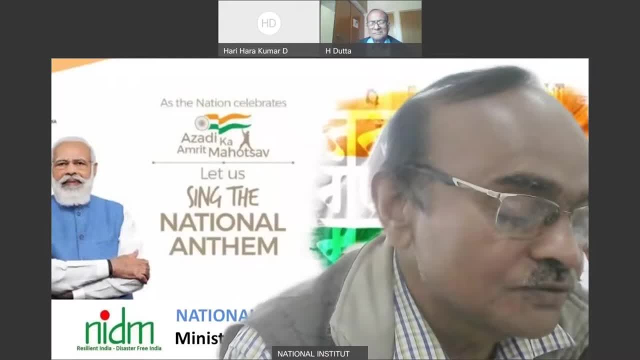 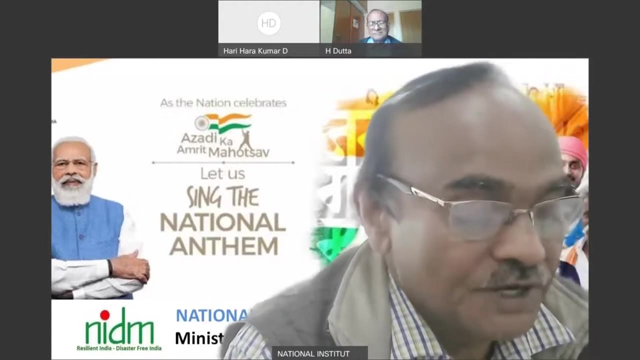 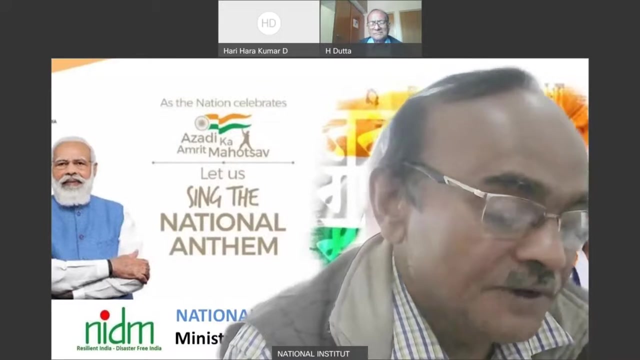 Expedition to Antarctica. He holds to his credit three science and technological contributions for the first time in history of mankind. With his vast Antarctic experience, Dr Datta led team for inducing acoustic radar as a technology for the detection of precursor of earthquake 24 hours in advance. 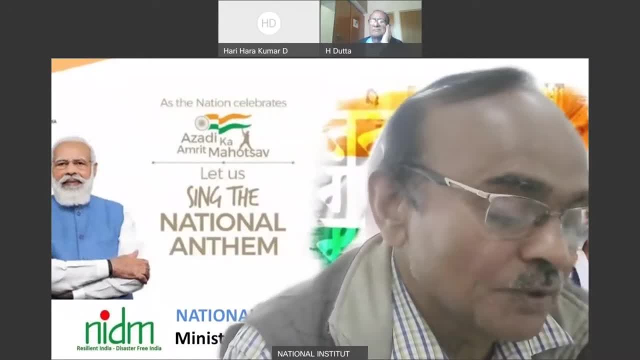 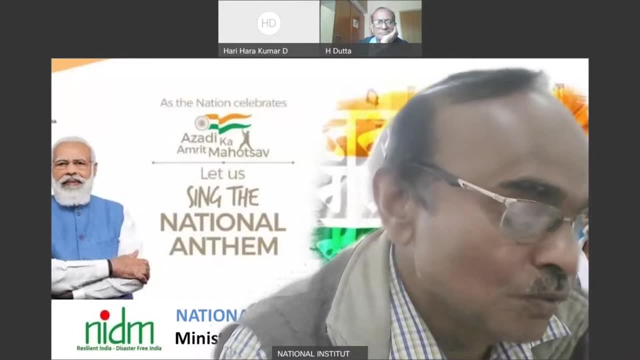 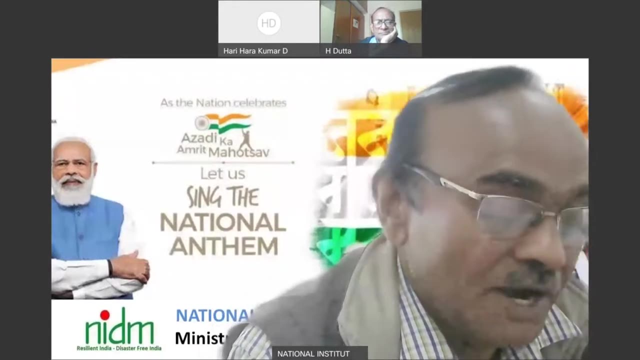 And patent has been granted by the World Intellectual Property – property, and Dr Datta is currently is only Indian who presented India's scientific and technological might in the Republic Day Parade at Rajput, New Delhi. He is the first in the world to design, develop and run ship-borne acoustic radar over the 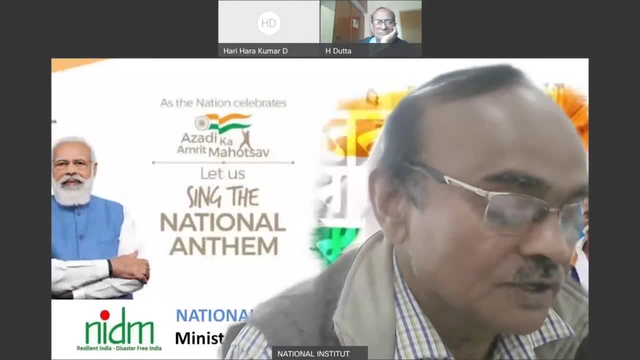 East Antarctic Ocean. He served as the Founder Director REM Tech, SAMLI, and then served as a Professor of Electronics and Engineering in Swami Vivekananda Swabharti University, Mirat. Dr Datta worked as an Advisor of Research and Development in the Silver Line Prestige. 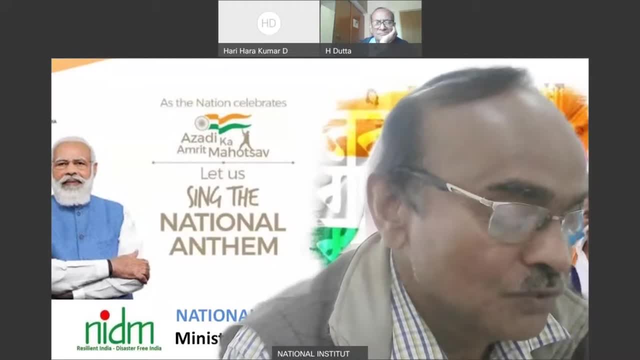 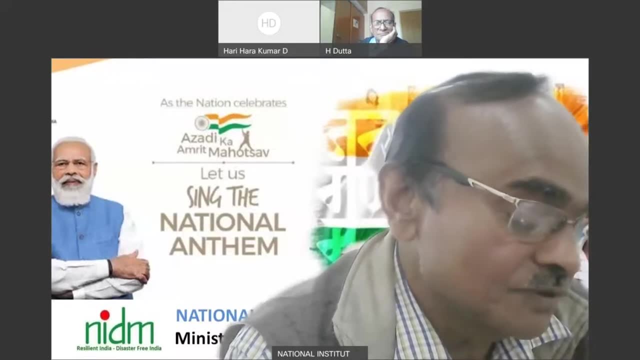 School, Ghaziabad, and presently he is Senior Advisor of Subram Technology Pvt Ltd, New Delhi, a company dealing with the defense, research and development. Dr Datta has transferred acoustic radar technology to various companies in India and holds a copyright. 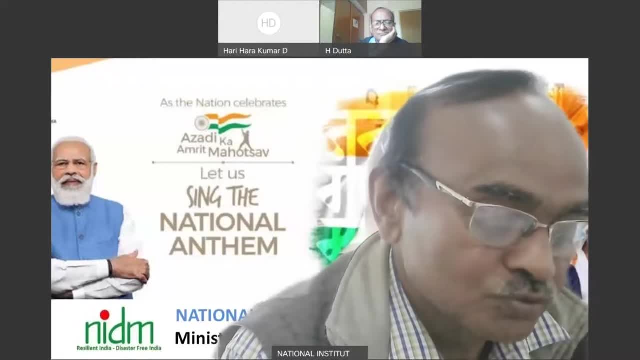 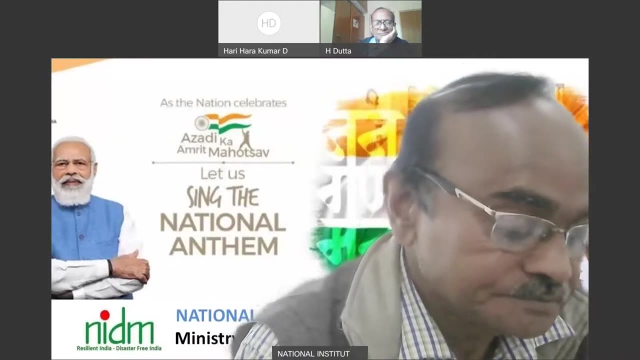 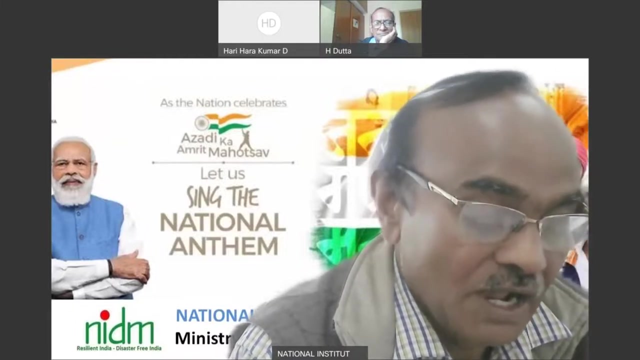 on the optical illumination laws, a new thought inducted for the first time in the history of mankind. Dr Datta has supervised nine PhD theses on the atmospheric dynamics and has the book on Antarctica. His important contribution is the publication of book on Antarctica, The Most Interactive. 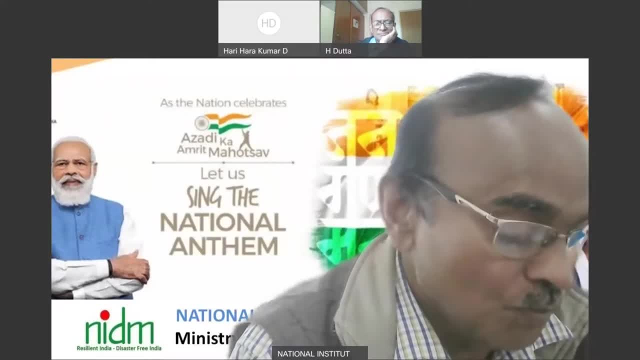 Ice-Ear Ocean Environment from Nova Science Publishing. Dr Datta is the Founder Director REM Tech, SAMLI, and presently he is Senior Advisor of Subram Technology Pvt Ltd, New Delhi, a company dealing with the defense research. 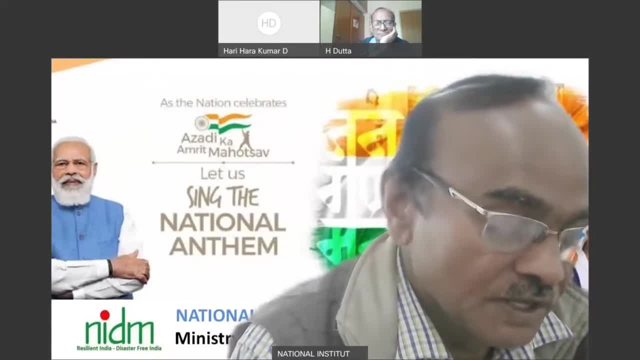 research and development. Dr Datta has a stake in nature and he has been working with the National Science Foundation on this topic since 2016.. In the past, he had worked for the National Science Foundation of the Indian Ocean USA. 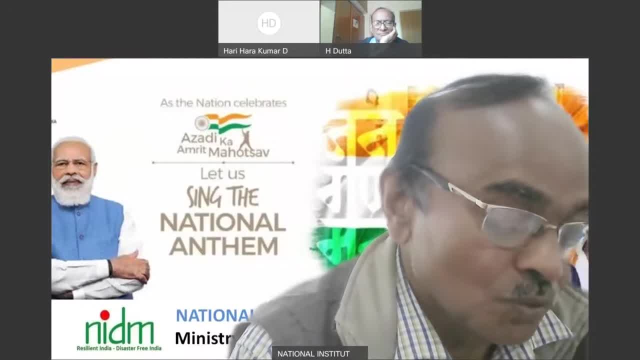 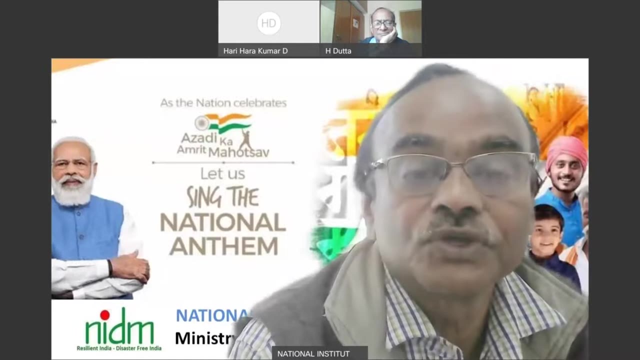 With this vast experience, Dr Datta is elevating India as a top writer on Quoracom, where he answered 1,900 questions quite fast on subjects like Antarctica, earthquake or atmospheric sciences, which have more than 16 lakh views. 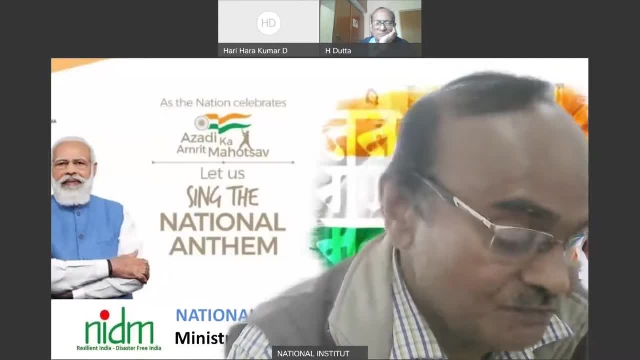 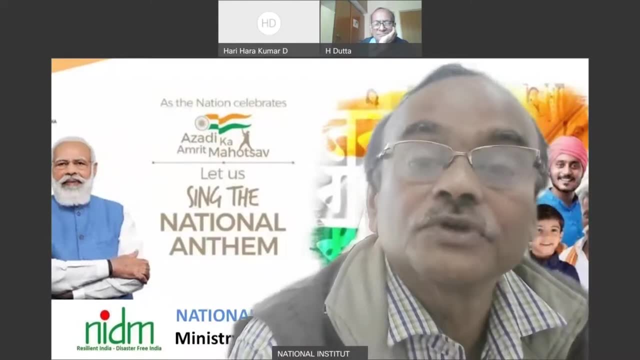 So he is having vast credentials in his life and he is having full enthusiasm still. work in the field of the Campus, Science, the Principle of Science and the Education of Science, work on this field. earthquake and radar also Now. with this I would request Dr Datta 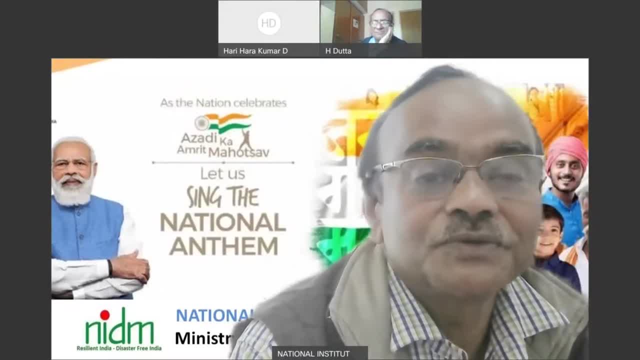 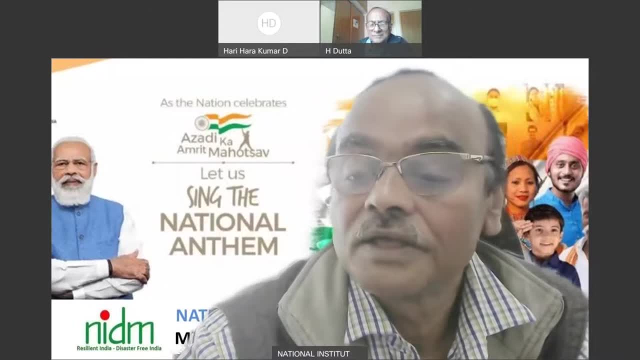 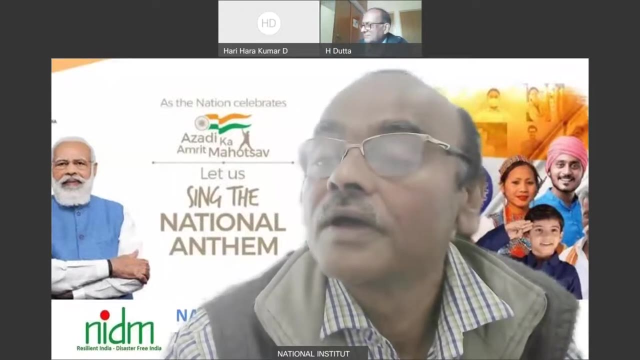 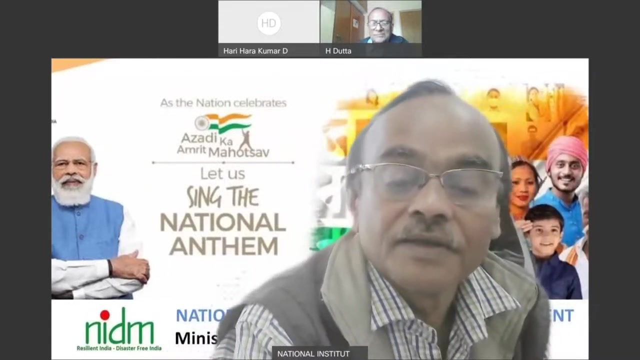 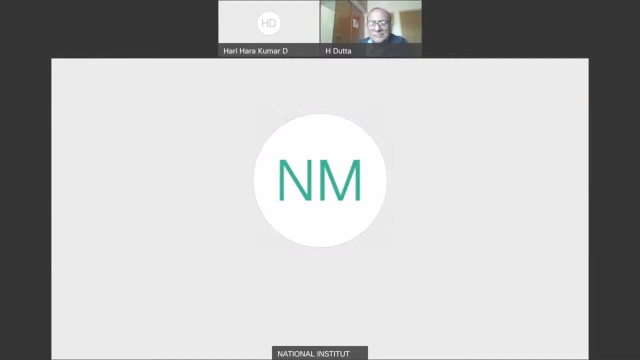 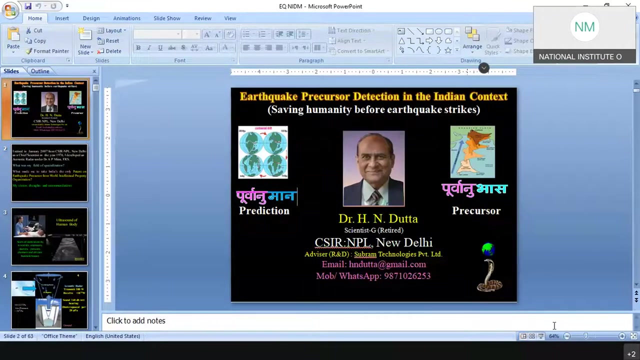 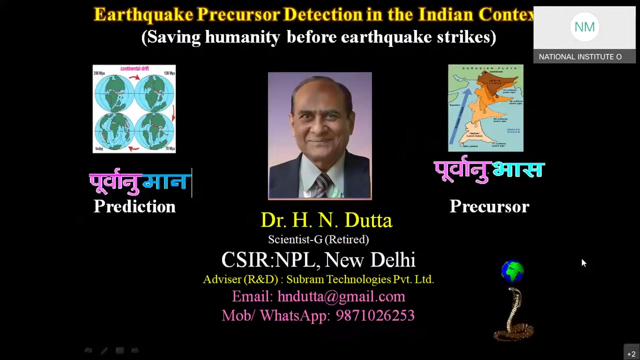 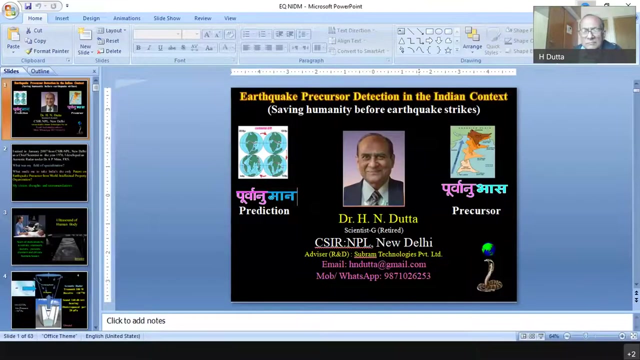 please take the stage and continue. please continue his webinar, Dr Datta, please, You can load your PPT. Good morning, Is it visible, sir? It is visible, very much Okay, And voice is clear. Yes, it is clear, sir. 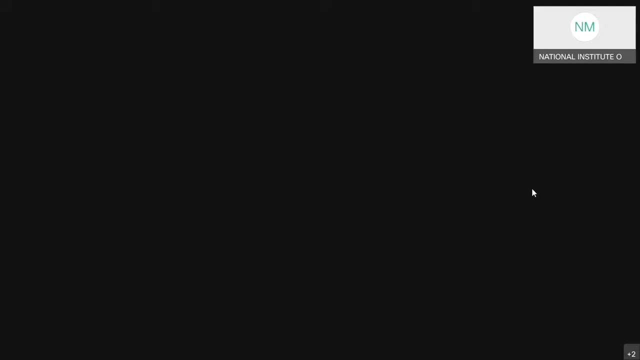 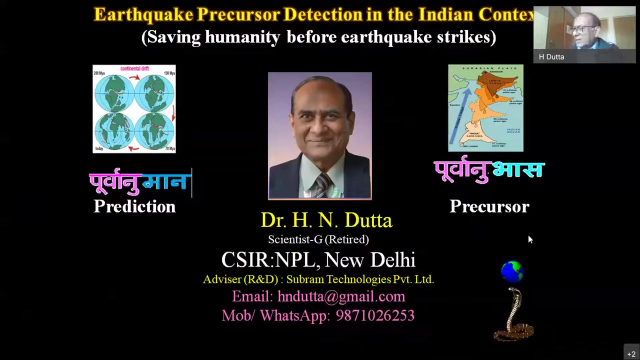 Okay, Okay, That's fine. Just a minute, sir. Yeah, Okay, Okay. So good morning everyone. Honorable Dr Surya Prakash, Honorable Dr Haldar, distinguished members from various organizations and dear participants. 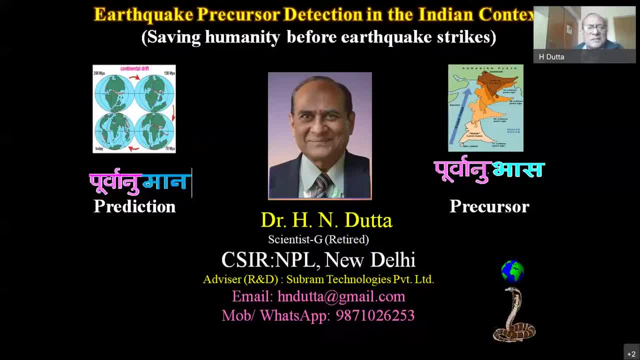 While I speak on a very, very complex subject- earthquake precursor detection in the Indian context- let me confide that I have absolutely. I had absolutely nothing to do with seismology or earthquakes. I'm basically a designer of various types of acoustic radars. 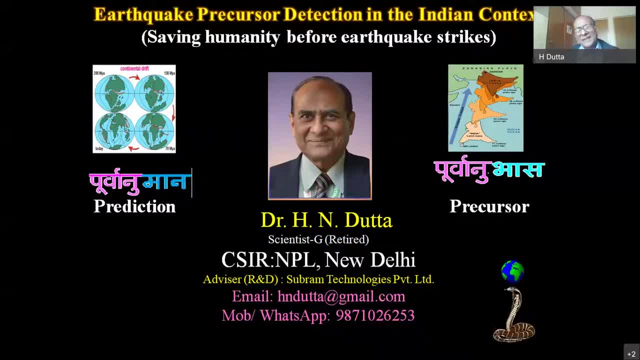 But one day what happened, and that's the story I'm going to narrate- that I detected the precursor of an earthquake and led India to have what is called an international patent from the highest intellectual authority in the world, the World WIPO- World Intellectual Property Organization. 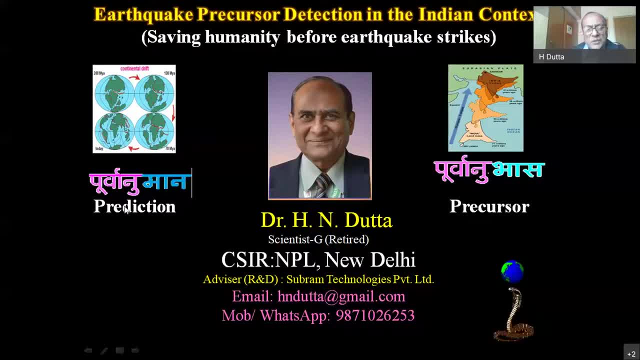 Just now Professor Rao said: well, prediction is impossible. Prediction is impossible because there is no data. See our whole knowledge about earthquakes. the data is available only, say, for the last 100 years And in 100 years at one particular point, to find the probability. 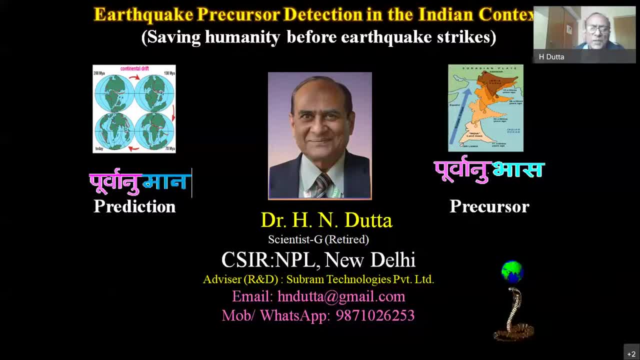 of occurrence of an earthquake to the level that will be acceptable to the masses is impossible. But then there is a hope We can find the precursor Purvanubhas. I am having a feeling. see, many times you must have seen when you come out of your home or come out to your 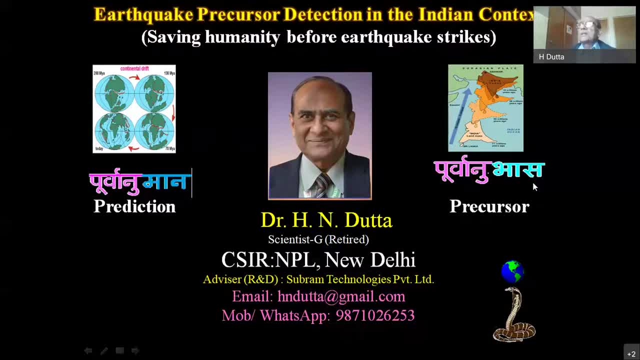 office, particularly because you know what is called thunderstorms are in the evening, you feel as if there is some changes happening in the, in the what is called the atmosphere, And the clouds are there and there is a thunder, And then you say: let us wait, Let us wait. 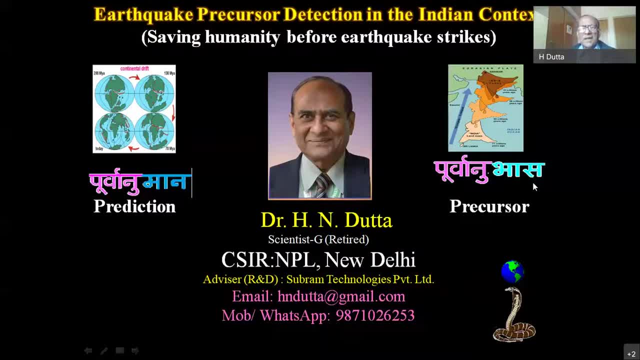 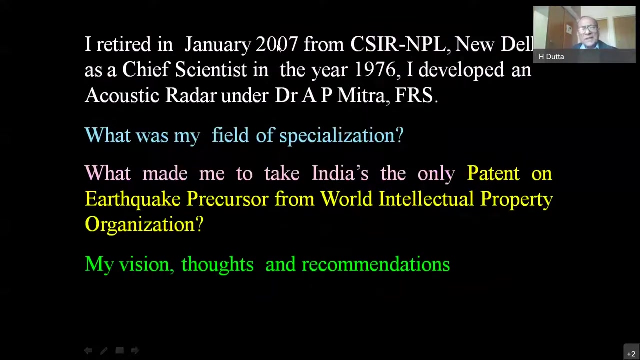 for some time, because it is going to rain Ninety-nine percent of the time it rains. You had not predicted, But you felt, yes, there is going to be a rain and there is a rain. It is as simple as that. That means what we require. we require so, but before going, let me say that I retired. 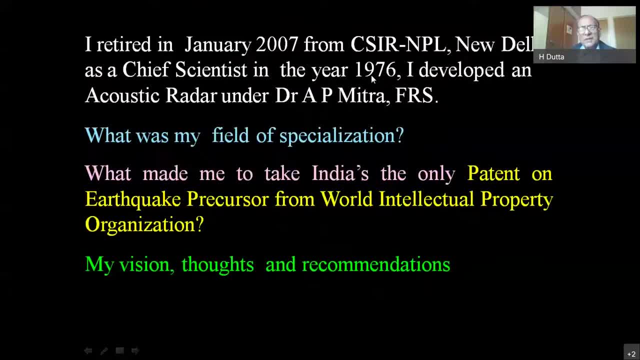 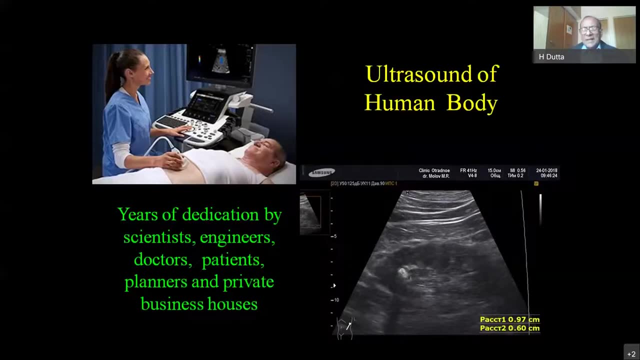 in 2007 and I joined NPL in 1976. So I will divide my talk in three units. What was my specialization before I took this patent? And now? what are my vision, thoughts and recommendations? We have all seen an ultrasound. In ultrasound, the doctor is or the, or the attendant, or 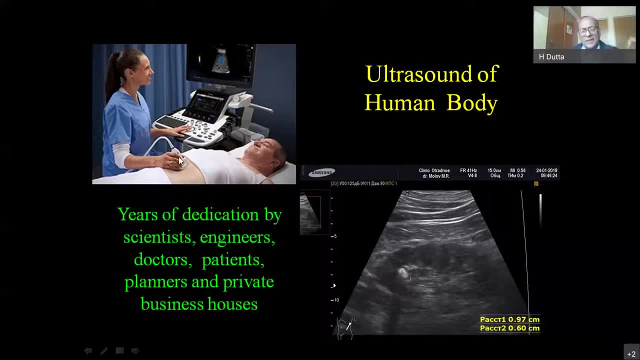 the or the doctor is, you know, moving this probe? Ultrasonic waves are transmitted inside the body, Yeah, And these waves get reflected or scattered with the surrounding space. The waves are being transmitted from the first wave to the second wave, And then the wave is moving. 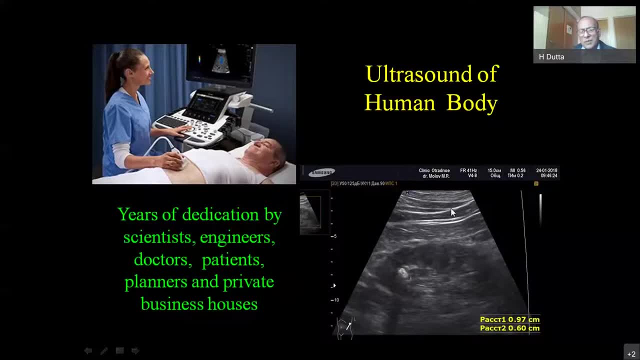 back and that energy is picked up and is plotted in the form of what is called a plot, for which the interpretation is given by a radiologist or ultrasonic specialist And one is able to say, yes, there is a kidney, there is a stone or whatever it is, and is able to even 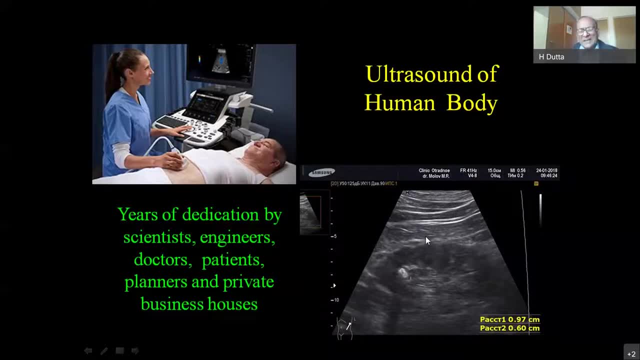 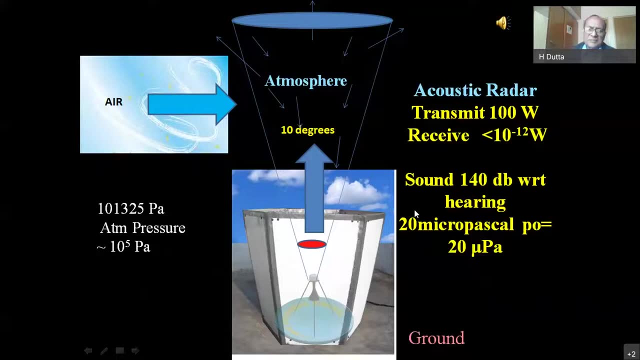 give detect the ailments Exactly in the similar fashion. so this is an ultrasound of the body. we have an acoustic radar. I transmit a very powerful pulse into the atmosphere, pip. So this pip is about 140 dB. I mean it is louder than your car horn but is only 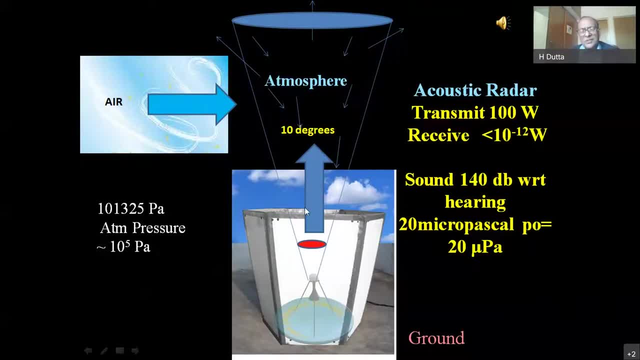 for 50 milliseconds, Okay. So when this sound goes into the atmosphere, my antenna is sitting on the ground all around. I build a shield so that I should not become a nuisance, Okay. And at the same time, I am able to receive very, very feeble signals, because 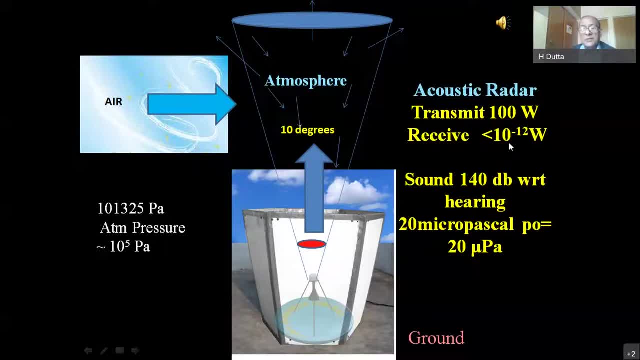 I transmit about 100 watts of power and receive only 10 to the power, minus 12 watt, minus 13,, 14 watt. So it's a very feeble signal. But then through signal processing we are able to get a photograph of air. So what I am doing, I am transmitting a pulse of 50. 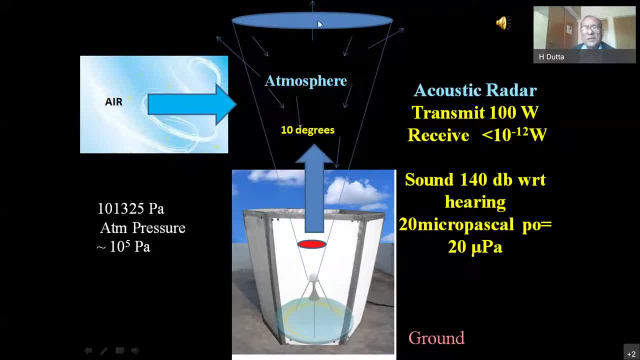 milliseconds. It goes into the atmosphere for three seconds because the sound velocity is about 340 meter per second. So it takes three seconds to go up and three seconds for the back scattered component to come to my antenna. There I pick up the signal, the scattered signal. 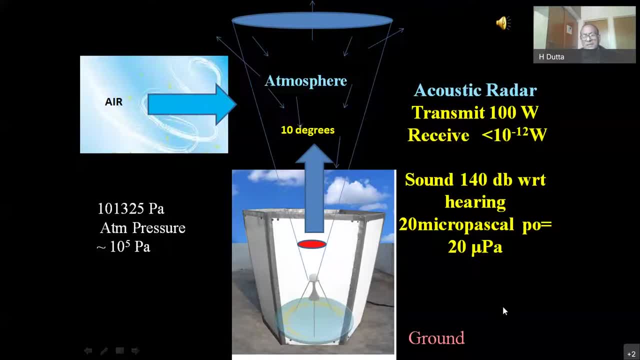 So after every six seconds I have to transmit a signal- pip- and then wait for and immediately start receiving the signal. This technology I developed in 1976. And let me tell you, like a mobile, you see that the first mobile and the mobile which you have received now I'm 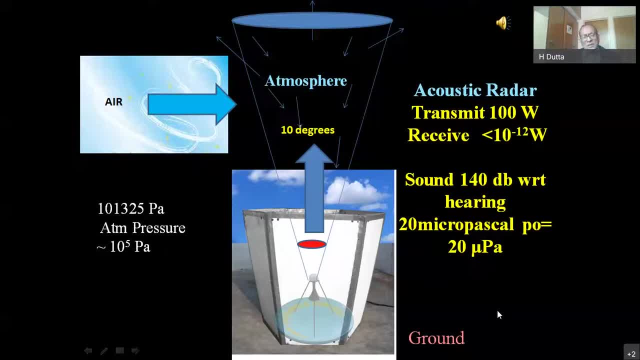 sure there must have been 200 different versions, because it is not easy to keep the technology alive. Either the hardware will change or the software will change. So fortunately I was in a position to keep the technology alive, So I am now able to transmit the signal. Okay, And then after three seconds I am able to transmit the signal. So I am now able to transmit the signal, Okay, And then after three seconds I am able to transmit the signal. So if I do a remote control, I can use the remote control and I can record the signal. 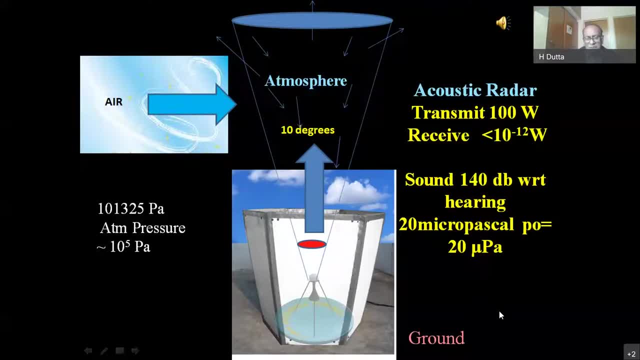 through the remote control and I can record the signal through the remote control. So I have been able to use this technology for more than 34 years And, of course, this is a very promising field, as you will see, And if somebody is interested to work, I 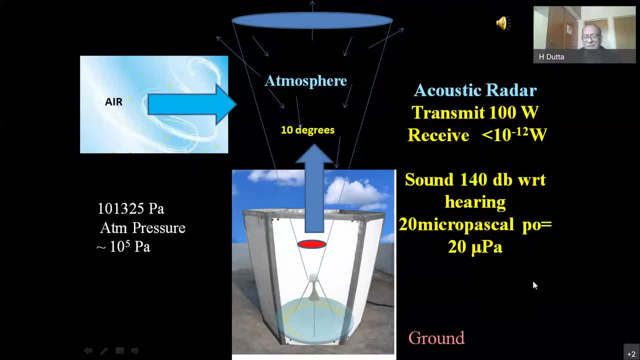 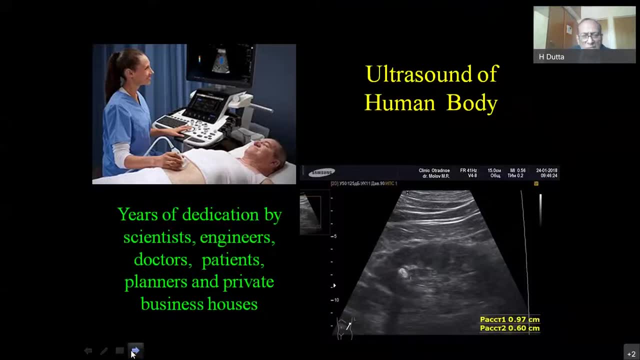 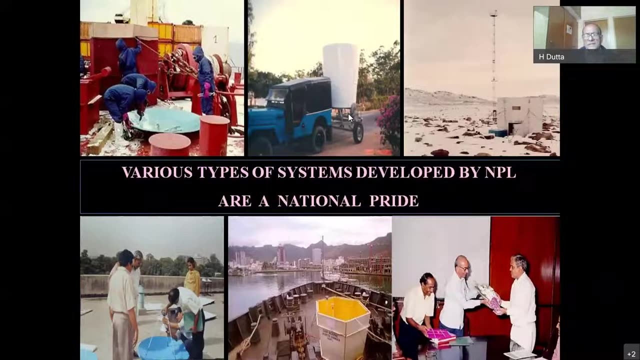 will be the happiest person to help. So these are various types of acoustic radars that I have developed, you see, because of the use, because it gives photographs of air, So naturally I had established it on the while I went to. I went twice to Antarctica. 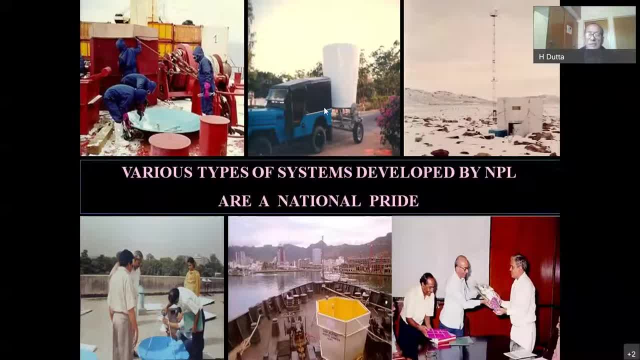 and by ship. so I had established on board the ship and this is what we had established in Antarctica and I transferred its technology. and I could transfer this technology to our then Honorable Prime Minister President of India, Sri Shankar Dayal Sharmaji's son. 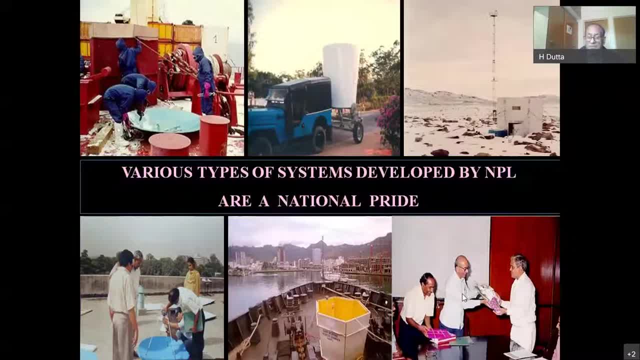 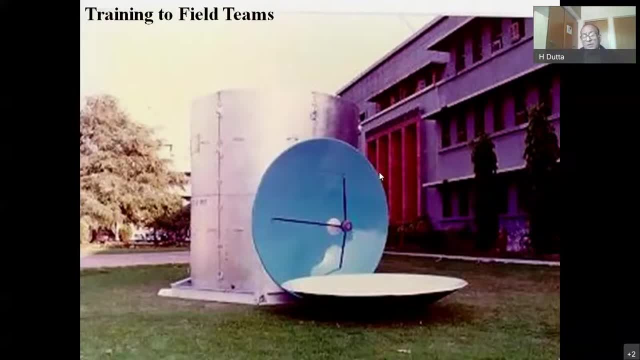 He had a company and we had transferred our technology to that company as well. Of course, you need to have two systems: one working in Antarctica and one working in the office- our own office- so that we are able to train the people. 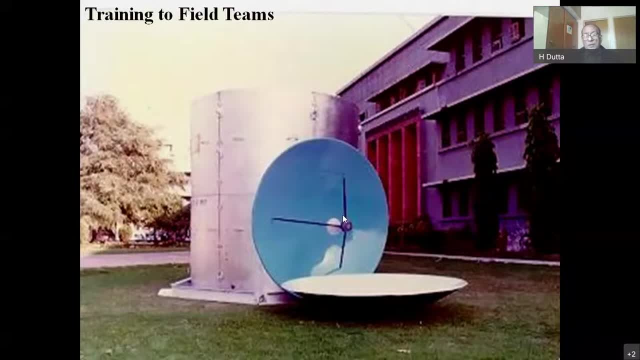 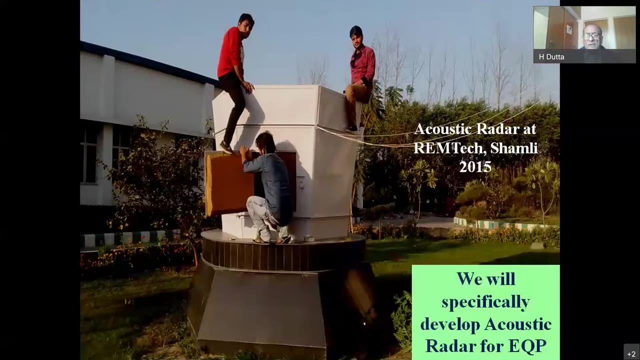 because every year I cannot go, I will have to send people. I was working as the convener for the whole CSR Antarctic program and I had deputed large number of people from various organizations and various universities or institutions, So this is the instrument we have placed. 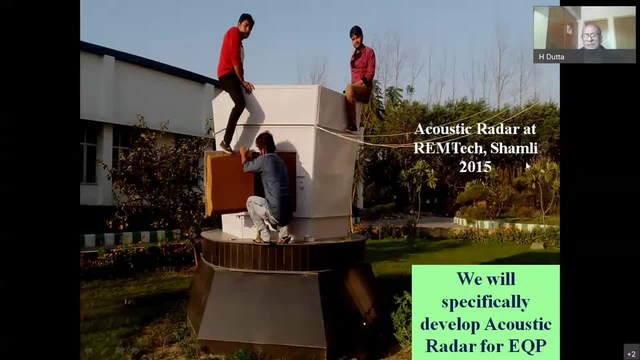 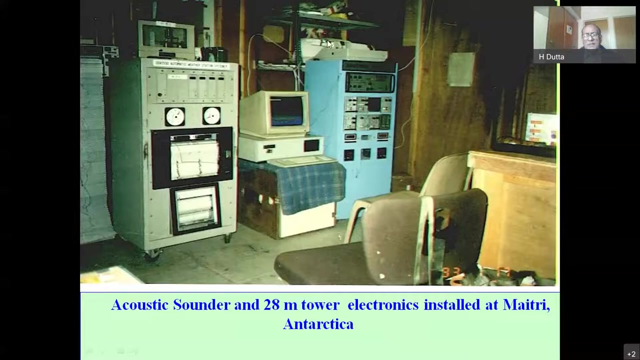 in engineering and management at the Institute Shambhala in 2015.. And these are for certain other specific purposes because engineering students were there, but we will have to develop a new radar for This equipment. this Just when we had placed it in Antarctica. it was a huge instrument because everything was in duplicate And you know, at that time our laptop was only a 286 or 486 based PC, which nowadays, thankfully that PCs are very, very, very fast. 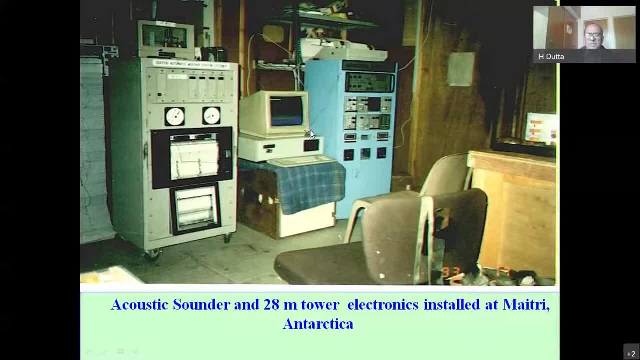 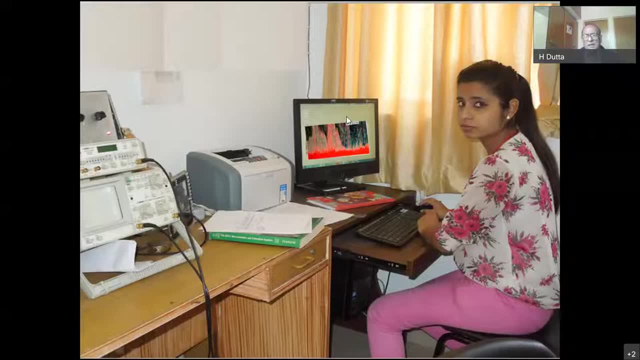 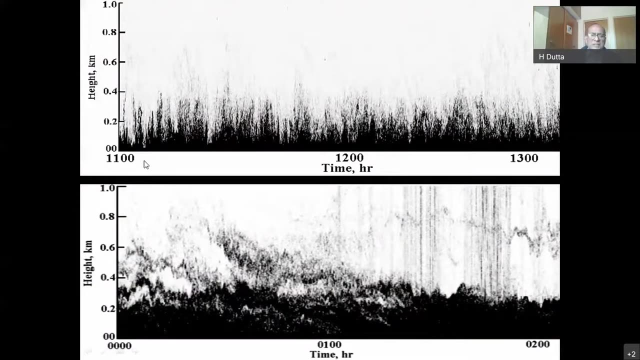 And signal processing has taken over. So the instrument itself is there is nothing called instrument. The electronics is only 5% and rest is all software. Now the question is this: what do we see When I say that? okay, it gives me a photograph of air. this upper one is the photograph of air during the daytime. 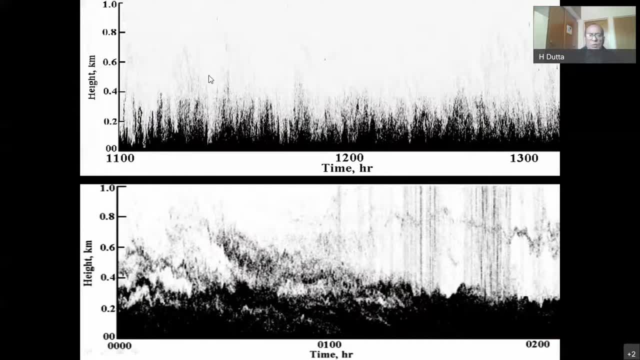 You can see the hot air parcel is going up and the cold air mass divided, The white portion is coming down. So here we transmit a pulse. you know, 6 seconds it takes to go up and come down. Then in the next line, third line, fourth line, fifth line. So over a period of about 5 minutes I'm able to know what exactly is happening into the atmosphere. 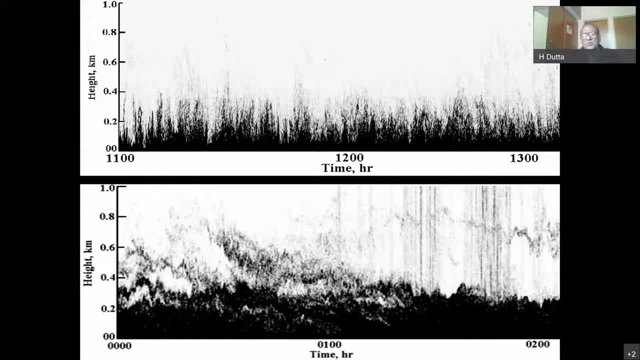 So this is a photograph of atmosphere, and we have utilized these photographs because I installed these radars for about 30 places in India For environmental monitoring and for the clearance of the what is called the EIA- environmental impact assessment clearance- for installing a particular industry or factory, or something like that. 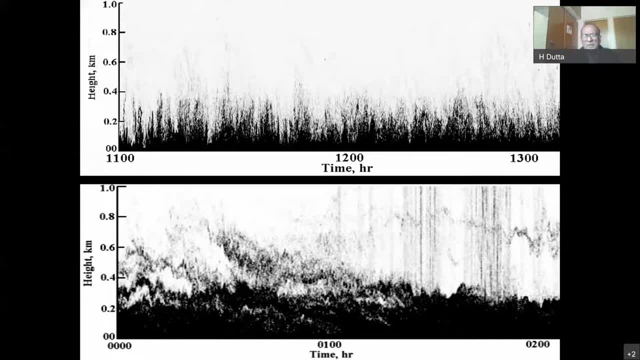 So these were part of what is called Ministry of Environment, where the clearances were being given In the nighttime. you see, the atmosphere is like sleeping. You have the stable atmosphere because here the temperature on the surface is much higher Compared to the temperature above at an altitude, So the thermal energy is forcing the air to move up. 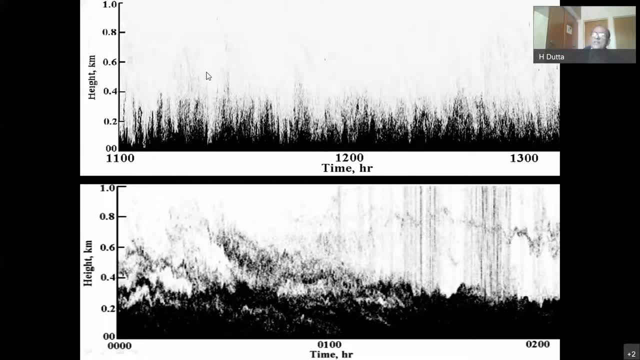 The question is this: what do we see? After all, when we look at each other, we see only the reflectivity from the surface, from the face, And on the basis of that, our mind is able to reconstruct and able to see. yes, he's a person, she's a girl or a boy, or a clock, or something like that. 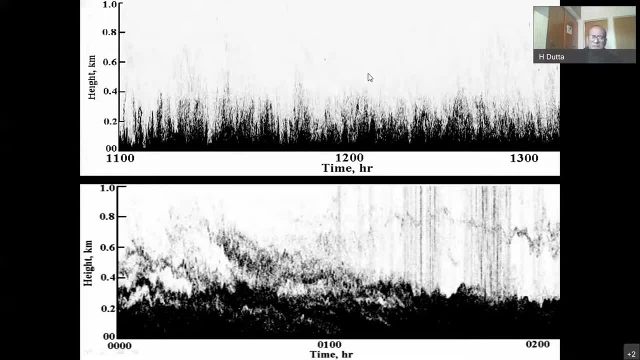 Or a laptop, because this is what is called the pattern classification. So, but once the atmosphere is stable, it is not stable in the sense there are so many wave motions are there, like a stable, what is called ocean. If you throw on a pond, if you throw a rock or a stone, you can see the repulse. 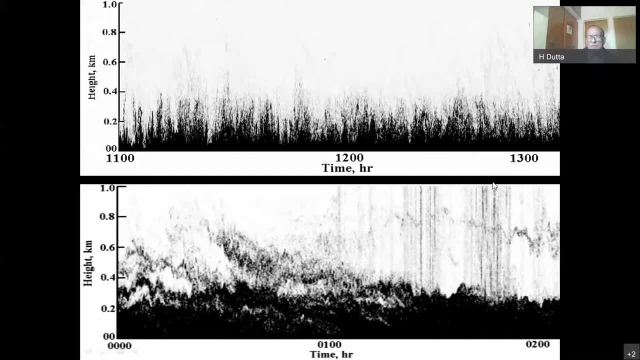 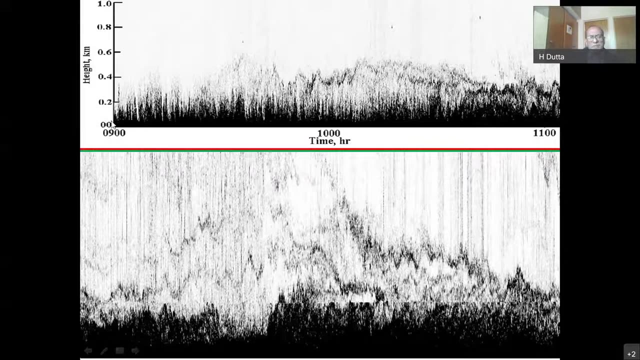 But during daytime, because the churning is taking place, you cannot see any movement of a wave motion In the in the lower atmosphere. Yeah, this is again the, the, the layer is sitting on the top of and, since we are monitoring it on continuous basis, 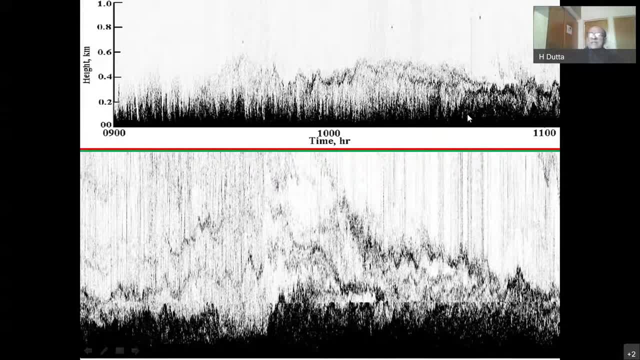 Naturally, it is like a dog. you have trained a dog to identify your own, what is called family members, and is standing on your gate. as and when it sees a stranger, it starts barking. So not that you have. you have predicted the, the, the, the coming off a stranger at home. 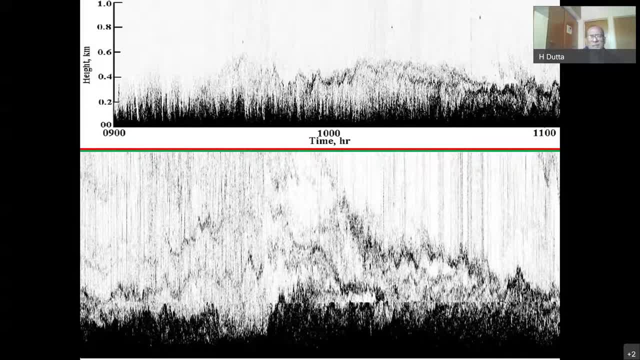 But since you have a watchdog watching the uh the gate on 24 hour basis, so anything new will be recorded by this particular technology, So it is the fastest, cheapest, the most economical instrument all over the world. The most economical instrument all over the world. 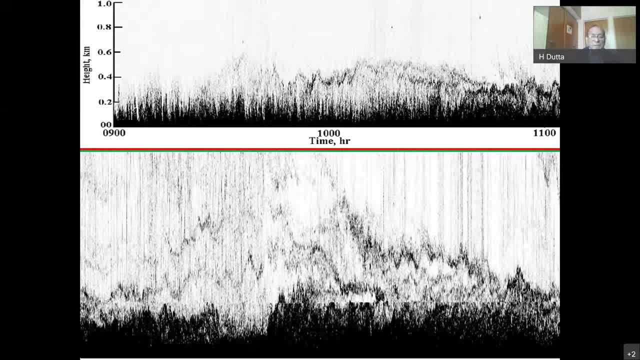 For monitoring the lower atmosphere. Fortunately, the lower atmosphere is sitting right on the skin of the earth, On this surface. that means if there is something in the art Which happens, it must get Amplified or transferred to the air. This is what we had expected, So you can see even the air bubbles. You can see thunderstorms. 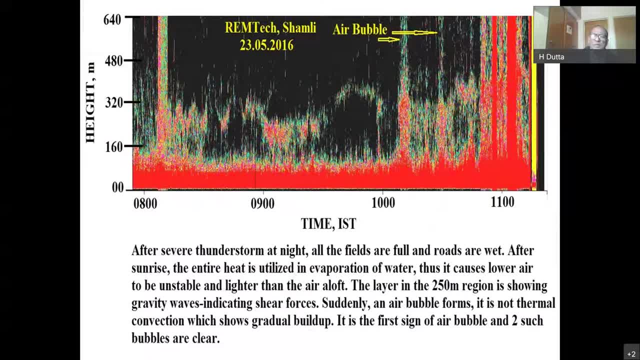 So you can see even the air bubbles. You can see thunderstorms. You can see even the air bubbles. You can see thunderstorms, anything, uh, what is called land, the sea breeze? at what altitude? Uh, this is what is happening. How many gradients are there And all those things. It's a, it's a very simple technology, but then, uh, you need to have the interpretation of the data that you recall. 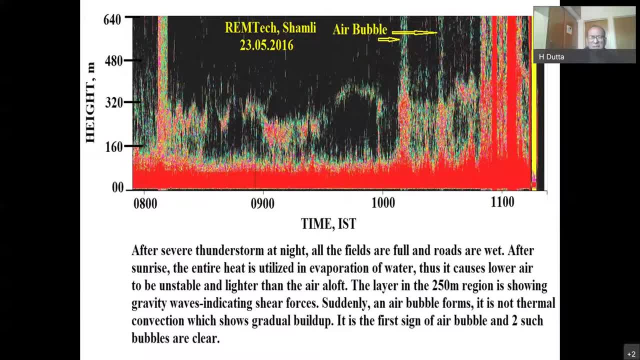 But then, uh, you need to have the interpretation of the data that you recall. So I'm. since I was working with the electronics, I developed the whole system In 7776, and I was invited by to deliver this lecture. 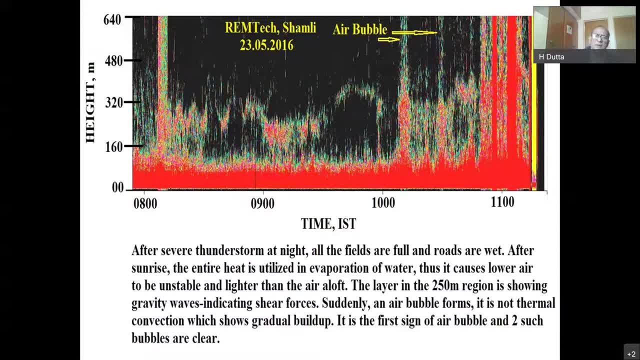 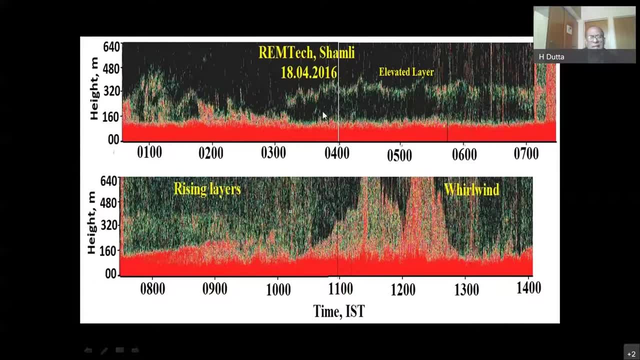 By the Department of engineering and since then I never looked back. Okay, the most happiest person, because we had established: you can see the wind, Oh my goodness. Anything that you can imagine will be recorded, but it should not be less than 5 minutes, because I cannot just on the basis of single line Say yes, This is what is happening. 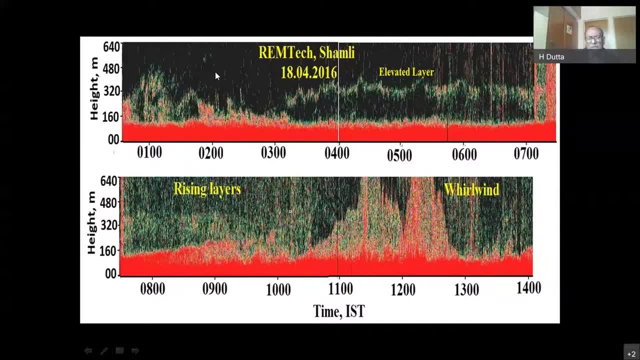 You have to wait for and for a phenomenon to really Uh be apparently recorded on the, on the what is Uh. on the on the what is called the, You can see the gravity waves, the motions in the atmosphere. 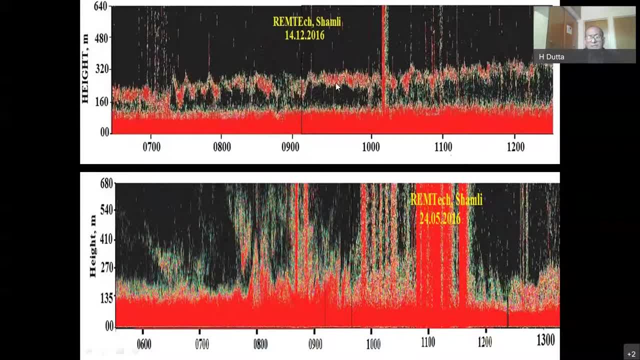 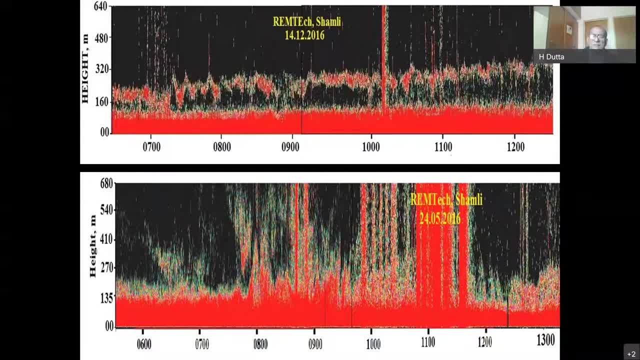 Uh, all around in the form of ripples and uh, the. the particles move vertically up and down And the energy flows in the, In the, in the horizontal direction. so these are. I had that what is called uh. you know the experience. 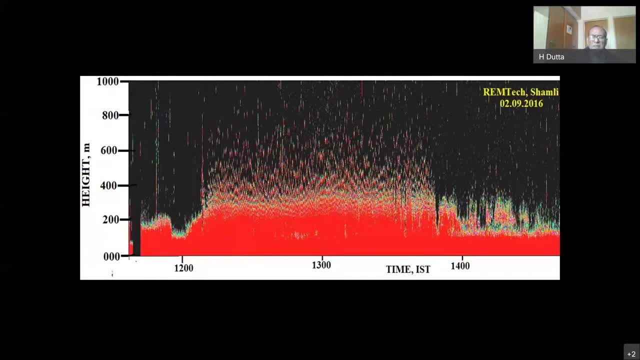 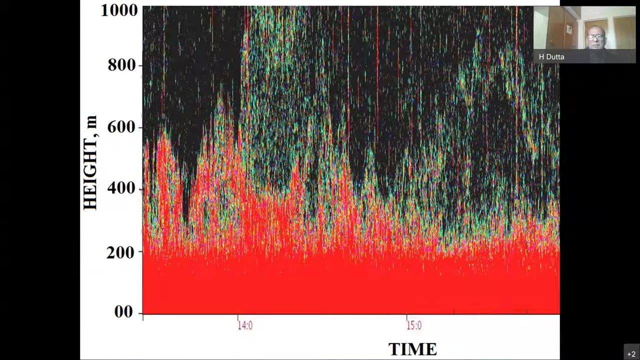 Of developing and putting the things in the field. My goodness, you can see the what is called the impact of uh- moisture content into the atmosphere. pressure differences into the atmosphere. What is that going to happen? How the churning is taking place. what is happening to air because of various processes. 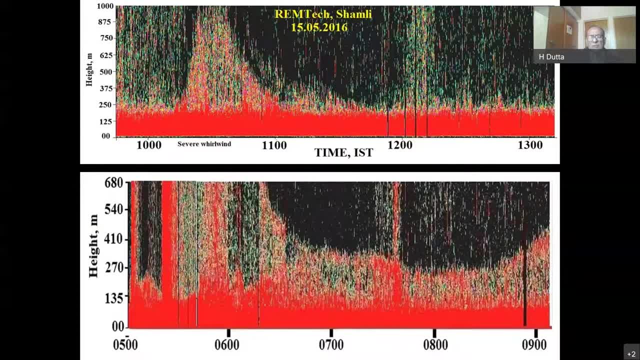 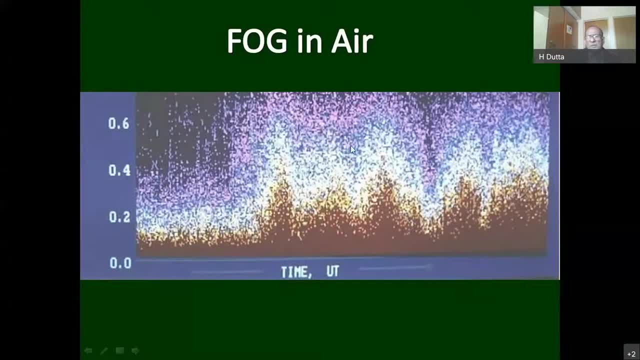 And that happened into the air. So with this like fog in here, I was invited by by so many. you know, for fog monitoring over northern India is very important that sitting on the ground I know that fog is about 800 meter thick. 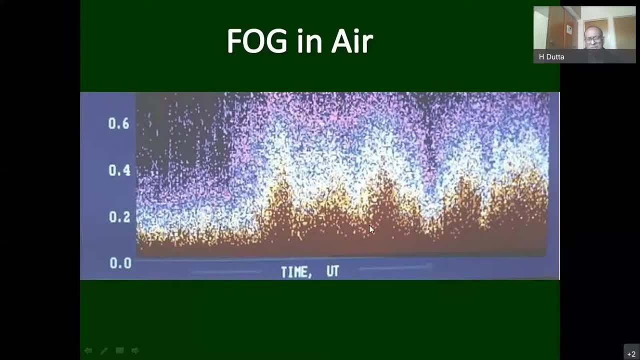 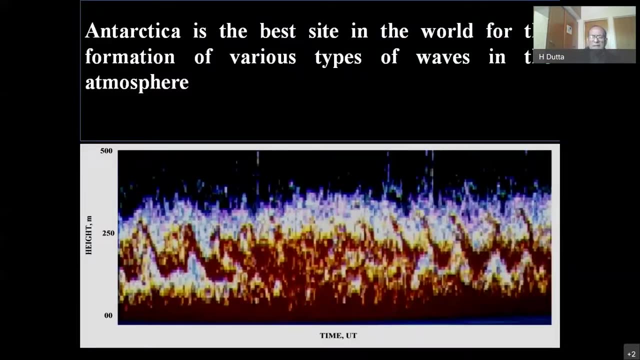 And it has so many gradients in it. Okay, So you know that, at what time the fog is going to dissipate, how the fog is forming, all those processes. And when I established myself in Antarctica, I had 2 experiences: 1.. 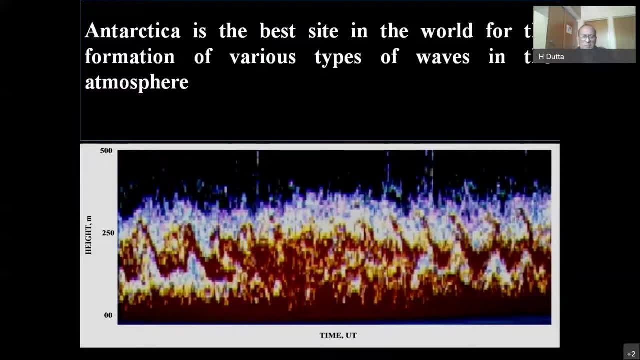 The experience 1, because Antarctic is so cold, It is the best place to study gravity waves. It is the best place to study kids with different kinds of emotions, Because the atmosphere there is more stable And I also experienced um Several, what is called cyclones. 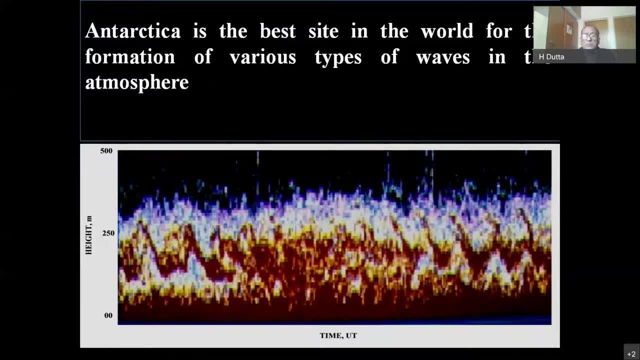 My goodness, sitting in the ship when your ship is caught in a cycle on the the way. uh, you know the turbulent waves. Uh, you make an impact. uh, you hold your ears and pledge that next time I will not come. 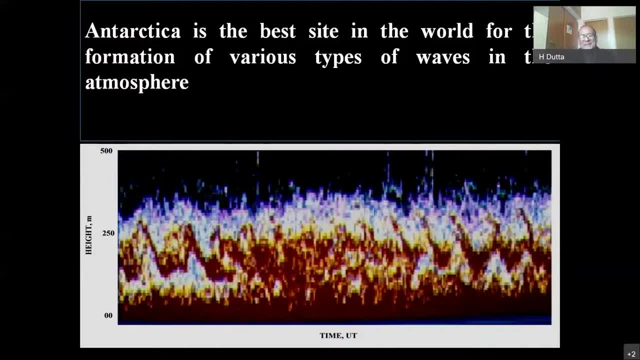 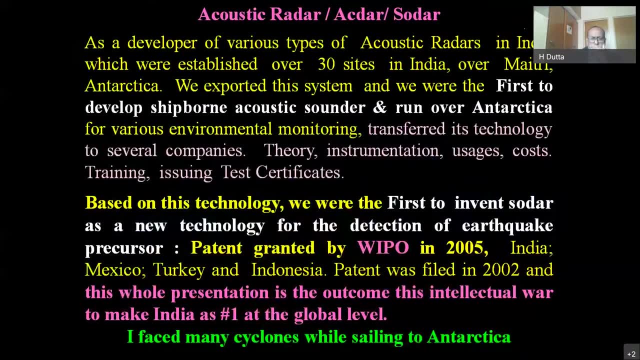 But then when you go reach in Antarctica, then, uh, you forget that pain because ultimately, pleasure and pain, uh, both are connected with each other. So, as a developer of acoustic radar over 30 sites in India and Antarctica and the person who had transferred its technology, 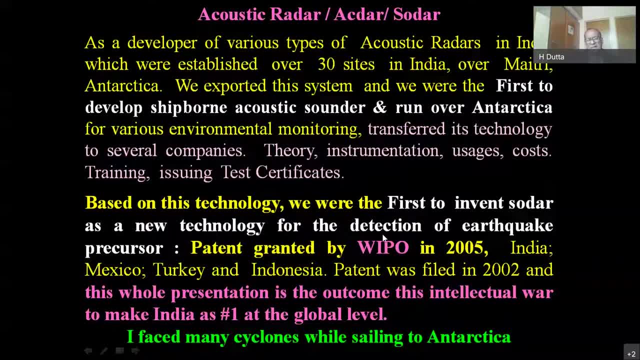 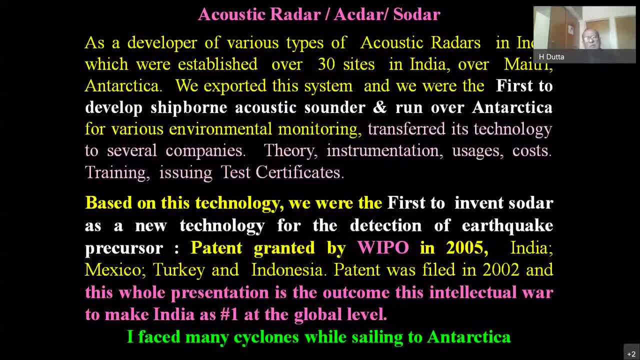 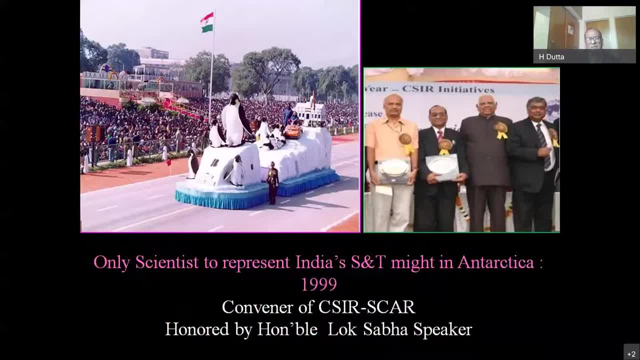 A developer and electronics engineer and I had absolutely nothing to do with, Uh, what is called uh, uh, uh with the system, or In the year 1999, I was In the year 1999,. I was. 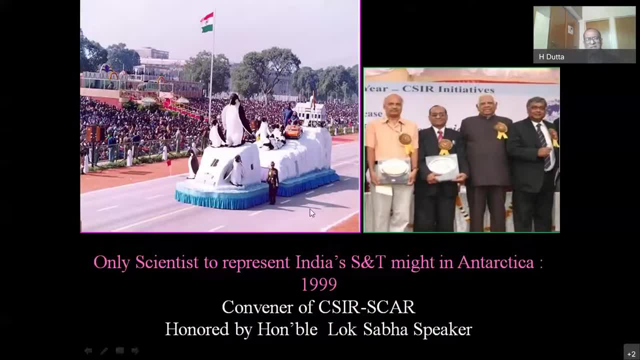 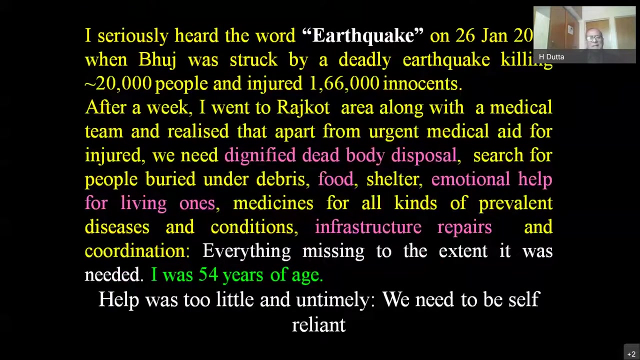 In the year 1999, I was chosen to represent India's might, science and technological might in Antarctica, And perhaps I'm the only 1 to have this kind of attainment, or credential whatever you may call. Then I was on a read, The then looks of our speaker, for my lifetime contributions in the field of 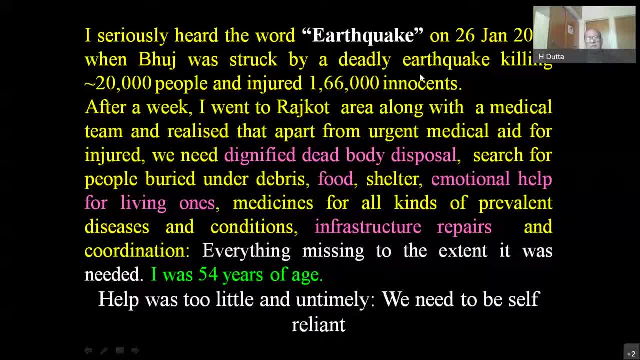 of Bhuj when Bhuj was struck by a deadly earthquake. After about a week, I went to Rajkot along with a team and realized that, apart from urgent medical aid and injured people, we need dignified disposal, a dead body disposal, search for people buried under debris. We need food. 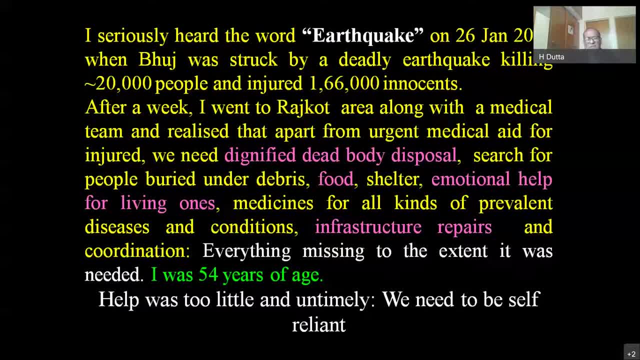 we need shelter, we need emotional help for living ones. living ones, medicines of all kinds of prevalent diseases and conditions Everybody was taking, you know, medicines for injury or and all that. Nobody thought what happens to those who are pregnant. Nobody thought what happens to. 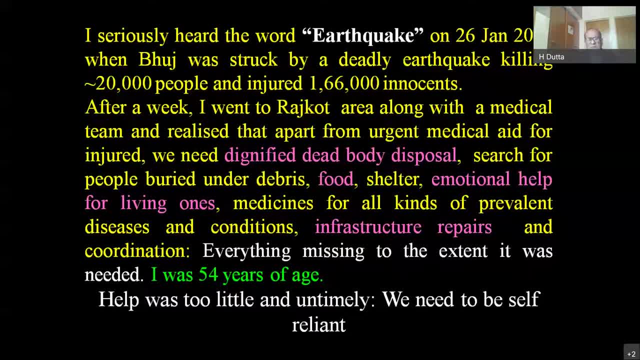 those who are having heart attack or something like that. So infrastructure repair very important, As Professor Rao said. well, landslides or the roads are blocked, then what do you do? And coordination, Everything missing to the extent it was needed. I was 54 years of. 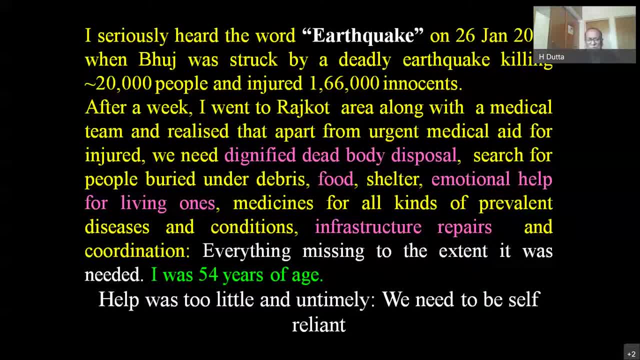 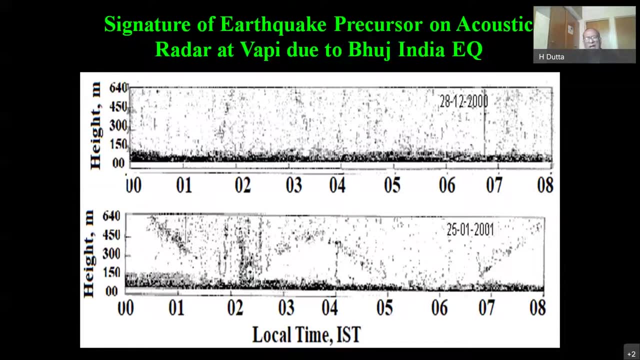 age and I knew that help was too little and untimely And therefore we need to be self-reliant. When I came back in the year 2002, we were having a system- acoustic radar- working at Wapi- It is about 300 kilometers from Bhuj- And I found that there is a signature. there is a large 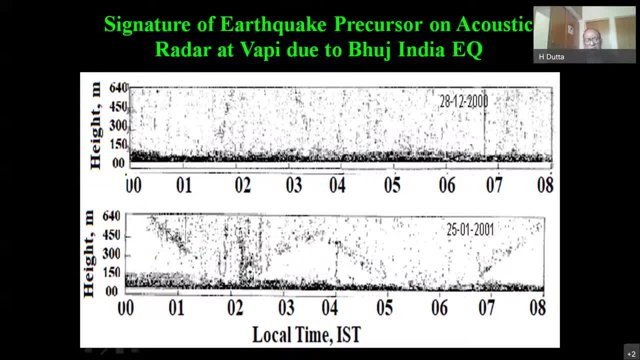 amplitude And the longest period of wave in the atmosphere, And that was on 25th of January. The gentleman you know: he had switched off the system at 8 o'clock in the morning because next day was a holiday And when we received this, I saw this data. I thought that this could be a precursor. 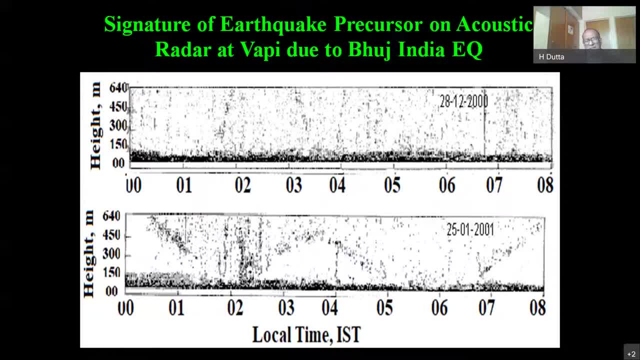 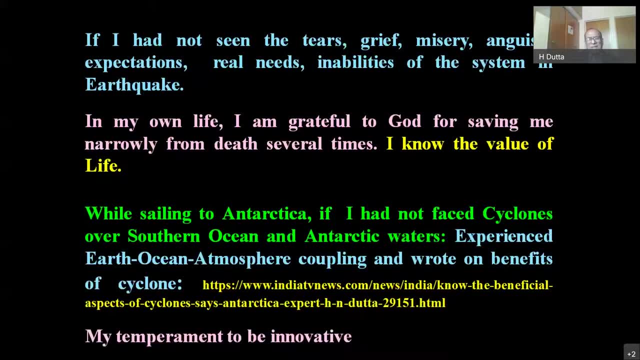 So if this is a precursor, then what do we do? Then I, I studied, started studying. Okay, I decided that, okay, let me send this paper to either Nature Or take a patent, international patent, Because this means this technology can be used for detecting earthquake. precursor. because nobody had in the literature ever claimed. 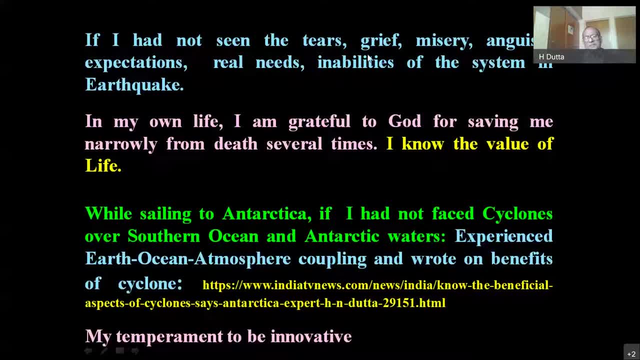 So, dear participants, if I had not seen the tears, the grief, the misery, the anguish, the expectations of the people you know, during earthquake and in my own life, i am having a very strange coincidence. i am grateful to god for saving me narrowly from death several times. 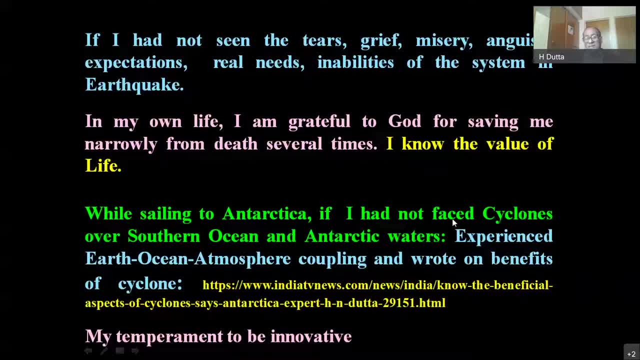 so i knew the value of life and while sailing to antarctica i had seen, oh my goodness, i have faced cyclones and worked on what is called earth, ocean, atmospheric coupling, and and then also i wrote a long these things on the, on the benefits of cyclone. you know, whenever there is a cyclone, 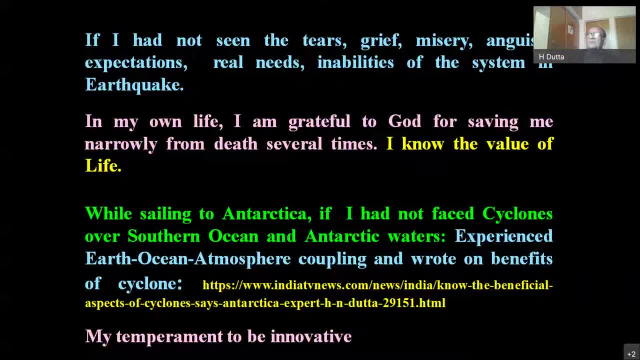 everybody will say: killer, cyclone, killer cyclone. other cyclones are. it is the cyclone which generated humans. it is the cyclone which is so beneficial to various other components of nature and therefore let us stop calling cyclone as a killer. a cyclone, you know, and my temperament to 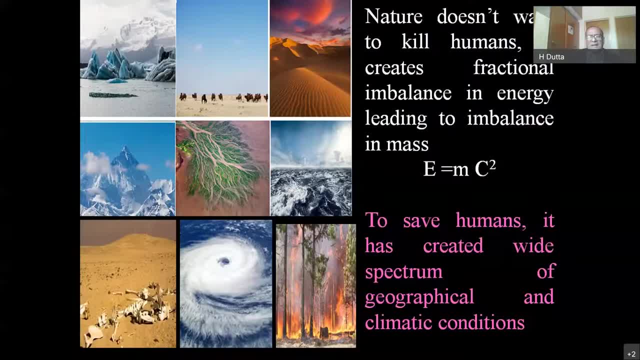 be innovative with all these things. i looked at the nature once again see nature has created heterogeneity so that if there is any catastrophe in one, the people are going to be saved in other, in other regions. nature doesn't want to kill humans, but there is a small energy imbalance- is equal to mc squared- and that we have to face because 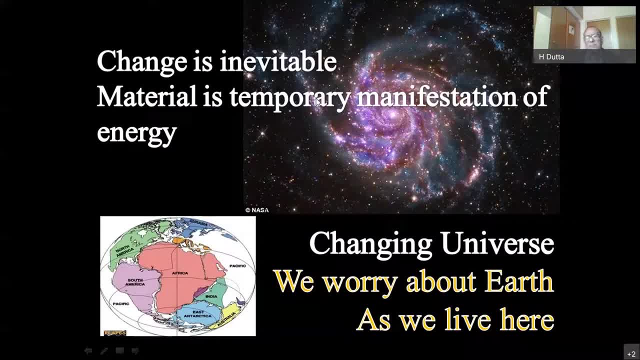 the whole world is. the change is inevitable. material is a temporary manifestation of an energy. the whole world, the whole universe is changing. we worry about earth as we live here. since we live here, that doesn't mean the change will not be there. the moment change stops, that will be the end of earth. 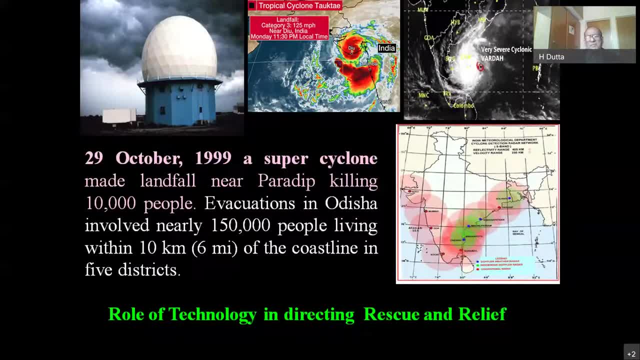 50 years back, everybody was interested to predict a cyclone. but now prediction is is secondary because we know, we have developed the technologies. we have the what is called cyclone cyclones being mapped from the, from the satellites, as well as we have the radars, the satellite is 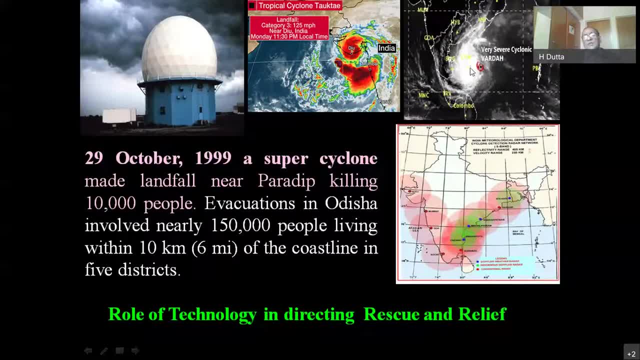 made. how do we say we are not measuring cyclone? a cyclone has a property that it shows in the form of clouds. so, in fact, we are measuring clouds, we are, we are seeing the uh, infrared, through infrared or optical images, and we infer then, yes, there is going to be a cyclone. now, of course so. 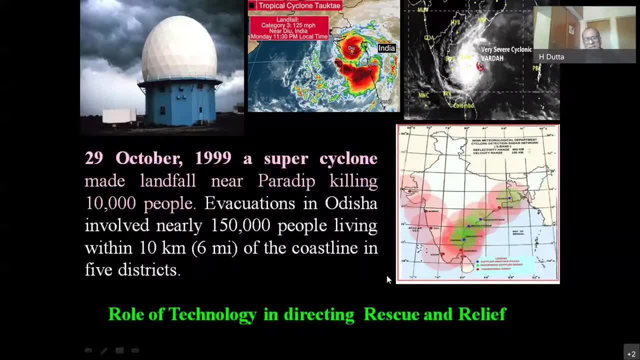 in 1999 about 10 000 people had died and now, of course, thanks to ndrf and the and idm and all those organizations, nobody is dying. i mean, if 10 people are dying, they will die in any case. so that is the kind of what is called effort which will be required. 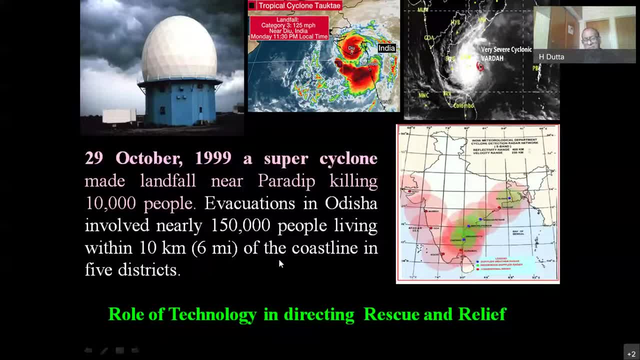 in earthquake also- and i'm i'm sure so, the role of technology in darkness, directing rescue and relief. It holds the key. Unless we develop technology, unless we develop our own instruments, borrowing instruments, buying instruments will not lead us anywhere, because we don't calibrate our system. Once we have purchased, we do not have the facility to calibrate. 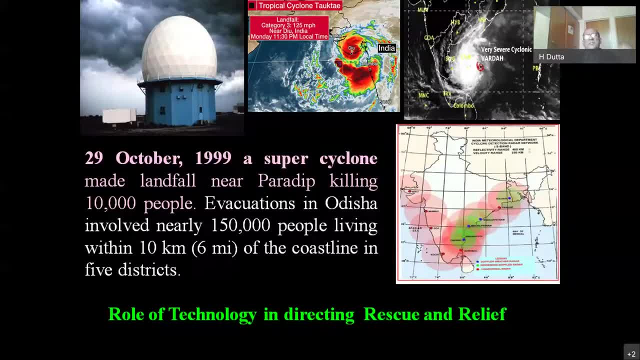 Sitting in NPL, I was issuing test and calibration certificates yearly for all the radars, because changes will take place. something is working in the field. Obviously, it is bound to. something is going to happen to the system. Well, dead bodies: How do we handle dead bodies? It's a billion dollar. 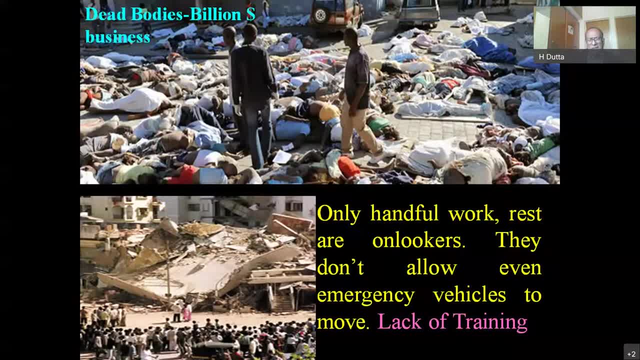 business for many countries And unfortunately, as Professor Rao in the morning said, well, are we involved? Only a handful of people will work and rest. We work as an onlooker And not only an onlooker. we work as an onlooker. We work as an onlooker And not only an onlooker. we work as an onlooker And not only an onlooker. we work as an onlooker And not only an onlooker. we work as an onlooker. We work as an onlooker. We don't allow even emergency vehicles to move. 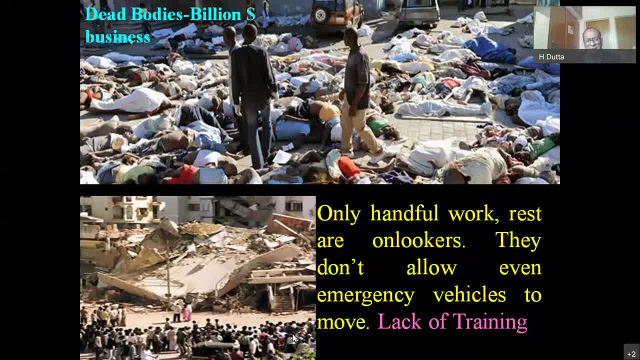 because I want to see, even if one person removes one kg of part of this thing, that training is not there. We feel as if it is the job of just 10 people who are working, who have come from various organizations and they are pouring their energy. No. 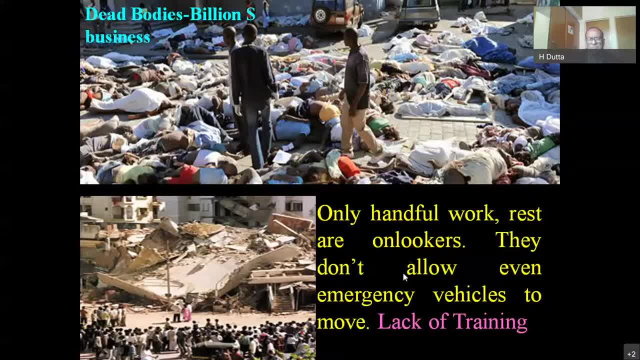 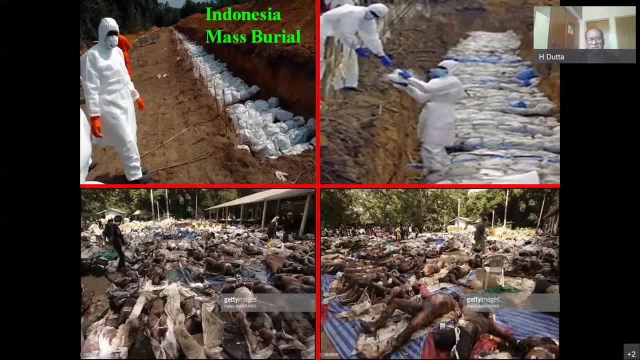 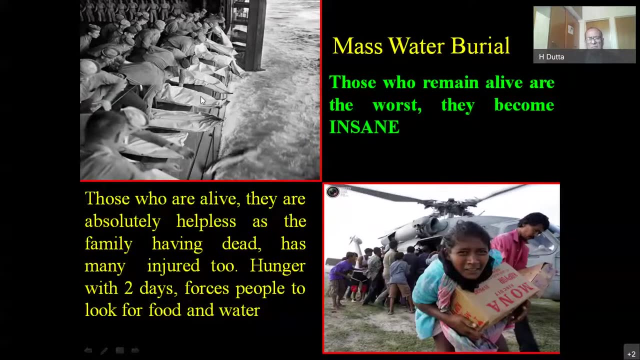 we never think that it is our job. So Maas-Barrion, this is Maas-Barrion. I mean at the national level and just after two days, this is very important- What is called the Maas-Barrion? because in the coastal region, if suppose there are five lakh or 10 lakh people are. 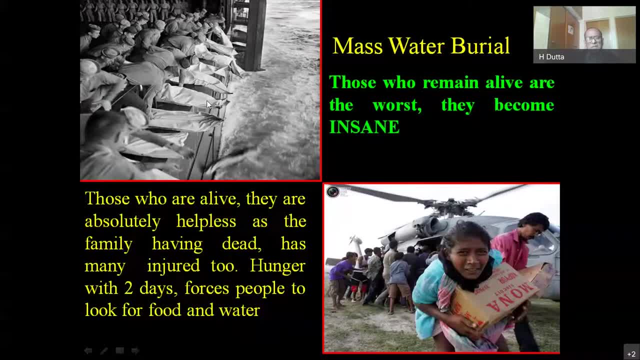 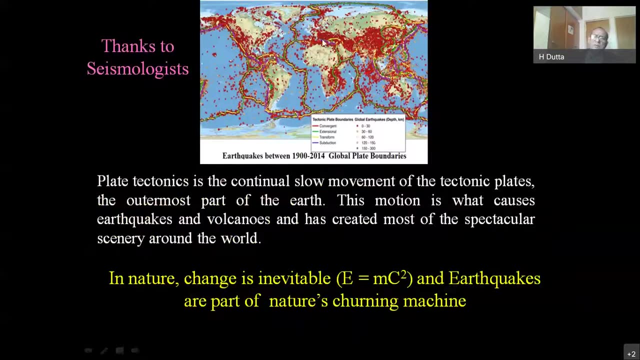 going to die in a fraction of a second, then what do you do? Are we prepared for that? So we have to change our mindset in the national interest. Thanks to sysmologies. So a person as an atmospheric scientist, when I look at this, I know that. okay, here is the probability for next. 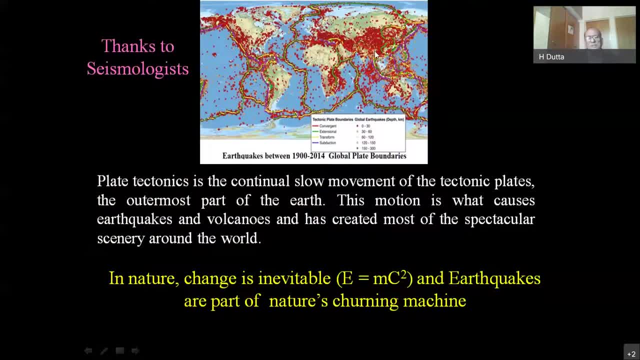 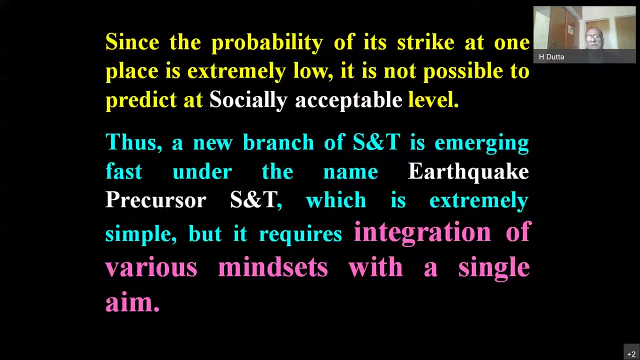 earthquake to come And unfortunately, or fortunately- the danger looms a lot as far as India is concerned. In nature, change is inevitable and earthquakes are part of nature's churning machine. So very important, because the probability of striking at a place is extremely low. 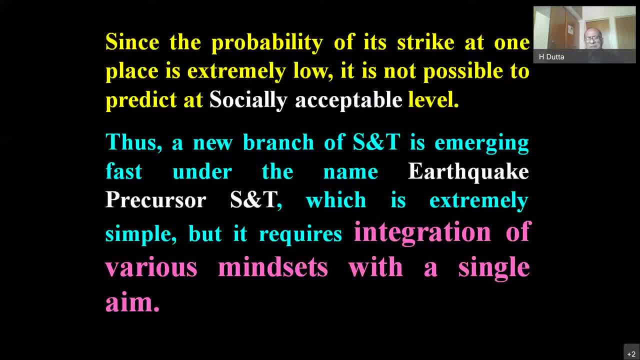 and it is not possible to predict at the socially acceptable level. Socially acceptable level means I can say: okay, please be away from your building, sit in your park with your bread and butter for just six hours. 10 hours for a day. I cannot say that. okay in October. 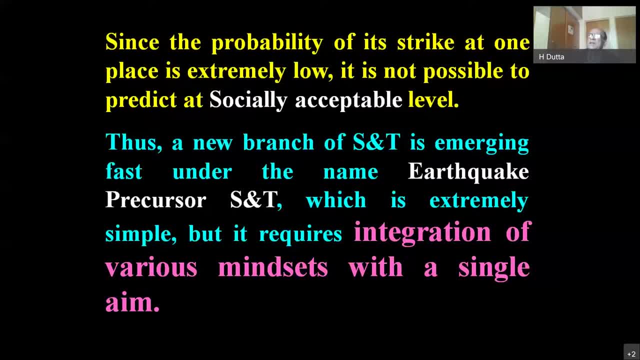 2023, there is going to be an earthquake in Delhi. Nobody is going to stop the work and people will, So that's socially acceptable. Okay, Therefore, earthquake precursor science and technology, which, of course, will require an integration of various mindsets with a single aim. 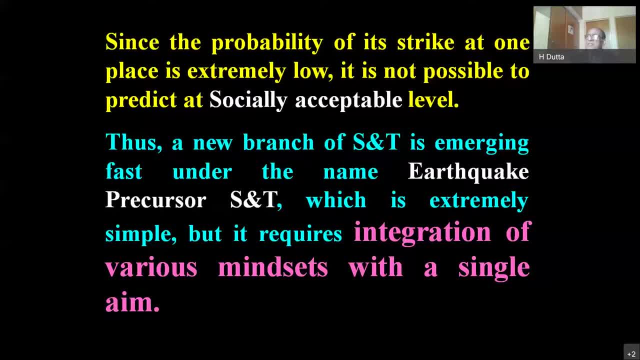 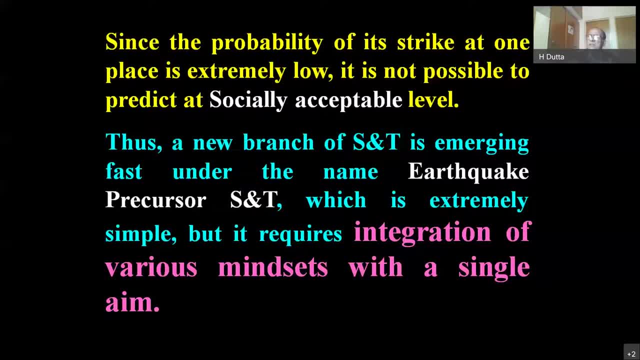 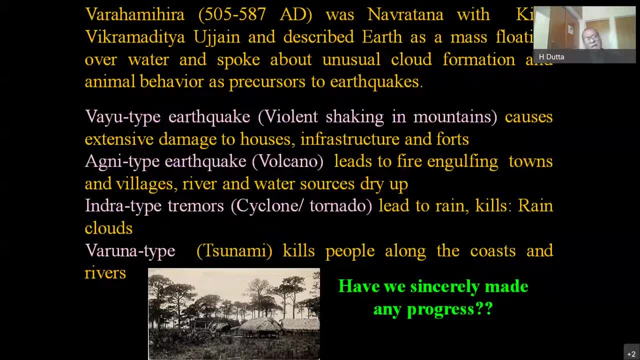 Let us coordinate with each other, let us pour our energy, and our focus is right now To have an entire comparison, to have everything put together and get the what is called the benefit for the society. If we look at our own, what is called civilization? Barham Mitra had: 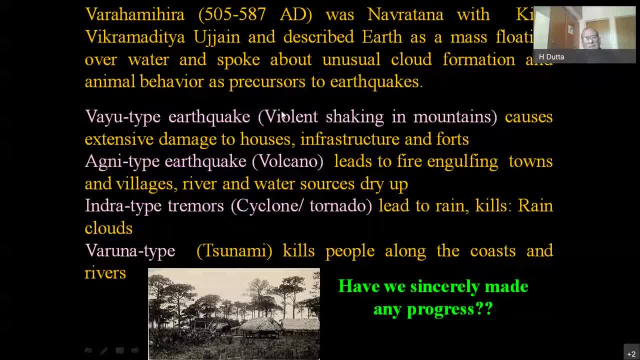 you know, in 505 AD he had very well documented that what kind of earthquakes exist in our India And you know, Vayu type earthquake, violent shaking in mountains, Okay, And then Adani type volcano resulting to this Indra type with cyclones and tornadoes, and Varna type tsunami. 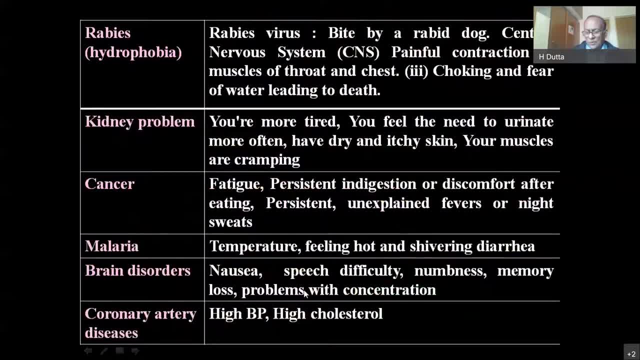 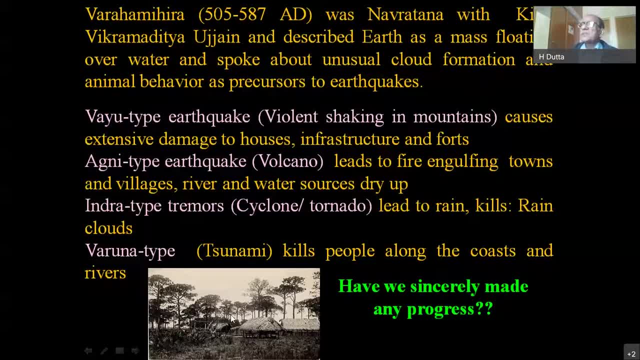 Now, what have we done since then? We have only given a new, new, new, what is called terminology. And although people were living in just huts, they were not concerned about the death because of falling hut. They were concerned because of the changing wide 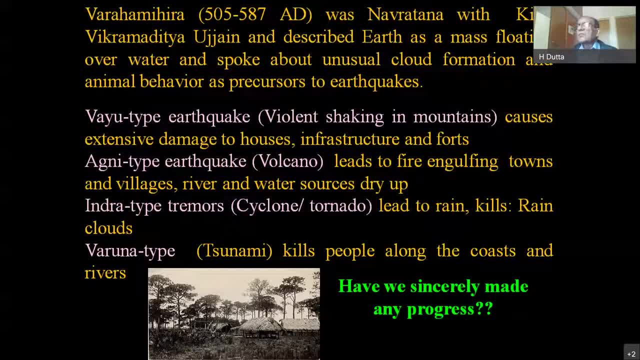 scale patterns, like the river is going to change, The mountains are going to fall to a level where they are going to create a catastrophe. So you question ourselves: have we made a sincerely any progress? We have given new terminology. we have developed few instruments. 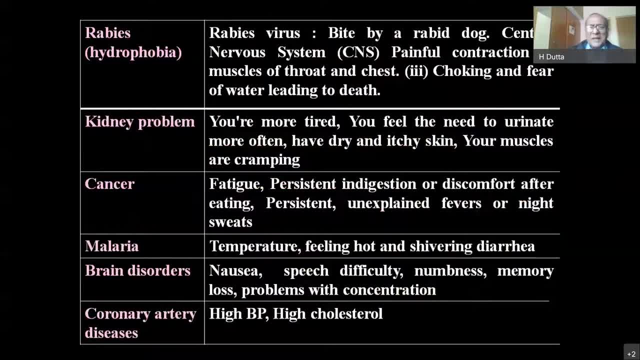 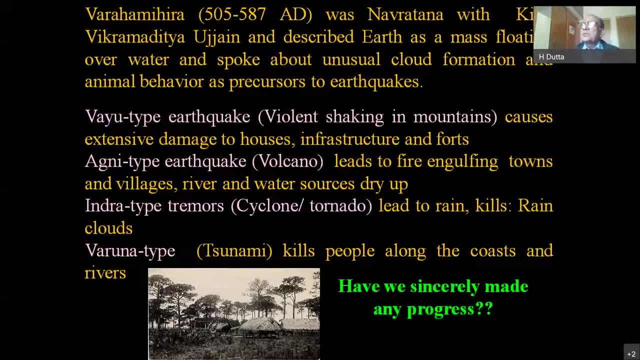 That's it. If you see medical science, the problem here is in many an earthquake. unless an earthquake comes, I will not be in a position to diagnose, Since it is coming once in every, say, 10 years. so I will have to quietly sit and wait for. 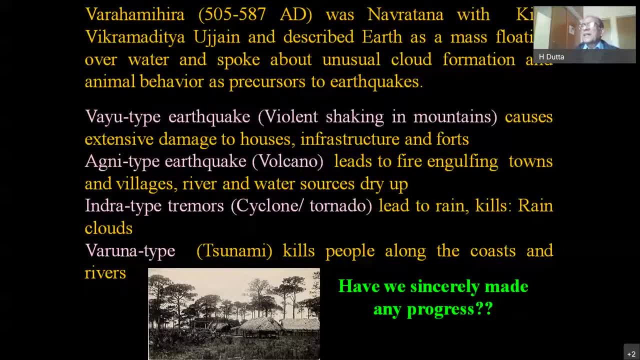 that Okay. And what happens? In 10 years of time, your boss will say: you are not working, you are not doing anything here. Leave this field Because they want. we do not have patience in our system. If somebody says I am working in earthquake precursor, you will have to. 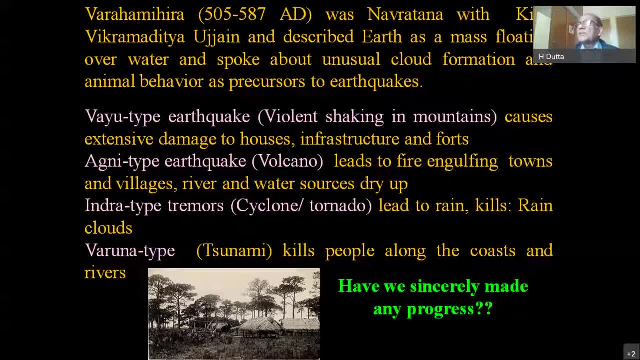 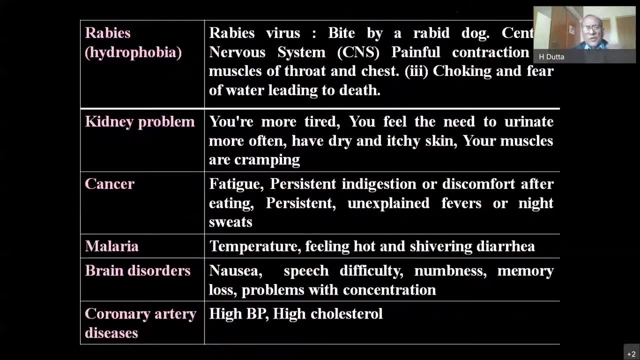 have patience. You will have to have what is called the faith. Yes, I am working sincerely, but I need an earthquake to make the progress. If we look at the medical science, because so many patients are there, the rabies doctor finds that okay. if you are choking, I mean. 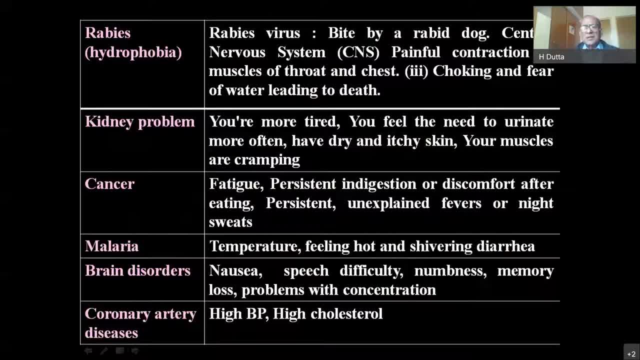 these are the symptoms. Okay, These are the symptoms. So, based on symptom, the doctor knows the problem In kidney. he is not checking the kidney first, He is just seeing that your muscles are tramping In: cancer, malaria, all these things we have. 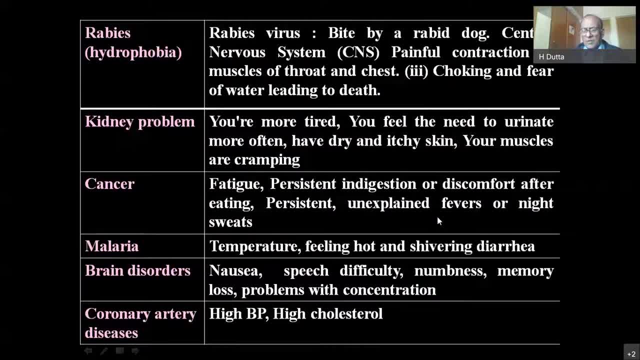 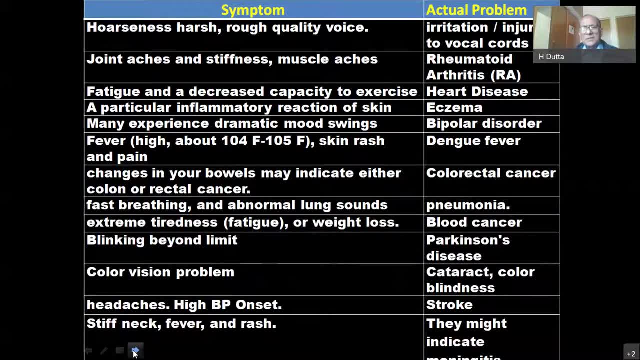 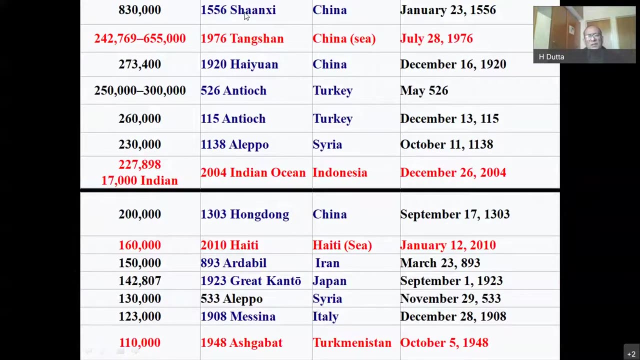 been in a position because there was a what is called sorry, because the patients were there. So, symptoms and the actual problem, Medical science is very nice. In the case of earthquake, 8,33,000.. 8,33,000 people died in China. When we see all these figures, we think that these figures 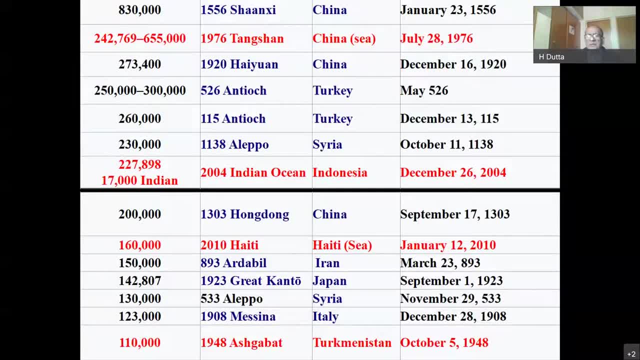 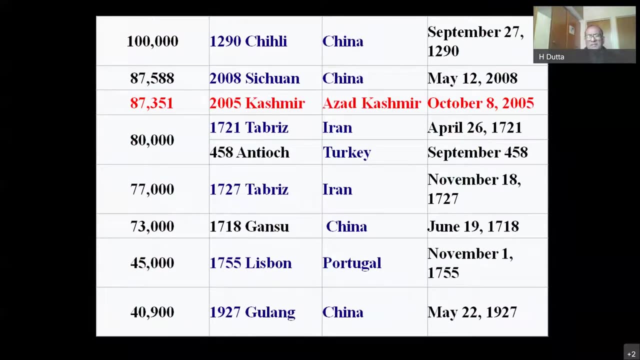 belong to some other nation. Ladies and gentlemen, these figures, any of these figures will work in, even will be seen in India in very, very close time, Because already these stresses have built to such an extent that I mean we will have to face 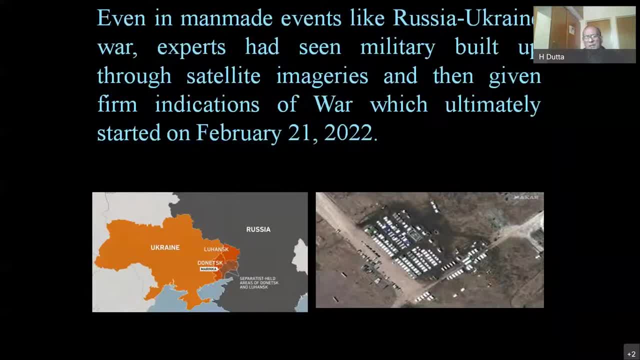 Now, even in man-made events like Russia-Ukraine war, we had a precursor, because from the satellite images people could see: yes, there is a buildup of army, There is a buildup of infrastructure going to be used for war, And then people had predicted: So this is, these are precursory. 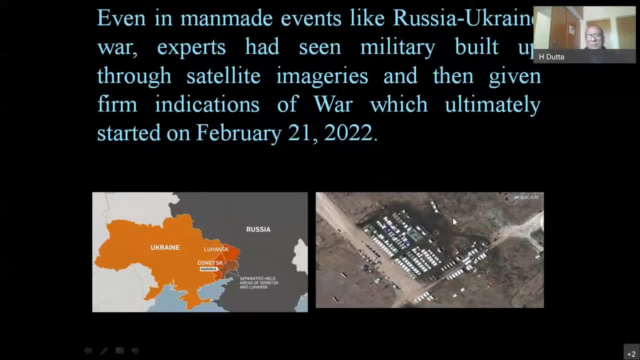 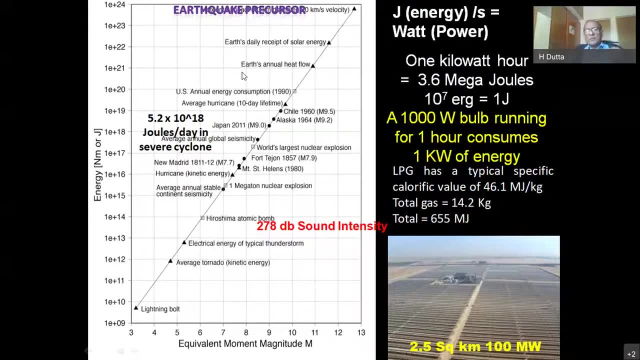 signatures. Okay, You don't have to predict a war, but precursor is seen. Now comes the question: how much is the energy and what is earthquake? Why do we have to worry about earth Earthquake? If you look at the energy in a very severe cyclone and earthquake, it is. 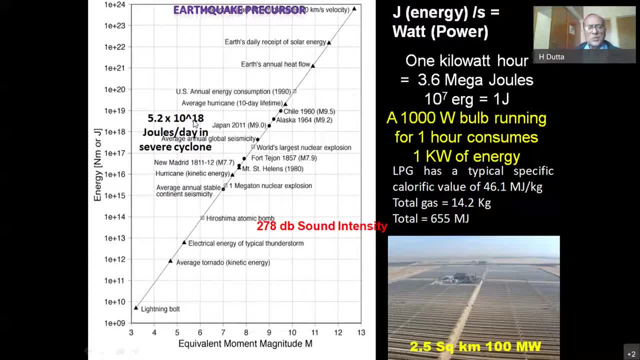 the same, exactly about 10 to the power, 18 joules of energy, And in earthquake in Japan that m is equal to 9, it was also the same. The issue is: in the case of cyclone, the decay takes place over 5,, 6 days, 10 days. 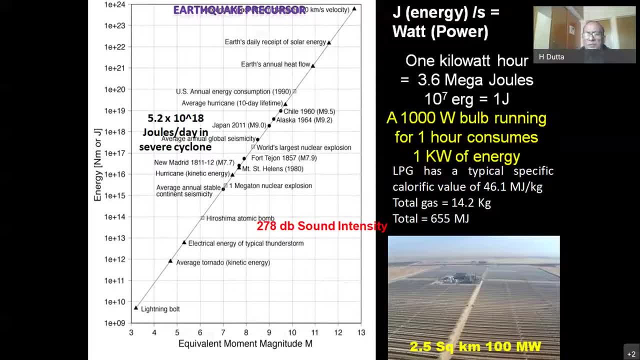 It builds up in about 5, 6 days and it decays in 5, 6 days. So the energy release per second is extremely useful, And that is why I say that cyclones are useful for the benefit of the humankind or the nature. But in the case of earthquake, the decay takes place in a 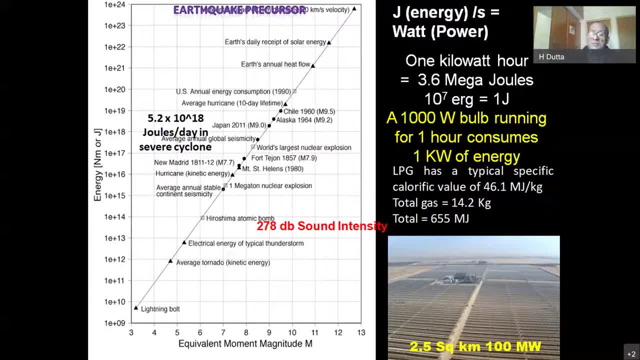 period of just a couple of minutes- 2 minutes, 3 minutes. So massive amount of energy getting up, Energy getting released per second is important. It is not the total amount of energy, The total heat that the energy consumption in US annual is 100 times more than the energy. 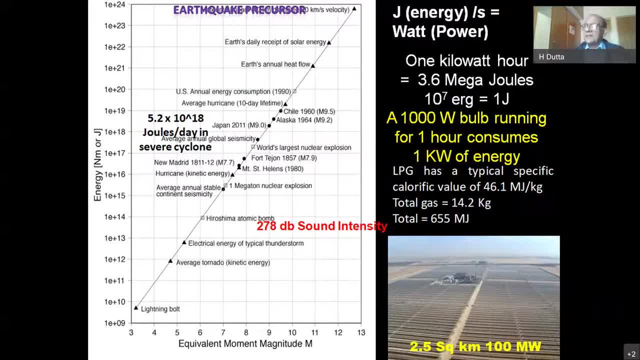 in an earthquake, But then that energy consumption is slowly being consumed. It is like a nuclear power plant or a nuclear bomb. Energy is same, but their energy is useful, and here the energy is destructive. It is the energy So in nature. since earthquake releases, the energy per second is the highest. 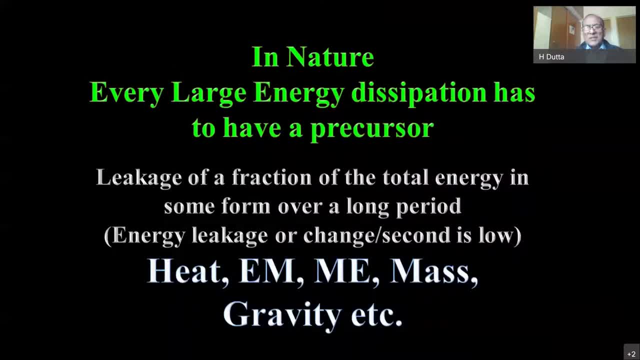 and therefore the destructions. But in nature, nature has given something very important because, as I said, nature doesn't want to kill humans. Every large energy dissipation has a precursor in some form or the other. You cannot have so much of build up of energy. 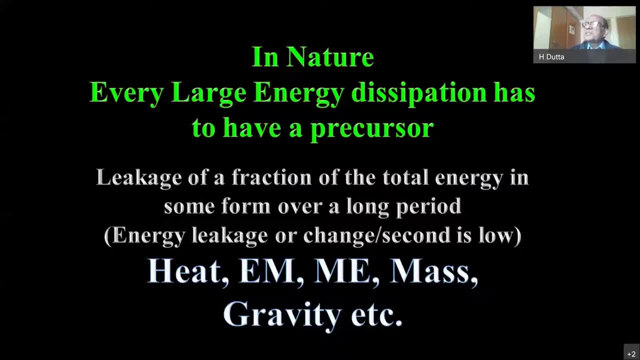 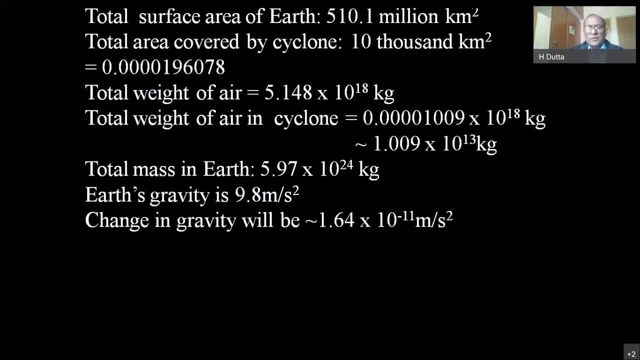 It is not a slaughtering, It is not Nature, is not a individual or things. There is very swirl in nature and everyómテ não tem at all a八 de uma positiva distribuição de energia interested to slaughter the people. Nature is interested to save the people And therefore 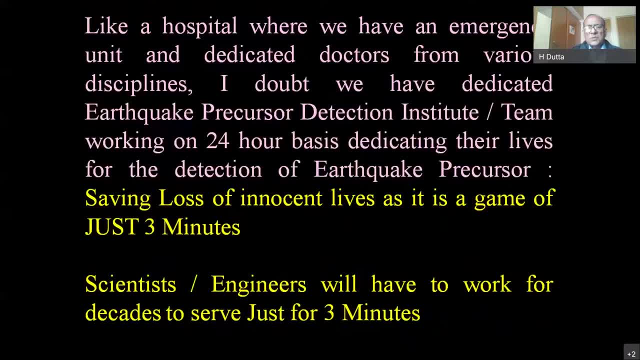 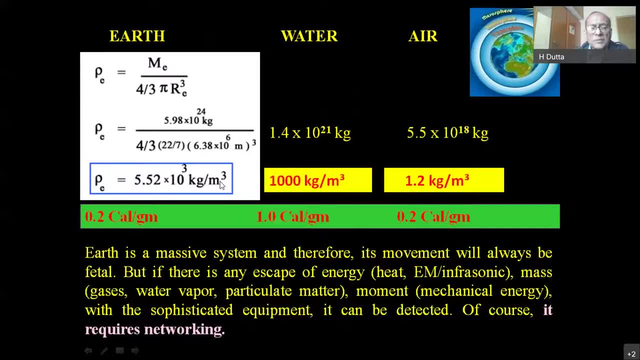 see if – I mean, I will just skip these two slides. So what I did? I studied this. okay, earth is about 5,000 kg per meter cube, 5,500 kg per meter cube and water is 1,000 kg per meter cube and air is only 1.2 kg per meter. 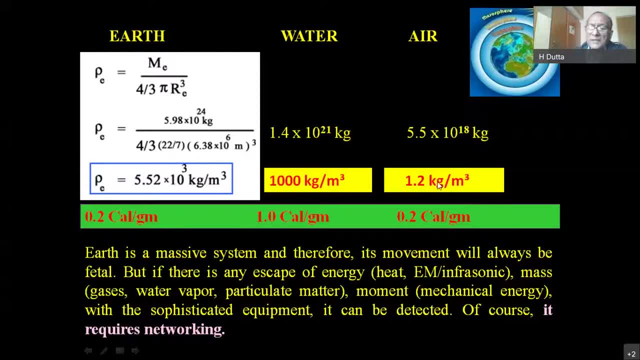 cube, So I am 5,000 times lighter than the earth. So if earth 1 kg if – so I am billion times and my total mass is 120 to the power 18,, while earth has 10 to the power 24.. So 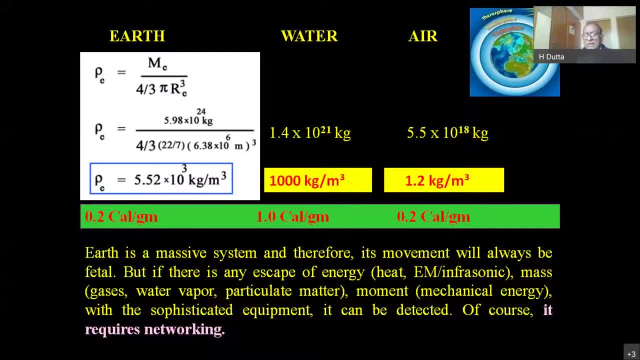 I am million times lighter. Since I am million times lighter if I have to scratch a line. I have already scratched a line, But if I have to scratch a line on my table, it will require 5,000 times more. So I have to use more of energy in order to make a scratch And in solid once you have. 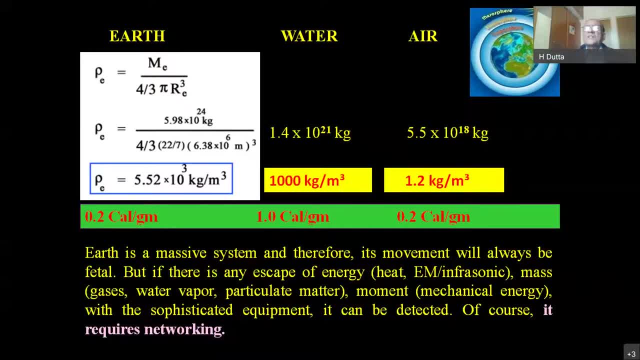 made a scratch. it is permanently visible to us, our eyes, and we say, oh, there was an earthquake and because of that this line or this fracture is there. In water it will be 1,000 times okay. less energy. That means if air is going –, if earth is going to leak. 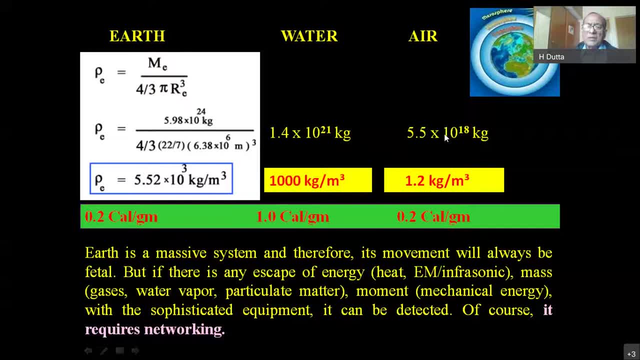 any energy, even if it is –, Okay, 1%, it will be a million percent change for me in the atmosphere. That was the basis for me to think: yes, there can be an earthquake precursor and I need to calculate. So based 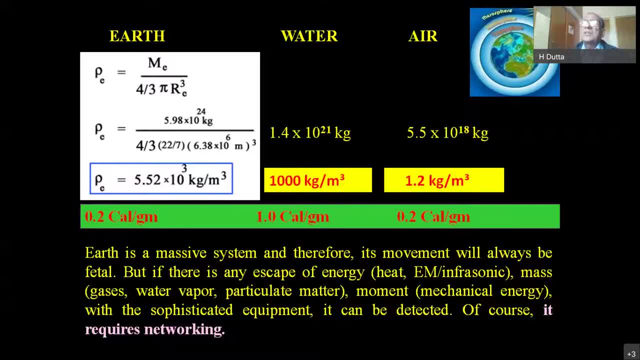 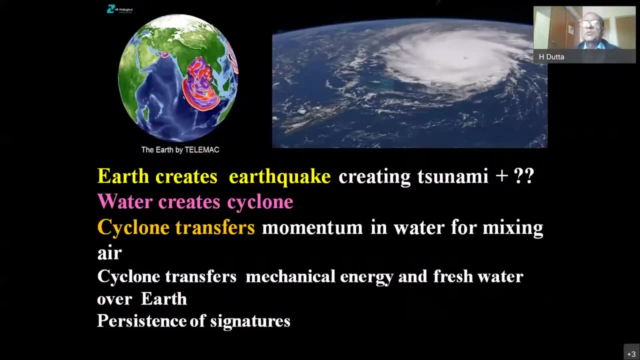 on that. I studied thoroughly about the seismology and earth atmospheric coupling and communicated that paper to nature. Nature asked me three questions. I could solve only two questions. I could not solve three. for the third question, which I had written to about 50 organizations and nobody, 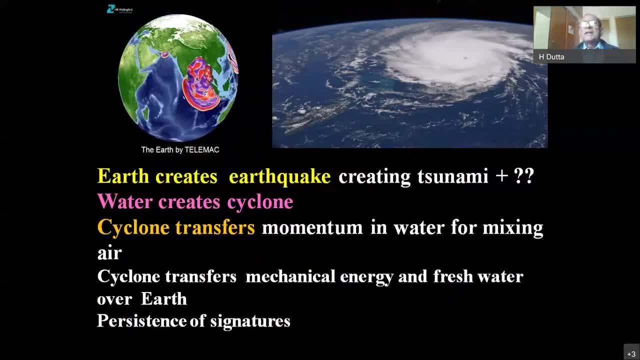 came forward to support, but still I can share that and you can publish a paper. So, earthquake, you can see the impact in the atmosphere if it is – because earth, otherwise air, is not visible, But on my instrument it is visible. So in the atmosphere you can. 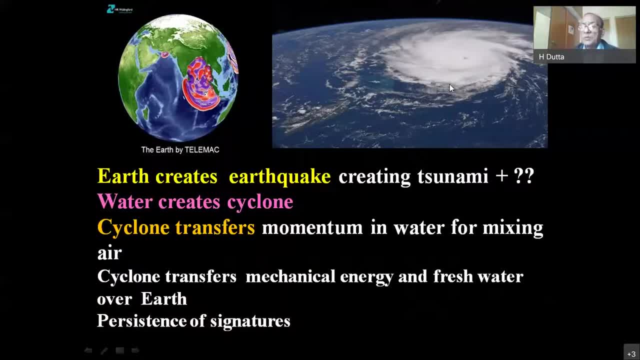 see the impact in the atmosphere, But on my instrument it is visible. So in the atmosphere you can see the impact in the atmosphere, But on my instrument it is visible. So in the look at this you are able to see a cyclone. because it is water vapor is associated Clouds. 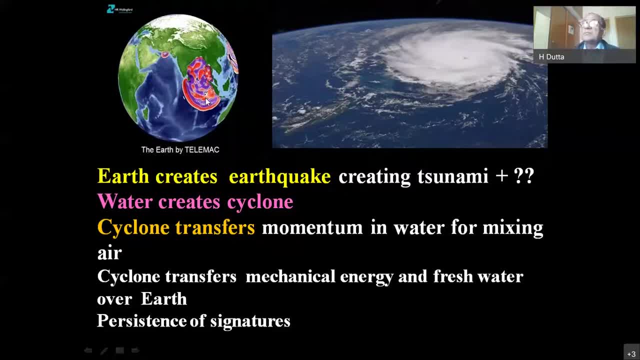 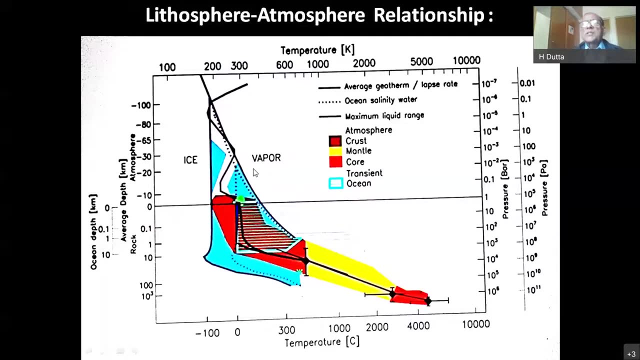 are associated. You are able to see tsunami because physically you can see and the pressure difference is there. It moves at a much slower rate compared to what happens in air. So these are all the lithosphere-atmosphere relationship. Couplings are there And wonderful. 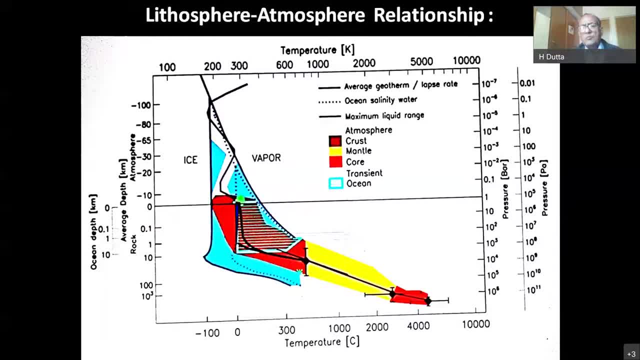 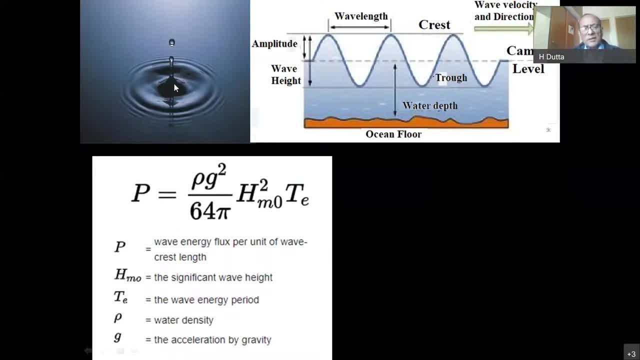 that, how much energy is released and how much is going to be changed. This is what. since you are just throwing a bubble or a stone or a rock, you can see number of what is called waves being created and you know the energy. And similarly, exactly in the similar 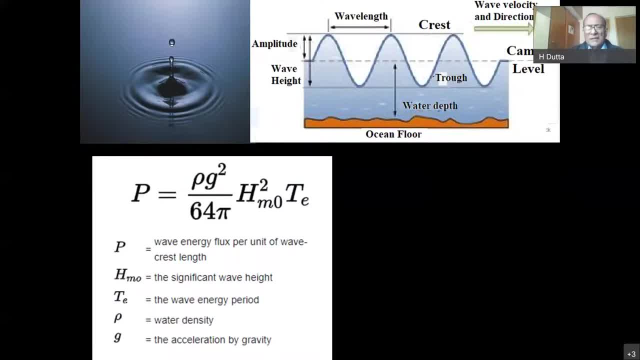 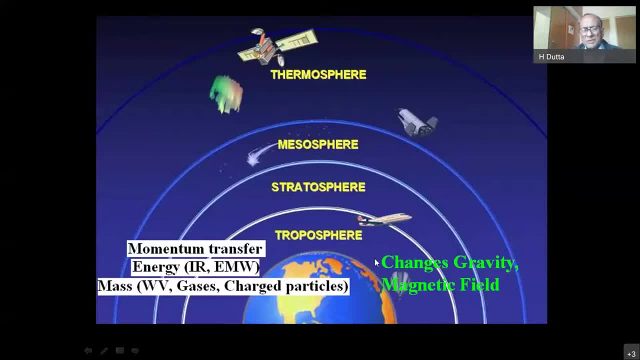 fashion are the waves traveling in atmosphere. And so, if you look at the atmosphere, nature has gifted atmosphere, Just not for the sake of just breathing. I'm sure such a massive system of 10 to the power, 24 kg- having such a light system of 10 to the power, just 18 kg, million times lighter. 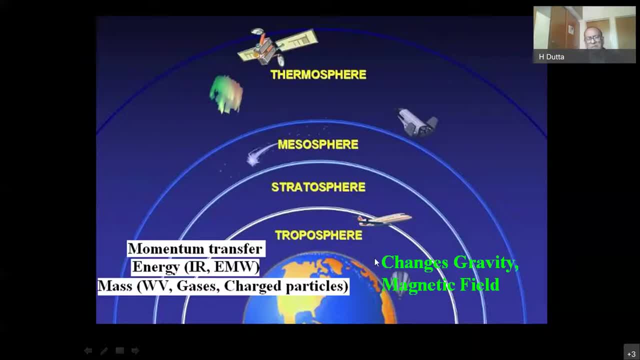 must have been created in order to see whether there is a momentum transfer, energy transfer in terms of electromagnetic waves or infrared, or a mass transfer- water, vapor, gases, charged particles and particles coming And they are. they get amplified, As Dr Rao in the morning showed you, the TEC being measured. 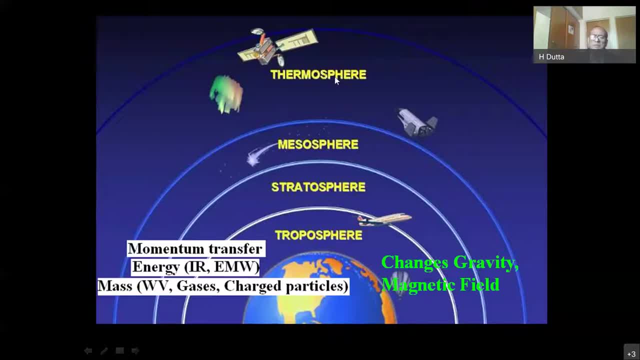 I also published a paper very, very initially and we published in International General Remote Sensing about the TEC. But as you go away from the surface, the errors will increase And fortunately I sit right on the surface. Okay, And then there are three changes in the three. 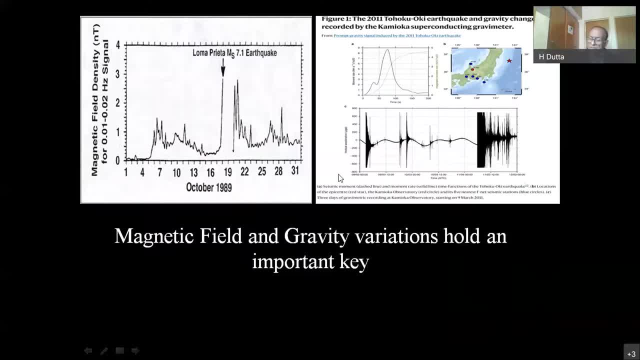 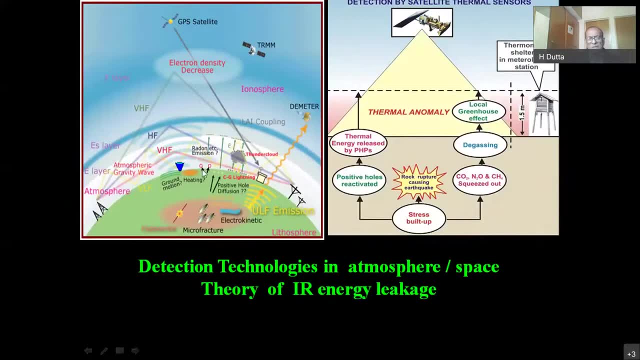 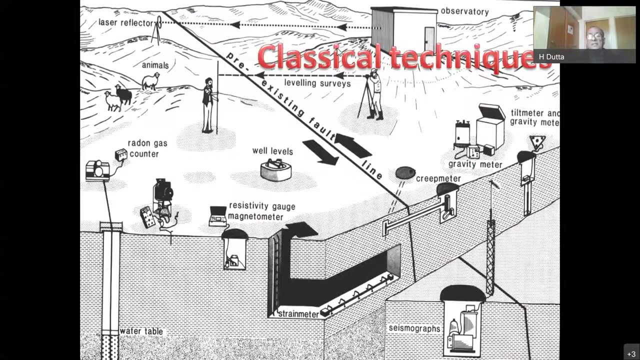 components of the magnetic field and gravity field. They hold the important key. And then these are the systems which we need to see. The basic problem is seismologists had made in classical thinking because seismologists thought that okay, because it is an earthquake, so its precursor. 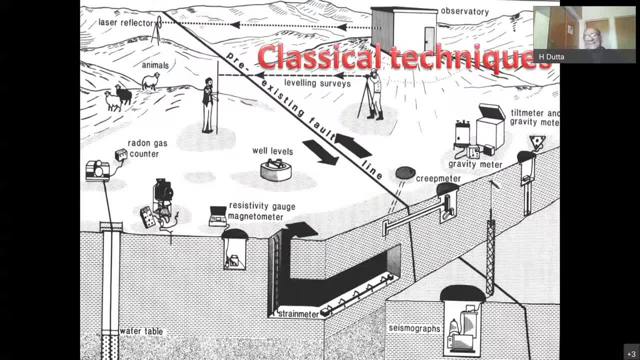 must be sitting in earth. That is wrong. The precursor is sitting in here. The precursor is sitting in the energy. You don't have to look at the earth in order to know the precursor. That was the. I mean. all these thoughts came to my mind as a lay man, as a person who had 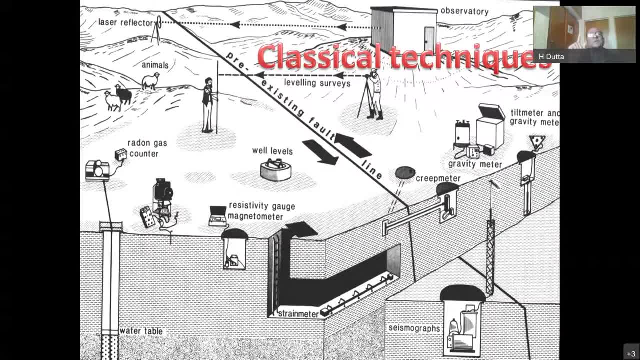 never studied what is called earthquake And I was 55-year-old, I had decided that, okay, let me file a patent. Okay, Because India had no patent in the field of earthquake precursor. Dr Kudwila Singh. Dr Kudwila Singh. 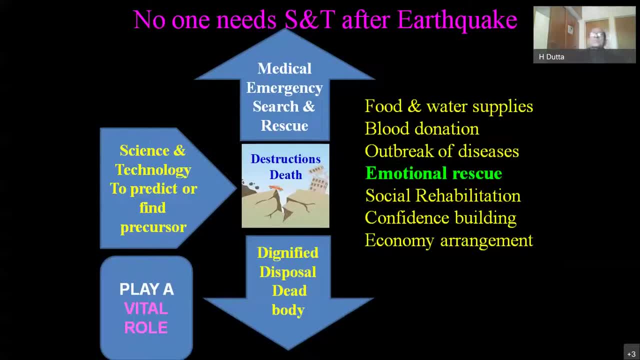 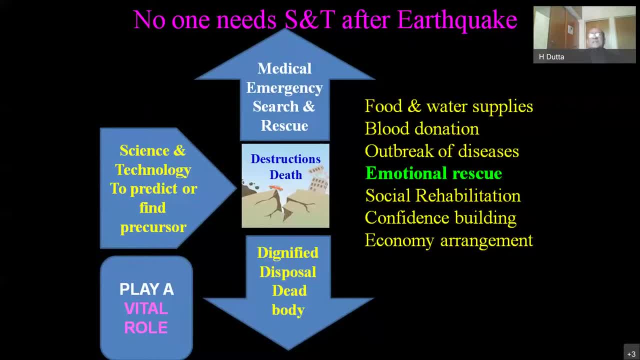 was in 2005 that the patent was granted. so three, four years of my life i had. like a mad dog, i worked to get that patent because you have to first deal with your liar, you have to deal with your what is called planning and monitoring agencies- this and that. 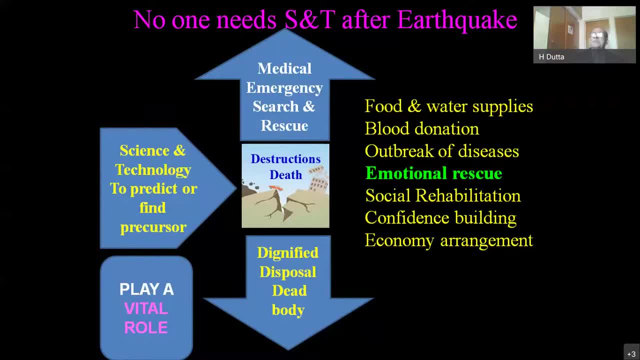 you know, when you are working for the first time you have to face so blunt questions, comments and all that. have patience, work on scientific lines and be bold. i'm sure the the nature was great. no one needs science and technology after earthquake. science and technology: you must find a precursor and play a vital role, because then you need to. 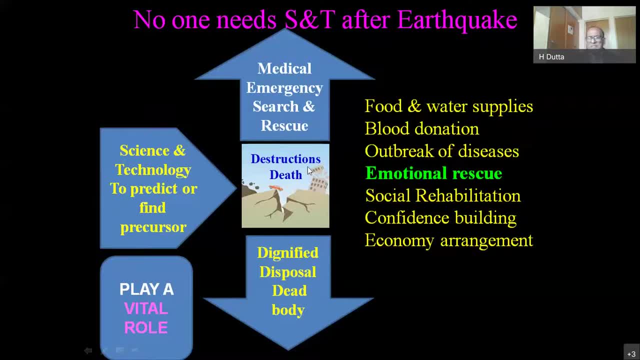 you will stop medical emergency death destruction. you nobody can stop, but you can stop death. you can stop dignified disposal of that body. you don't have to worry about the dead bodies like this is what is happening now in in cyclones and the rf and nidm teams. you know they are able to. 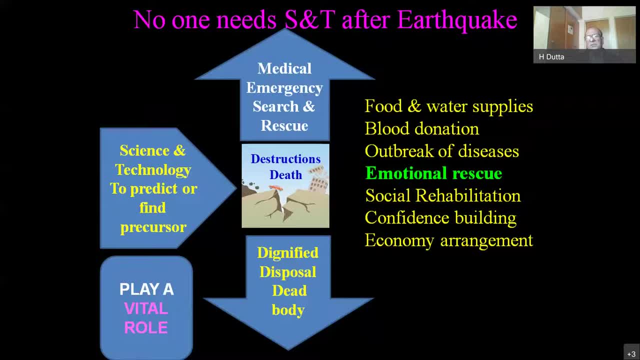 handle so well, but you require the energy of food and water supply blood donation. you know you will be able to handle so well, but you require the energy of food and water supply. blood donation you will not require. there will not be an outbreak of any diseases. you don't have to go for a emotional 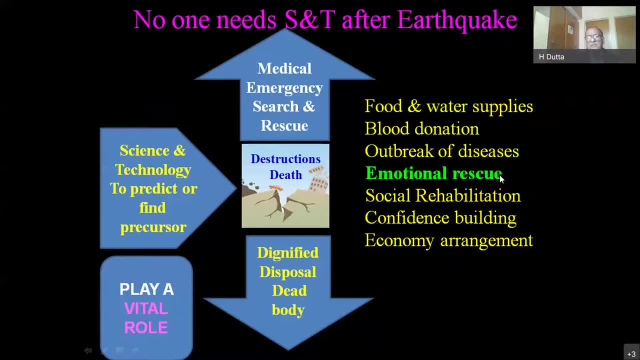 rescue. this is very important aspect which we never touched. the woman force has to be, have to be, has to be there in order to give you emotional rescue. don't worry, if your father has died, i'm your father. if somebody has died, i'm your mother. we will take care of you. 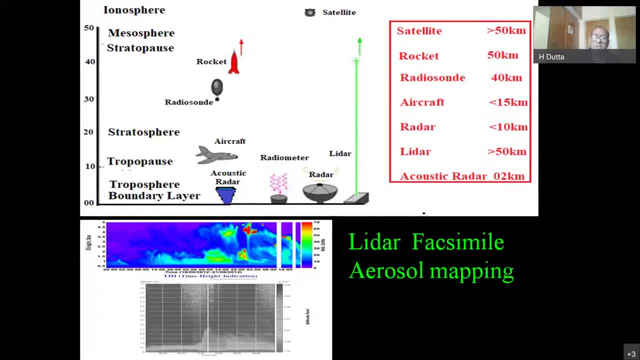 so, ladies and gentlemen, large number of observable techniques are there which we need to try. so, ladies and gentlemen, large number of observable techniques are there which we need to try, which we must put them in an integral part, as an integrated part: lidar light detection and ranging immediately, the moment you know, aerosol. 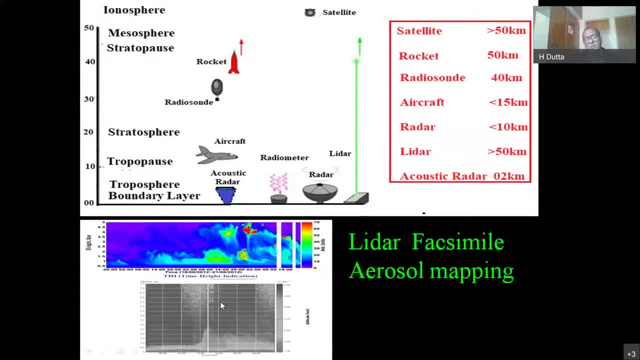 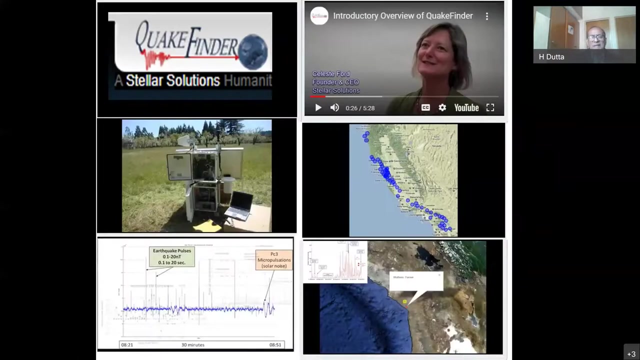 saying concentration will increase from the surface. you are sure? yes, this is because of the earthquake uh precursor. so you have an acoustic radar, you have radiometers. so radar, eventually it will be the rar, dar, acoustic radar and satellite. they are going to be the rules of world as far as earthquake precursors are concerned. there is a company called quack finder. 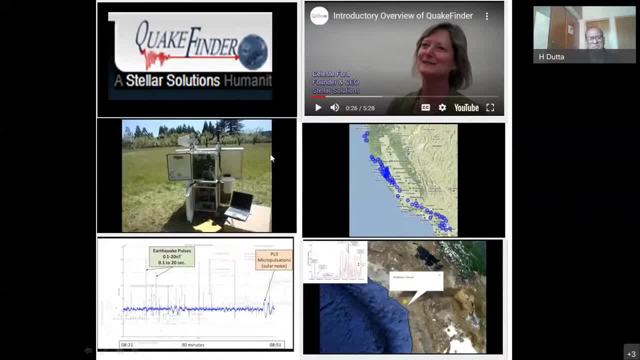 oh my goodness. they are working in 40 countries just monitoring, you know, three components of the magnetic field. i'm in touch with this company, the gentleman doctor, the, the main principal scientist. i'm working with them. okay, um see, if they are. they are california based, the company is. 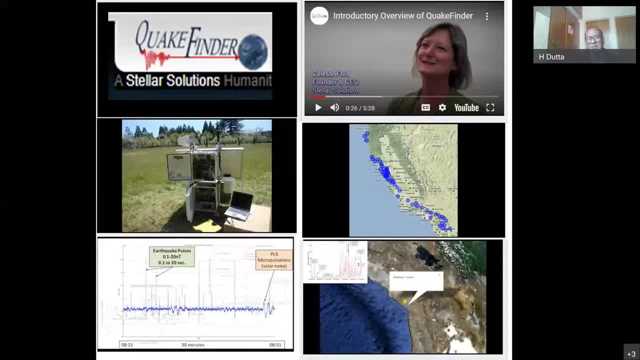 in touch with them. okay, um see if they are. they are california based. the company is in touch with them. okay, um see if they are. they are california based. and uh, they are working in 40 countries because we do not have an earthquake in india. that doesn't. 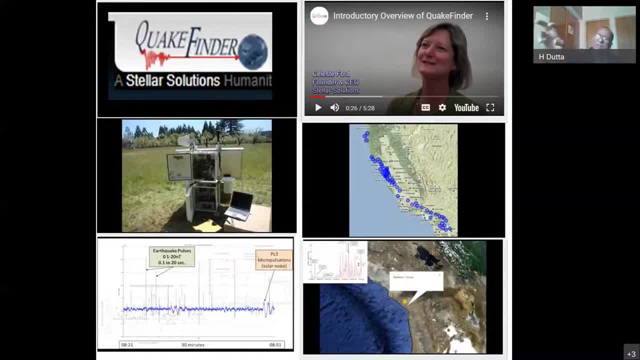 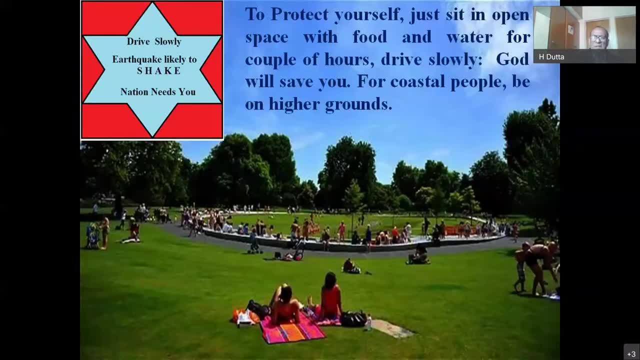 mean earthquakes are not elsewhere, so we have to go there in order to get the experience. it is not a problem of india, it is the problem of the whole world, and to protect yourself you don't have to go anywhere, like in the case of cyclone. you have. 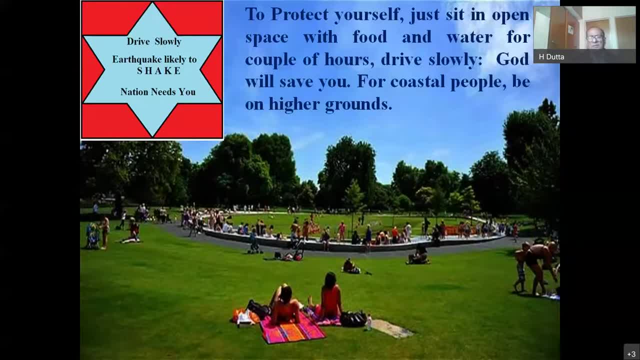 to shift all the people you know deep in the interior of the, you have to just sit in the parks, you have to sit away from the infrastructures because earthquake- if a big earthquake is going to strike, please believe, because of our infrastructure, with tall infrastructure, tall buildings and our density of what is called the population, is going to be a real disaster. 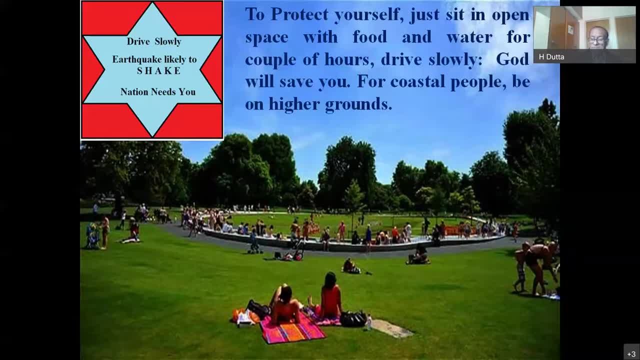 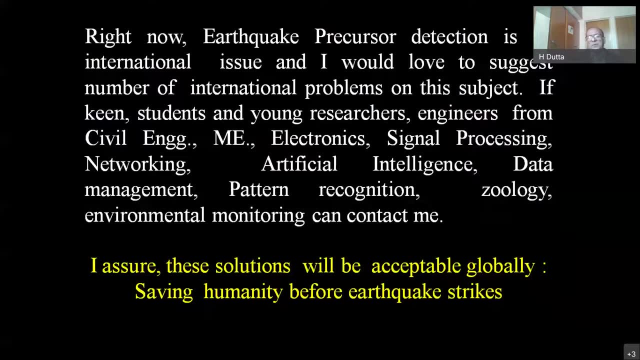 are we prepared for that? god only knows. so, right now, earthquake precursor detection is an international issue and i would love to suggest- uh, specifically, i am addressing the young participants- their kids. you see what is the difference between you and me? i have the experience and you have the 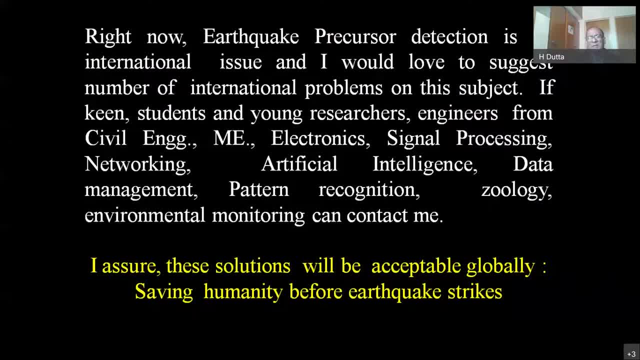 energy. let us couple it. so i would love to suggest a number of international problems on this subject by taking an international patent. i know i know there are more number of questions to be answered and but let me tell you all that phd or, if you are interested, 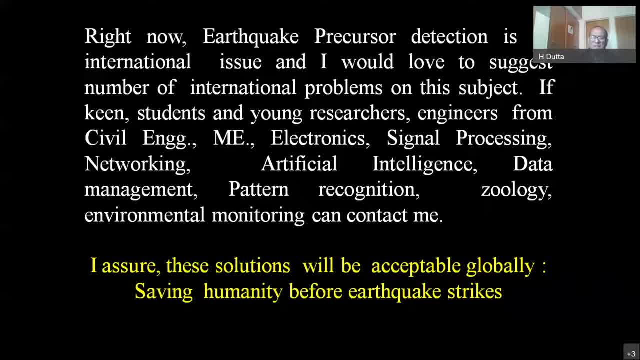 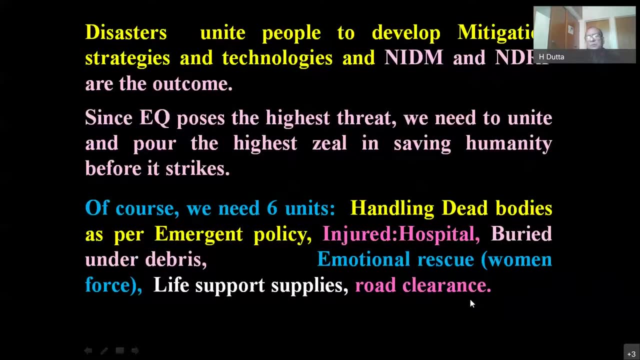 to start your own industry in this area. i'll be able to help and and your problems will be well acceptable globally. and we have to save what is called save humanity before earthquake strikes. that should be our motive. so disasters unite people. if there are, there are no disasters. 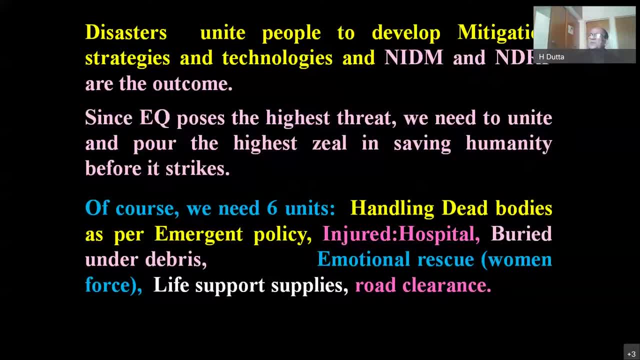 we will never be together like: look, look at ukraine. they're together because, because there is a disaster, there is need. so disasters unite people to develop meetings, to develop communication strategies and technologies, and an idm and ndrf are the outcome. since earthquake poses the highest level of threat, we need to be united and for the highest zeal in saving humanity. i 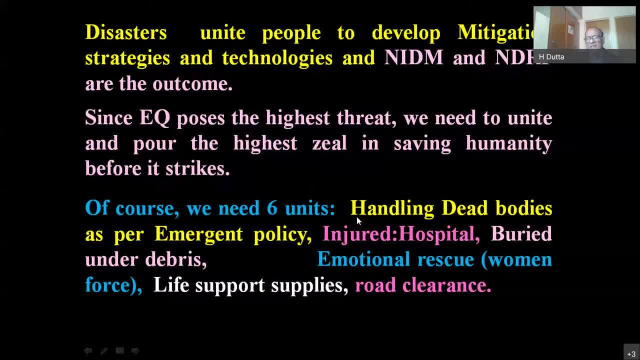 personally feel that while handling- because this is what i experience- there should be different types of teams handling dead bodies. because that body is, they'll go in a different has to be handled. it's the last priority to be handled as per emergent policy of the nation injured, they need to be carried to the hospital you have to find. 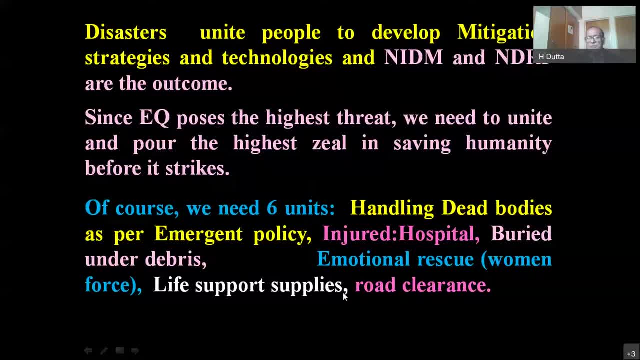 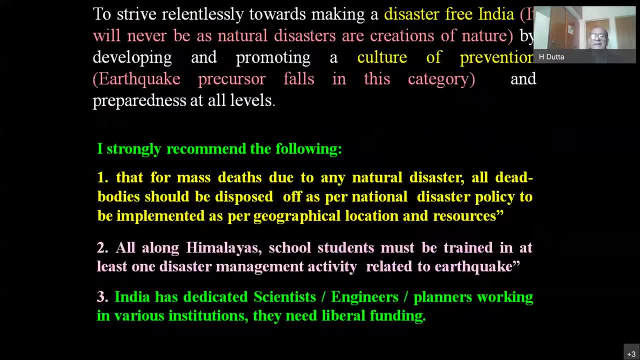 by find people buried in and then emotional rescue, life support system and road clearance is very important. so in an idm i could see that you have written to make india enough towards making india disaster free. let us change it. it can never be disaster. we are challenging god. we are challenging. 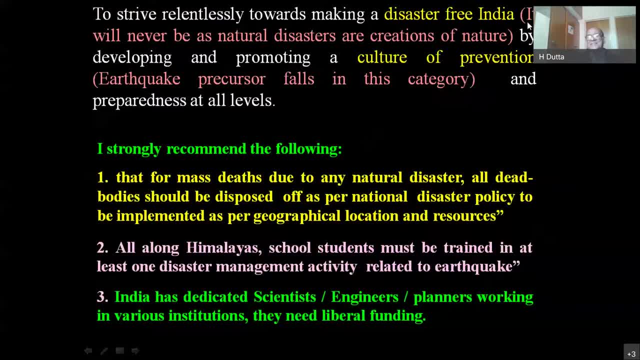 nature, disaster free cannot be there. we can minimize, okay, we can minimize the impact because it is equal to mc square, brahma vishnu mahesh. so change is inevitable. ultimately, the earth will decay, earth will die one day. okay, so please change it. and then i strongly recommend the following: that 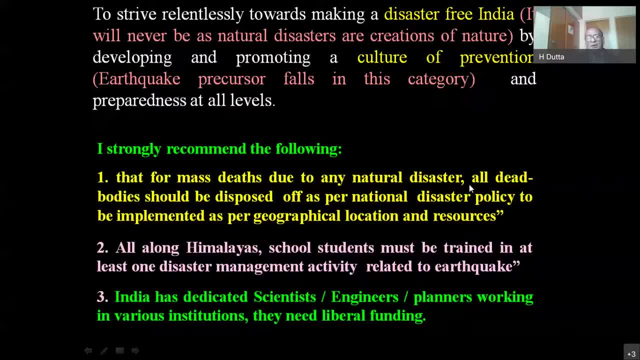 for mass that's due to any natural disaster. all that body should be disposed of as per national disaster policy, to be implemented as per geographical location and resources. somebody has died around the coast. the best is the sea burial, which we do not have. we have never accepted it. 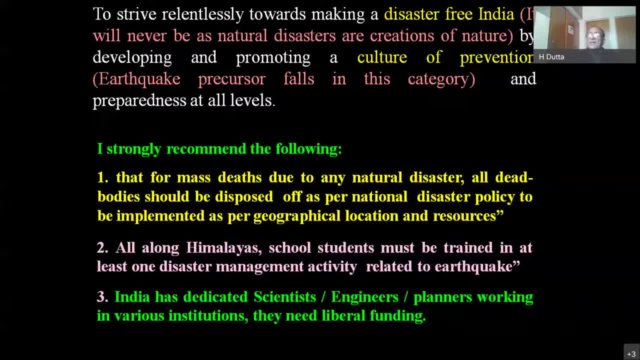 please change it. this is the need. see, once you are dead in a disaster, then we look at the government. then government has to frame a rule. okay, i was going to work in a country and i wrote to them that if i died while working in earthquake precursor in india, i was going to die in a country and i wrote to them that if i died while working in earthquake precursor in india, i was going to die while working in earthquake precursor in india. 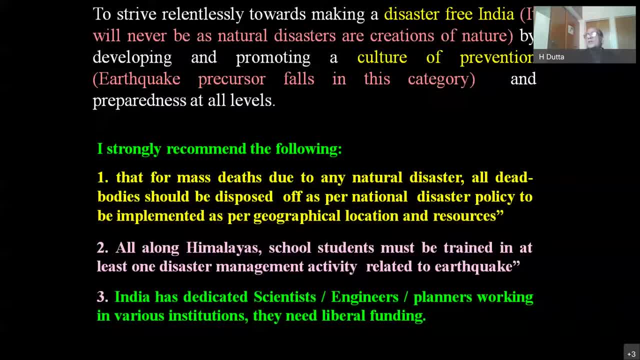 in your country. my body should be disposed of as per the rules of the of the society over there. i cannot isolate that. okay, i'm from india and i must be buried as per my- uh, my, my, religion. no, the religion doesn't come, it comes the nation where you are working. 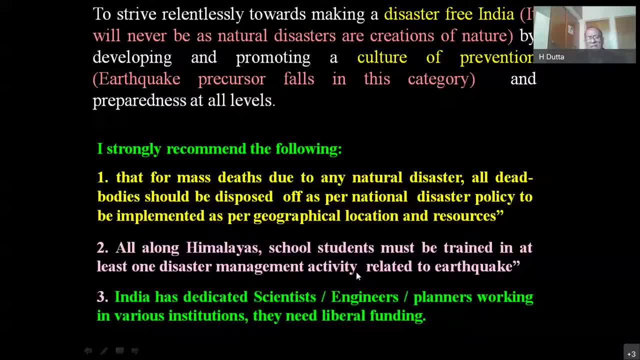 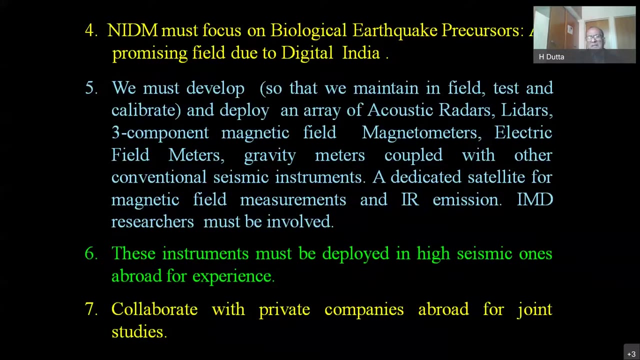 all along himalaya. all the students must be trained in one at least one disaster management activity. very important. india has dedicated scientists and engineers and working institutions. they need to be given liberal funding. um, i'm sorry. the funding itself is an idea. must focus on biological earthquake, because the kind of respect i have developed for for our reptiles. 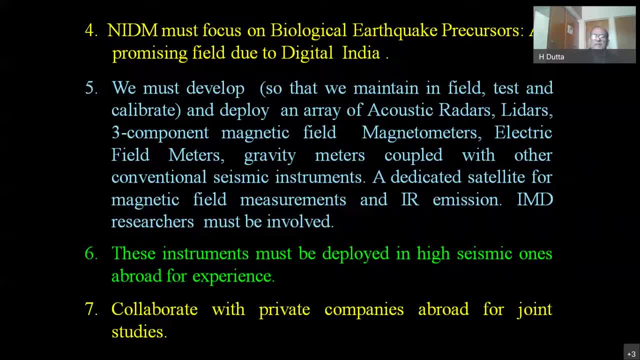 my goodness. i'll just explain to you a promising field due to digital: digital. india- you have to just put a tag, you have to put them in. china has started a laboratory for, you know, reptiles and, my goodness, they are the best biological precursors we must develop and maintain. 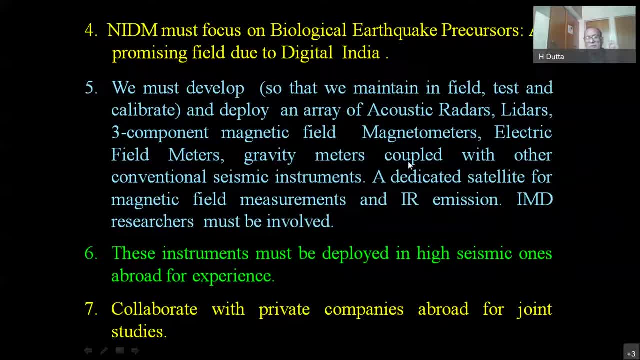 developed technologies, okay, and technology so that we know we we are able to repair, we are able to find, calibrate them, we know we visualize the data because it is, it is for the useful usefulness of the humanity and these instruments must be applied not only in seismic uh, what is called active zones. 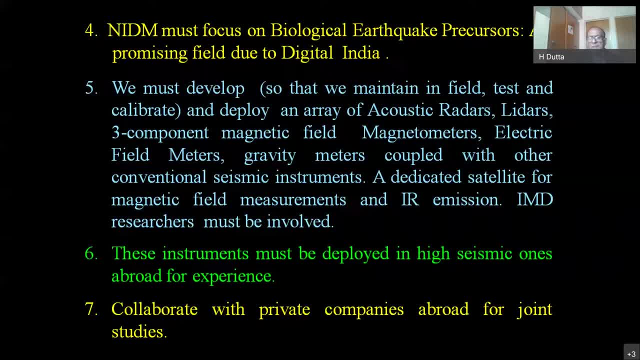 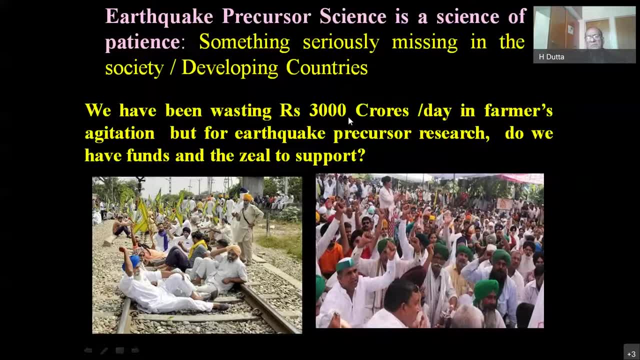 and uh, we must put them even abroad and collaborate with private companies. uh, brought for joint, uh, what is called observation. we have been, you know, wasting 3 000 crores of rupees per day in farmers. education continued for one hour, continued for one year. but do we have the money? 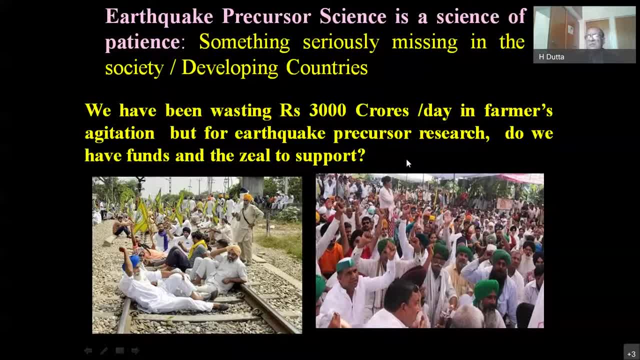 for earthquake precursor research. if we last 10 crores, oh my goodness, 10 eyes will be there and people will desire the result. outcome: as i said, there is no patient. people will say, okay, you are fine. what is the objective? what is the? how much? what are the? 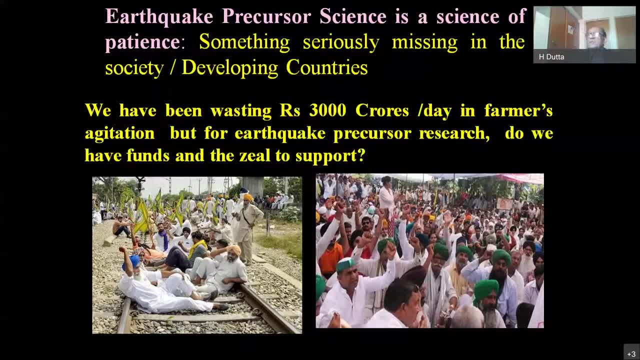 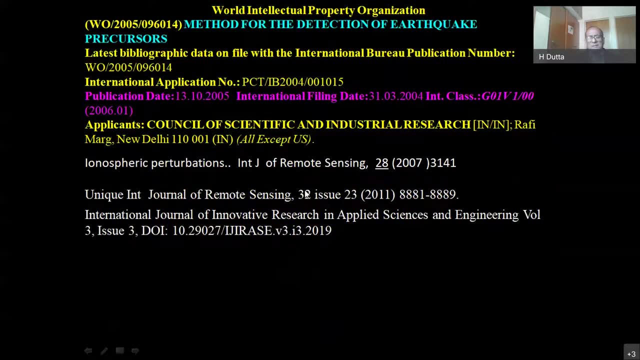 milestones. my goodness, you don't believe your own scientists, you don't believe your engineers, and give them freedom. that's very important if we have to work seriously. so these are some of the publications which we did in international general of remote sensing and this is the. these are the details of the what is called patent that we have. 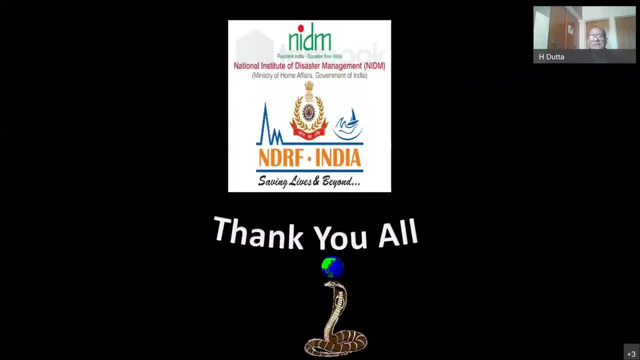 taken and with these words, let me thank nidm and ndrf. a great job indeed you are doing. i'm very happy that you are in delhi and since i am from delhi, i must thank you all. thanks to all the participants and distinguished members. my goodness, the kind of respect after taking, uh, you know what? 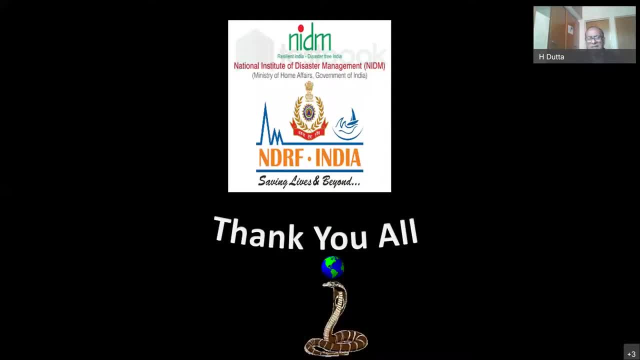 is called the earthquake precursor patent, the kind of respect i have developed for king cobra. wonderful, wonderful instrument, it doesn't it? it doesn't require acdc, it can eat both vegetarian, non-vegetarian, lives for years together and it climbs onto the trees in order to minimize the 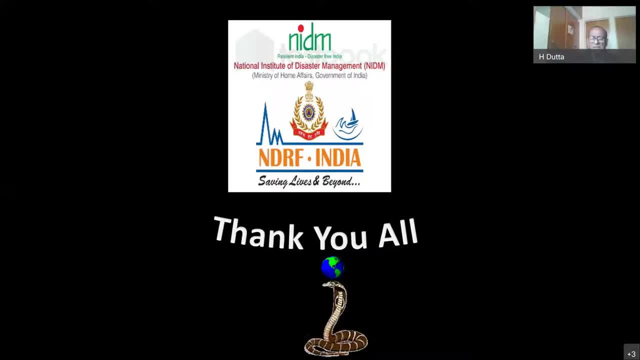 electrical potential near the surface of the earth. it is. it has got no years, so it is seismically active, the wonderful instrument which nature has gifted us, and, i am sure, rishi munis, and that is why we respect them, that is why we worship them. so, with these words, 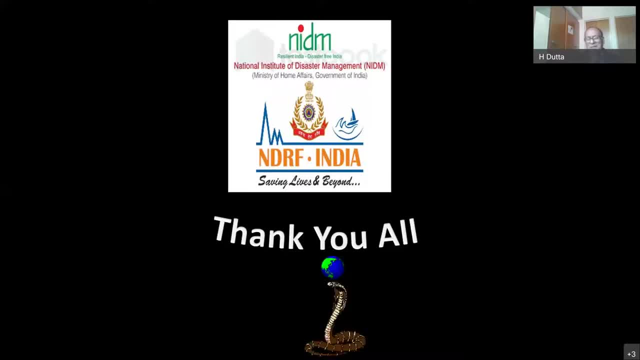 let me thank you all and thanks dr halder for giving me an opportunity to express myself. thanks, dr. you have given excellent talk on this precursor of earthquake throughout life, what you have done, especially on the radar activity in antarctica in the odd climate, what experience did you have in the buttocks of the attacks in the world of about you know back them. are so many things, so many things throughout life and, obviously, the 24 hours that we are happening in the coming week. you have shown us the exact steps which will help you to take these steps so that they are very effective in the future. so thank you very much, i would. Mooji, you are welcome to. 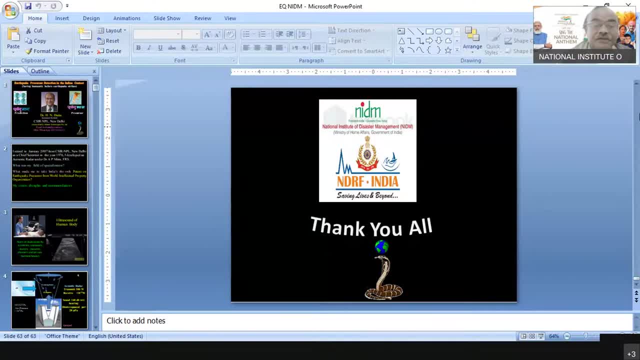 experience you have especially, and you rightly said, that is the very best place for absorbing or for getting all types of waves. and from there you have started, and before that was you have started your journey, and how the this precursor especially. you were rightly told this is the. 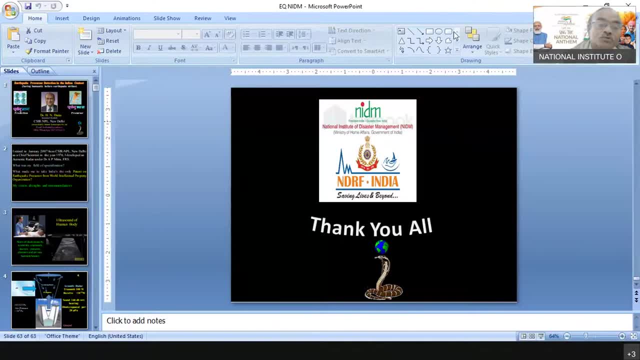 integrated things and it needs patient to work out for the precursor. now. i thank you very much. now with us, our professor ramesh singh is with us, so he wants to put his certain views on this. so i welcome dr professor singh in this context. now we are handling the stage. you can continue what you. 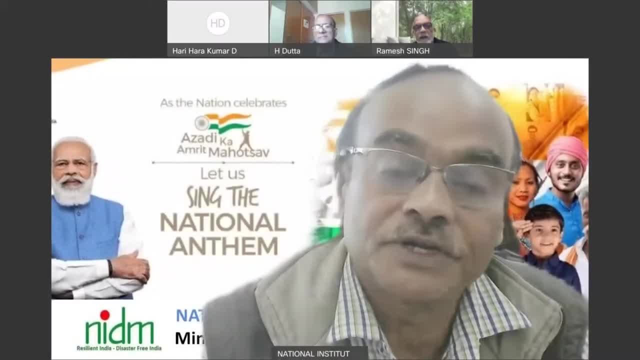 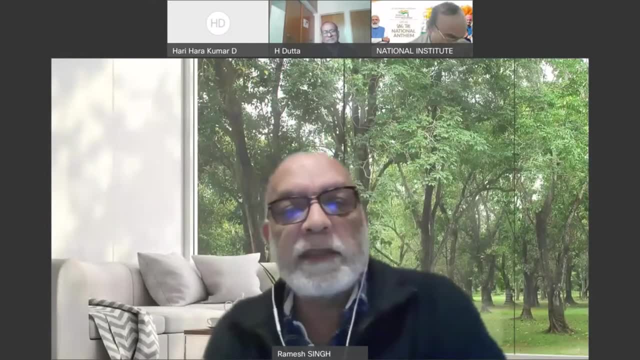 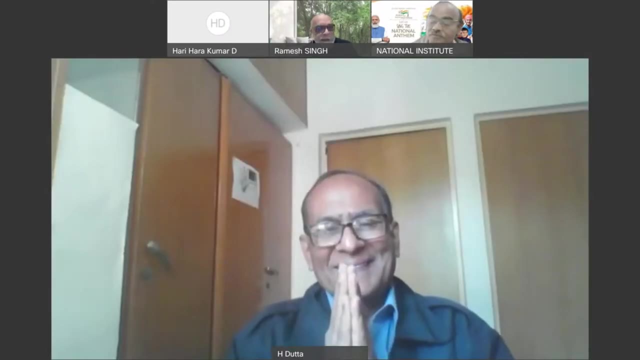 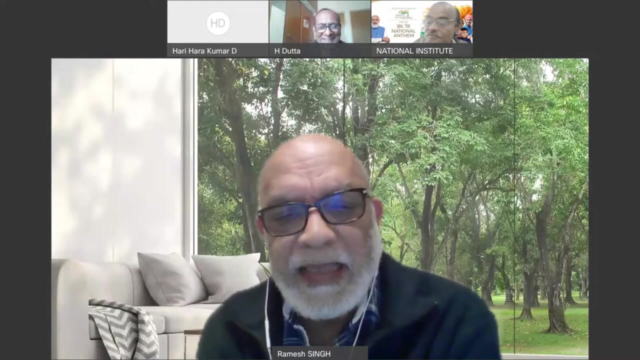 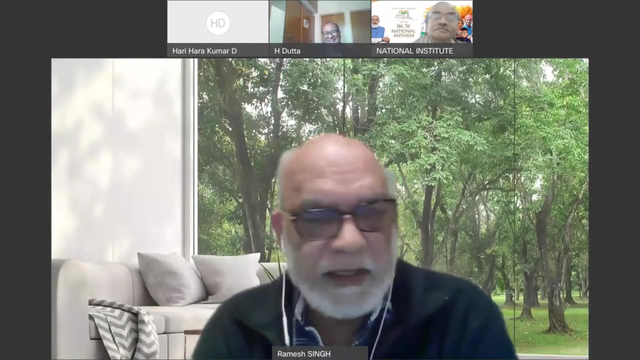 would like to add or what you would like to complement further. thank you, dr haldar, dr surya prikash, so i hope you remember me. i'm very happy that you, you presented very uh, your gravity waves and also great you for the patent. i remember 20 years back. 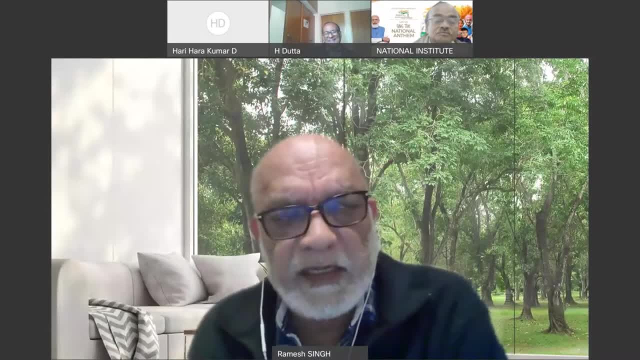 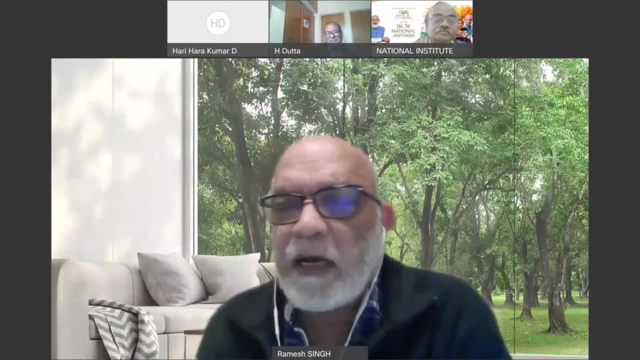 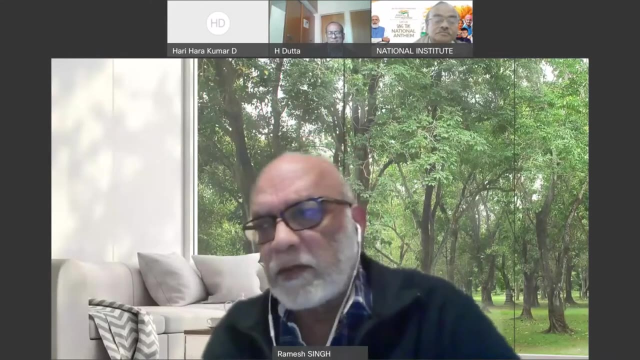 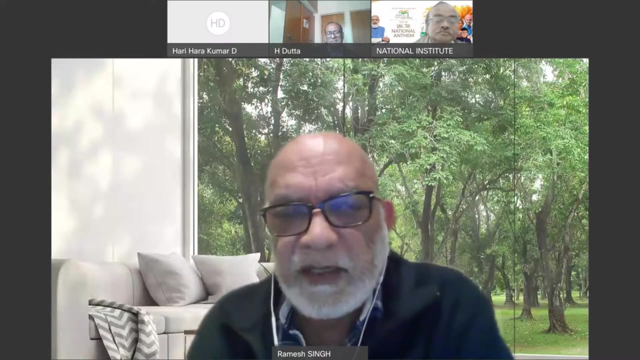 dr dutta was very much excited with this observation, what he did and, of course, the earthquake is very complex phenomena and we make a complex and i'm also working since so many years and whatever the um Dr Datta experienced, that he submitted a paper in Nature and things like that. 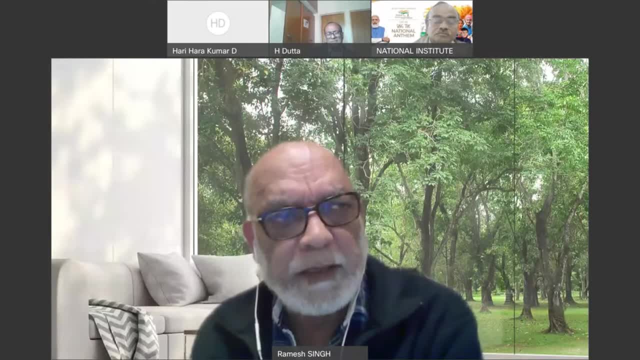 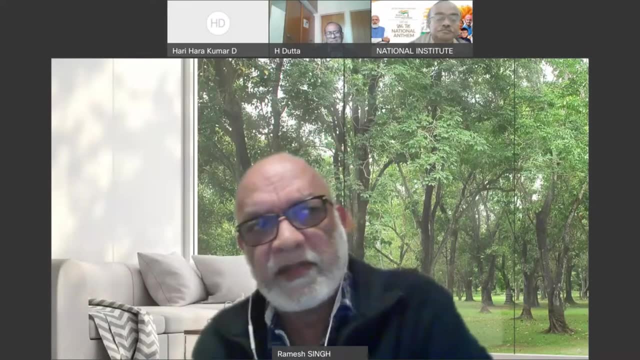 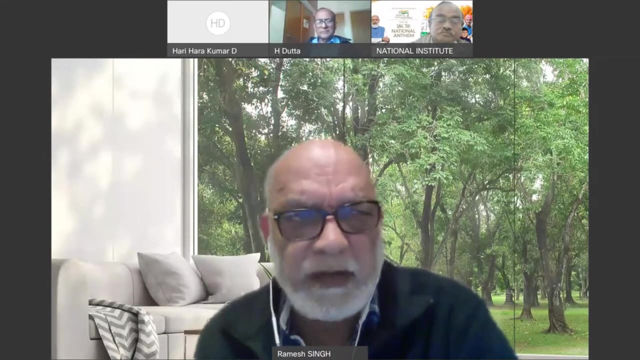 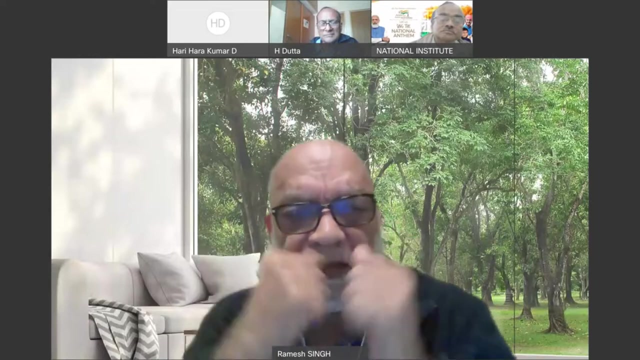 The Bhuj earthquake is a well-studied earthquake. okay, we did a lot of work And I know since the last three decades, in the name of the earthquake, people they fight, they quarrel, okay, and everybody would like to claim that I get a success in the earthquake. 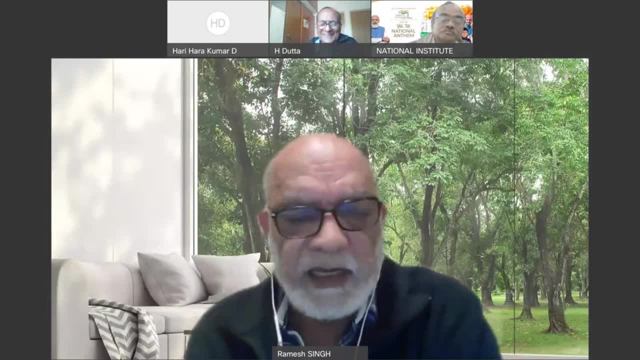 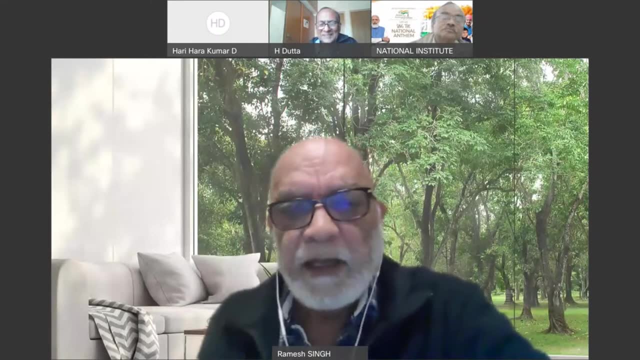 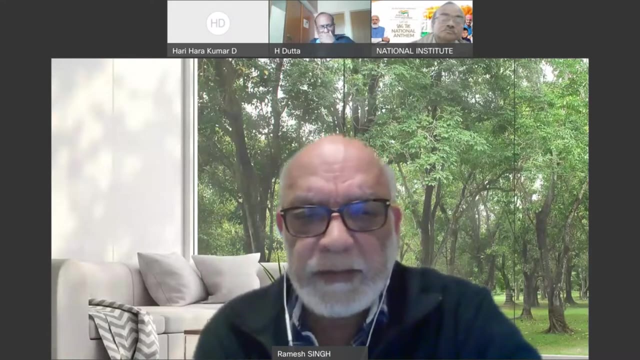 prediction, the precursory studies, And even our former President, Abdul Kalam, was very much excited. okay, The world has spent millions and billions of dollars. I'm sitting in the US In the name of earthquake precursor. I cannot. 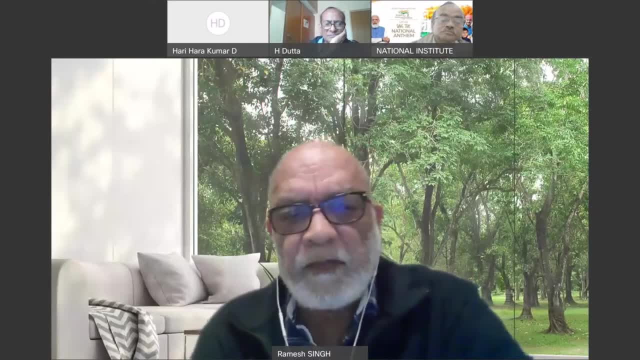 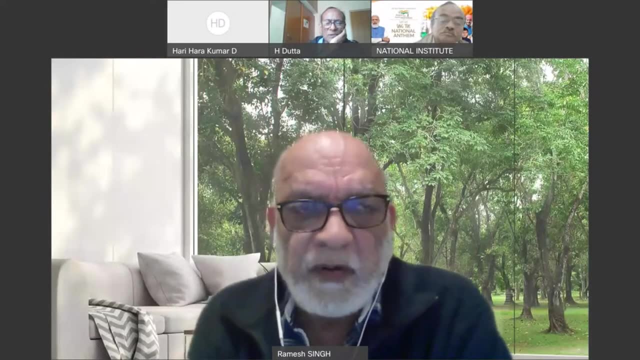 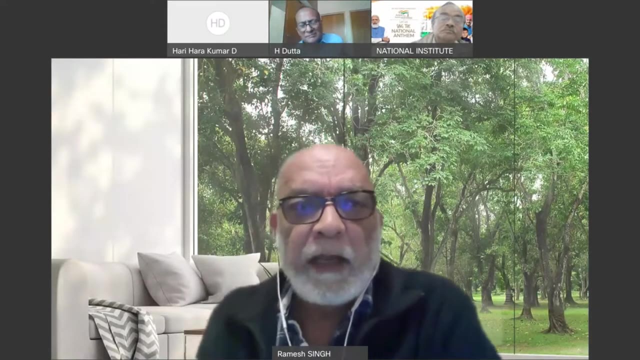 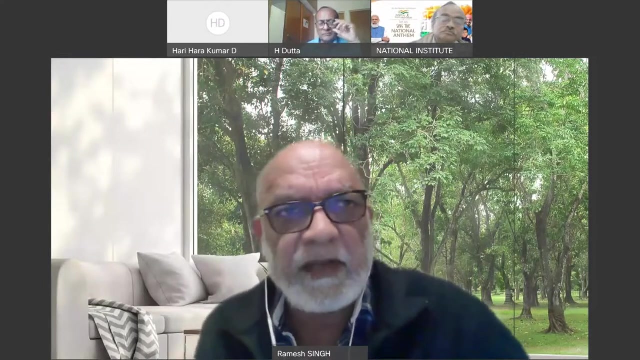 I cannot get a penny. And when the Bhuj earthquake occurred, there are so many parameters we observed And whatever the like. Dr Datta said he got a patent. I also got a patent on the surface latent heat flux And I also submitted a paper in Nature, and Nature asked the same question: what Dr Datta? 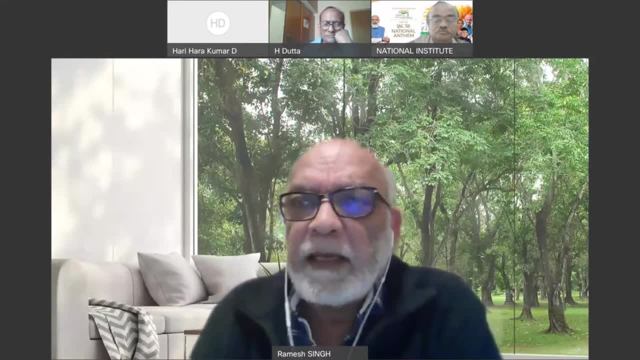 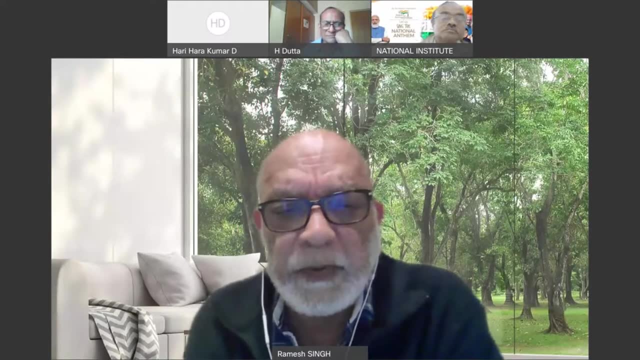 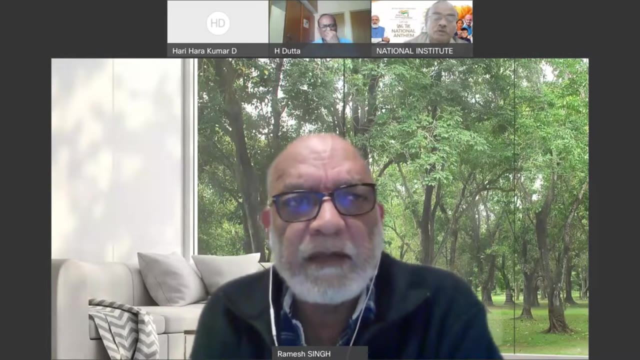 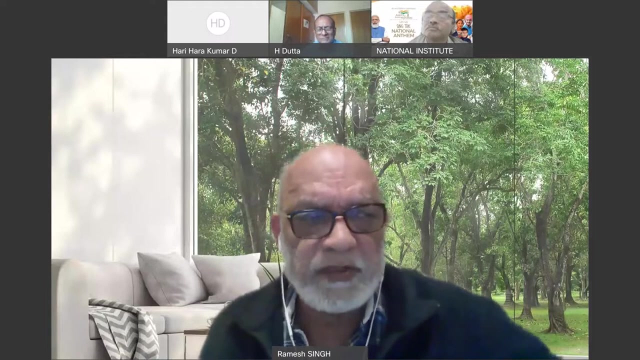 said He got, and I hired 15 students in my lab at the Indian Institute of Technology, Kanpur And I did not get the answer to the questions raised by Nature, people, okay, And after that I came to US- one of the students, he did a PhD and the people. 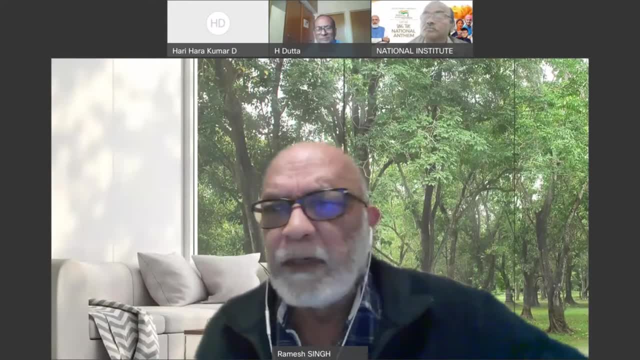 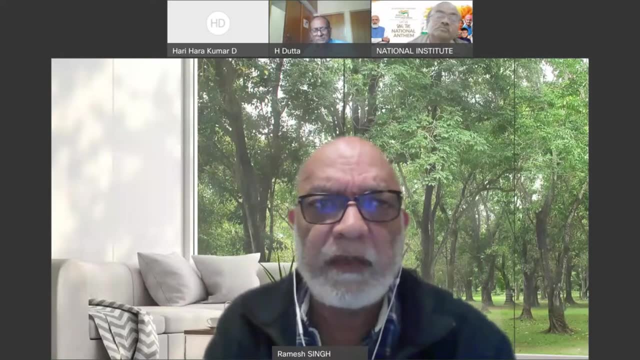 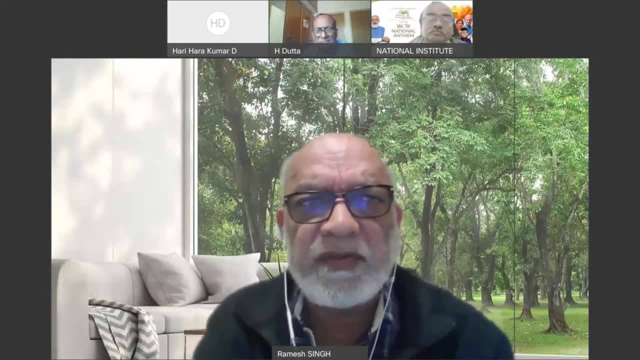 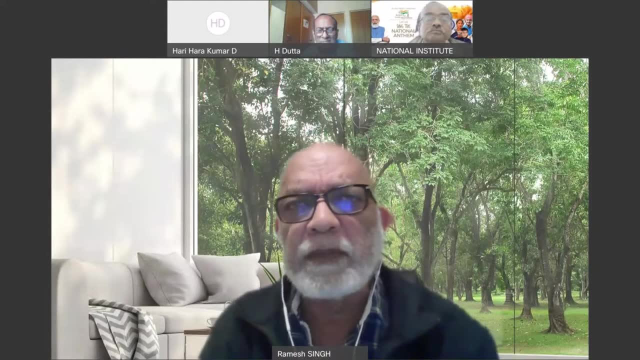 students to do precursory studies When I was doing my master's. since then, I know that people they are so excited that there will be an earthquake in Assam and they were doing a lot of measurements But we did not get it okay. 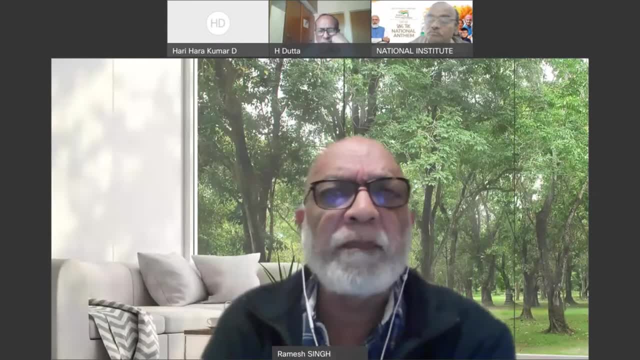 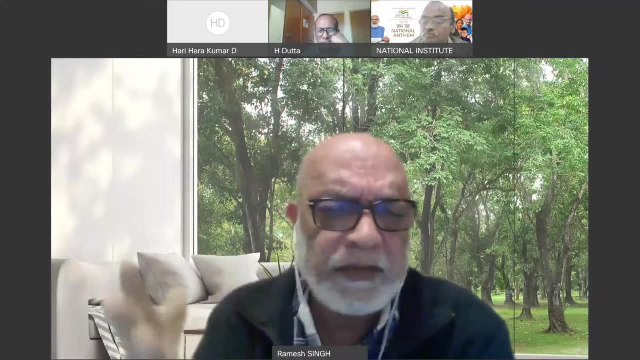 And I know in the country there are the multi-parameters observatories: One is in Assam, One is the somewhere up in Himachal Pradesh, One is in Gujarat. Okay, They are recording so many parameters, Okay. So this is really very complex and people like Datta if they do research, fine. 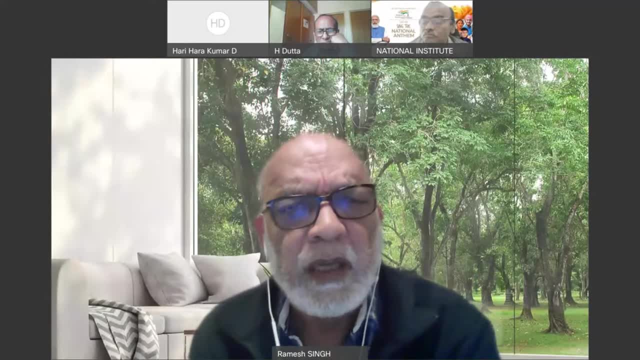 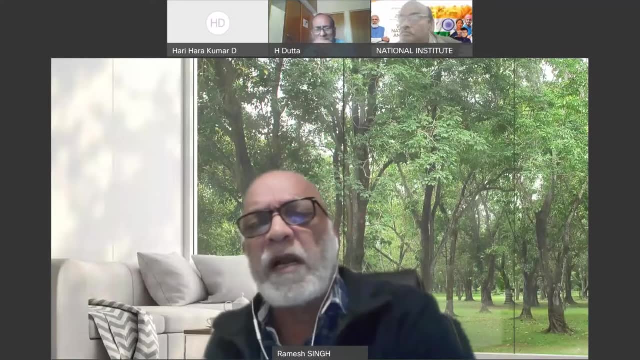 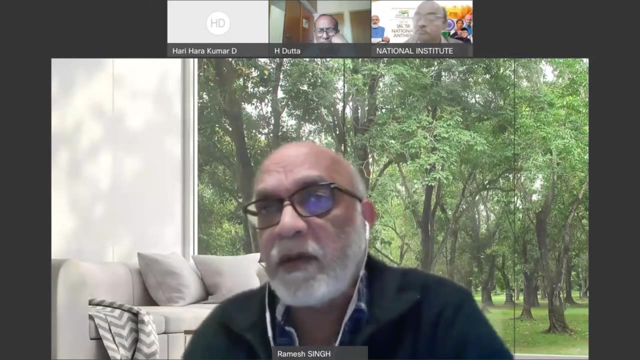 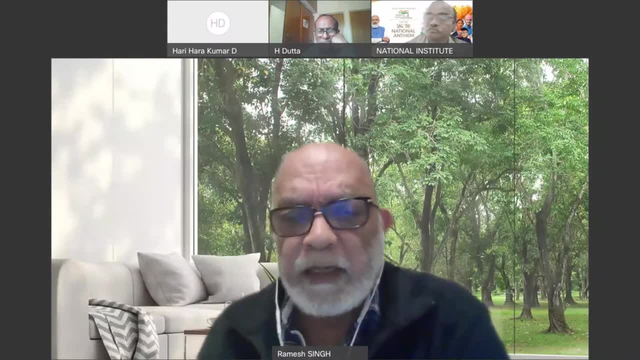 related within multi-parameters and, like in NIDM, I gave a talk on the coupling, the coupling between the land, ocean, atmosphere, atmospheric coupling- okay, associated with the all kinds of natural hazards. Okay, So I am a bureau member of the Electromagnetic EM induction. 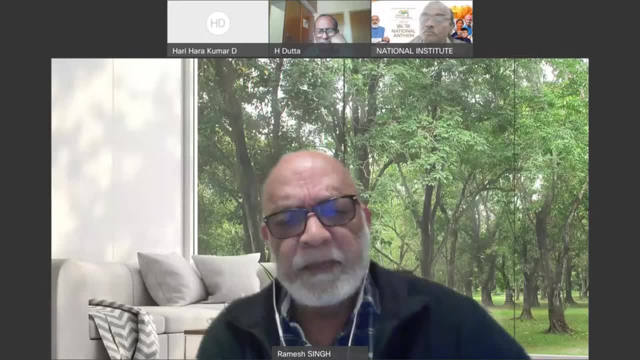 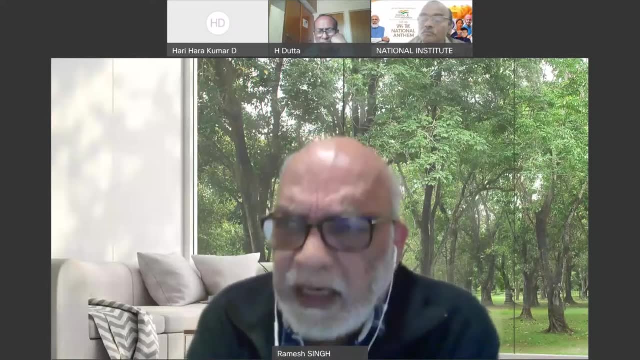 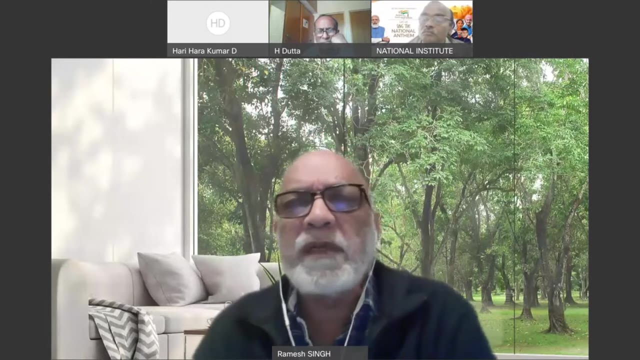 Okay, And we, always, we are trying to say: I what I hate people that they, based on the one parameter, they can say that, oh, I can't predict the earthquake. Earthquake is a very, very complex, okay parameter. 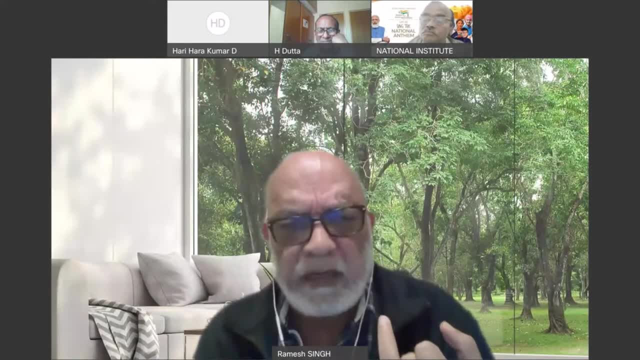 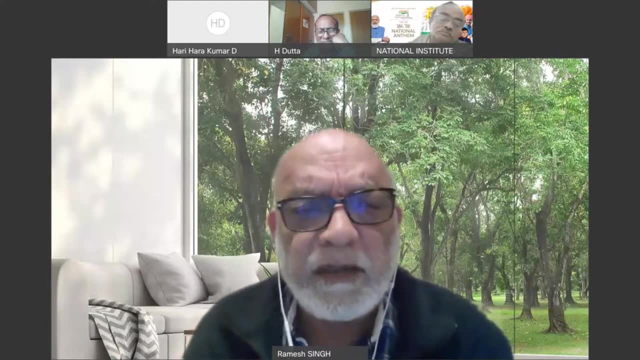 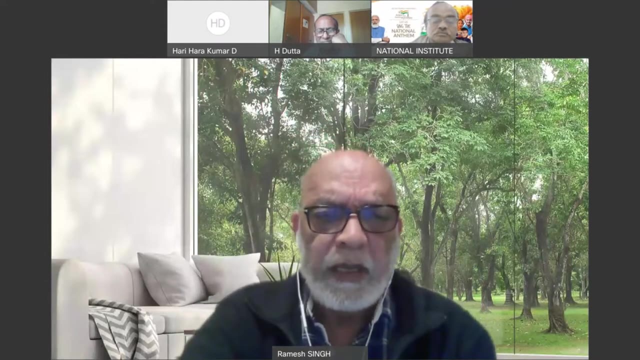 And we should not go to the press or any media. I know that there were people. they went to the television and they say, oh, tomorrow at 8 o'clock there will be earthquake in India. And they were behind the bar in India, you see, because there was no earthquake. 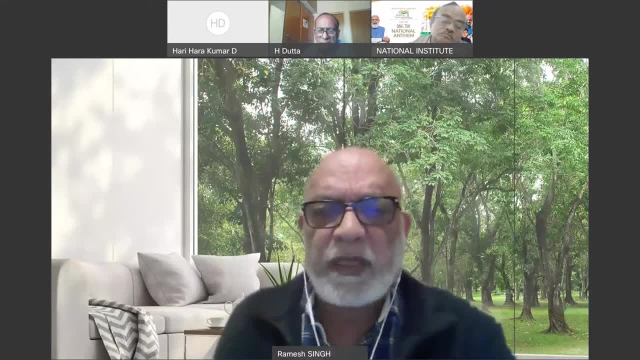 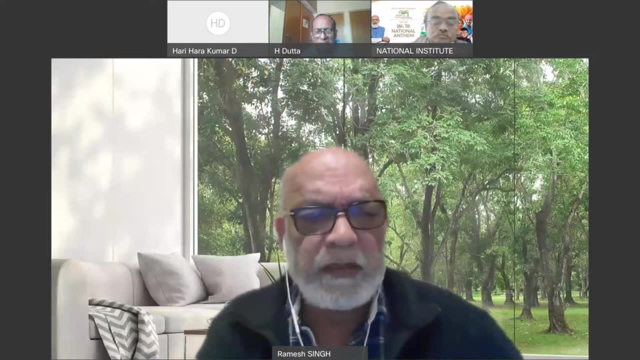 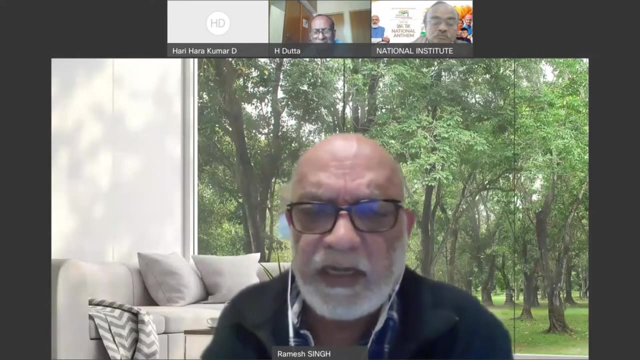 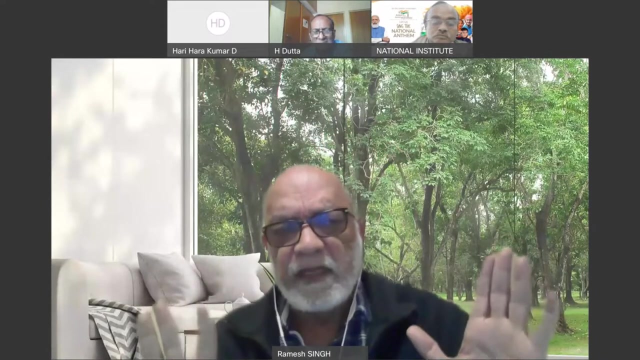 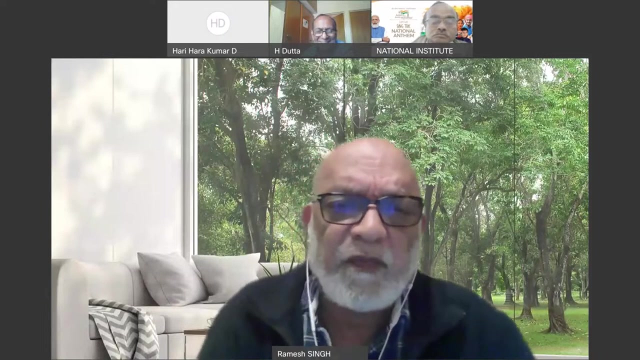 So precursory studies, of course people should study And whatever. And then, like Puranchand Rao, he said there about the animal behavior and other things And I also got very much excited- I put eight rats in the biology lab because the earthquake occurred in California. 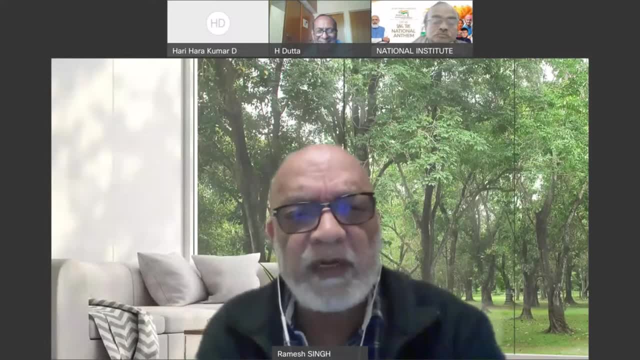 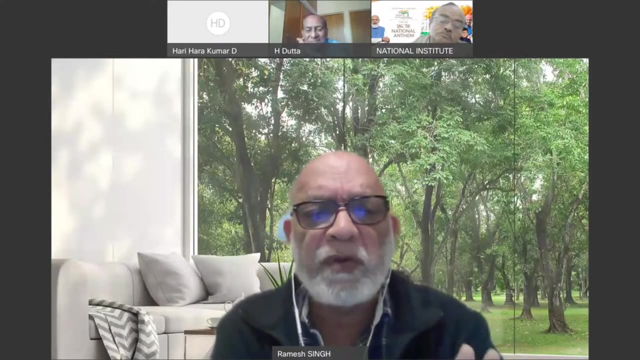 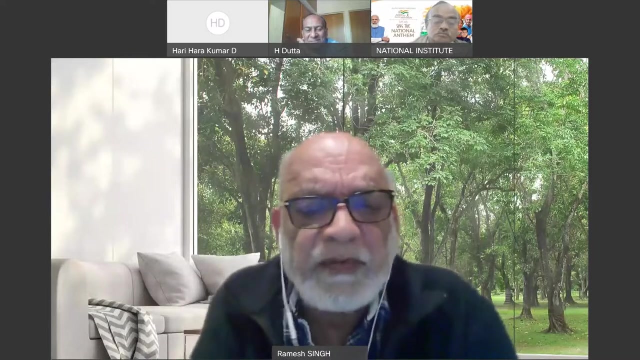 And then I found that even the rats started cheating us. Okay, And then there were so many people they published the papers on the animal behavior and the. I started saying, no, we should not do that. Okay, So there are people they try to do and whatever the Dr Datta you said, they quick what? 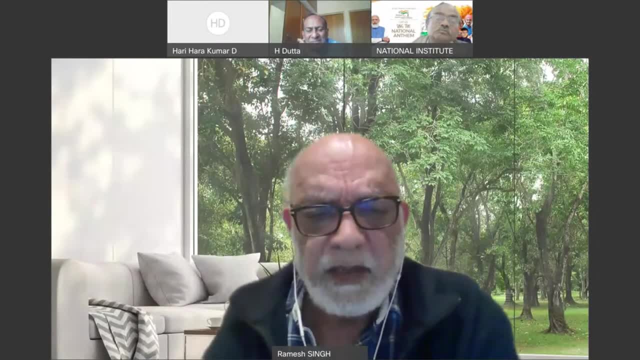 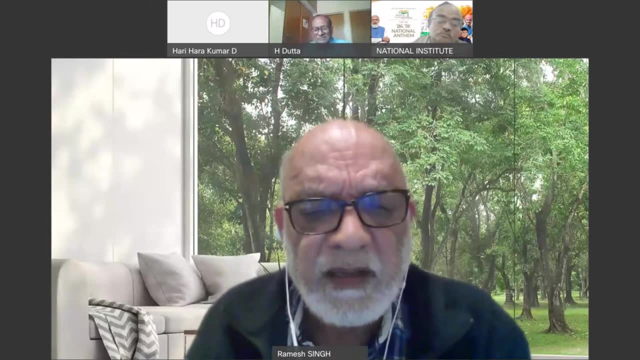 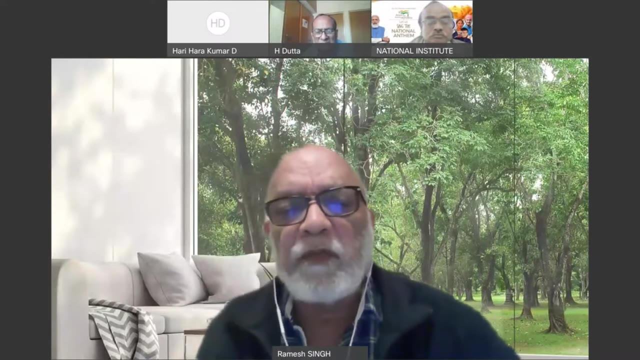 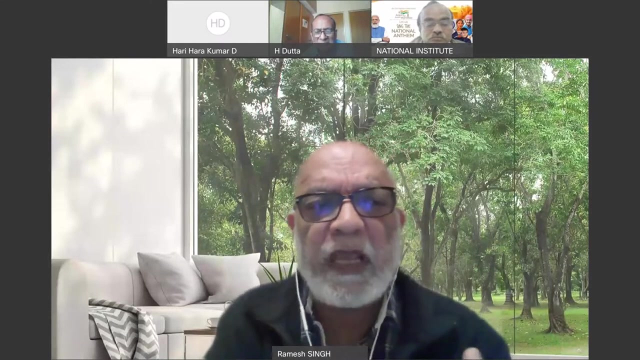 is it? They are my good friends, Okay, And they? nothing is happening, They are, They are really. they don't have money to do anything, Okay, So the I will discourage the young people to do this And whatever the? Puranchand Rao also said that there is the P wave S wave on the basis. 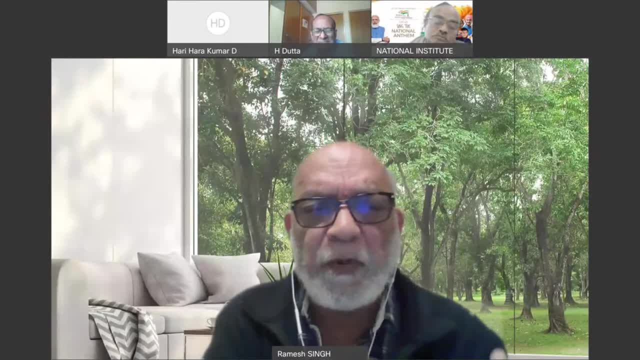 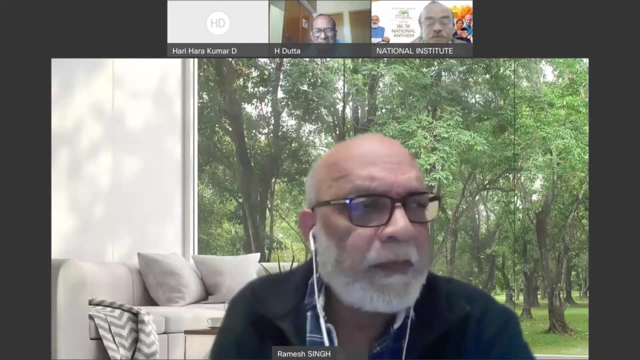 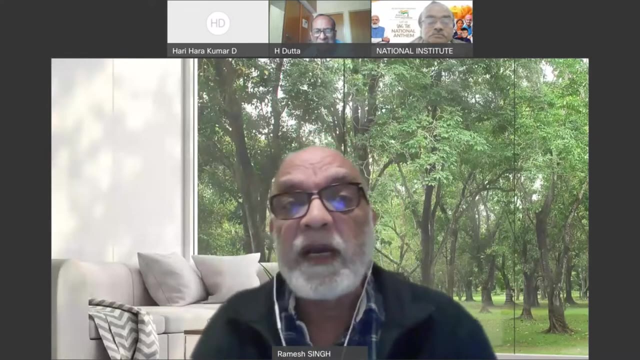 of the P and S wave. DST is supporting some of the proposal And a California event, The, the, the, The Stanford colleagues. they have developed the alert system So that may work. The signals: they show promising results. There are people working. 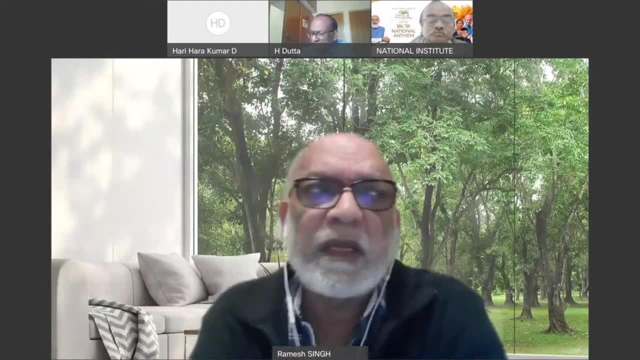 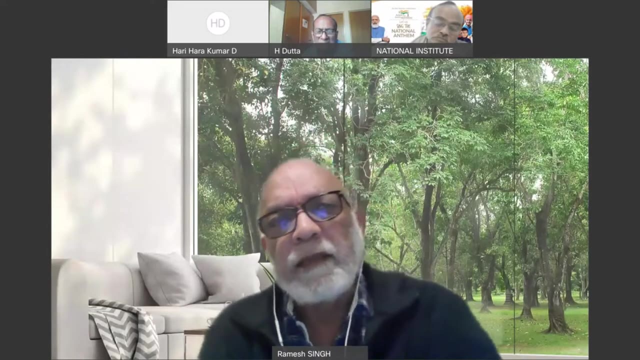 So we should, without money. if we can do that, then fine, Okay, But I would not like to encourage young people to do that, Because the earthquake is very, very complex. Okay, So the, the so these are the stories. 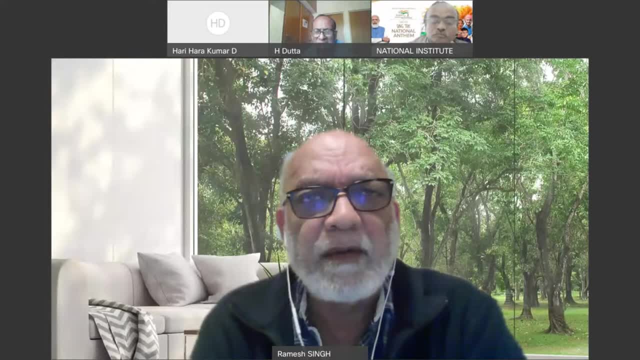 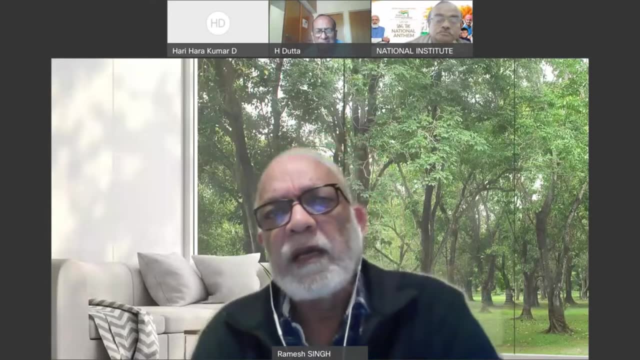 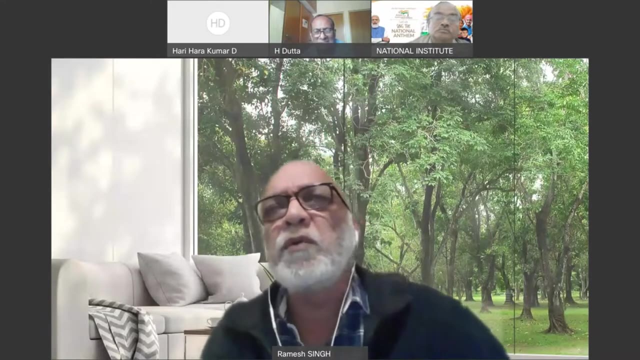 And Bhuj earthquake is well studied. Okay, And even in the Bhuj 2001 and 2003,. I had organized the conference in which I invited Dr Datta And Dr Datta said: no, I do not want to. I want that you should not publish my abstract. 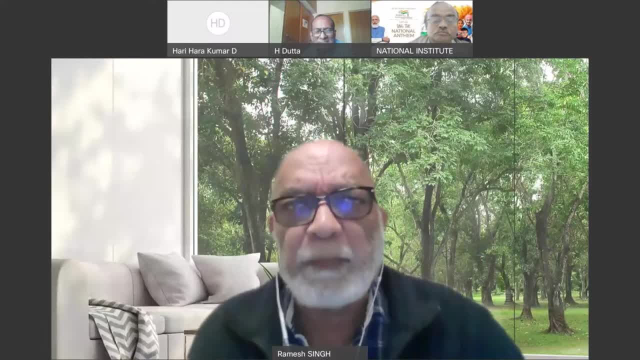 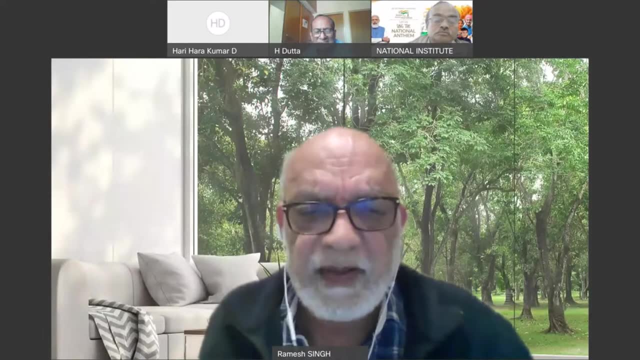 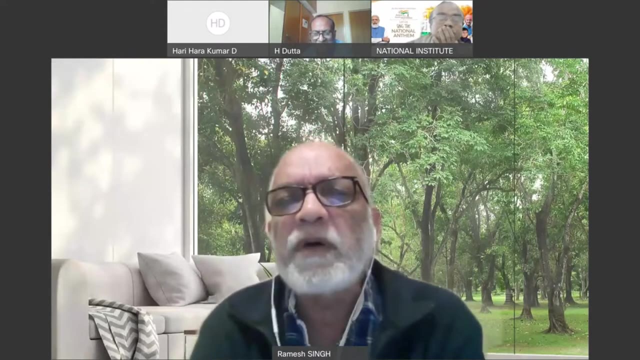 Because they were. he was going for patent And the patent. if you present that to your work, you may not get the patent. Okay, So I would like to say that this is a very complex thing. The interesting problems of the precursor studies. 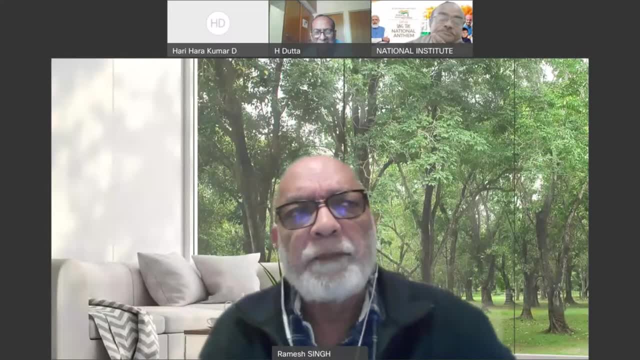 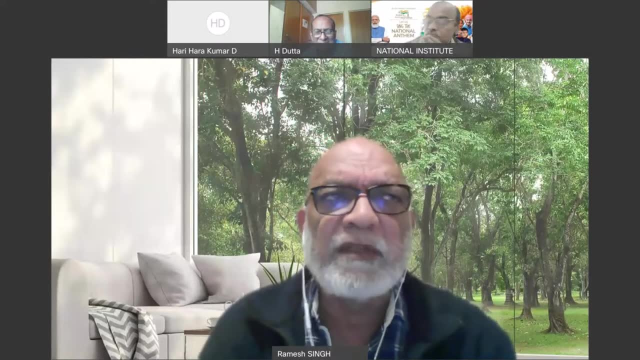 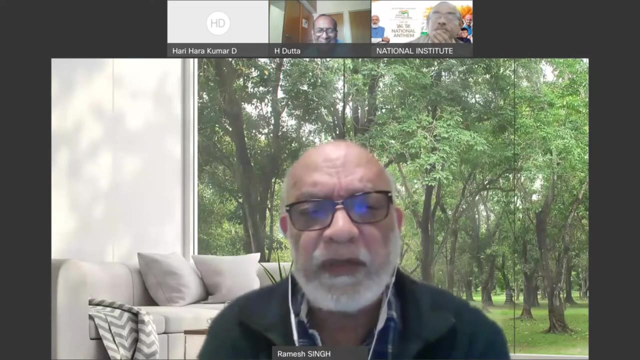 Okay, And one should try to become orthodontist. And here in US if you go to the doctor, They they will not prescribe any medicine unless they would like to see the blood test, the urine test, the sugar level and other things. 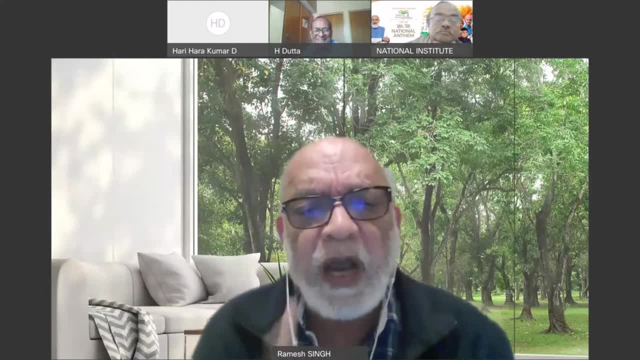 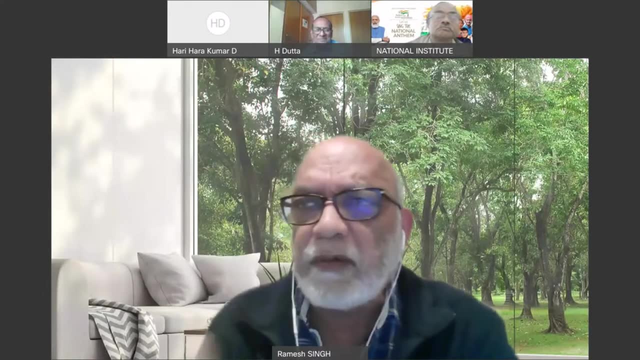 So let's become a good doctor, Okay, Orthodontist, And try to try to try to monitor all the parameters. integrate this, Okay, And I'm running the journal. I'm the associate editor of the International Journal of Remote Sensing. 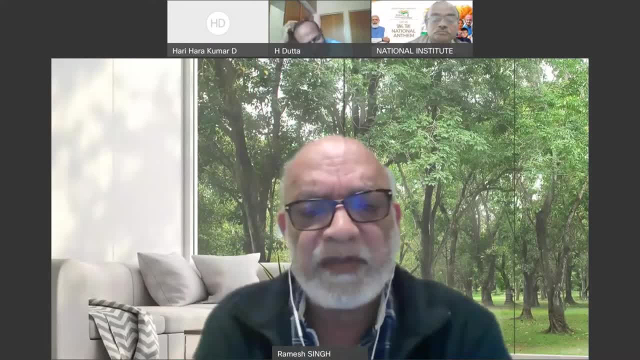 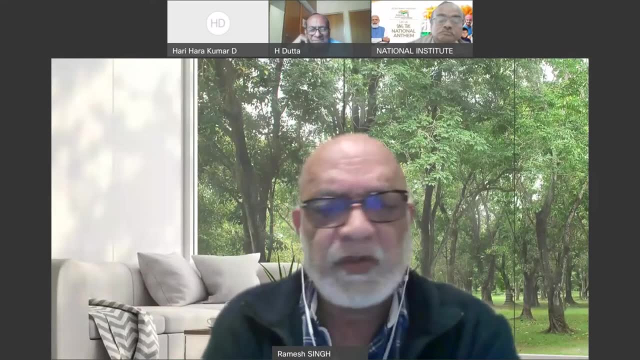 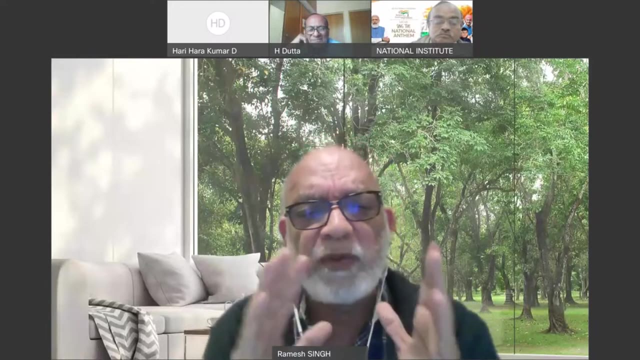 I'm in the Geomatics, Natural Hazards and Risk Journal, which is the 12th years, Okay, And there are so many papers people they submit And we return that because we would like to integrate this, Okay, So the output- precursor studies- is very, very complex. 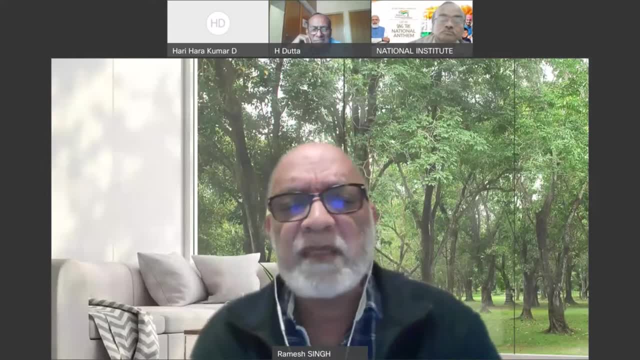 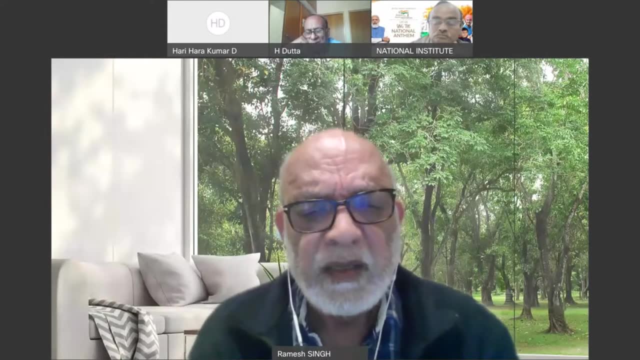 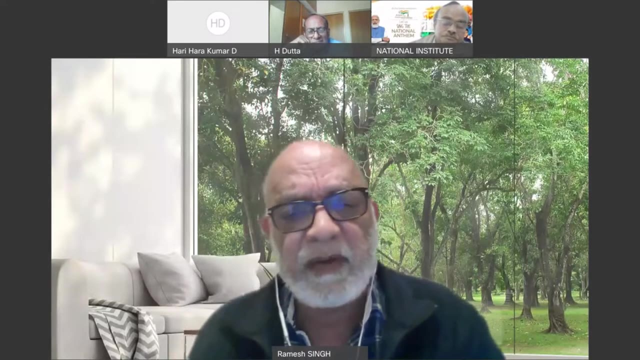 Okay, And let us not ask money. We should try to do. There are so much data that are available. Okay, We should make an effort. And even the water level is giving good signals, Okay, So there are many, many parameters. 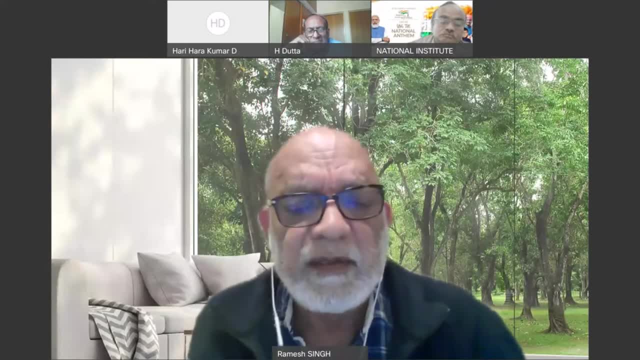 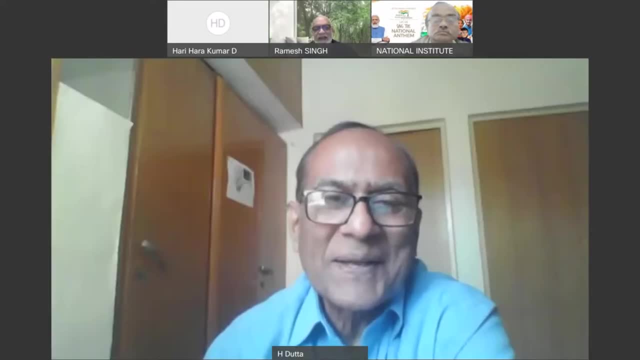 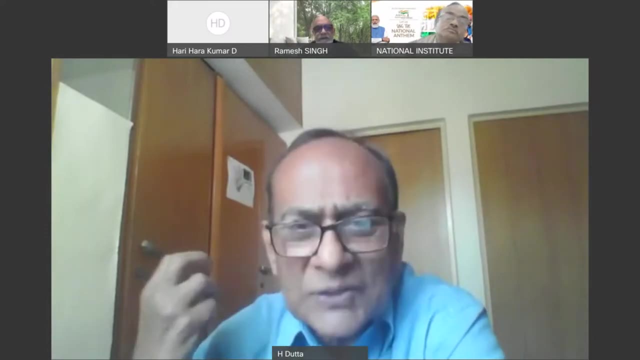 We should try to integrate this. So I'm sorry to disappoint you, Dr Datta, Okay, No, no, sir, It's a pleasure. I mean, unless we have what is called, what is called diversified brain, diversified views. 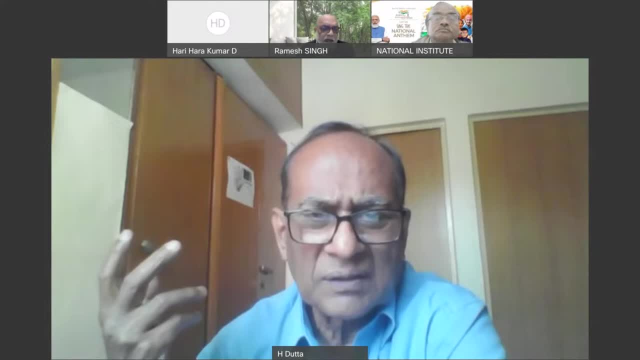 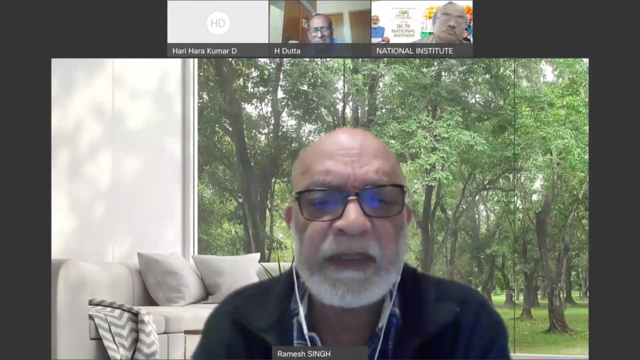 the progress cannot be. I completely agree. I completely agree. And we have spent a lot of money. DST has spent a lot of money And Birbal Singh, he put antennas in the Agra. okay, ground measurements and other measurements. 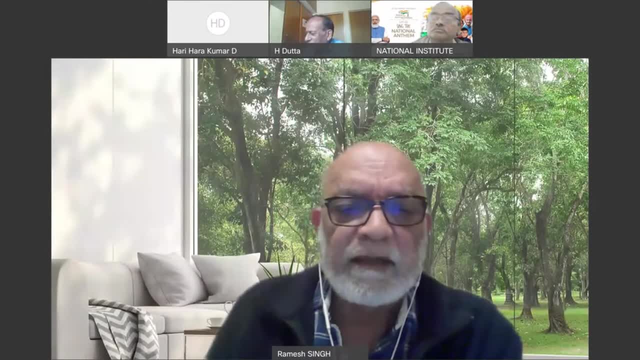 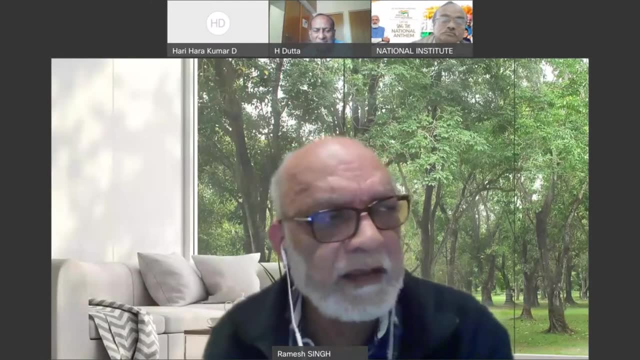 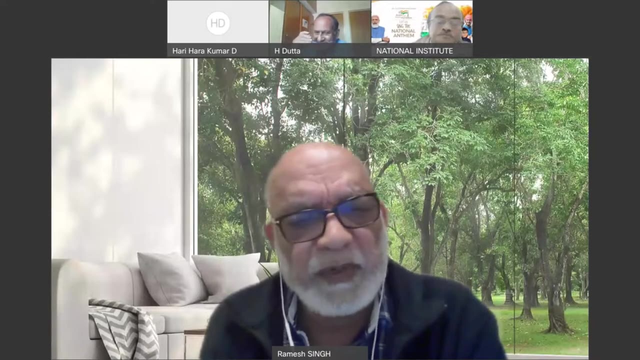 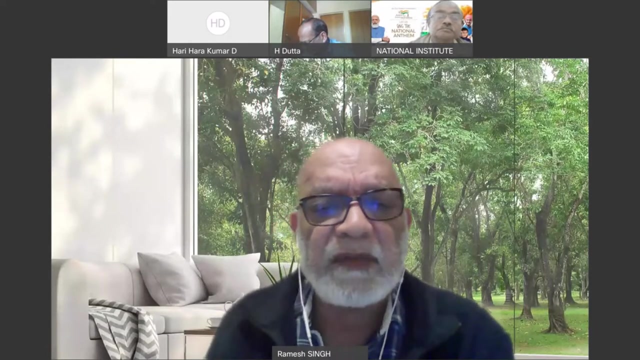 Okay. So these are the a lot of problems. So the young, younger lot like I would not like to encourage. Okay, And there are so many observatories. We have multi-parameters observatories are operational, Okay, Since the last five to 10 years. why not? 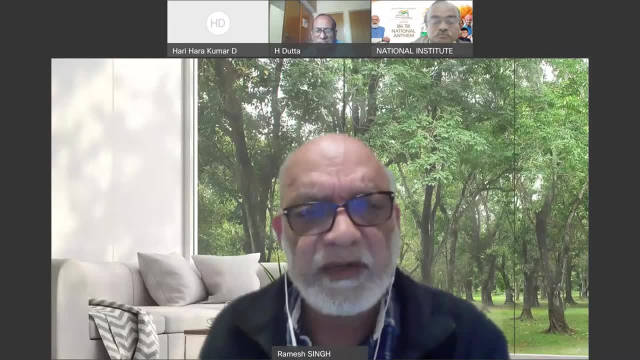 We should try to analyze this, build it, Build up these statistics. Okay To do that. Okay, So thank you very much, Dr Haldar, for giving me a chance to express my views. Okay, Thank you Okay. 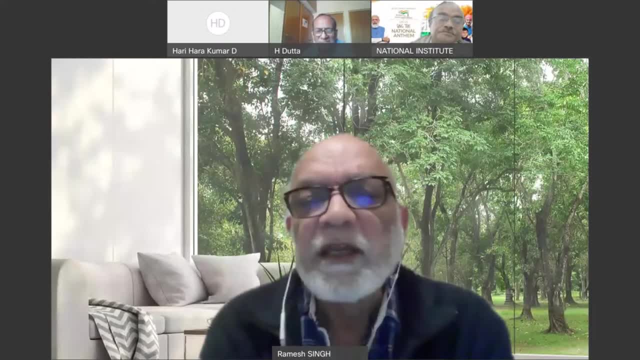 We have noted your observation and it's a great views. Of course he told what are the demerits and merits of that. It is a it needs integration And first data is available with us and it should be analyzed. But of course he has said that it needs integration. 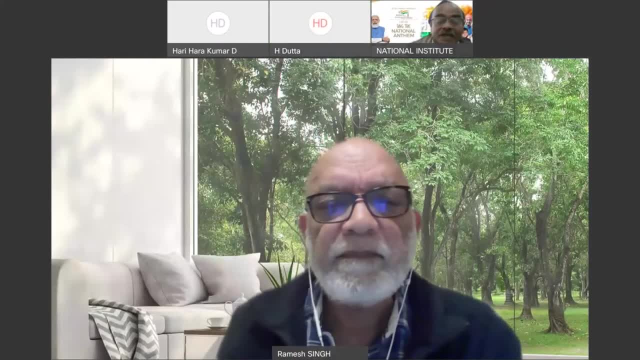 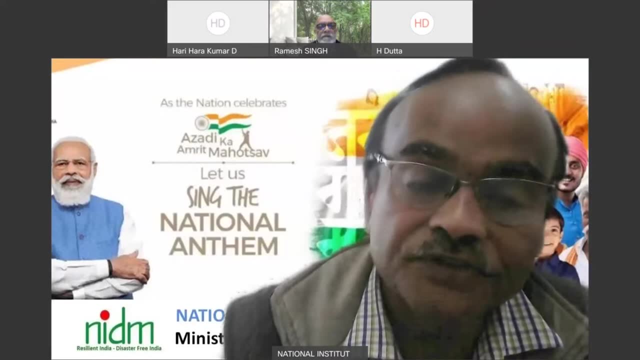 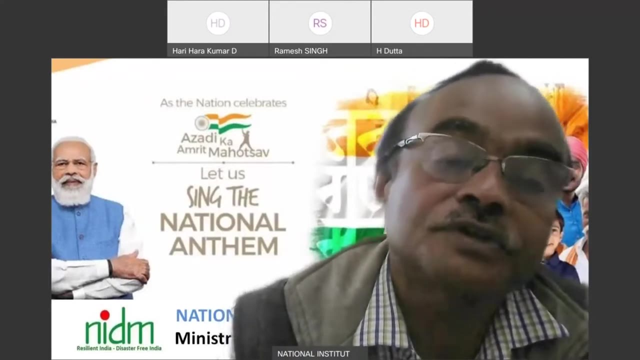 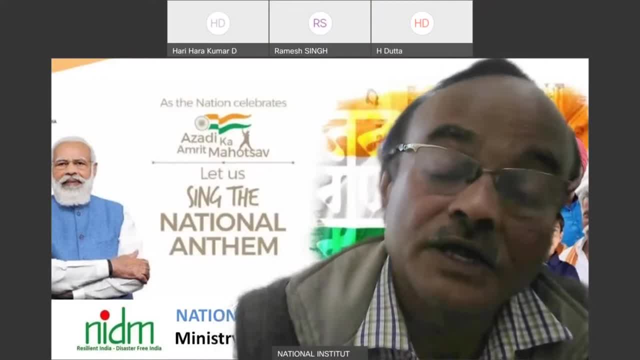 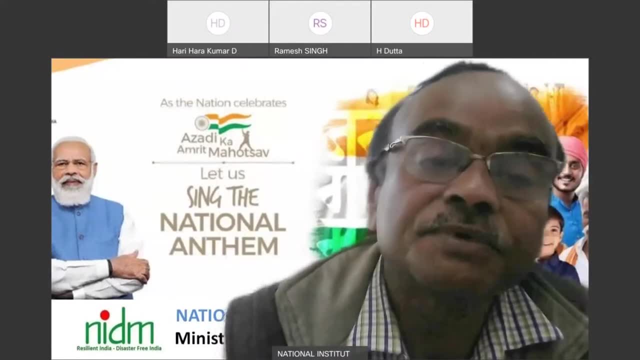 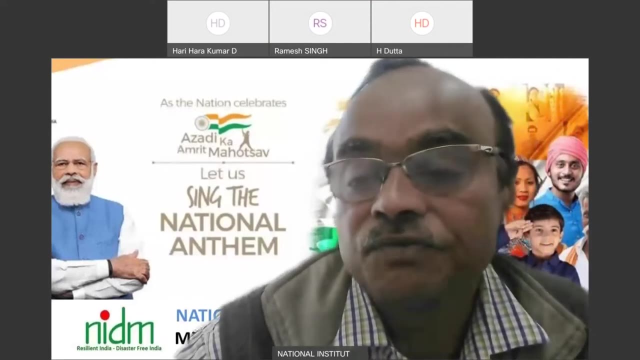 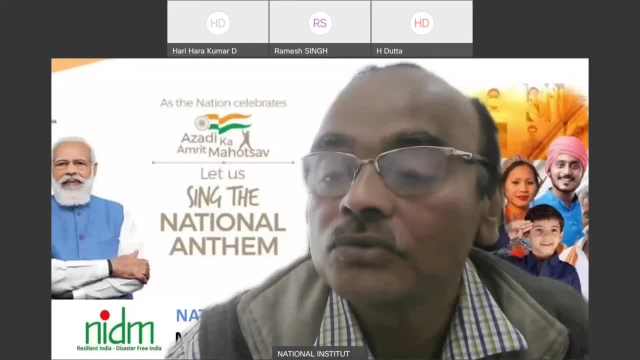 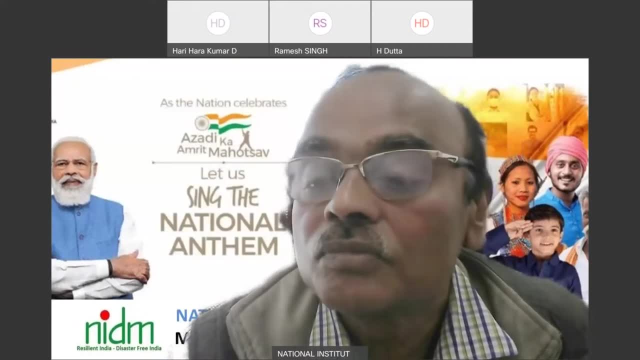 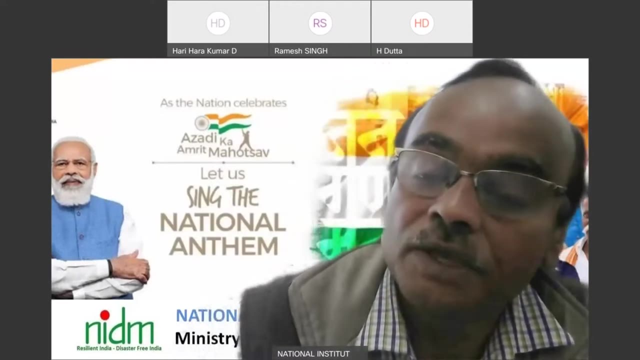 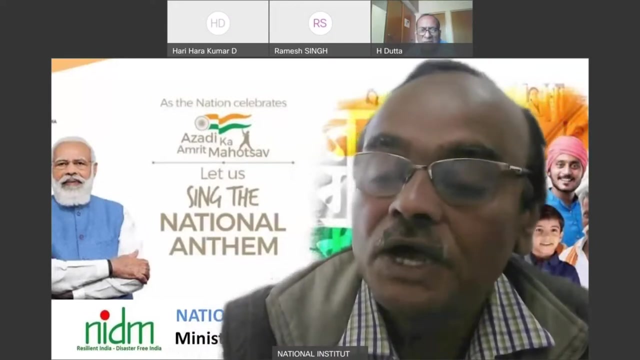 mit Yoshihri recovery. Thank you to once more. okay, doctor, sir, so far i could not find any question. everybody has praised for your work and what you have done for india. that is there. if at all anything will come, i will. i'll let me let me know you, and it will be vis-a-vis. after obtaining the answer from you, i'll post. 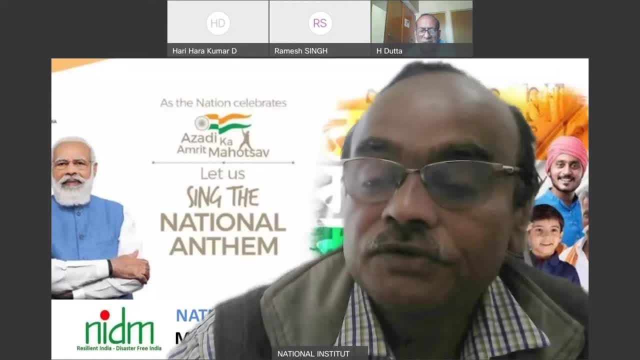 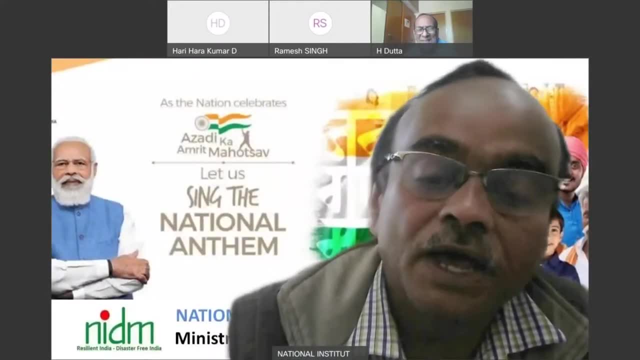 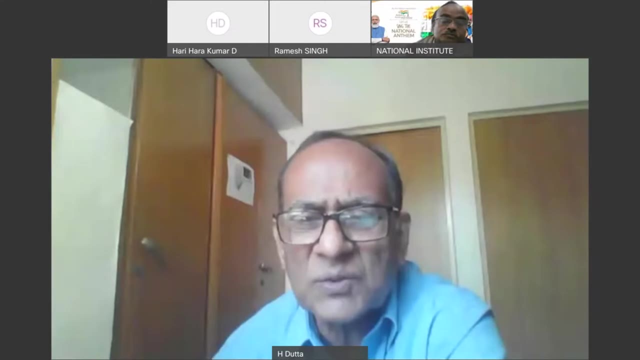 the things to the concerned participants. yeah, yeah, yeah. so i should appreciate that. you have done excellent work for the patent you are working on. the question is, yeah. so unless that, yeah, see, when you are fighting a war at the global level, you also understand? how do the, how do the human? 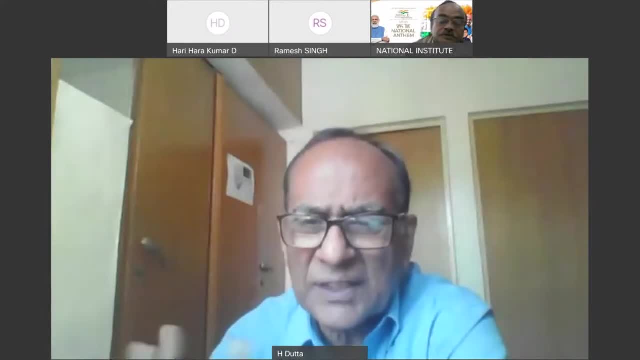 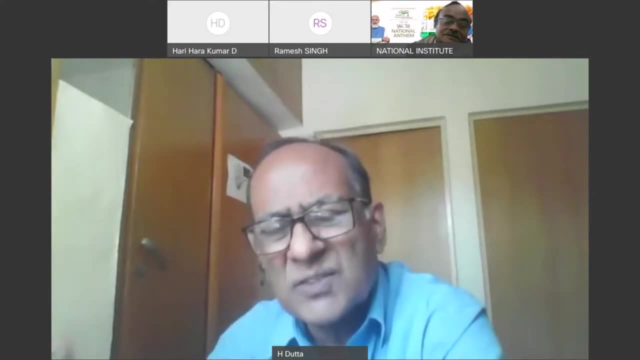 mindsets. you know they react: yes, okay, yes, that's very important. you see it, it teaches you a lot. and then you find that there are a number of unanswered questions which need to be solved because, ultimately, the mobile which we have today in our hands, it is an obsolete. within six months there is another version, so we 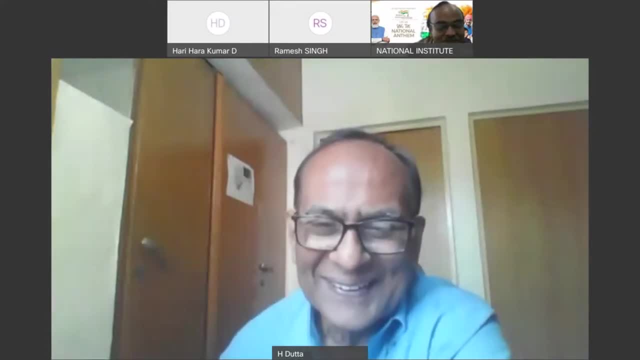 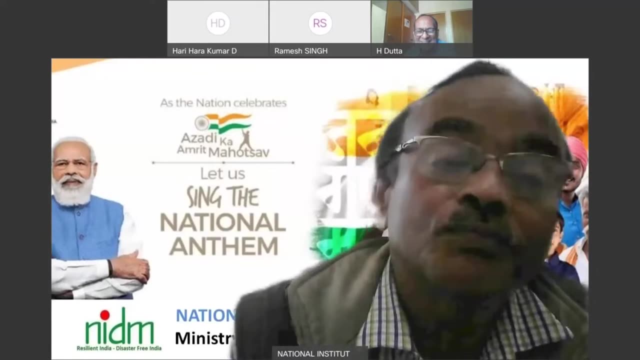 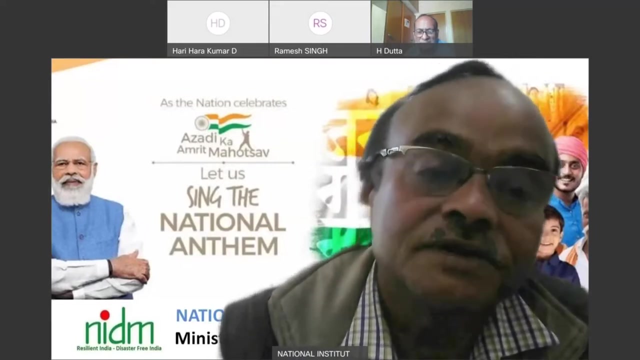 need to have. you know the changes and we should congratulate you. see it in india. a lot of persons are there. it is a 130 or even more. now you cannot answer each and every person's or that. yeah, but of course it is flourishing your patent. i should appreciate for that and national knows that what? 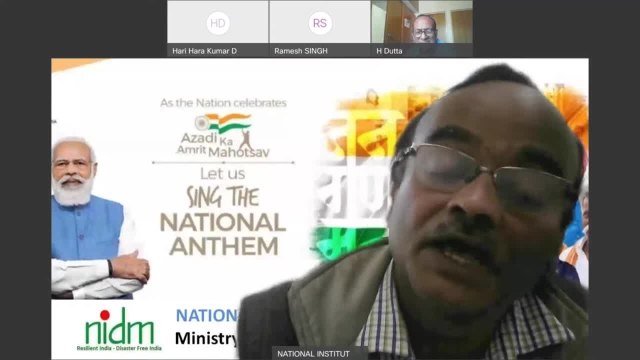 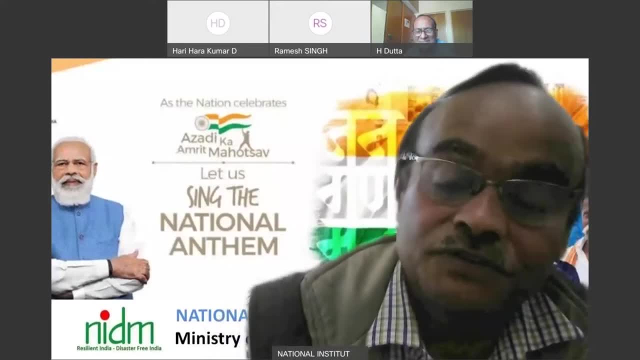 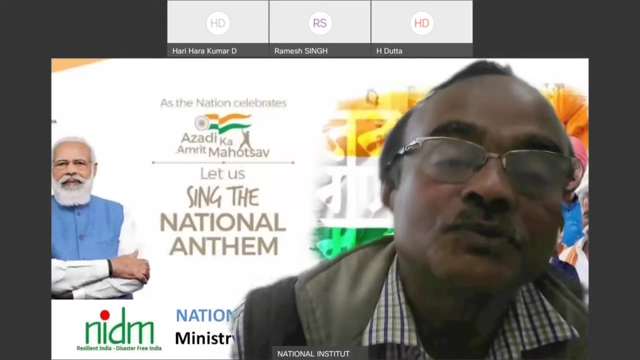 is your contribution for the recursion and i should appreciate for that and obviously you have given an excellent time precisely you have explained your work that i should thanks for that. now this with this, i'll put again: thanks to you. now, as a customary, i have to put my vote of thanks. 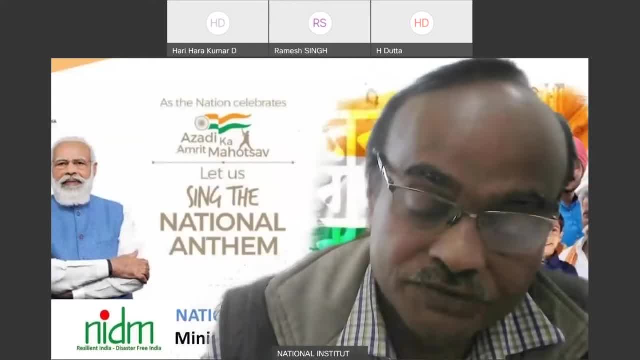 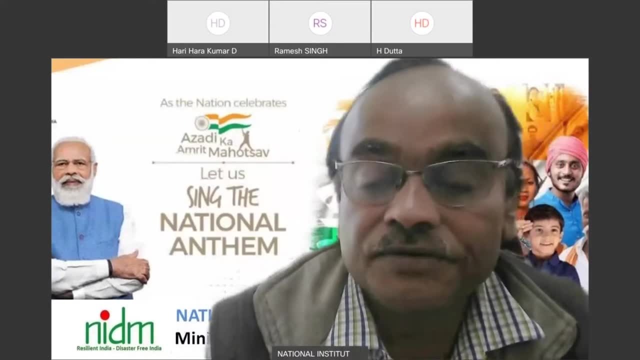 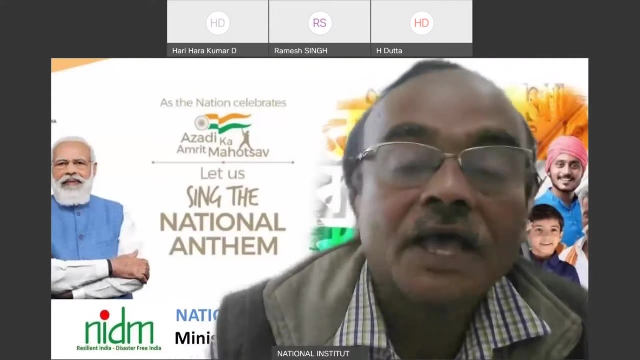 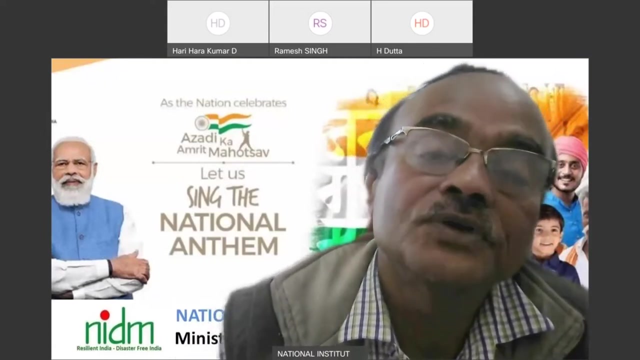 in this session now i in this uh that our executive director, uh ips, mr taj hassan. he has having he had put his great support to each and every individual speaker and also our these faculties to conduct this type of webinar and training, and it should make the public for awareness, for the preparation, mitigation. 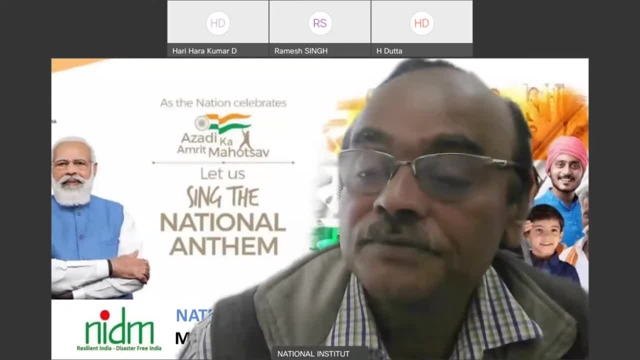 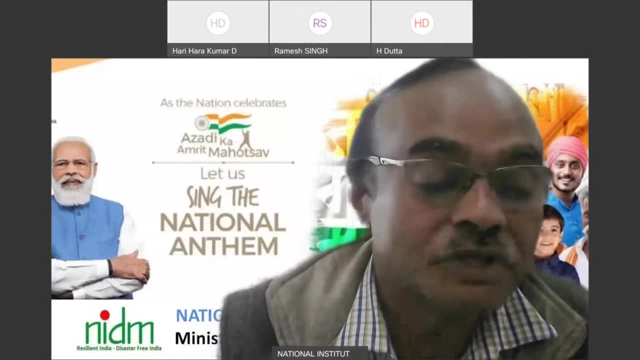 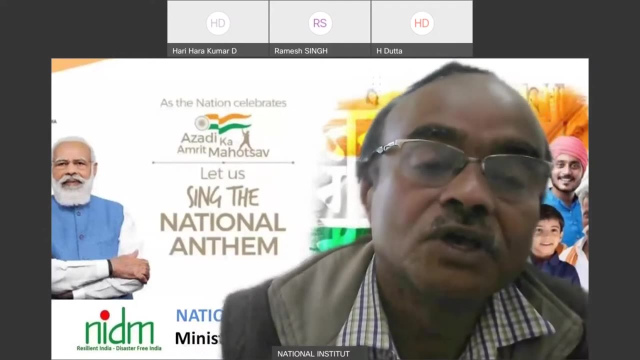 and what are the uh, what are the things for forecast there? he has used to support all the times. now our next two is our head, professor suryanos. he's always there to make the program in success and to support even. he is busy all the times for different programs in a day. 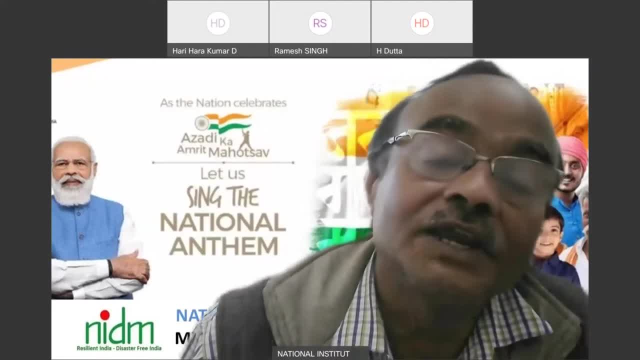 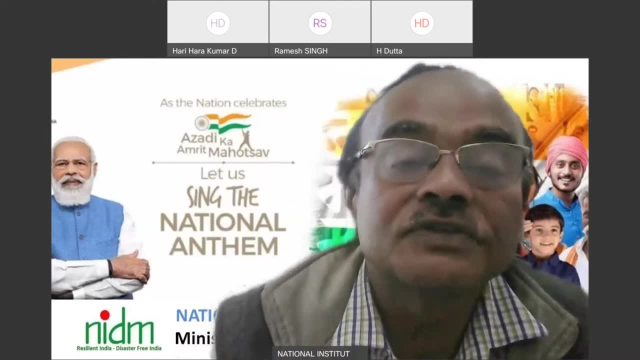 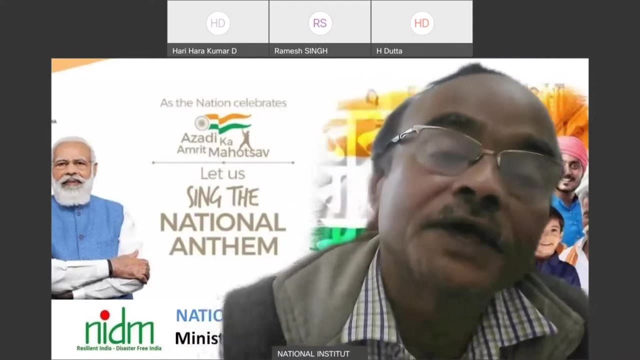 randomly. programs are there from beginning to evening, but still he wants to put his time for uh, to put support each and every faculties. so for that he has supported us also and in the past in it is there. So I put my heartfelt thanks to Professor Suryaprakash. Next, all the 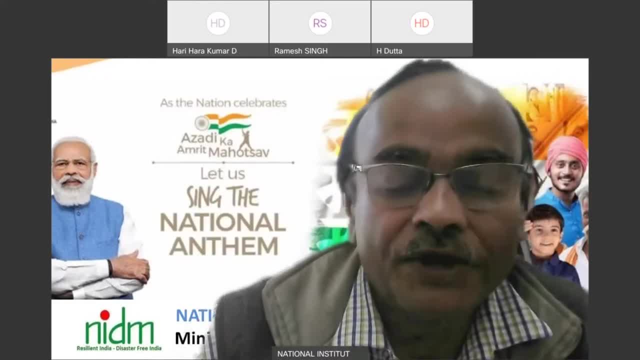 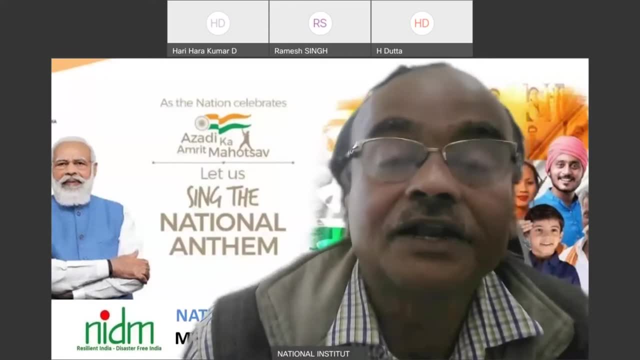 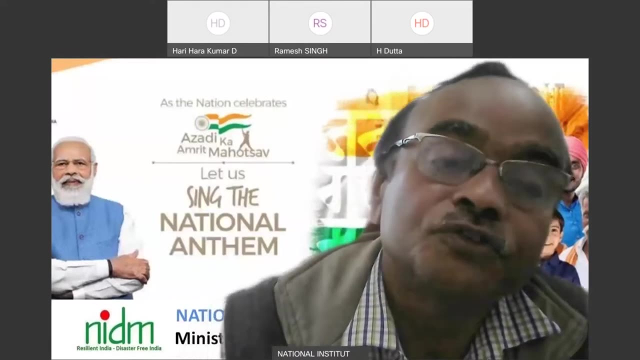 both the speaker, that is, Dr H N Datta. he is a quite senior man and he is working in this Antarctica. Of course he is not professional seismologist but still he is having lot of knowledge and lot of things he want to do in seismology also. So this precursor also. 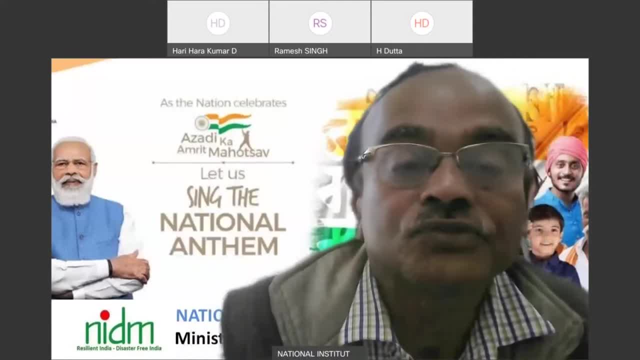 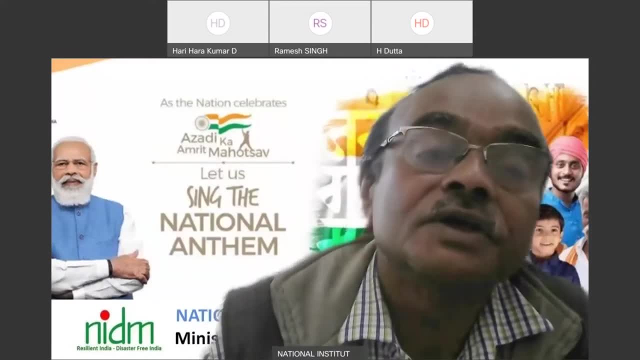 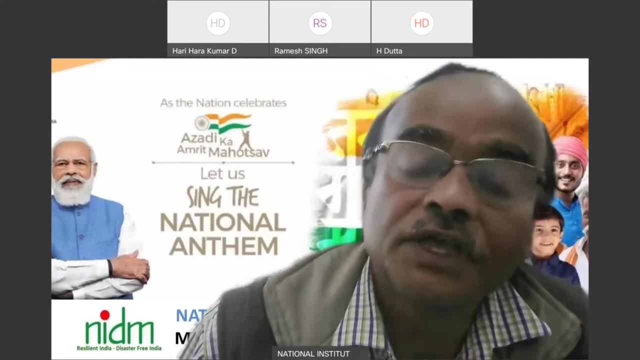 it is a good effort he has done. I put my sincere thanks to Dr Datta. Next is Dr P C Rao, Kuran Chandra Rao. He has given a very knowledgeable- I mean that- description and lecture to, for the participant and for the faculties. also He has put his views for. 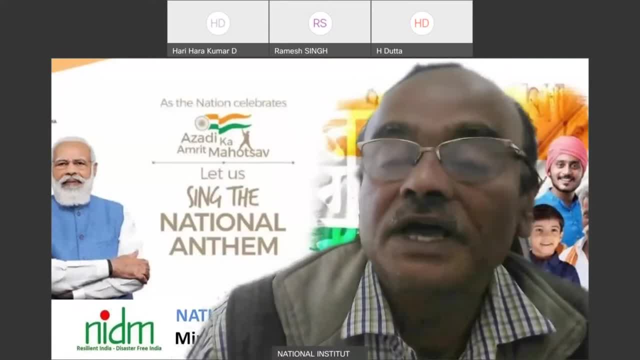 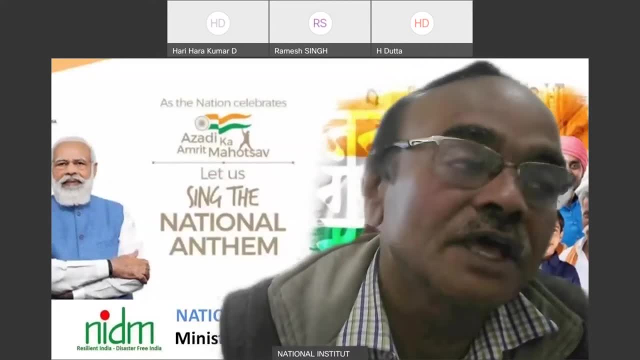 seismic zonation, microzonation in Jabalpur area and other area And he also told lot of animal behavior for that in precursor also And he has he told that it is a, it is an integrated thing for the precursor work work. 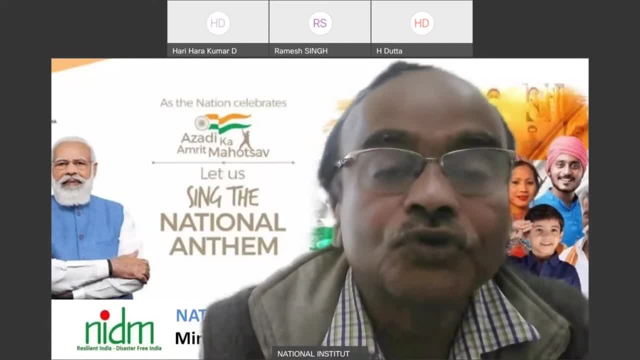 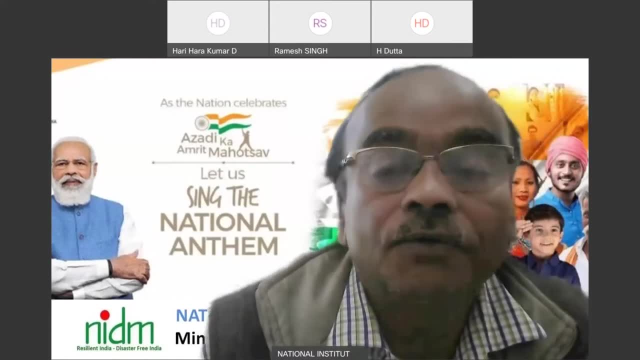 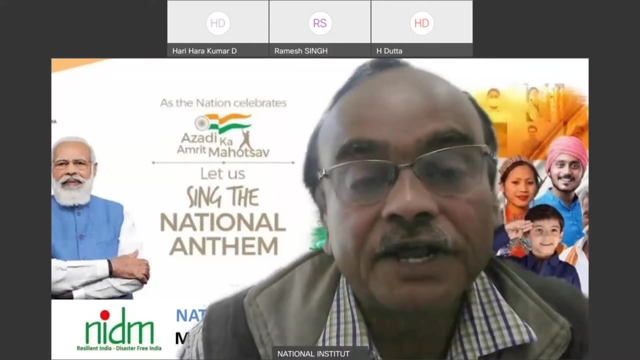 of earthquake. Now I put my sincere thanks to Professor, to Dr P C Rao. Now next is the our faculties who has joined, and Dr Professor Ramesh Singh. He has critically analyzed the seismic activity quite long time in India and abroad. He he had his views. 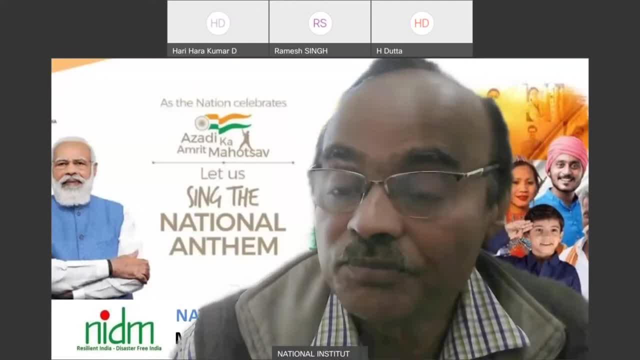 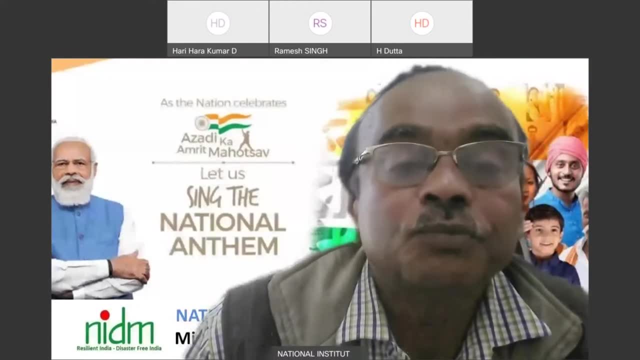 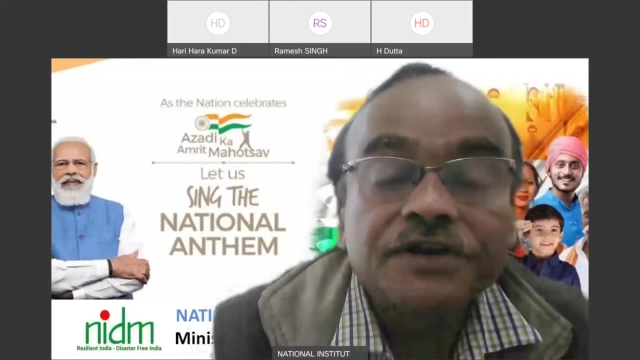 this Gujarat Bhuj earthquake and and other parts of earthquake. So he has critically analyzed. Still, he is having views for future also And I put my big thanks to Professor Singh. He has taken an interest to hear our this session and and he placed his observation. 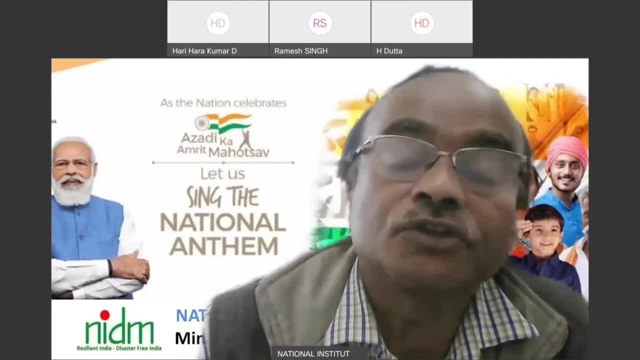 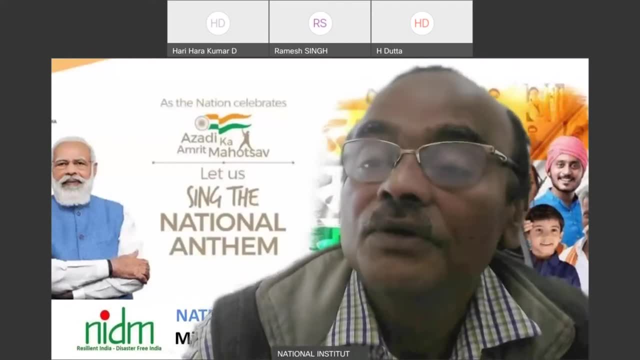 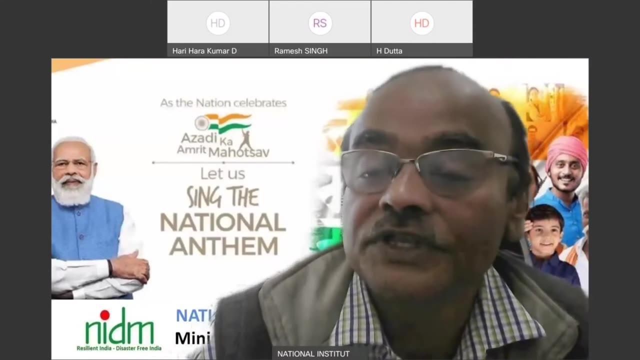 and comments. I I put my thanks, big thanks to him Now, the all the learned speaker participants Who are with us with the morning still in full swing, Geras, So they have learned, And within that, some professor also there they have put their, their comments is a very 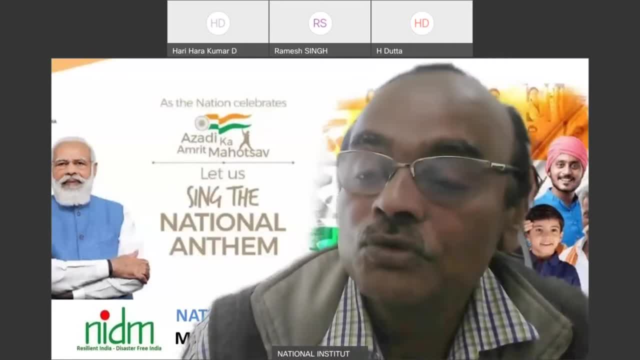 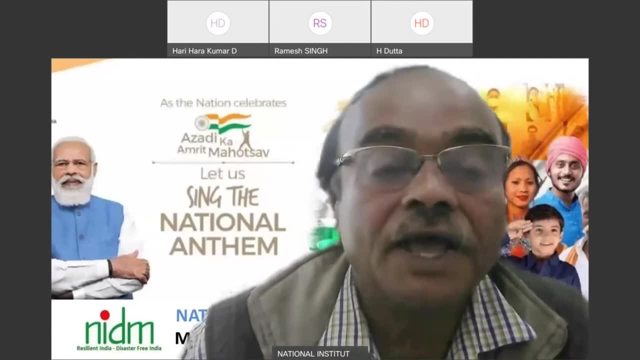 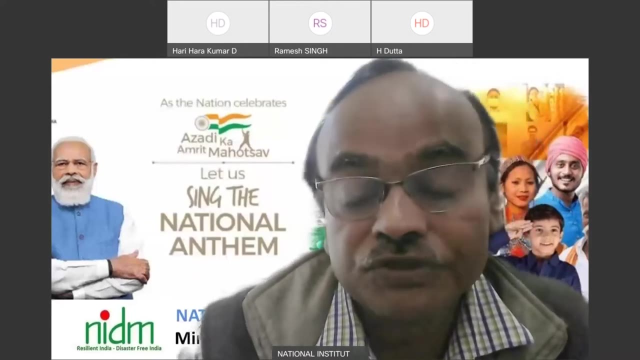 good things from the speaker they could hear And also- and he has given he told the NIDM is organizing nice themes and nice very efficient speaker in the in the particular or the relevant topic. So they have shown their gratefulness for this. Now I put my heartfelt thanks to all. 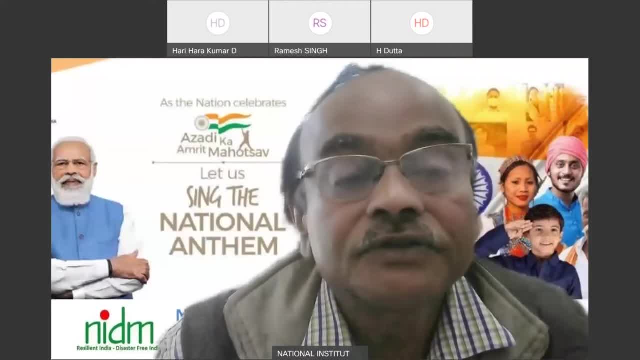 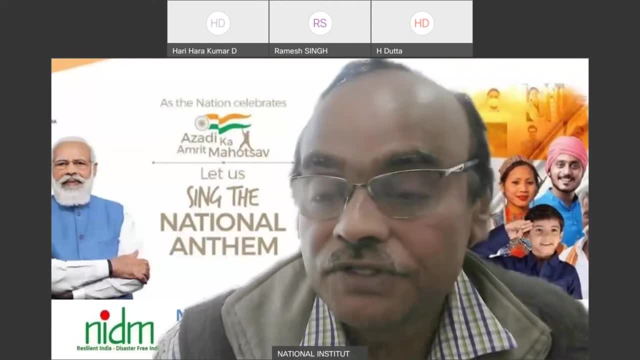 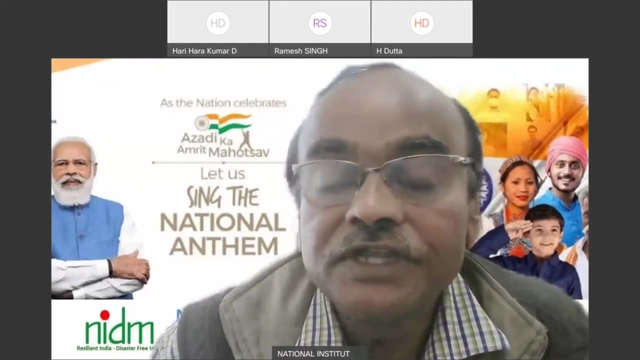 the participants who are joined and who has seen who has observed the speaker's address and our this, this Professor Ramesh Singh earlier he has also given lecture on that, So I put my very, very heartfelt thanks to all the participants. Now that IT team of 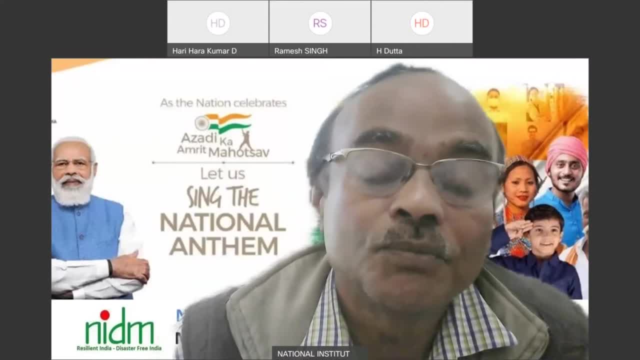